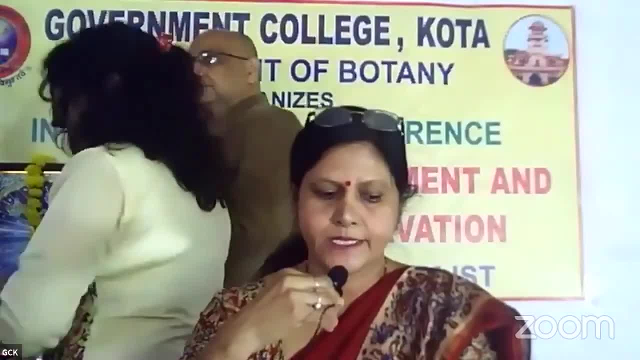 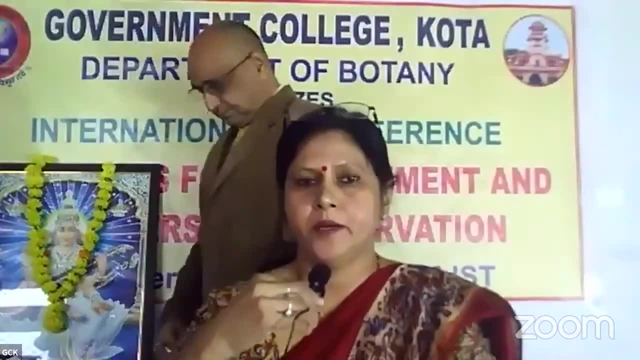 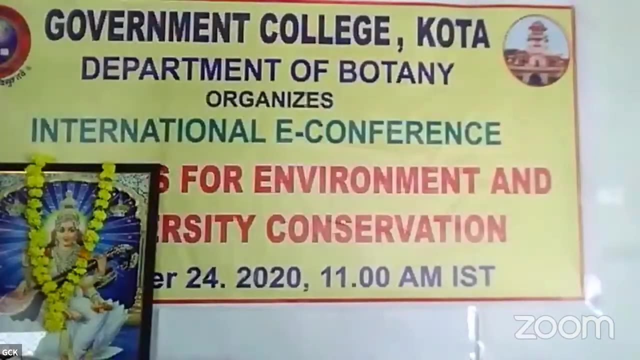 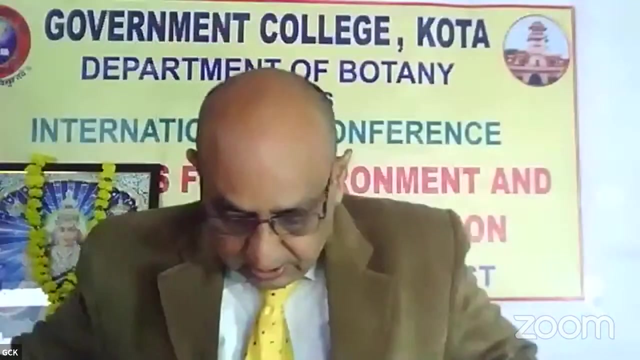 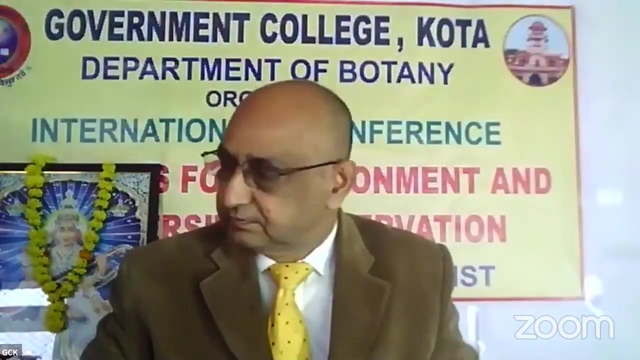 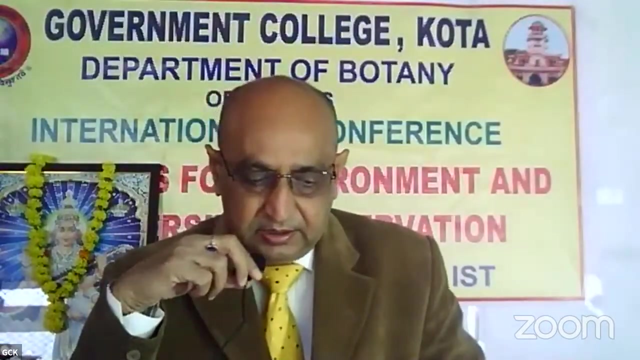 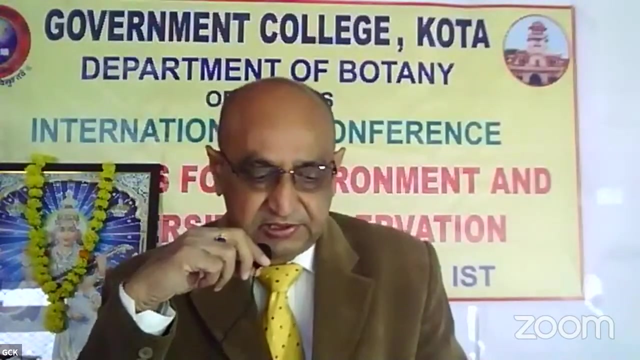 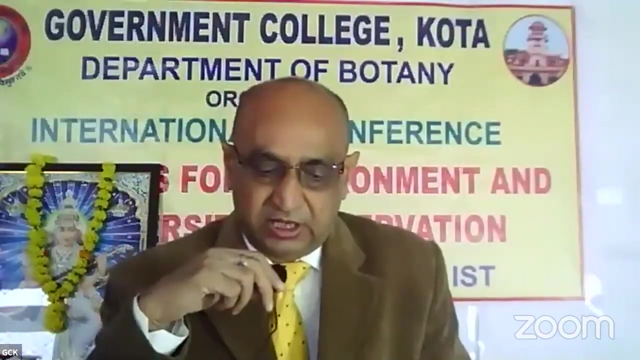 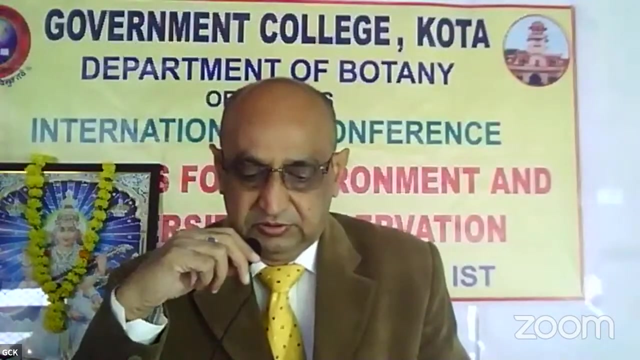 Deepa Jyoti Namostute. After that, I humbly request to respected Principal Sir for welcome address. Please join Principal Sir. Thank you, Good morning. It is my privilege to welcome our eminent speakers, Prof D B Khatka, Nepal. Dr Varla Andrew, Nigeria. Dr Prashant Singh BHU. Dr Avde. 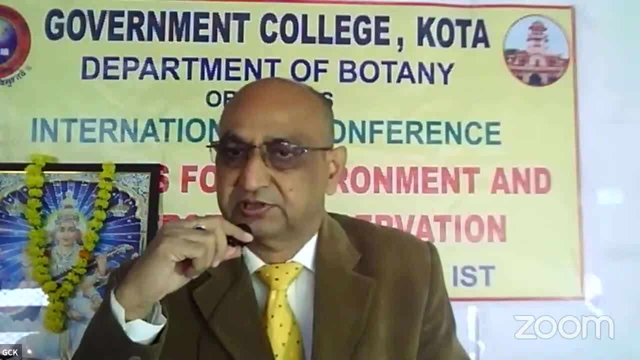 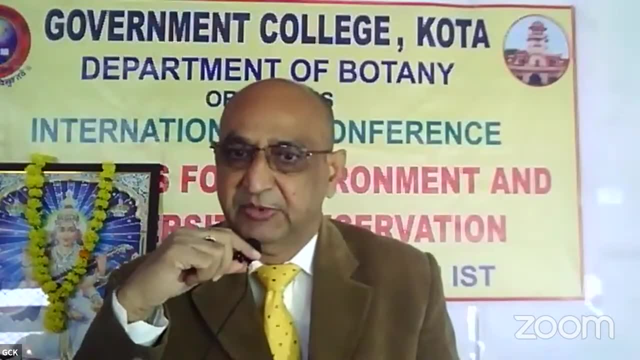 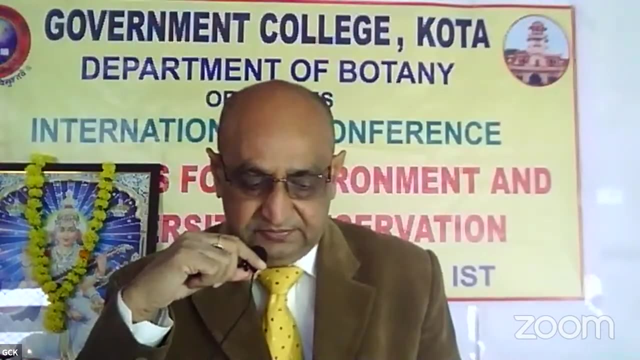 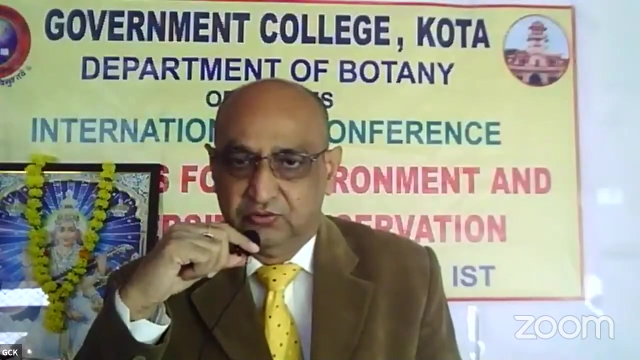 Srivastava Durga and Dr Sanjay Bhargava Kota, We are organizing International E-Seminar on Strategies for Environment and Biodiversity Conservation. This is again planned by Department of Botany, Government College Kota. 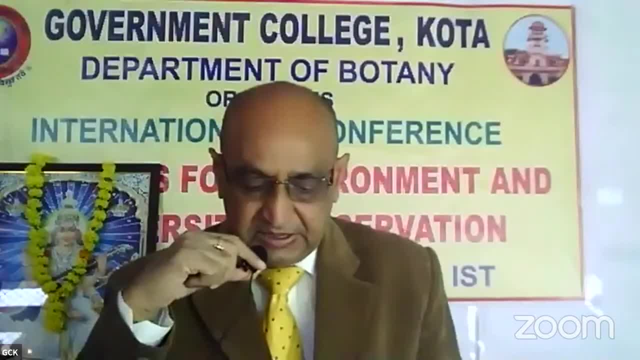 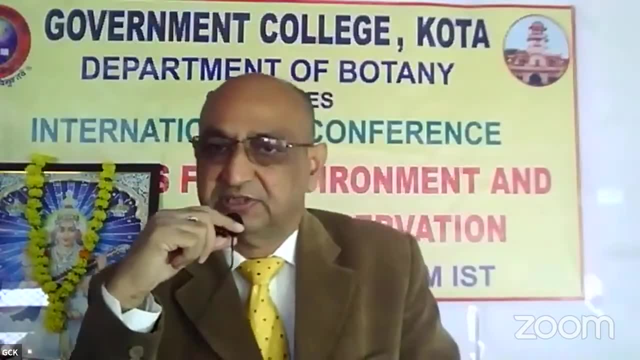 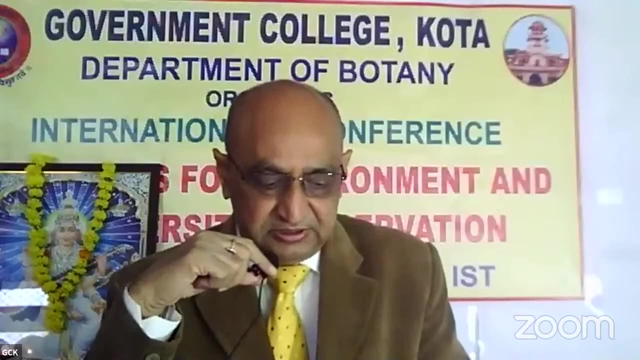 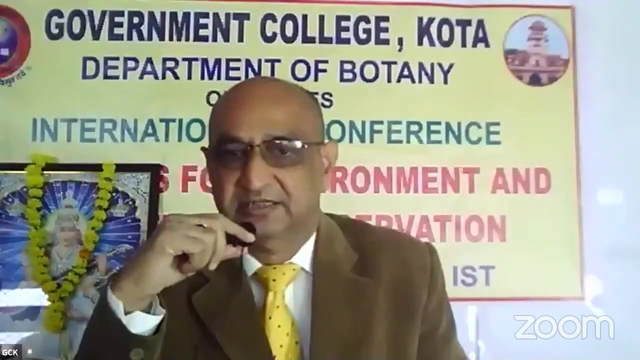 We are moving step by step. Earlier we had a national level seminar on Environmental Ethics, Conservation and Sustainable Development. We are now much more experienced, mature and sound with reference to our understanding of conducting seminars not only at national level and the international level. 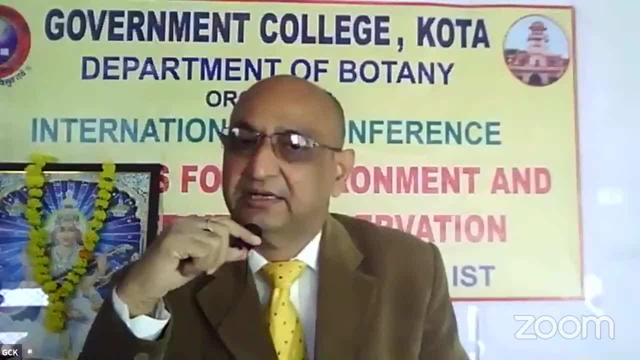 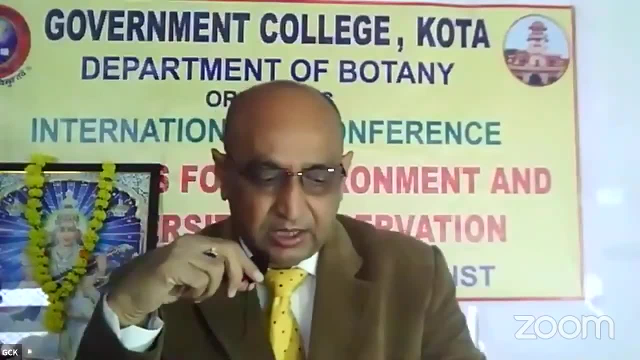 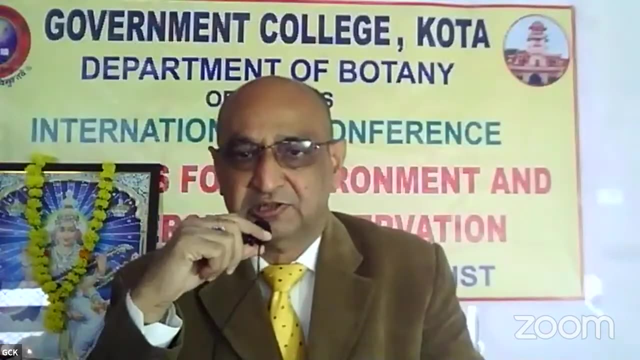 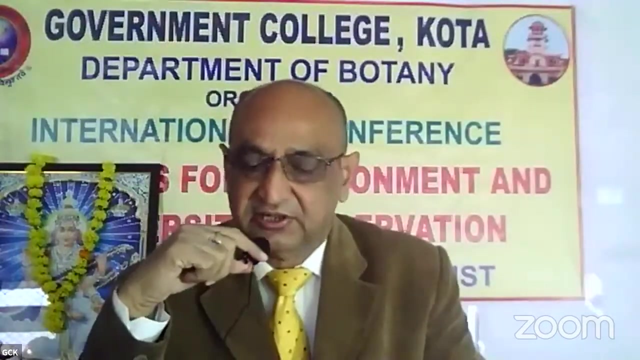 We are technically sound also, And we are improving day by day. I am a student of Science, and that too, of Physics. I do not know much about biodiversity. Even then, I try to understand it in a few words. Biodiversity describes the richness and variety of life on Earth. 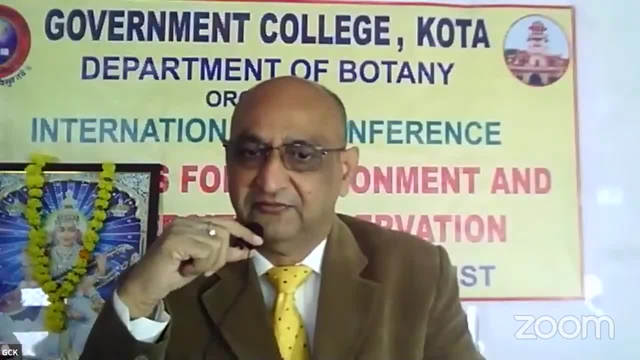 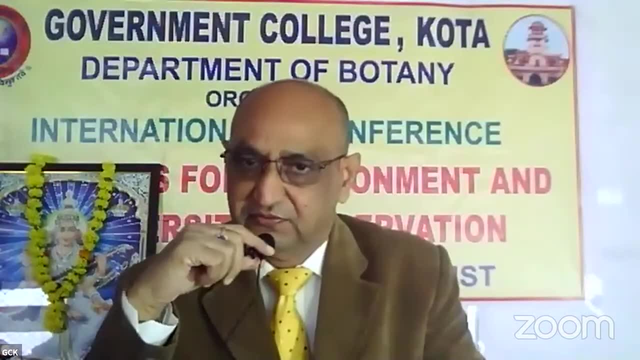 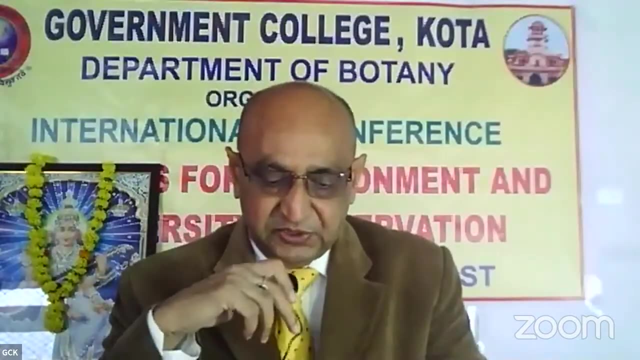 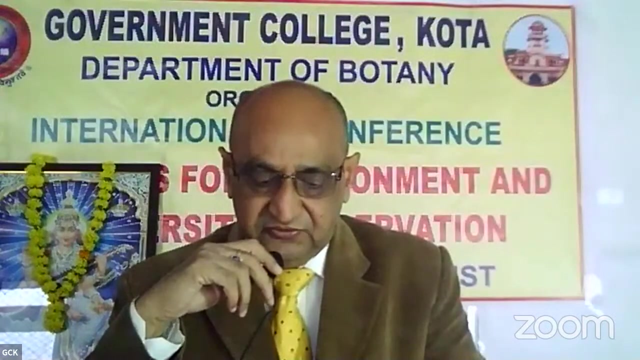 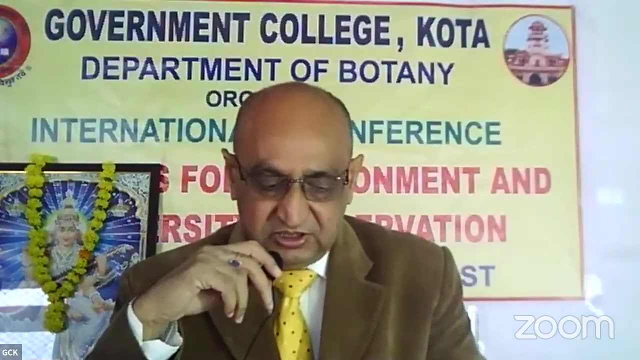 And this is the vibrant life on the planet. It is most complex and important feature of the planet. Without biodiversity, life would not sustain. Biodiversity preserves different cultures and spiritual heritage. Therefore, it is very important to conserve biodiversity. In few words, humanity is currently burning the library of life. 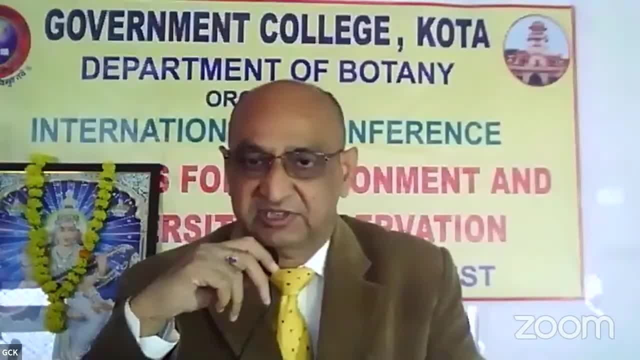 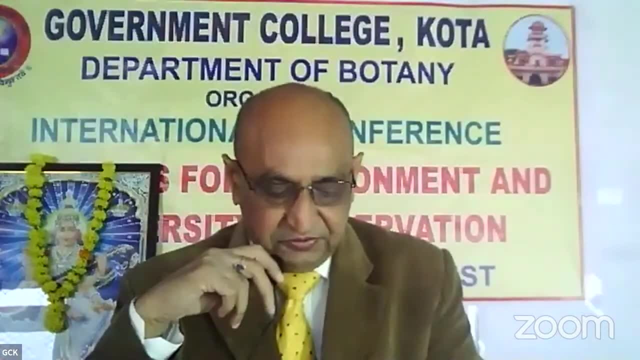 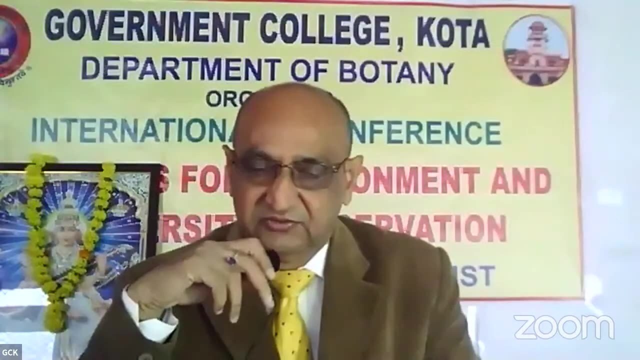 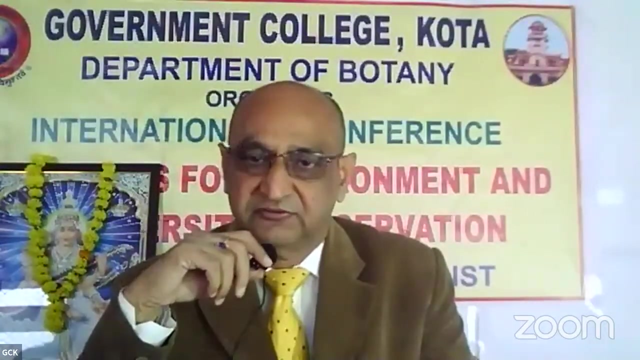 Therefore, to conserve biodiversity is the need of the hour. Biodiversity boosts ecosystem productivity too. Now a few words about college. This college is the biggest of the division- Kota division- Having 60 plus faculty members and 2500 plus students. 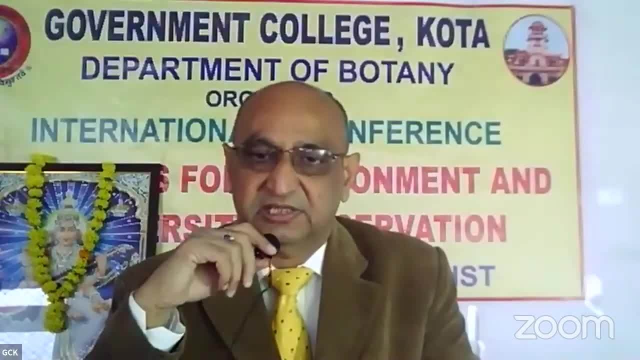 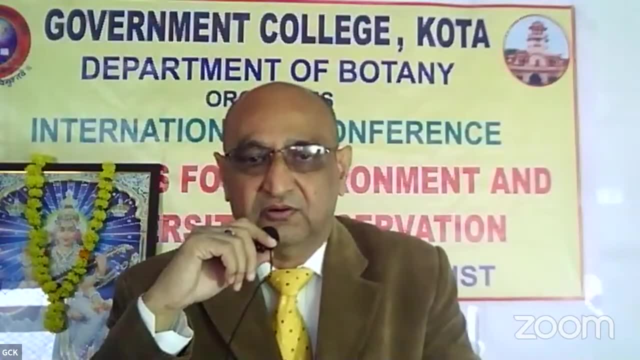 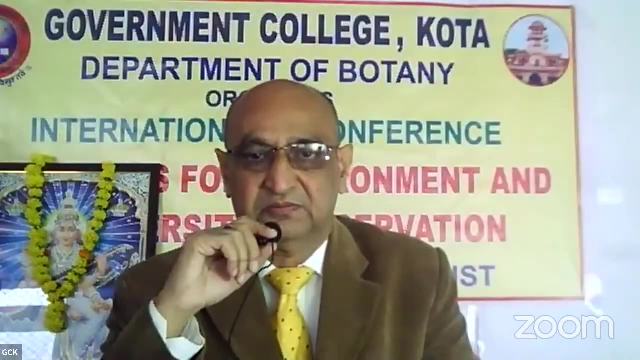 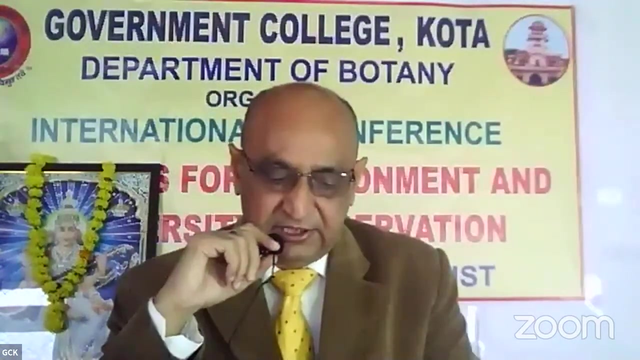 We have got a lush green campus which is in the heart of the city And that this college has so many feathers in the cap. We have produced so many eminent personalities, Not only in the academics but in the all sphere of the life, Thanks to entire botany department faculty members of the college. 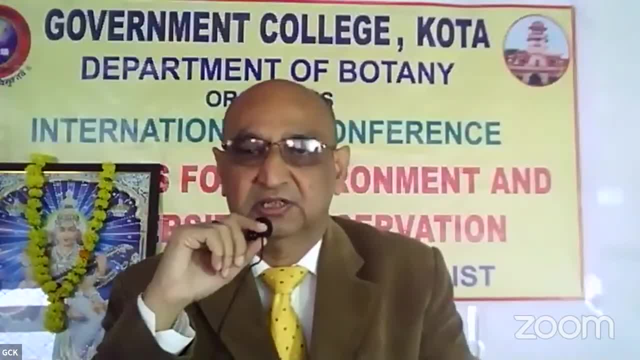 Dr Sanjay Bhargava, Dr Aguraj Parivar, Keep supporting us, keep doing all these things, And a day will come when we will be the masters of the world. Then we will be the masters of all these things. 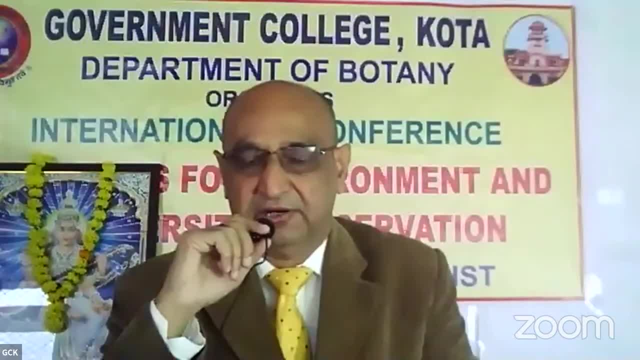 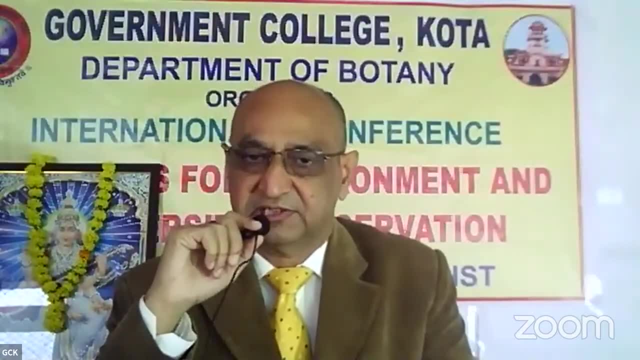 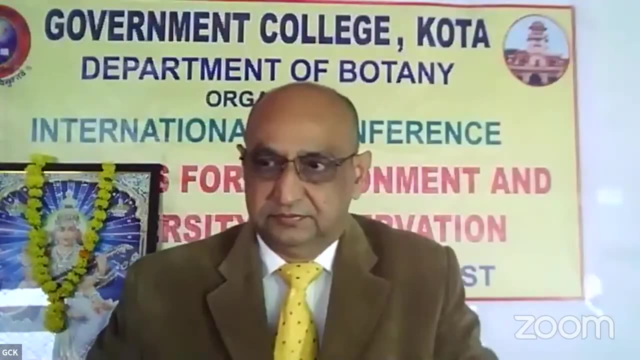 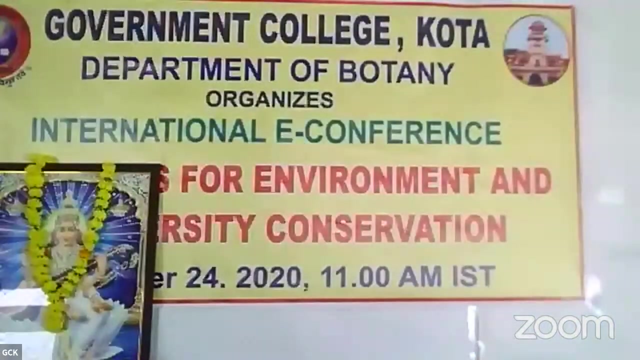 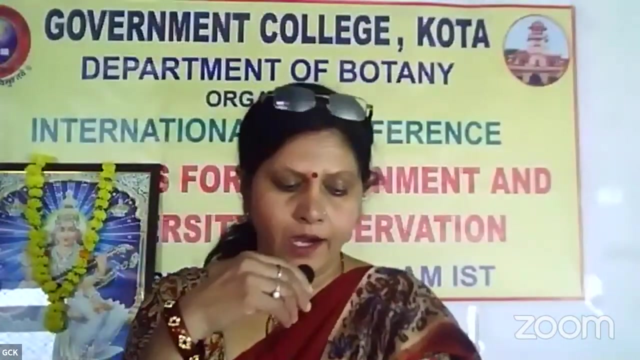 And the conservation is the need of the hour. Thank you, thank you so much, organizers, for today's program. Once again, congratulations and welcome to all the eminent keynote speakers. Thank you, thank you so much. I express my sincere thanks to principal sir for valuable words. 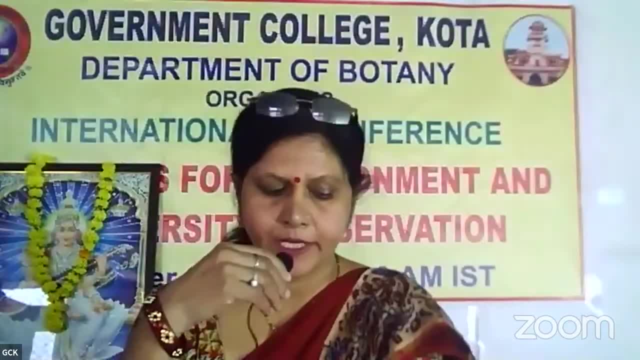 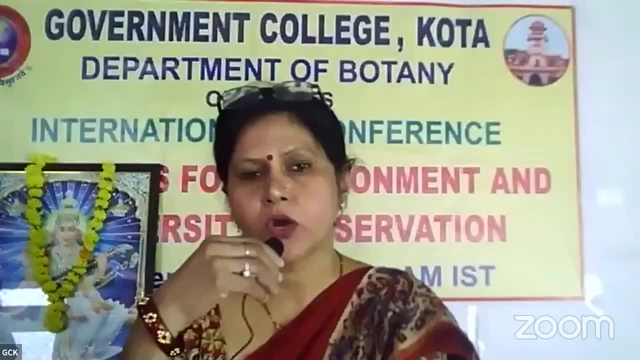 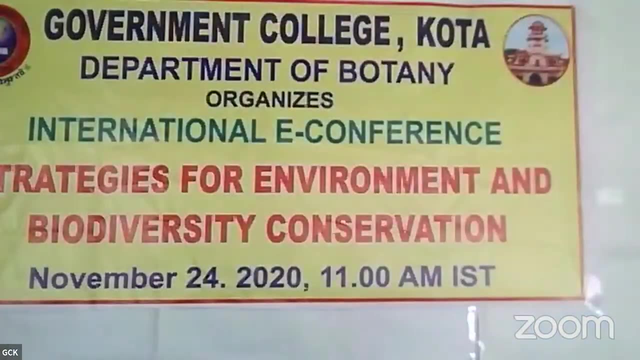 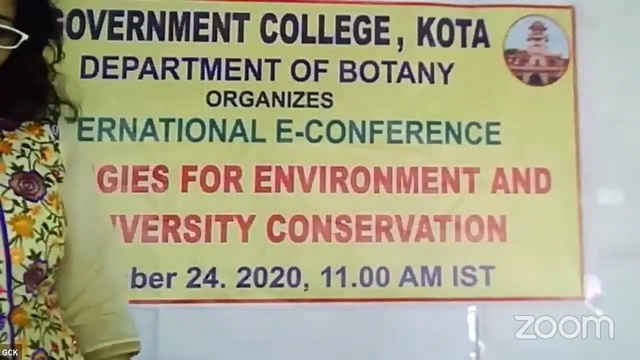 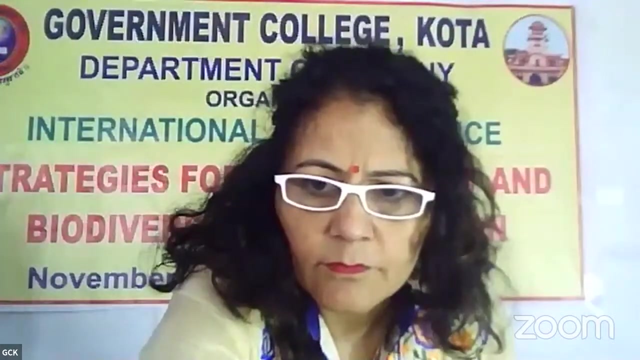 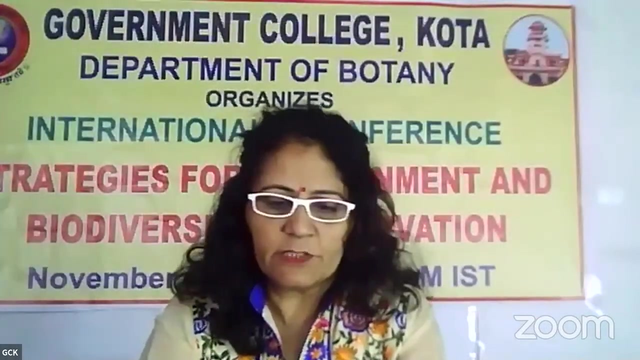 I cordially invite to head of the department botany, Dr Anju Kapoor. madam, Please come and share few words about the conference. Dr Anju Kapoor, madam, A very good morning to all the directors present here today. It is my honor and my privilege to be here today. 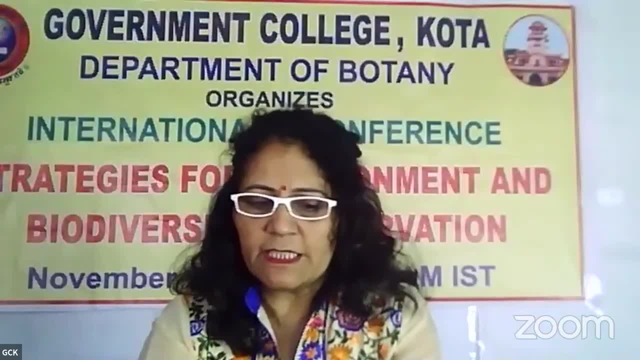 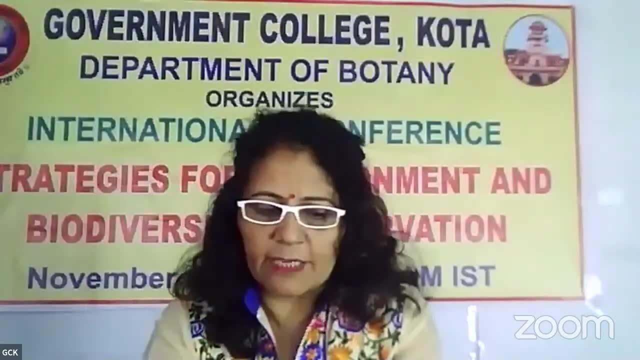 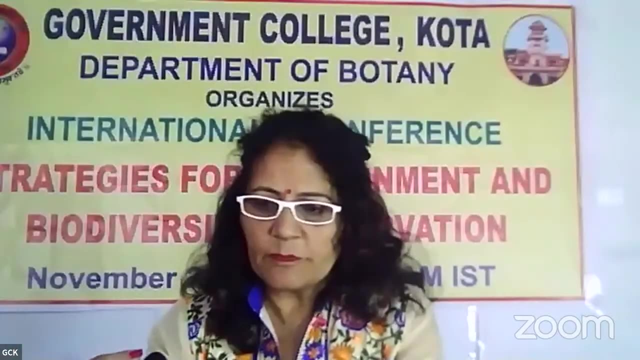 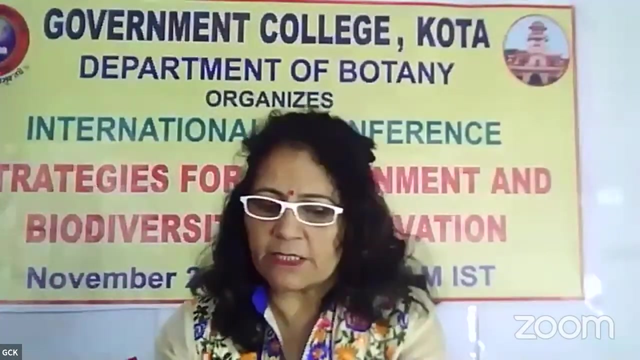 Because this day, 24th November 2020, marks the day of this fabulous international conference on strategies for environment and biodiversity conservation. Organized by the botany department at the government college quota, this international webinar is aimed towards understanding environmental issues at a global level. 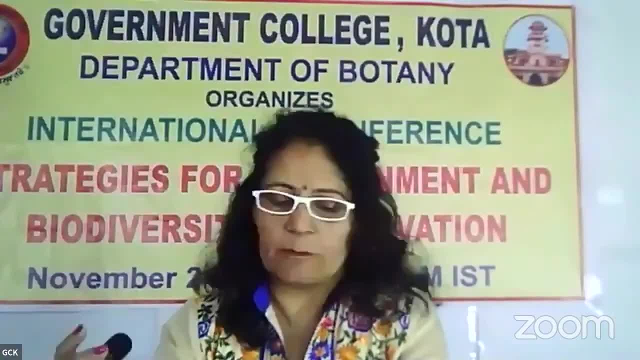 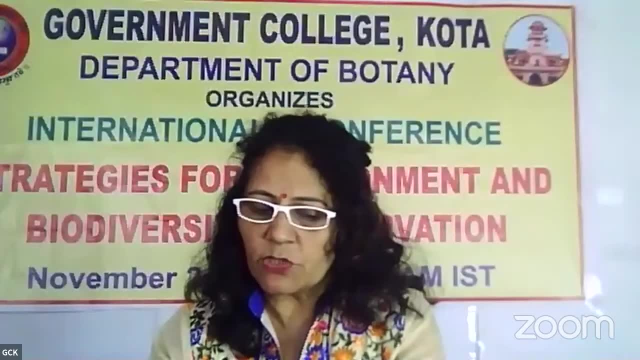 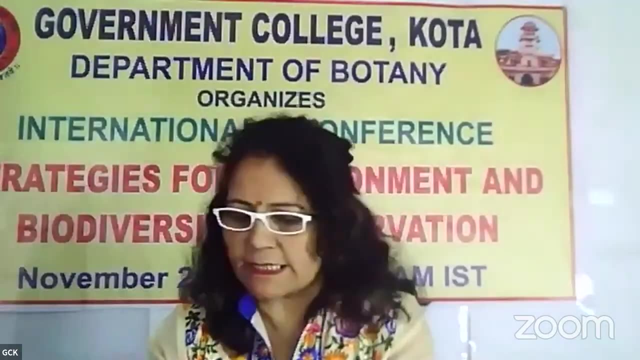 and finding the answer to these threats. My name is Anju Kapoor, head of the department of botany at government college quota, And it is my pleasure to welcome all our eminent speakers from around the world, The respected principal, sir, respected keynote speakers for the conference and all our beloved attendees. 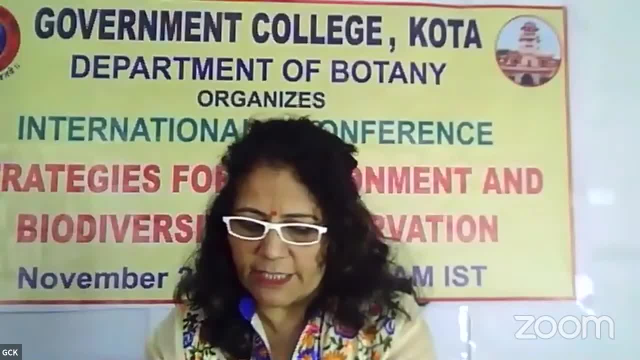 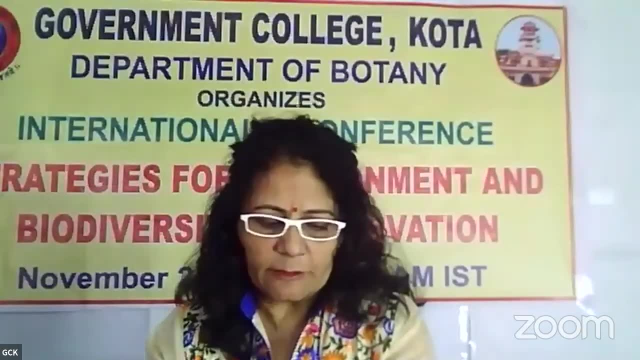 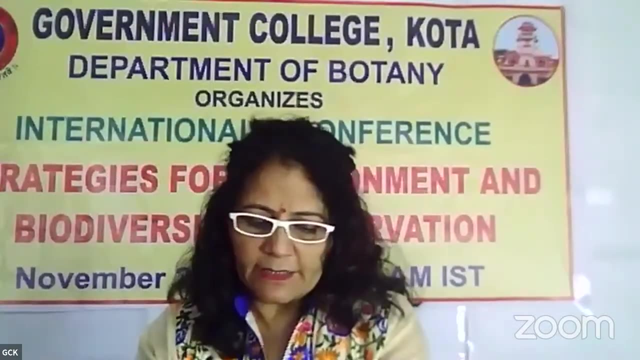 For the past few decades, the rate at which our natural resources are depleting has hit alarming numbers, While the level of air, groundwater and land pollution- land pollution- have also skyrocketed. As a non-professional and a citizen of this earth, 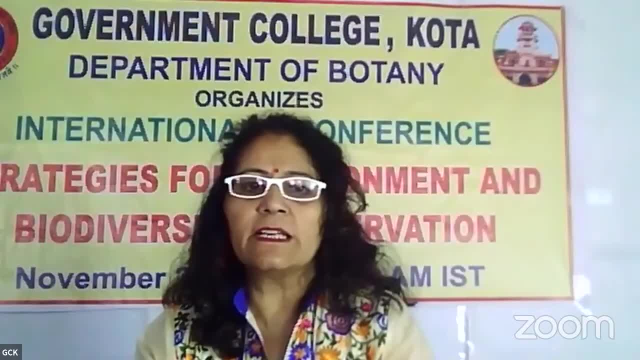 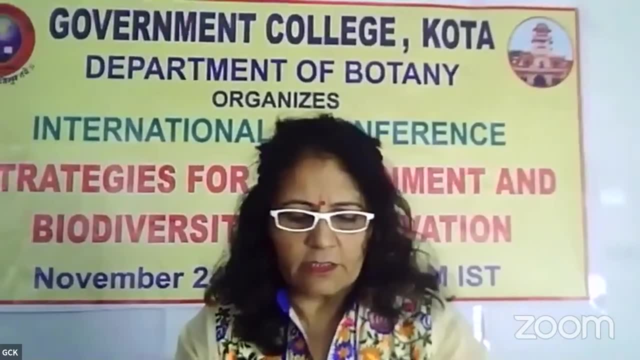 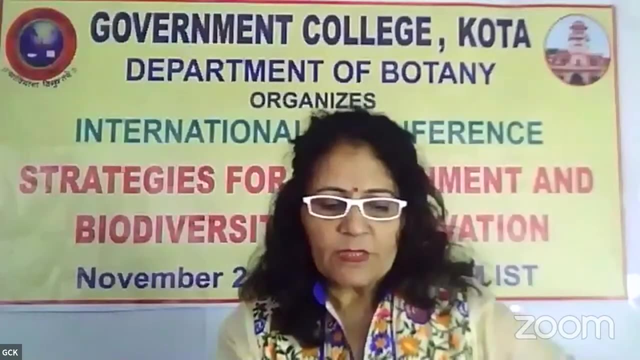 I have personally seen the effects of global warming on our lives. This conference, organized by the botany department under the supervision of the principal and patron of government college quota, Dr Jain Kumar Vijayavargia, seems to give voice to the experts that we have on our committee today. 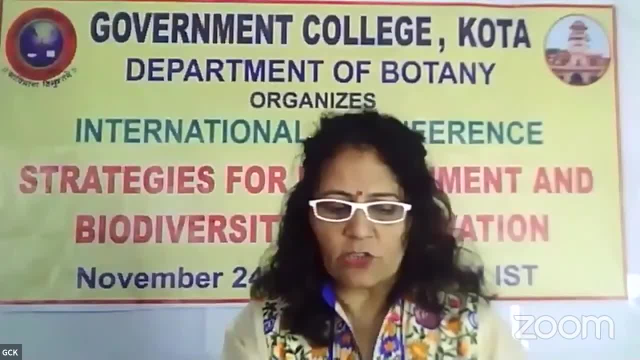 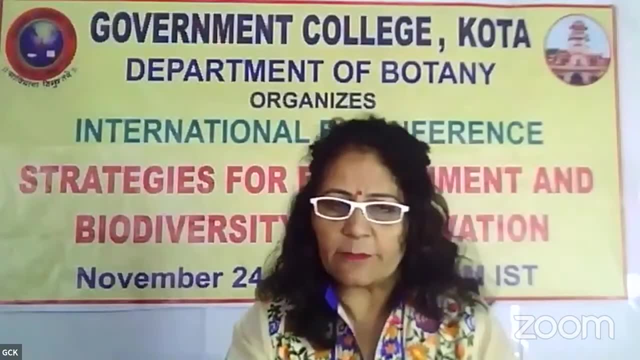 So they can come forward with their ideas and observations of this threat and looms large above us. today, Where the ozone layer is depleting because of our malpractices, we are furthering the damage by cutting down and burning our forests. This has not only resulted in the loss of our precious heritage- forests. 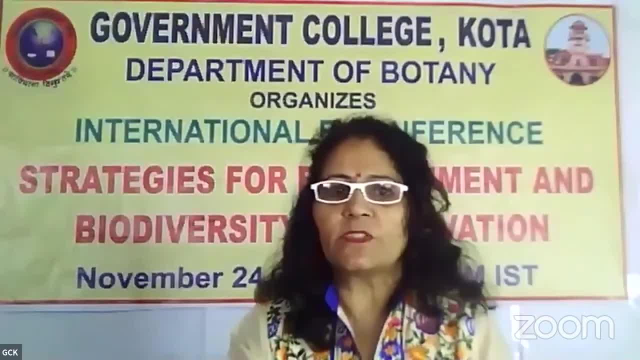 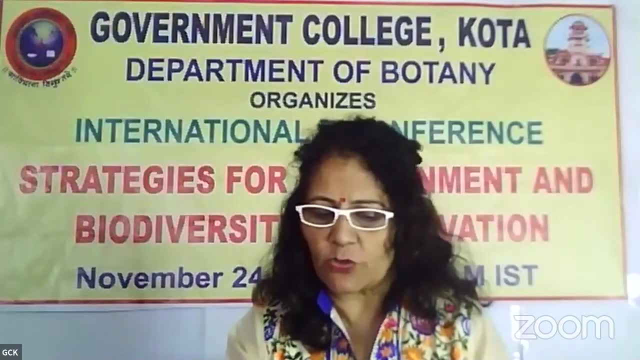 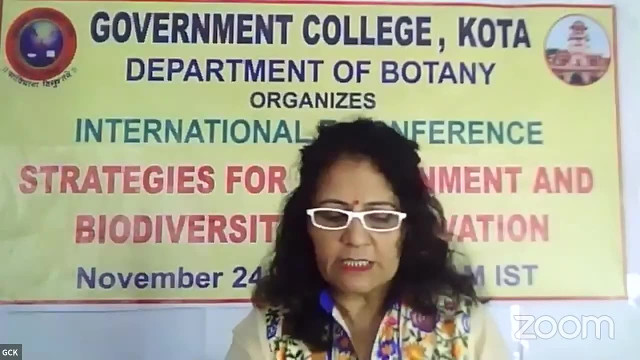 but also in the extinction of several species of the biodiversity. Further editing to these issues is a way: nuclear waste and being dumped and soil spills that happen at the sea. This e-conference is a small contribution we are making towards the awareness of these global issues. 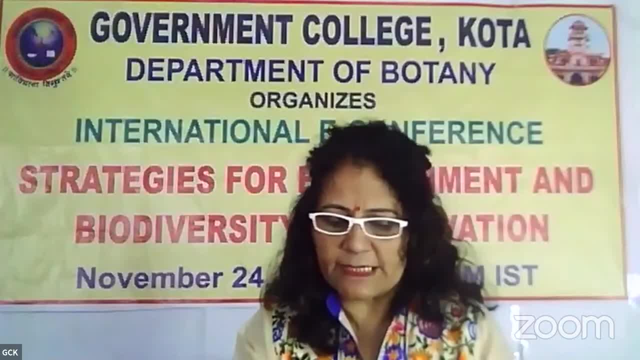 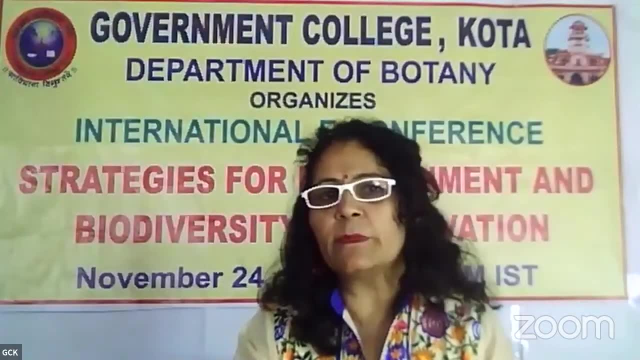 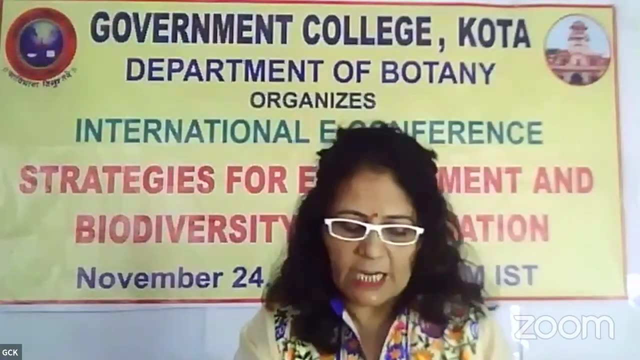 What's more. for this, I would like to thank our principal for his supervision today and, furthermore, appreciate you to my colleagues for their incredible commitment. It is therefore my pleasure to welcome our eminent speakers on the behalf of the department of botany government college quota. 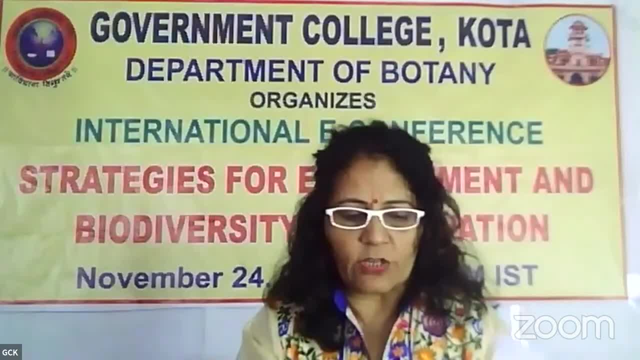 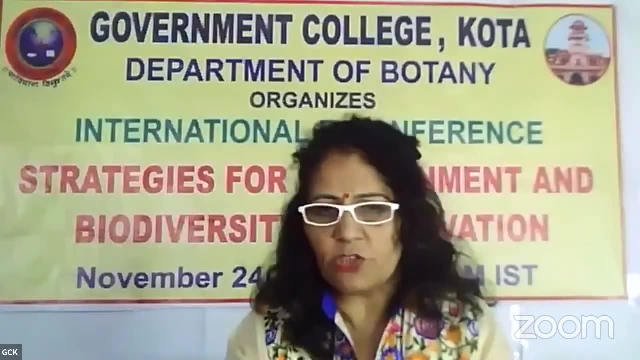 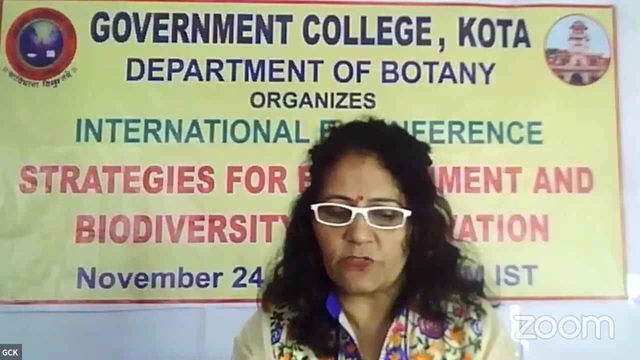 They have joined us from all around the world for this e-conference today: Professor Deva Bahadur Khatka from Tribhuvan University, Kathmandu, Nepal. Dr Barla Andrew Swinkor from IMO State University, IMO State, Nigeria. 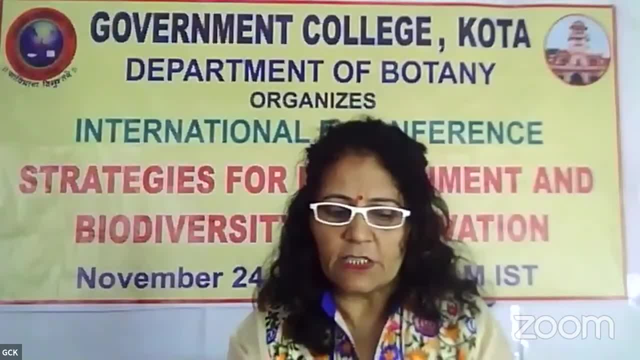 Dr Prashant Singh from BHU Varanasi, Uttar Pradesh. Dr Avdesh Kumar Srivastava from Durga, Chhattisgarh. I would also like to extend a special welcome to our special invitees for the day. 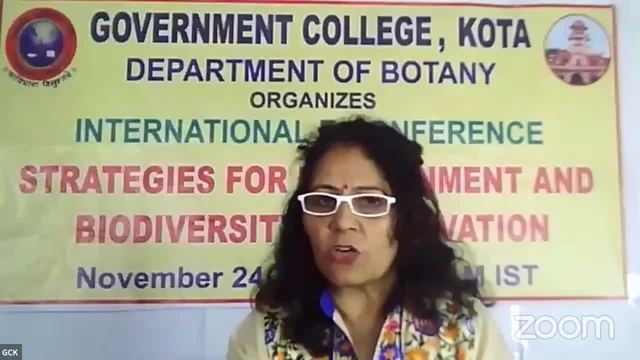 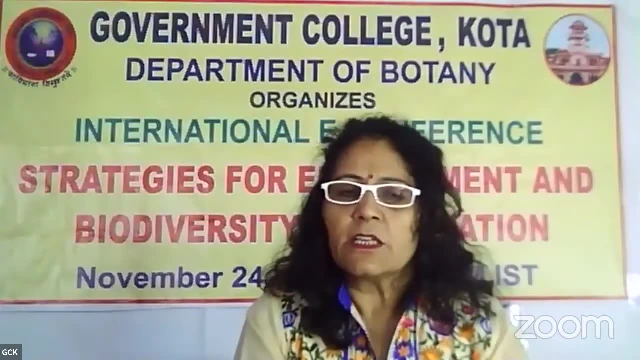 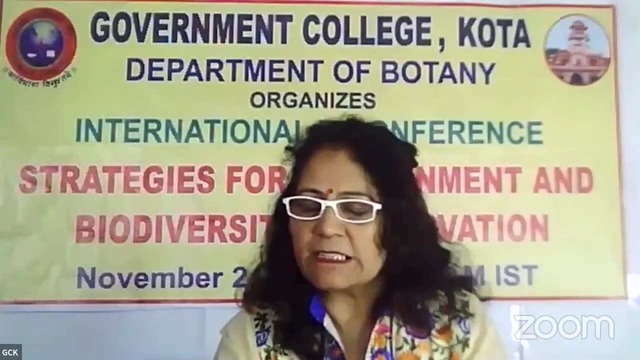 Dr Sanjay Bhargava, Regional Assistant Director, College Education, Kota, And Dr Raghu Raj Parihar, Journal Secretary, AI, FUCTO. Global warming, loss of biodiversity, extension of wildlife and loss of natural habitat are the real things and in order to fight this very disruption, 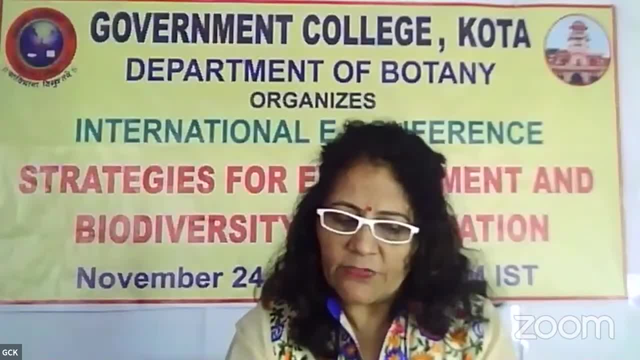 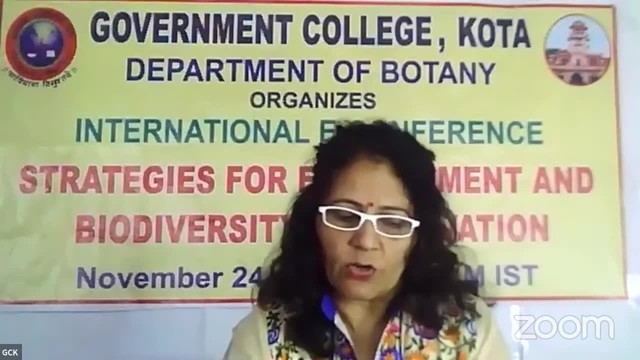 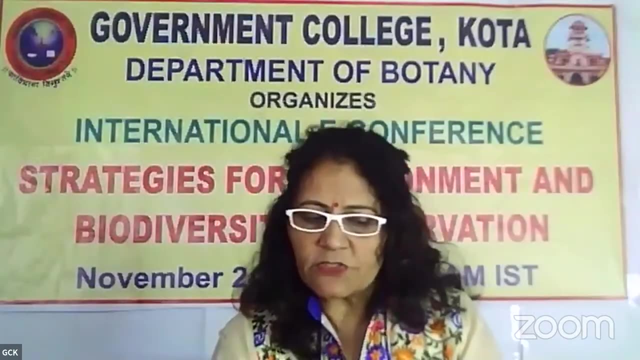 that we have caused to our environment and our world. everyone is doing their bit. We can continue to simplify the environment to meet immediate needs at the cost of long-term benefits, or we can conserve life's precious diversity and its sustainability. Biodiversity conservation must take place at the individual level. 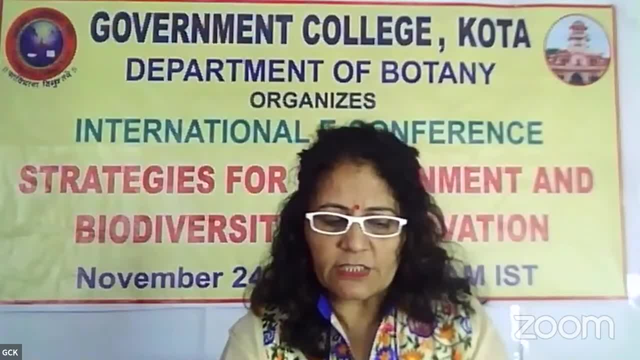 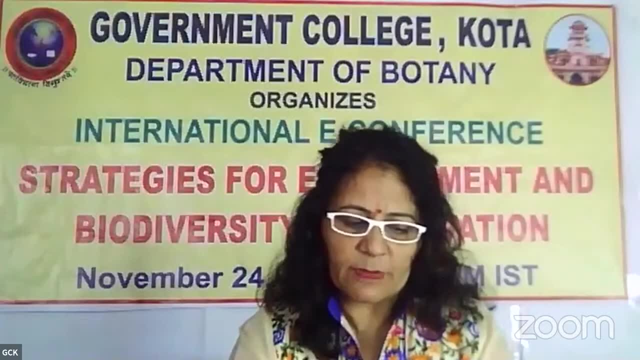 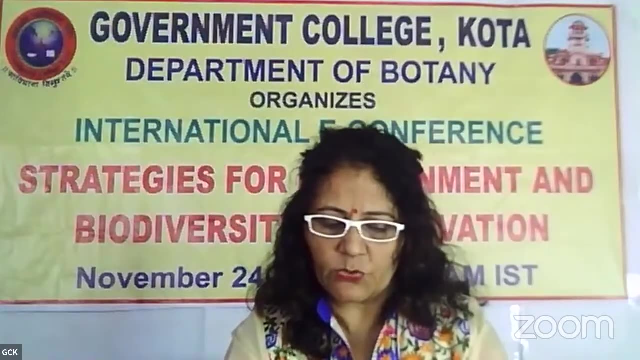 the global level and in between. Effective conservation effects begin in the field: forests, watersheds, grasslands, coastal zones and settlements where people live and work. We can participate in biodiversity conservation by increasing our knowledge of environmental issues, increasing our awareness of the impacts of biodiversity loss. 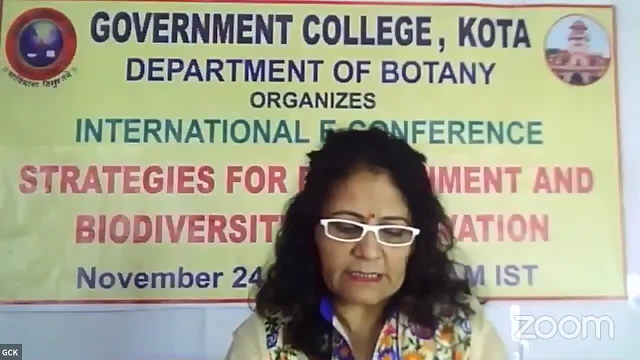 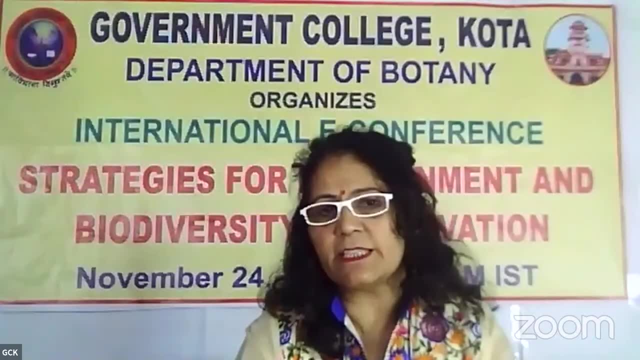 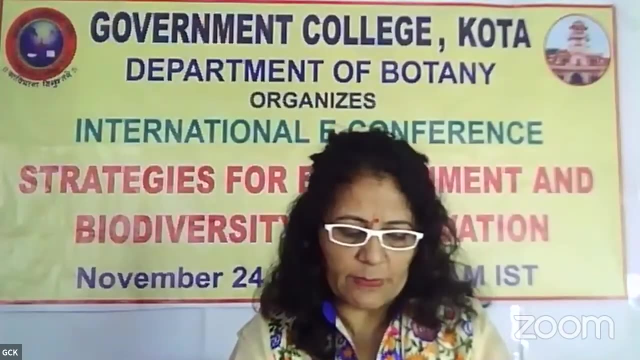 and increasing support for government policies and actions that conserve our valuable ecosystem. I am sure that this e-conservation conference has been an enlightening experience for many, as it has for me. Once again, I would like to express my gratitude towards our principal, under whose guidance this e-conference was organized by the Botany Department. 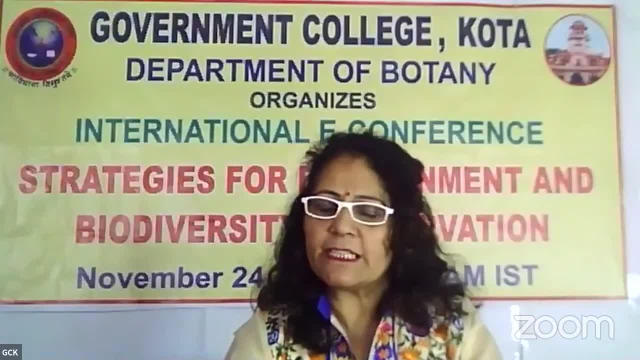 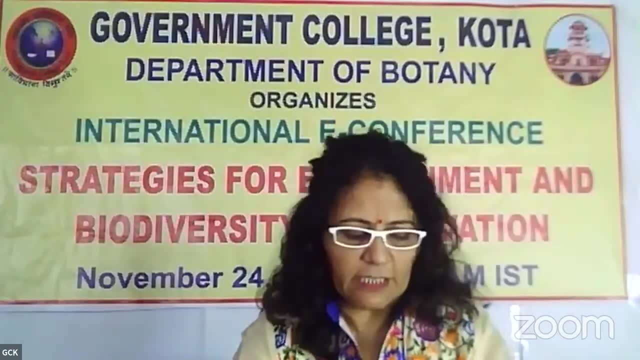 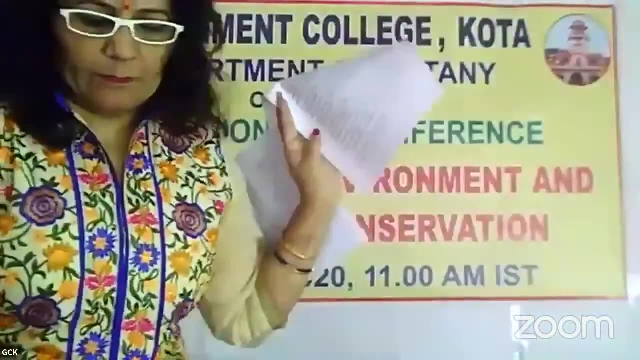 I would also like to extend my gratitude to our eminent speakers for sharing their valuable insights. I hope one day we will be able to save our Earth from the path that it is on. Thank you everyone, Thank you, Thank you all, Thank you. 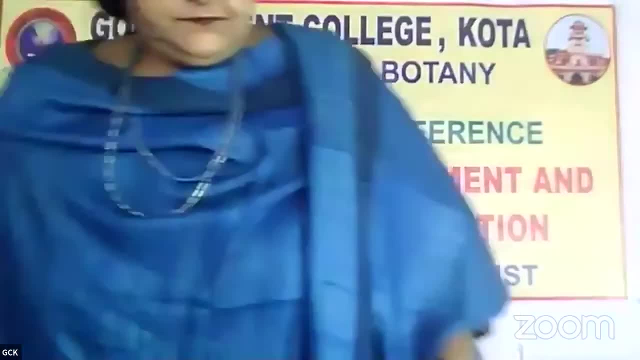 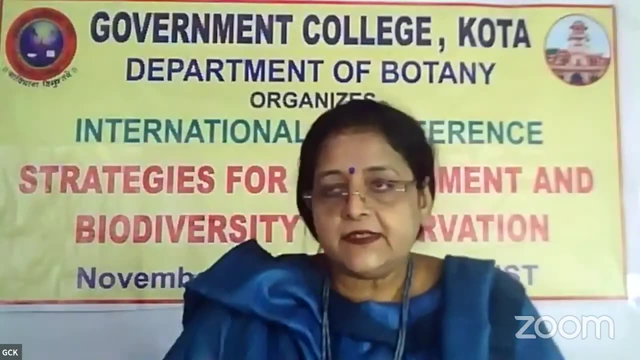 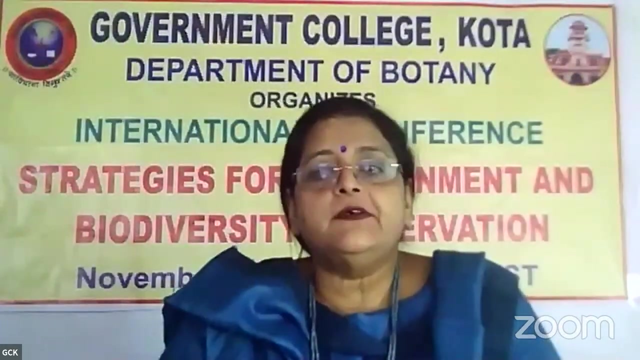 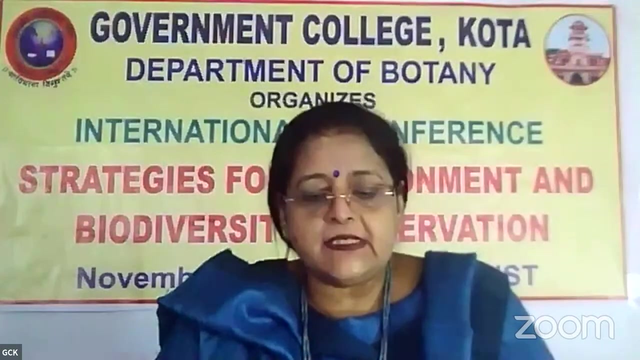 Dr Isha, Thank you. Thank you. Thanks, Dr Anju Kapoor, for briefing about the international e-Seminar I. Dr Vandana Sharma, Associate Professor, Government College Kota. welcome all distinguished guests, participants, faculty members, students. 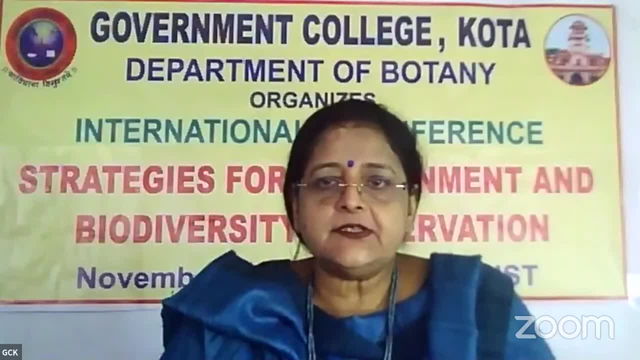 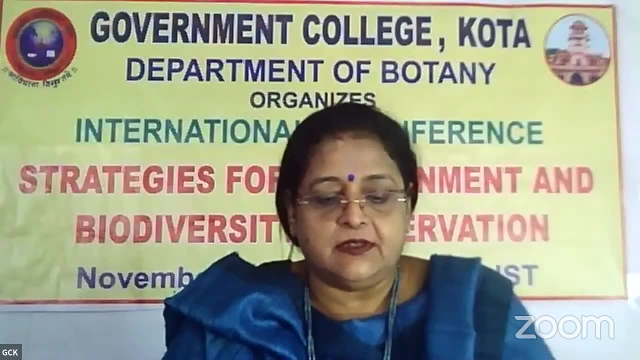 students, colleagues and Orthodontists and all participants, students in this international e-seminar. It is indeed a wonder that today, in spite of ongoing, unprecedented situation of this pandemic, we are able to connect to number of people from across the cities, states and even countries, Thanks to the progress and the technology that made this. 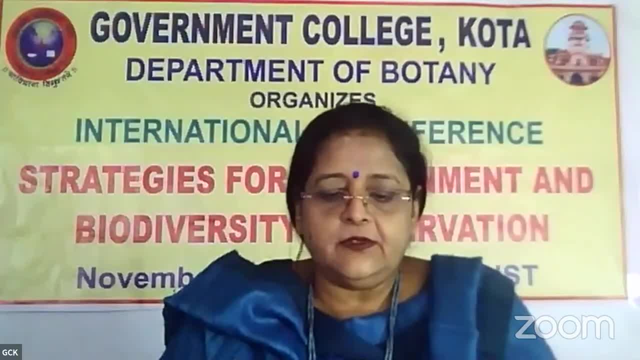 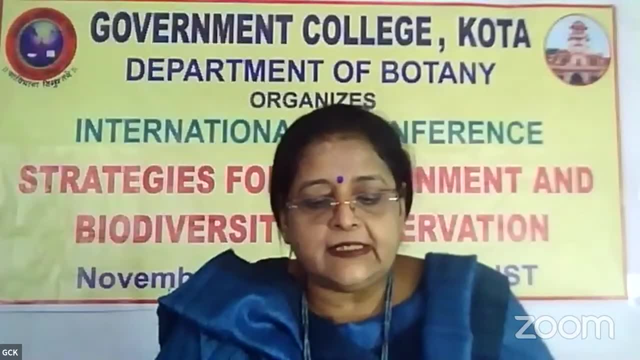 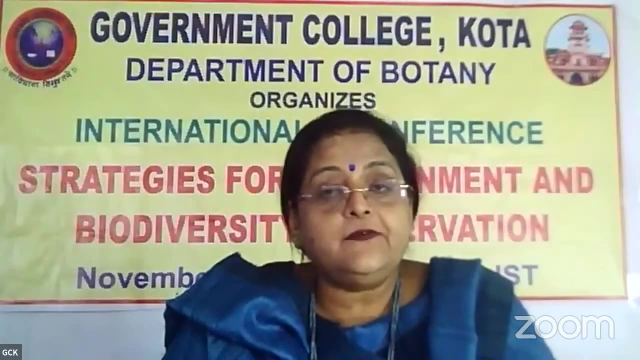 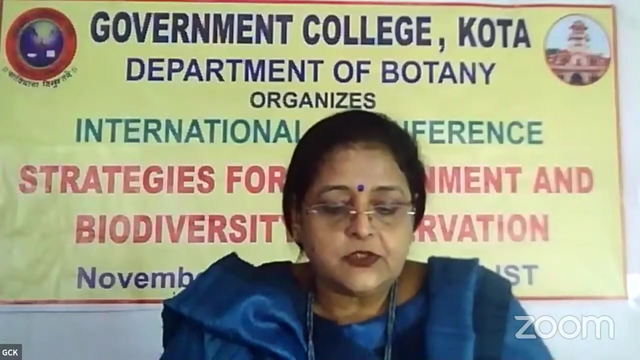 online seminar possible so that we could connect to people across the country and even further. Thank you all for taking time out and being with us. I am here to start first technical session of this e-international seminar. The topic of seminar, as ma'am Dr Anju Kapoor told you. 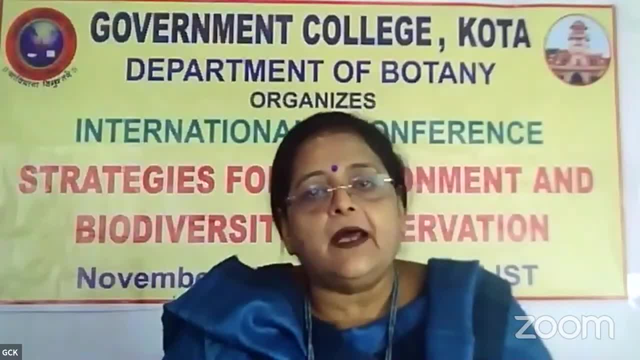 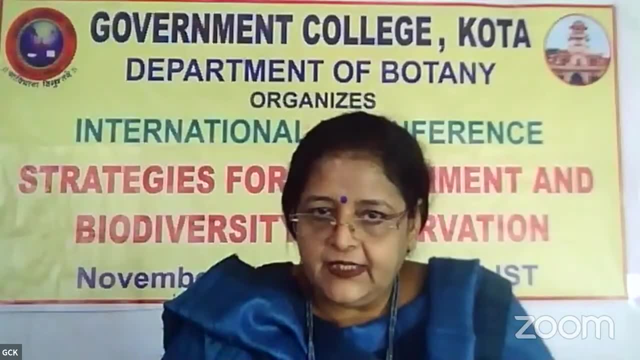 that it is the conservation of biodiversity and the environment. Both are asset to us. Saving the biodiversity and the environment is our duty. Conservation is the need of our. It is very essential for sustainability of healthier earth. Biodiversity is life. it is our future. 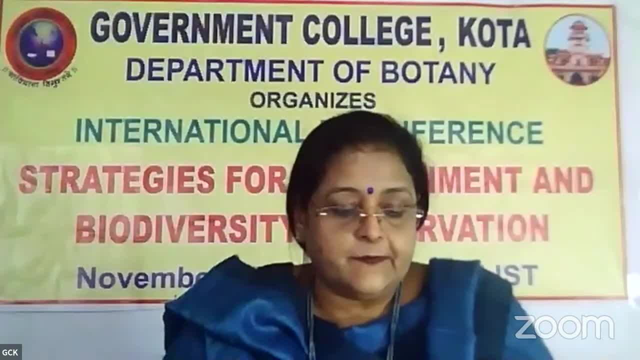 Now, without further ado, we'll turn the time over to speaker. Our first speaker is Prof Deva Bahaduradkarka. Please come Lo Rocracy, will trees come to you right now? in они четыре forms, Munich and Germany. ring culled, audi my ceiling because your home is not so pretty, Thank you. Thank you for your08. 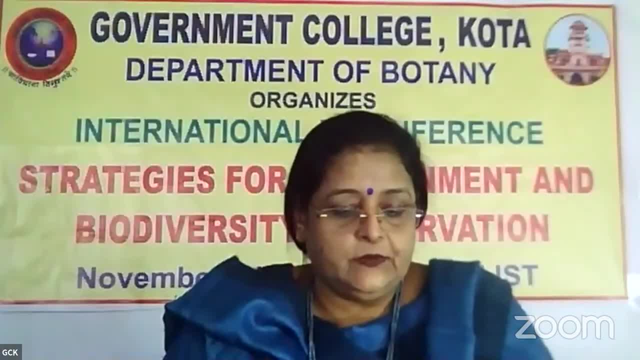 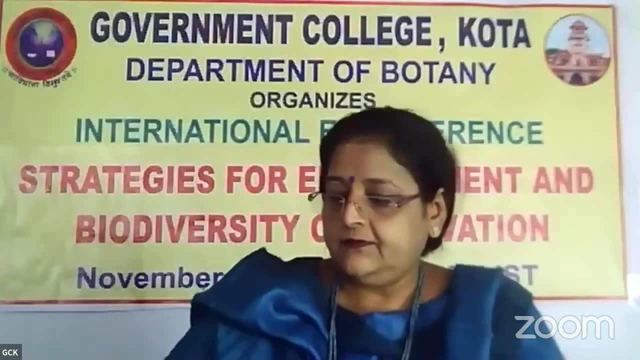 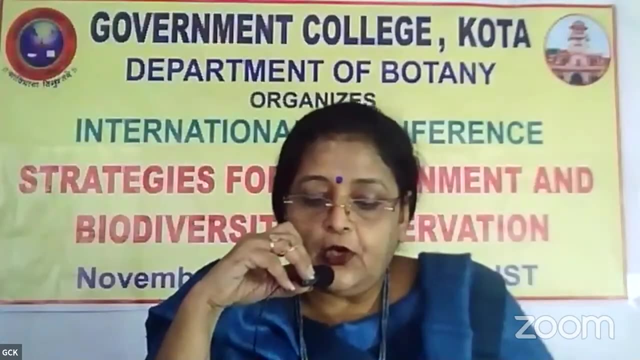 intellect from nepal tribune university, kathmandu. he is a dean of science. he has many laurels and accolades. a fellow of a fellow of royal nepal academy of science and technology, member of new york academy of science, vice president, nepal chemical society. his field of research are 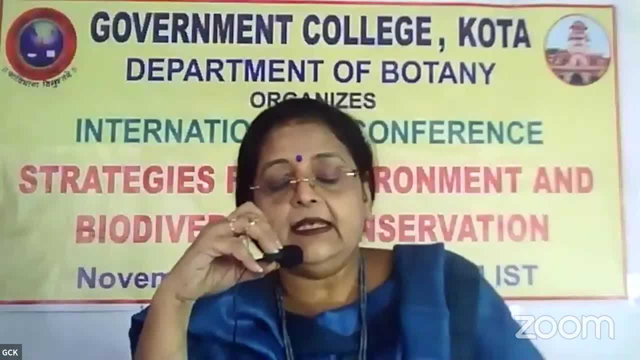 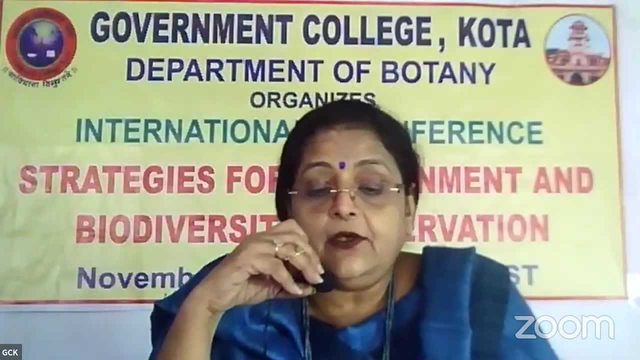 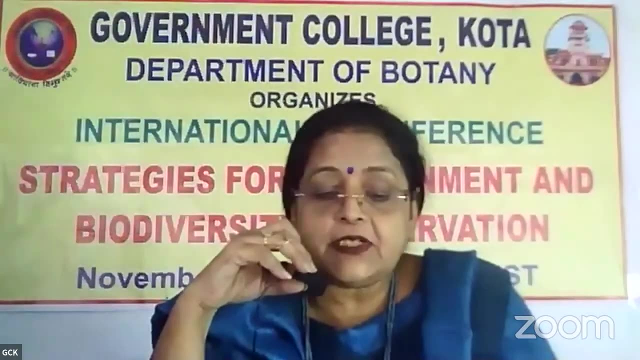 environmental science, solar cell and radiation chemistry. as a botanist, it occurs to me that nepal is in himalayas and hot spot of biodiversity. i'm certain, i'm sure listening to prof khadka will definitely enrich our knowledge of biodiversity of nepal and even 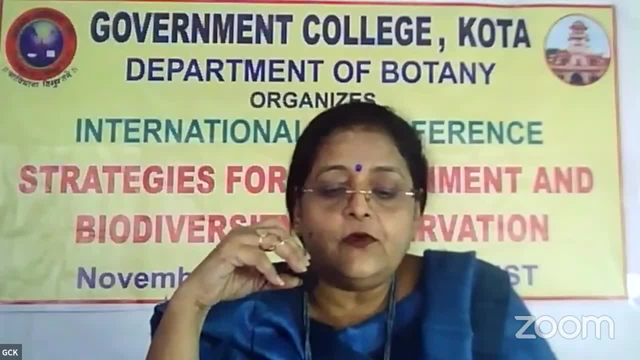 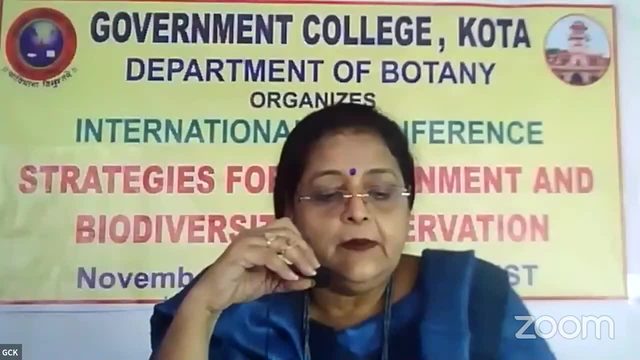 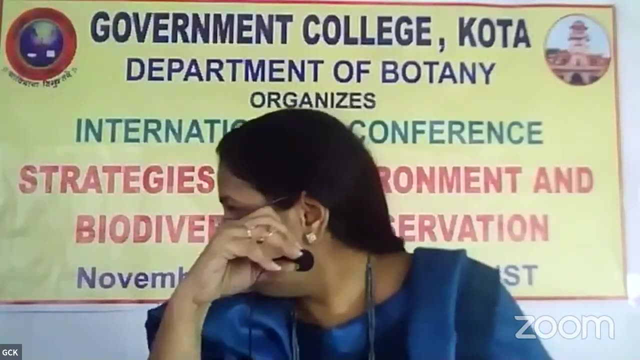 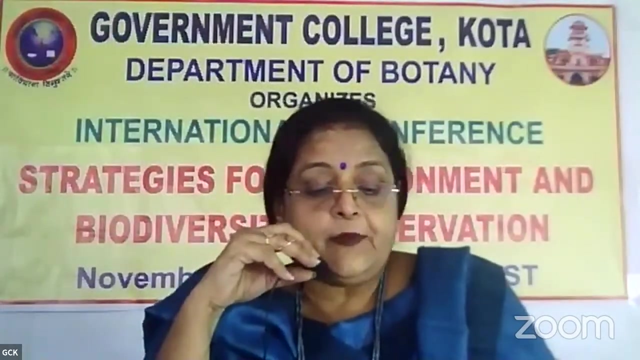 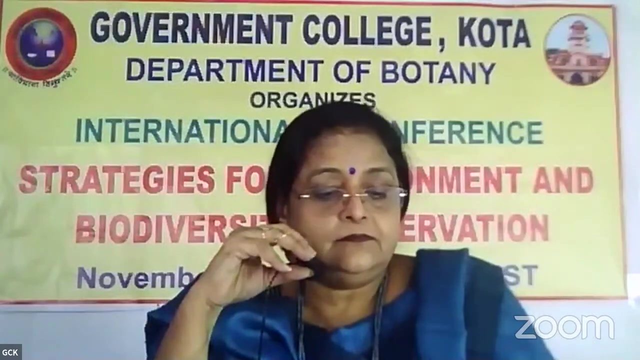 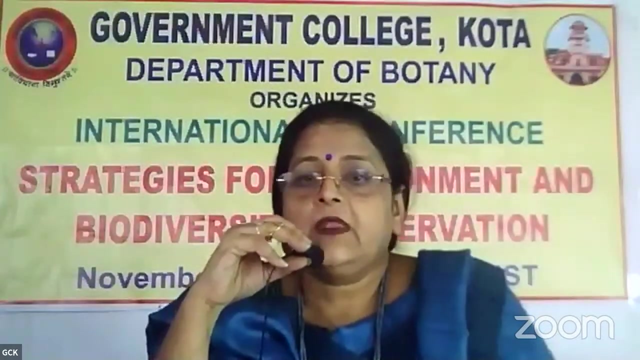 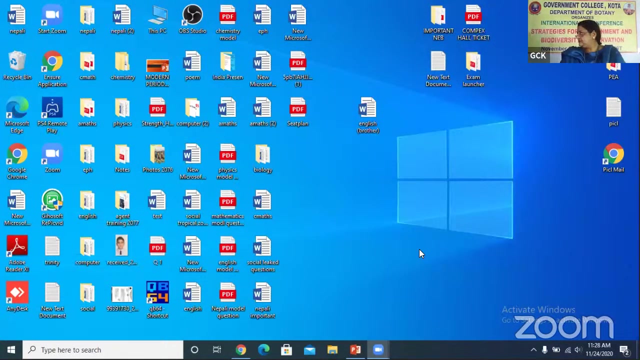 further. so let's not waste time. move on to our lecture, sir. i request professor deva to connect, please. people are eagerly waiting what you have in store, professor khadka. shortly professor khadka will be with us with his valuable views. absolutely um in the. 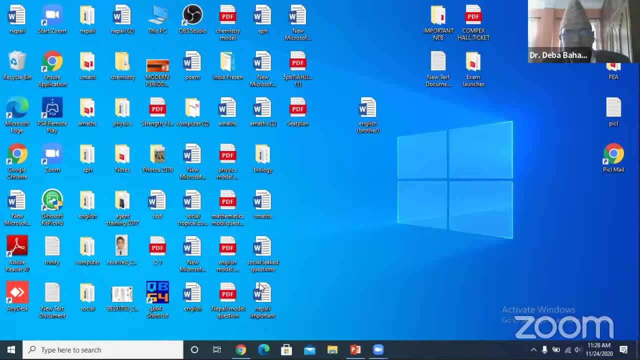 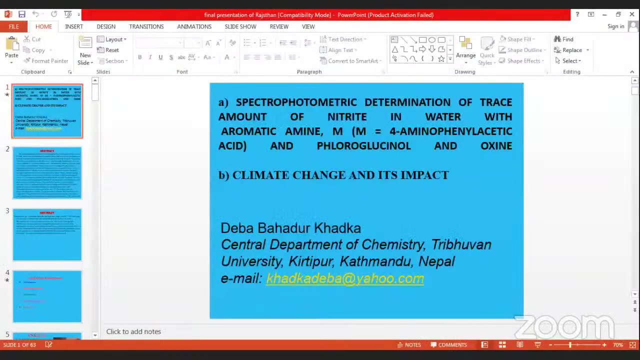 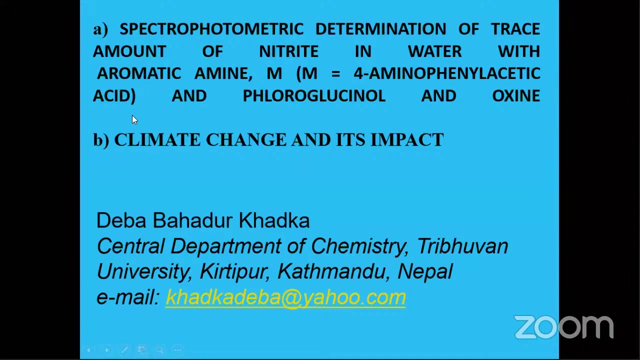 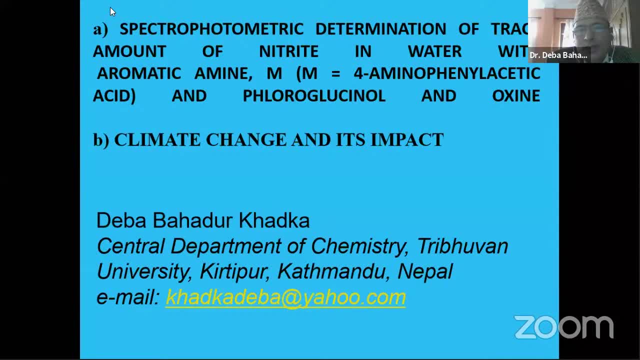 That means M correspond for amino acidic acid and photoresonance and obsidian, and the next is climate change and its impact. It is okay. So basically I am a chemist, as you already know, not environmentalist, but I am doing different types of project and at present I am a professor of Central. 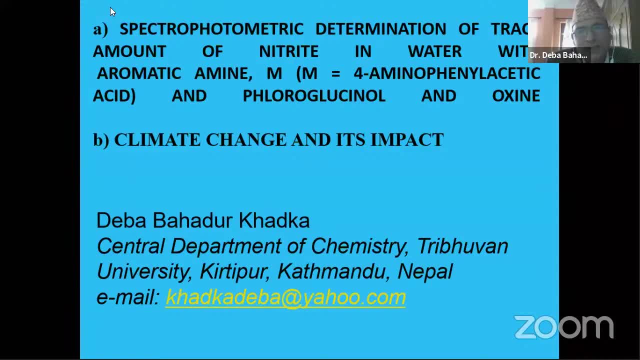 Department Chemistry and Environmental Science. So I am a professor of Central Department Chemistry and Environmental Science- chemistry and I just completed my dean position a few months ago. And the reality of life on the earth is known as biodiversity, And biodiversity takes into account all the living organisms present on the earth. 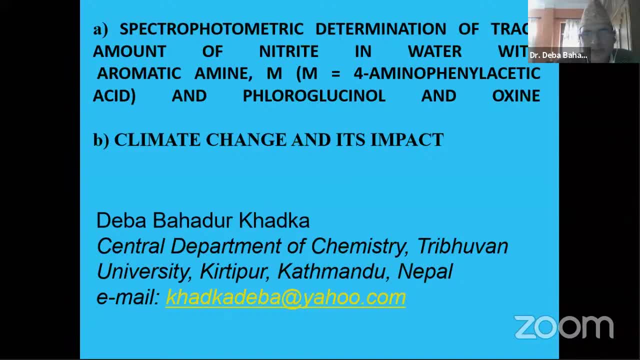 Healthy and good biodiversity indicate a healthy and good ecosystem. Therefore, biodiversity is very important, And a healthy ecosystem includes the availability of pure water, pure air, healthy land, good climate and a lot more. So biodiversity is very important, And a healthy ecosystem includes the availability of pure water, pure air, healthy land, good. 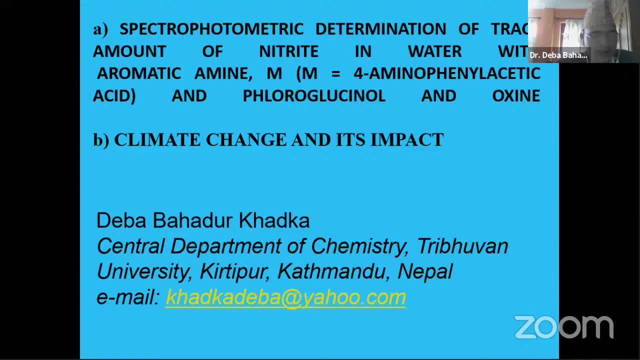 climate and so on. A number of factors like pollution, erosion, urbanization and depletion led to the loss of biodiversity. Loss of biodiversity has a poor impact on ecosystems. A threat of biodiversity means threat of humankind, So biodiversity is very important. 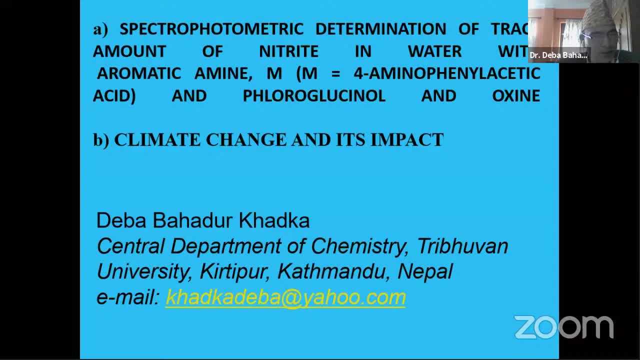 And I just completed my dean position a few months ago. And I just completed my dean position a few months ago And I just completed my dean position a few months ago. So environmental conservation is a wise management and utilization of natural renewable resources in a sustainable manner to ensure the maintenance of the biodiversity. 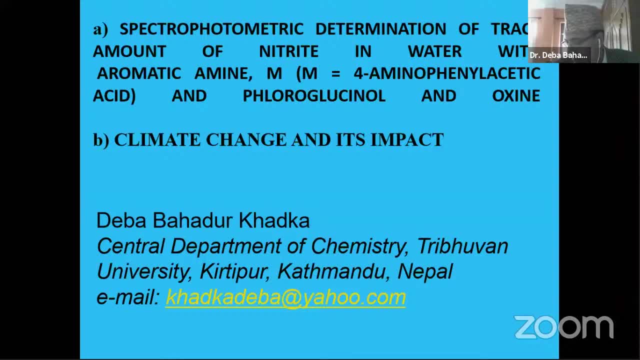 So, according to the international topics- international conference on traditionally environment, biodiversity conservation- there are so many strategies. There are so many strategies. limited time so I only prepared the two topics, which is also related to the this international conference. Some of the studies, like managing the biodiversity throughout the human environment. 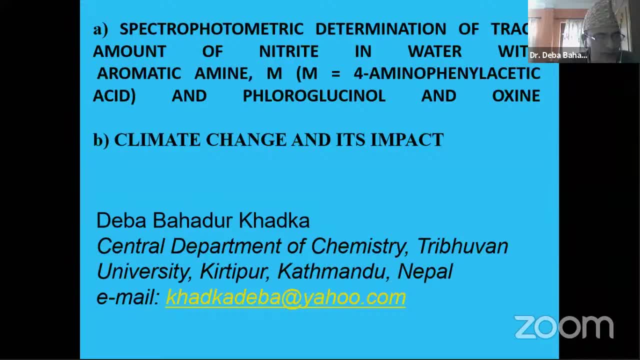 incorporate the biodiversity conservation into the management of biological resources. strengthening the protected area, conservation of species, population and genetic diversity. expanding the human capacity to conserve the biodiversity. First, I will talk about the environmental biodiversity. This is based on the primary data. 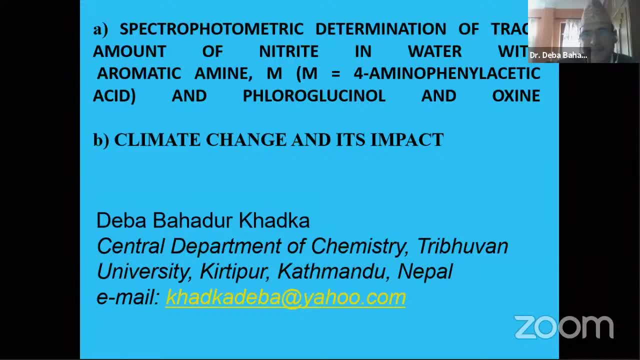 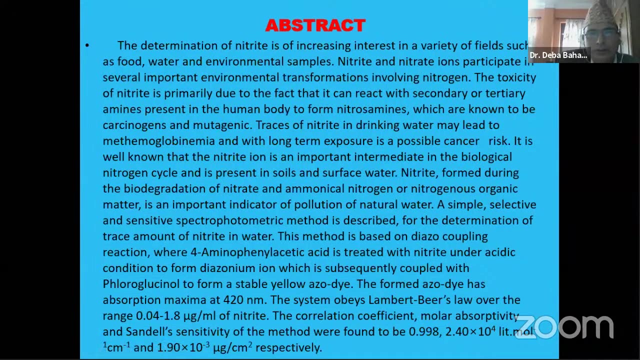 and secondly, I will talk about the climate change. in effect, This is based on the secondary data. So this is the first step. So these are my abstracts. The determination of nitride is increased increase in variety of fields, such as the food, water and environment. The nitrides and parts are relatively similar. 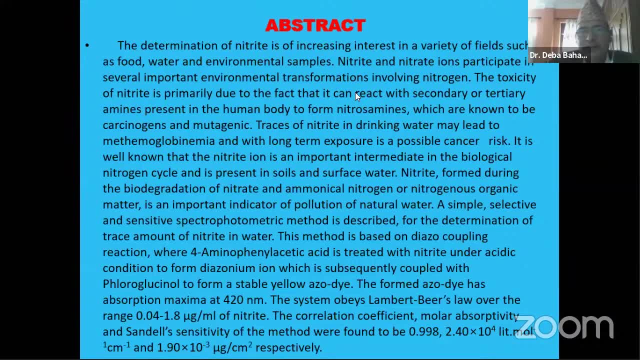 Several of these classes are also linked to environmental biodiversity. environmental and the toxicity of nitrate is primarily due to the fact that it can react with secondary or tertiary amines present in the human body to form a nitrous amine, which is known to be carcinogenic and mutagenic. 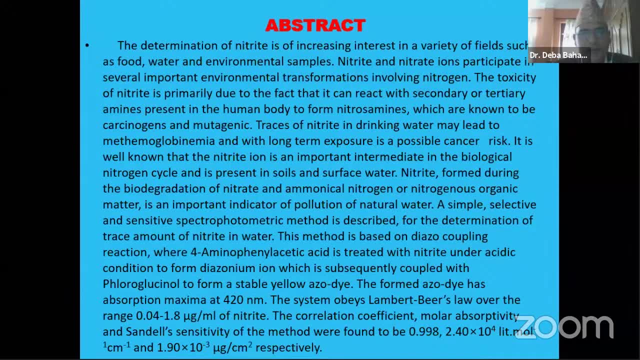 This amount of nitrate in drinking water may lead to methamoglomerulamide and, with a long-term exposure, is a possible cancer risk. It is well-known that the nitrate ion is an important intermediate in the biological nitrogen cycle and is present in soil and surface water. 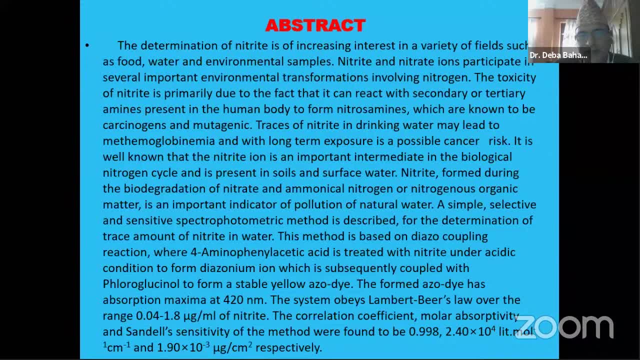 Nitrate form during the biodegradation of nitrate and ammoniacal nitrogen or nitrogenous organic matter is an important indicator of pollution of natural water. A simple selective ion-sensitive system can be used in the production of nitrate. The spectrophotometric method is described for the determination of the trace amount. 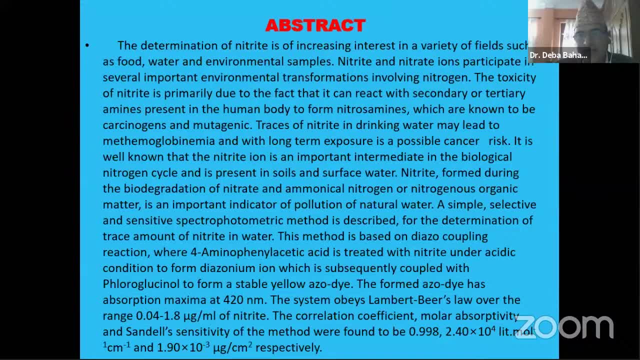 of nitrate in water. This method is based on diisocoupling reactions, where 4-aminophenylacetic acid is treated with nitrate under the acidic conditions to form a diisonium ion, which is subsingually. 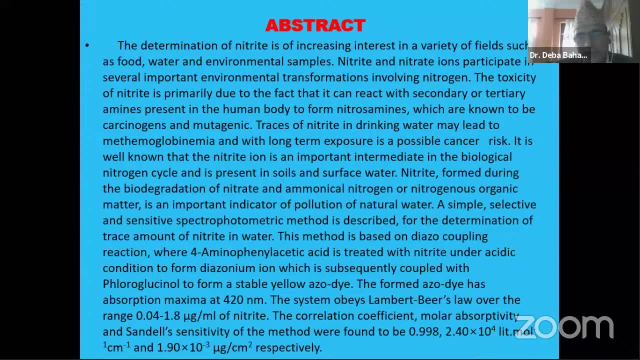 coupled with the polyglycinal to form a stable aloe-colored azo-dye. The formed azo-dye has been absorbed maximally In the same way. the system of a Lambert-Walsh law over this range and the correlation coefficient. 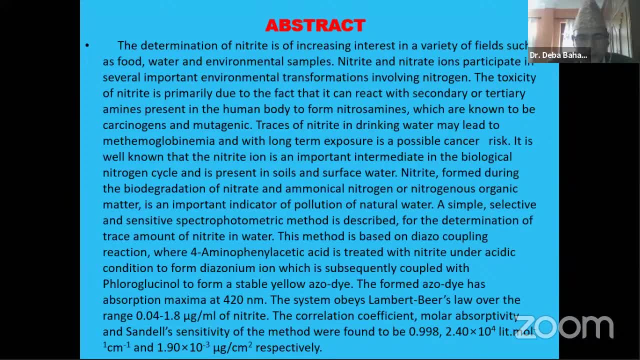 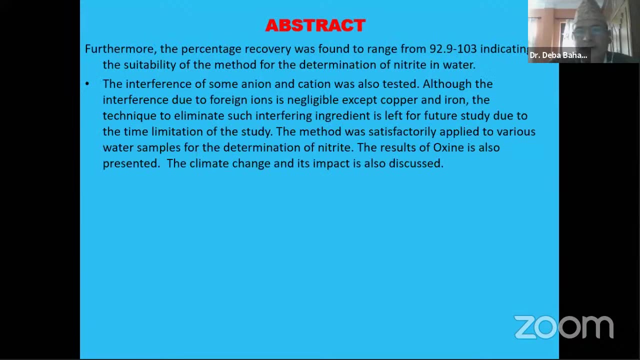 molar of the recent traceability of the method were found like this: Furthermore, the percentage range of the method is 3.5. 3.5. 4.5. 4.5. 5.5. 6.5.. 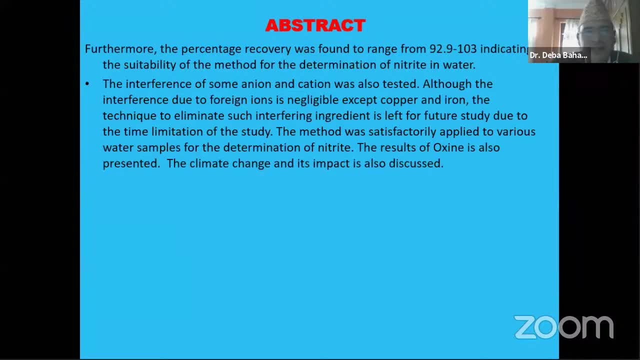 6.5.. 7.5., 8., 8., 9., 9.. 1.. 3. Indicates the suitable measurement of the method for the determination of nitrate in the water. Some of the interference ions has been also tested. 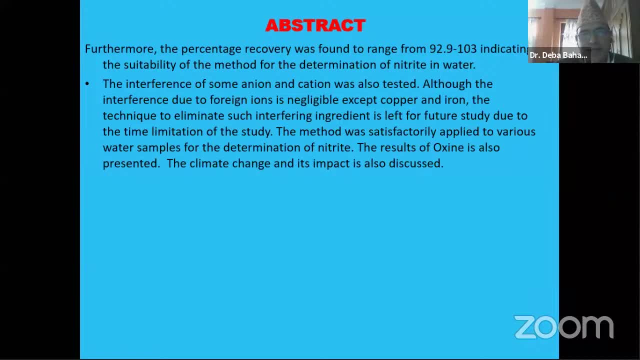 Although the interference due to the appearance ions is inexhaustible as copper and iron, the technique to eliminate such interference ingredient is left for the future study due Due to time limitations, the method was successfully applied for the determination of nitrite in water samples. 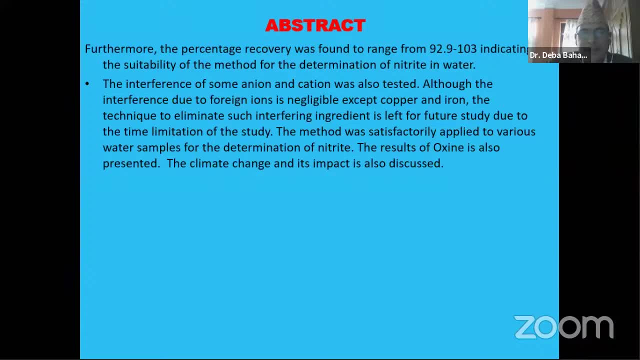 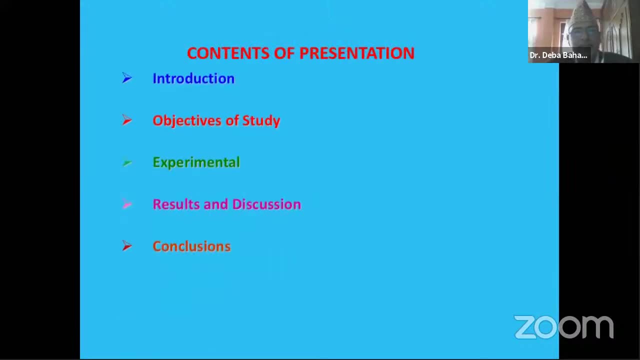 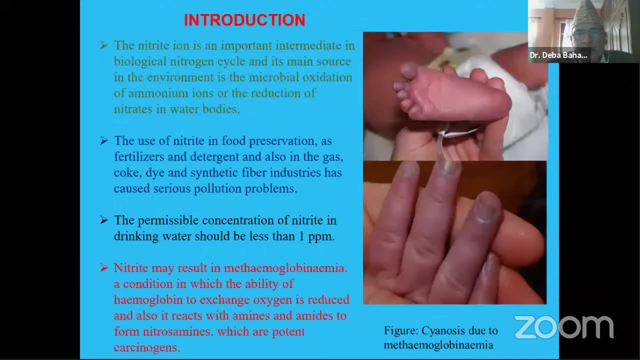 The result of the design is also presented and the climate change and its impact is also discussed. The content of my presentation: introduction, objective: experimental: these are under discussion According to the abstract, also mentioned briefly about the introductions and the use. 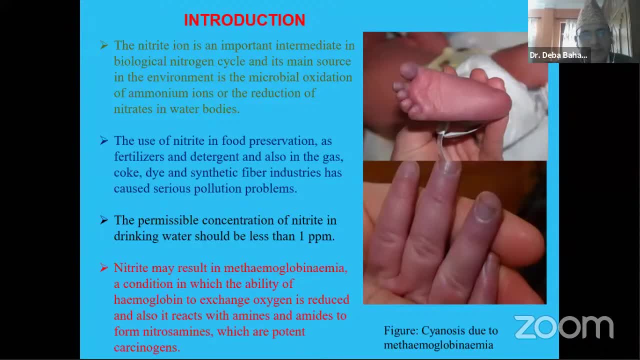 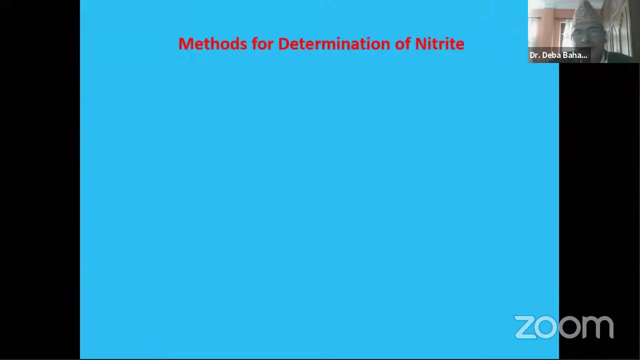 of nitrite in food presentations as a fertilizer and a detergent, also in the gas, coke dyes and the synthetic fiber industries, has caused serious pollution problems And the permissive concentration rate of concentration. The concentration of nitrite in drinking water is less than 1 ppm. 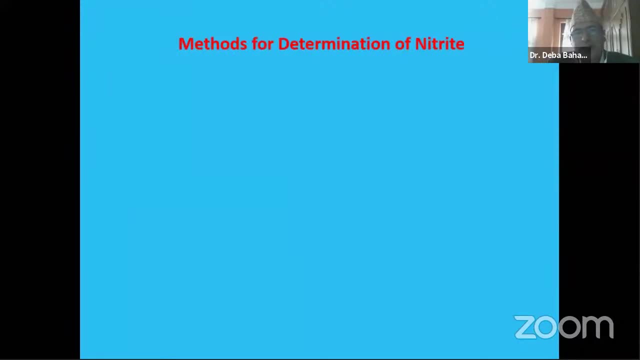 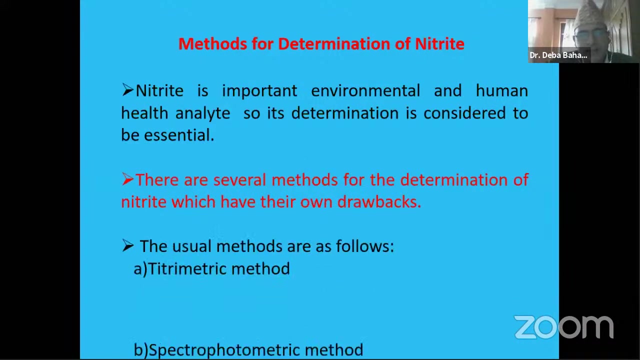 And there are several methods for the determination of nitrites in water, such as electrochemical detections, kinetics, chromatography, spectrophotometric methods. They have own advantages and disadvantages. The usual methods are the tritigmatic methods. This is the most useful when the amount of nitrite is high in the sample. 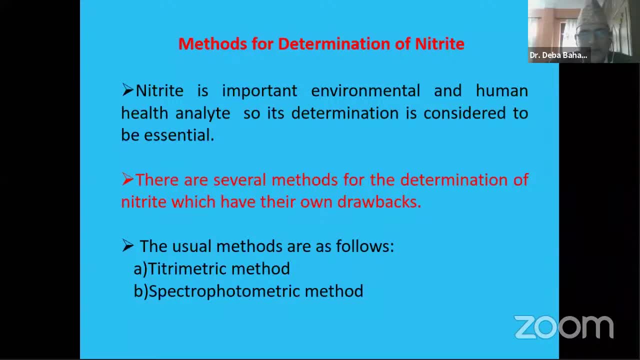 And it is very useful for the determination of purity of sample. But at low amount of level it is, it cannot work so well. On the other hand, spectrophotometric methods. The spectrophotometric method is based on the reaction. 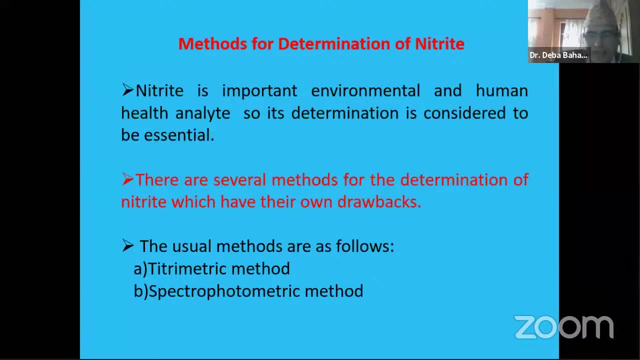 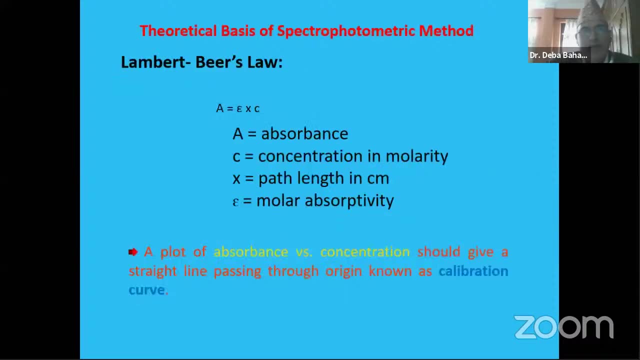 It means this is based on the reaction. And, yeah, spectrophotometric methods has been applied. The theoretical basis of the spectrophotometric method has been discussed: Lambert-Weir's law, epsilon xc, where the observance c the concentration of molarity. 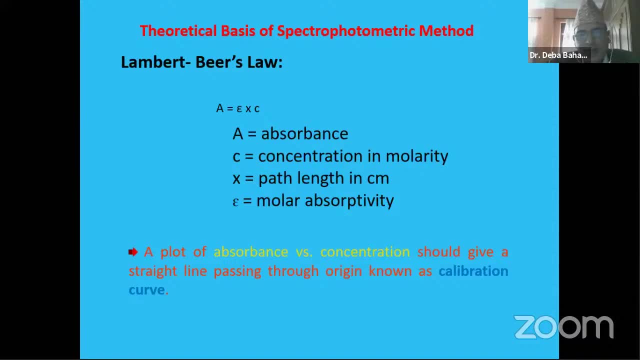 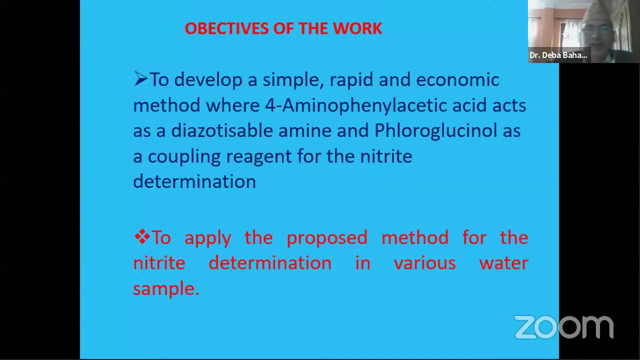 and x the path. By plotting the observance as a function of concentration, we can, by passing through the origin, we can get the curves which is known as calibrational curves, And the object of the study is to develop the 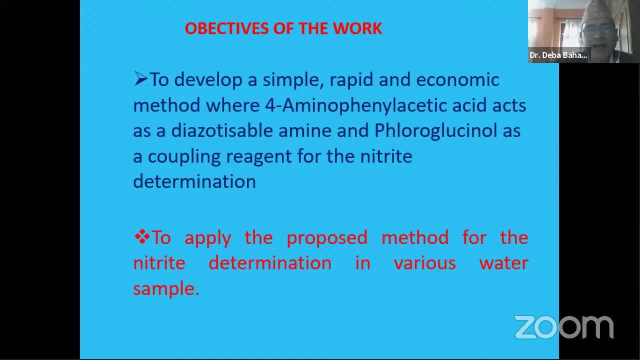 And develop the sensitive and methods where formalized as an active and some of the active and the active act as a disutable amine and fluoroglucan as a coupling region for the determination of nitride And the developed method is applied. 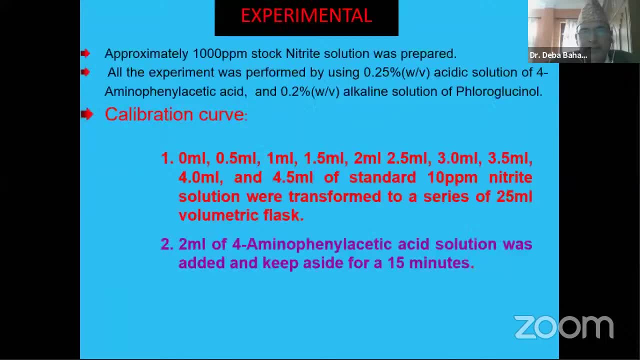 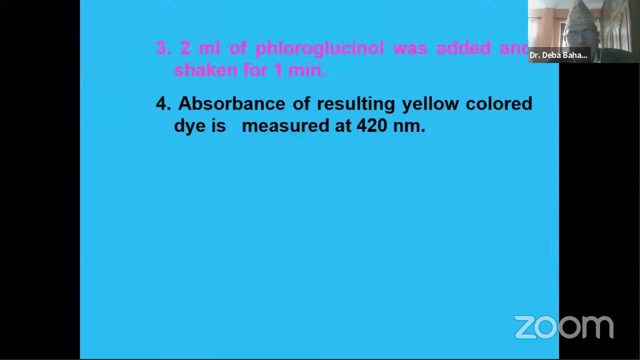 for the determination of nitride in various waters, Solutions and different types of regions has been prepared, and different amount of nitride solution is transferred in a 25 ml volumetric flux, and then the aromatic amine, 4-aminophenyl acetic acid, was added and kept aside for 15 minutes. 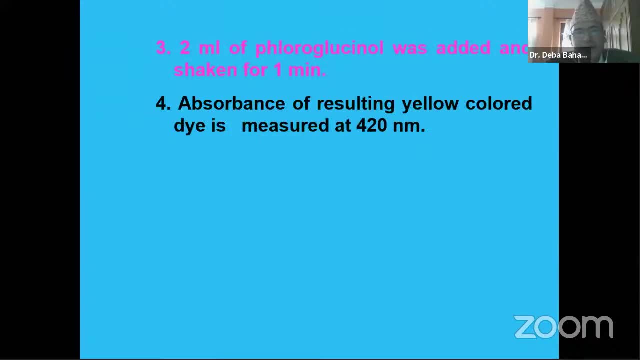 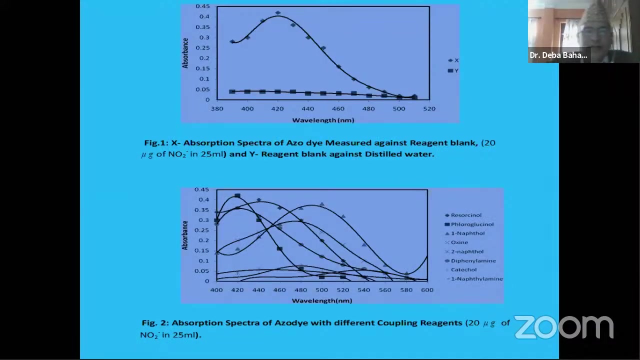 And 2 ml of fluoroglucan was added and shake well, And then absorption of resulting yellow colored dyes was measured at 400, 20 nanometers. Here I am presenting the two figures, How, one way we can determine the lambda max, by plotting the observance as a function of the wave numbers and one x and y. 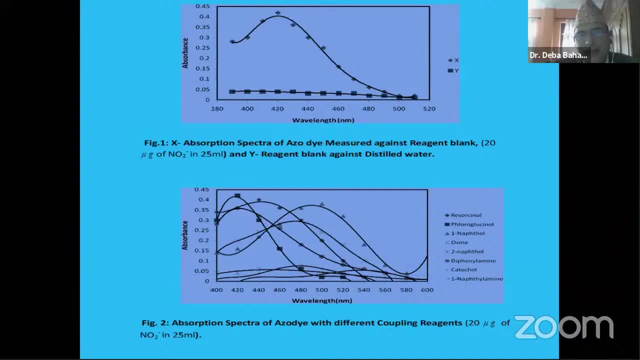 One is against the resin blank, Another is against the distilled waters. The lambda max is found at 420 nanometers. In this investigation, different types of- also coupling region has been tested and as a function by plotting function, as a observance, as a function of the wave number. 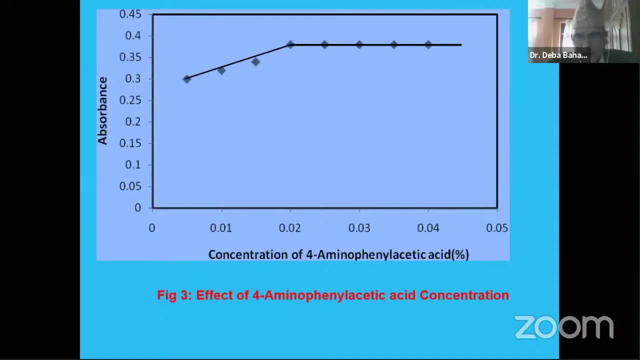 And for the recent optimizations, I have given the plot by plotting observance as a function of concentration of 4-aminophenyl acetic acid understandable. so i strengths 4 India альные color detection by adopting facts jadi, And then above the 0.02, absorption remains the constant and optimal concentration found to be 0.2%. 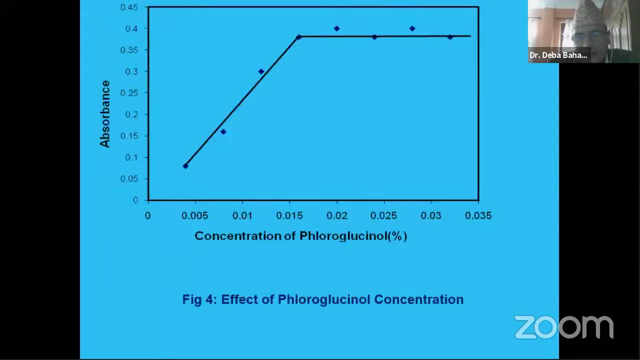 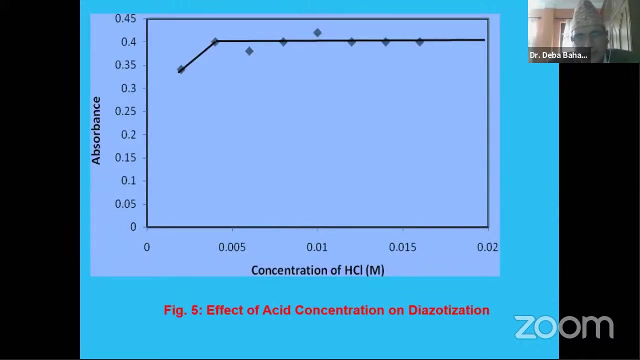 in final solution. In the same way, effect of chloroglycerin concentration has been optimized by plotting the absorbance as a function of the concentration of chloroglycerin. In the same way, by plotting the absorbance as a concentration of STLs. effect of acid concentration of 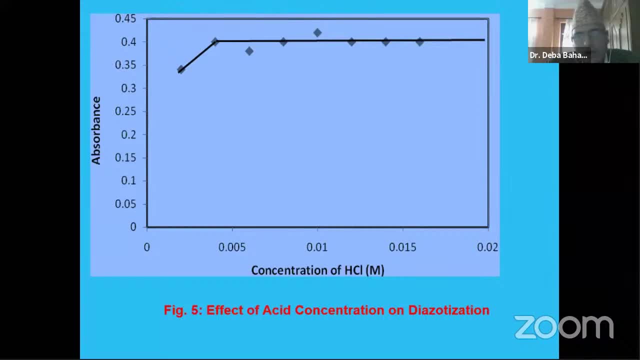 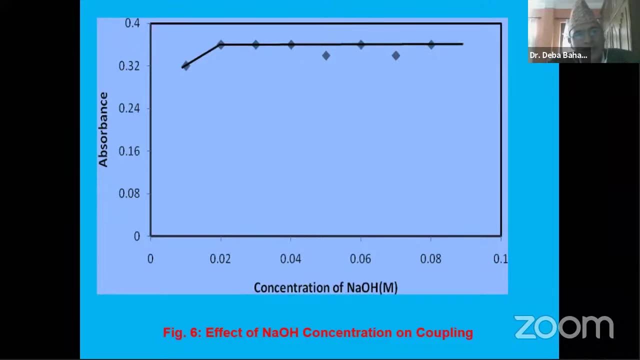 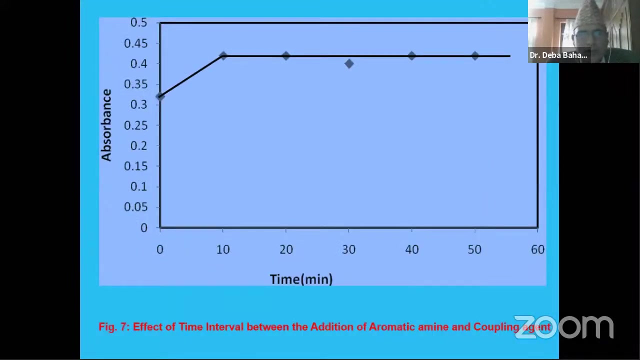 digitization has been also optimized And, in the same way, effect of ANUS concentration on coupling by plotting the absorbance as a function of the concentration of ANUS has been optimized by changing the absorbance as a function of the concentration of sodium hydroxide. Effect of time intervals between the addition of aromatic amine. 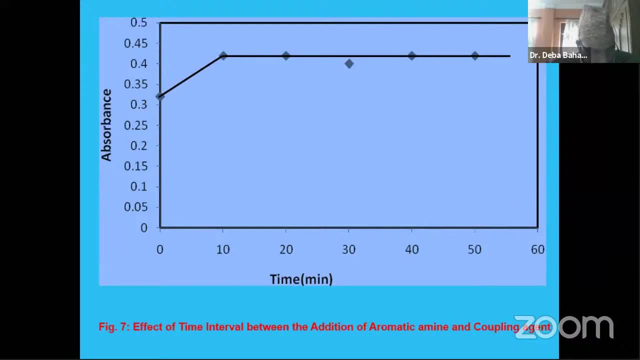 4-aminofluoric acid and coupling agent And by plotting the absorbance at the time in minute, the minimum times required. from the gravity is seen that minimum time required for the reaction should be at least 15 minutes. And adherence to by plotting the 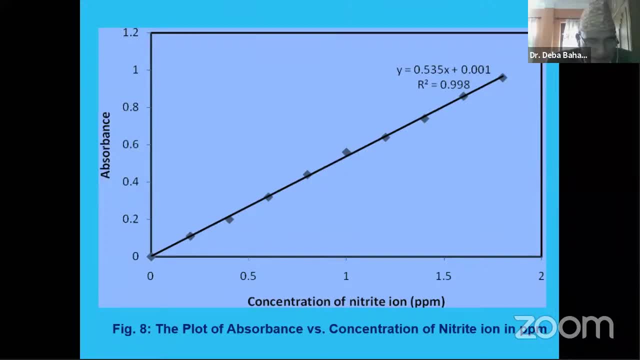 absorption as a concentration of nitrites, changing the nitrite solution So five micrograms to 50 micrograms in the final solution in 25 mL holy metered plus, following the recommended procedure, the absorbance of resulting azoidibs of Assassin's mom. 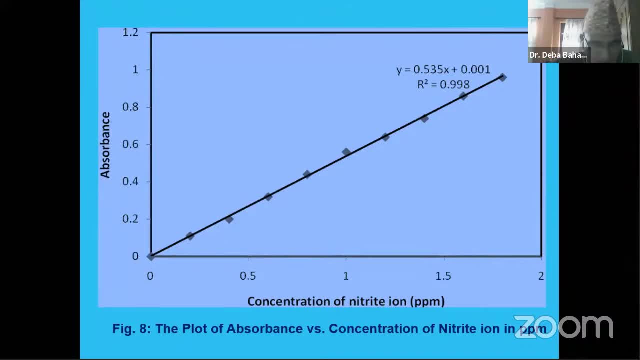 Effect of these quantitative measurements from ion waves in the same man at the immidiate noise. Azo dye is measured at 420 nm and from this we can find the method works well from 0.04 to 1.8 ppm of nitride. 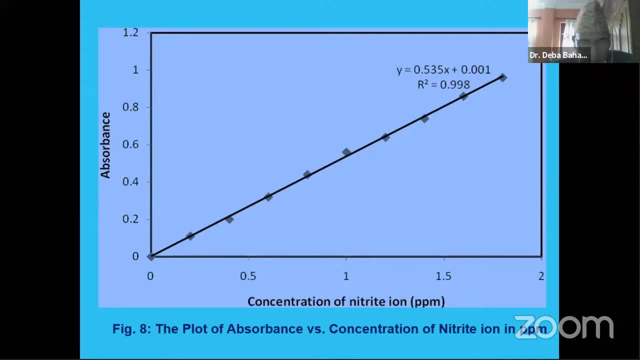 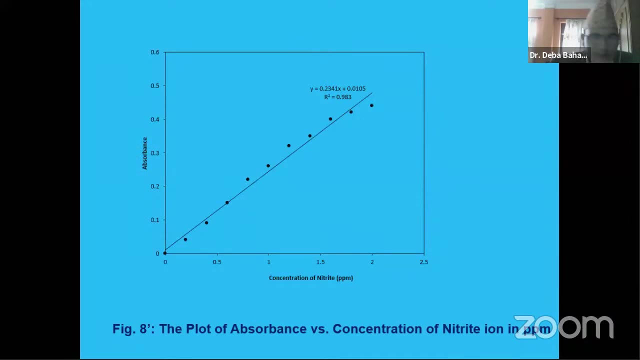 And from this we can determine the molar absorptivity sensor, sensitivity and correlation coefficients. In the same way, when the coupling region is taken as an example, by plotting the absorbance and concentration of nitride, similar types of parameters also can be determined. 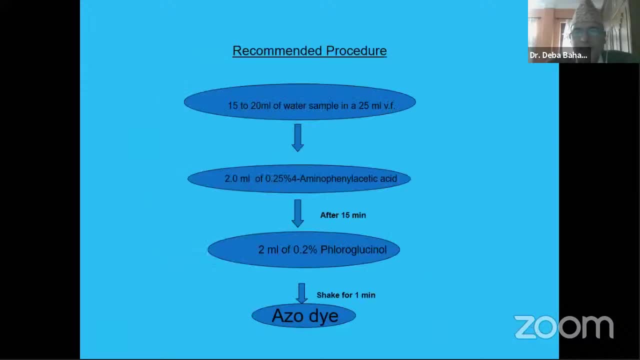 And these are the recommended procedures In the environment. sample like water: 15 to 20 ml of water, sample in 25 ml volumetric flask and then add 2 ml of 0.25% of 4-aminophenyl acetic acid. shake well about 15 minutes. 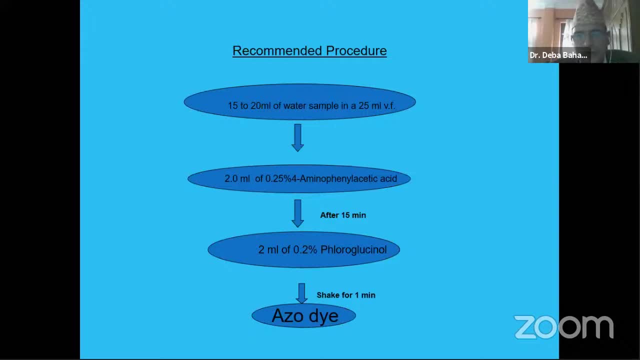 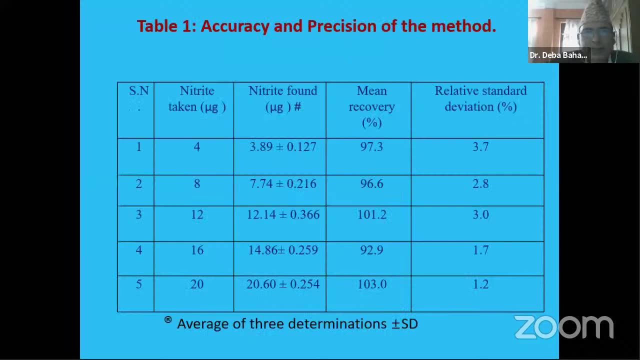 After 15 minutes, add the 2 ml of 0.2% pyroglycerol and shake well 1 minute. Then yellow color azo dye is obtained, And the accuracy and the precision of the present methods have been also tested under the optimized conditions. 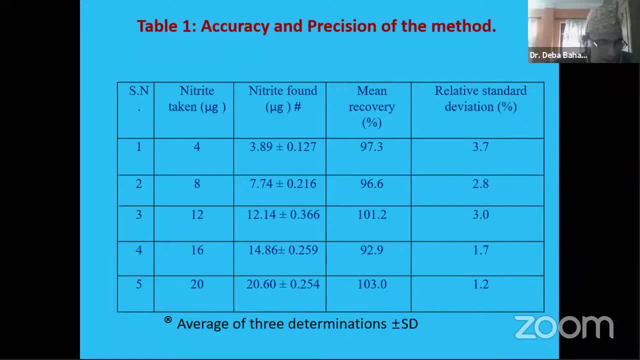 The accuracy and the precision of the purpose method was checked by performing the three-replicate determination of nitride. by taking the 4 to 20 micrograms of nitride in the final sample, We found the solution of 25 ml volumetric flask by the recommended procedure. 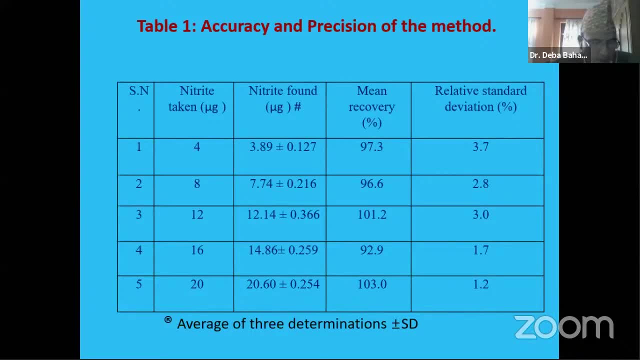 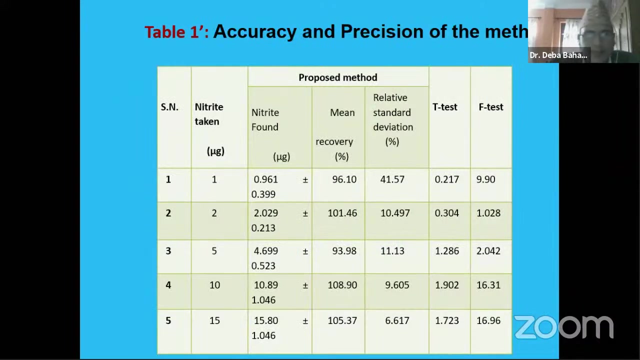 The percentage recovery was found to be ranged from 92.9 to 103, indicating the suitability of the method for the determination of nitride. In the similar way, the accuracy and the precision of the method also tested for the absinthe in the similar families. 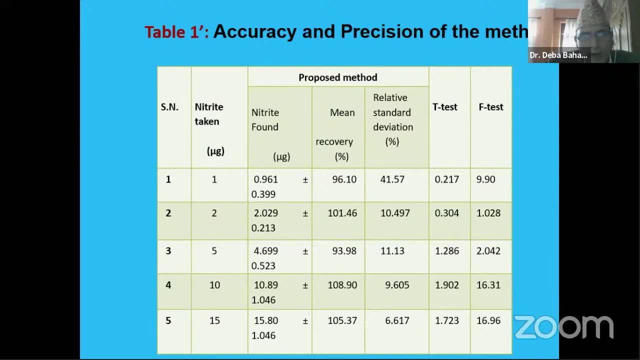 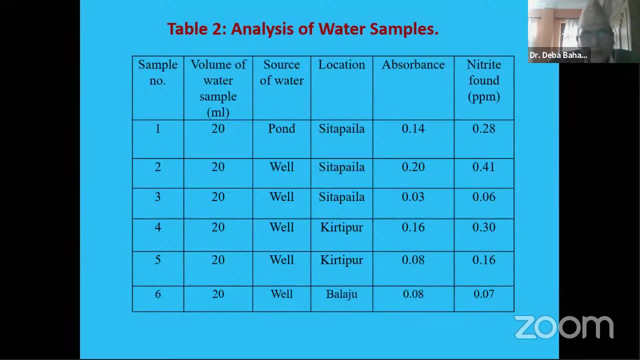 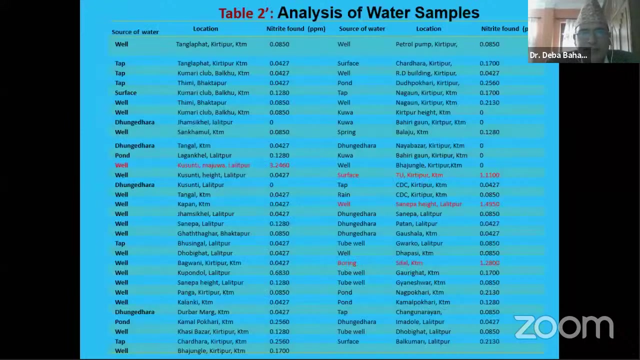 similar fashion by taking the nitride 1 to 15 and with the same parameters. also, the analysis of water sample has been done by taking the 20 ml of water sample and then the water sources like pond well in different locations of Kathmandu, and then we are getting the like this amount of nitride. and these are the some. 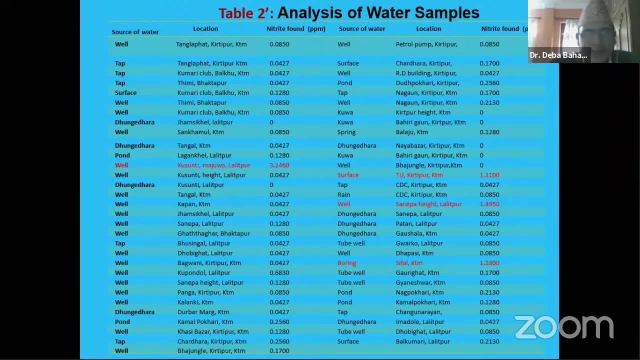 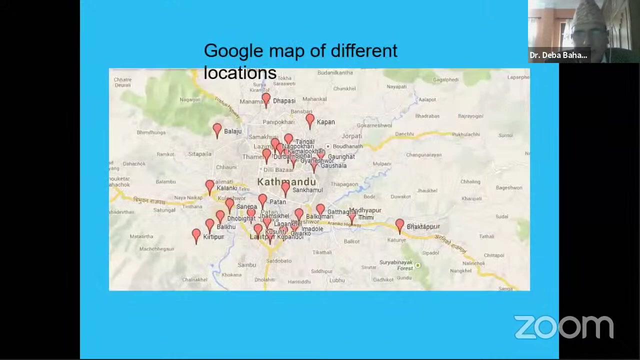 water samples taken in Kathmandu Valley in different locations, and, and, and by the recommended developed methods, and then we can see that somewhere above the permissible region, like in the well, and like this and this, and it means this: this type of study is very important. and which levels of nitride is useful for? 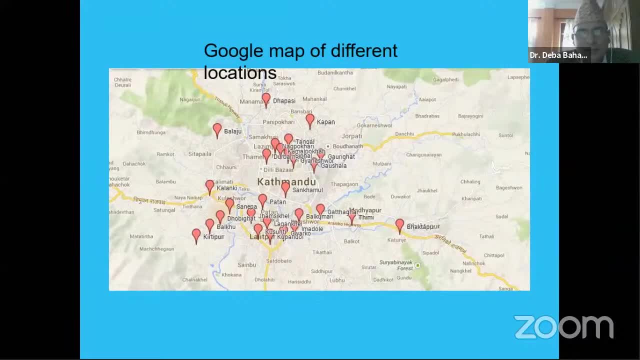 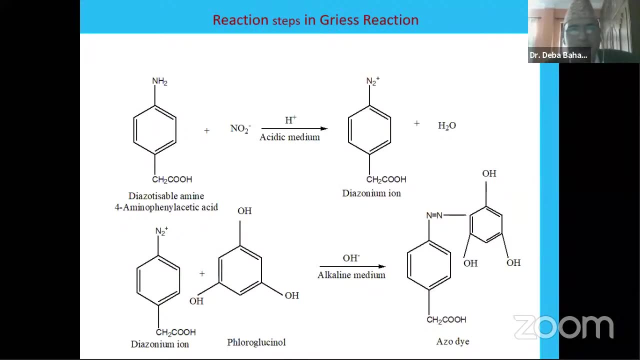 drinkable and this is the global maps of the Kathmandu Valley where the sample was taken and the reaction mechanism of the whole amino acid First for a full, that in the digestible amines and the folioglycines as a coupling. 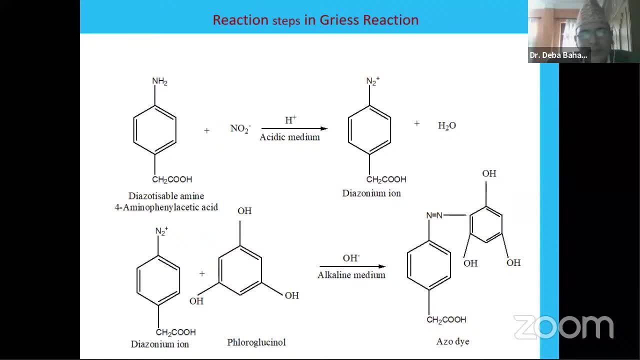 reagents, that means digestible amines, react with nitride in acidic medium to form of the diiodinium ion. and this diiodinium ion subsidence couples with the flouroglycines, as you see in the presence of alkaline medium, to form the yellow colored cathode dye. and this is 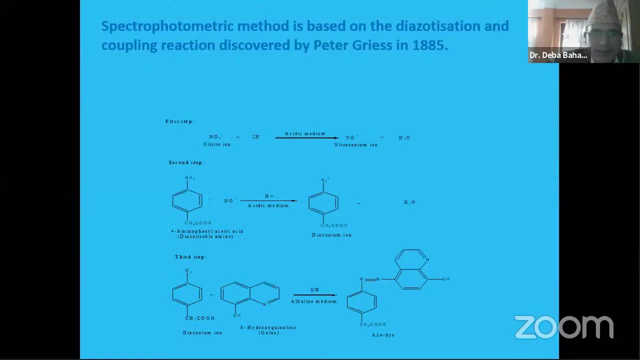 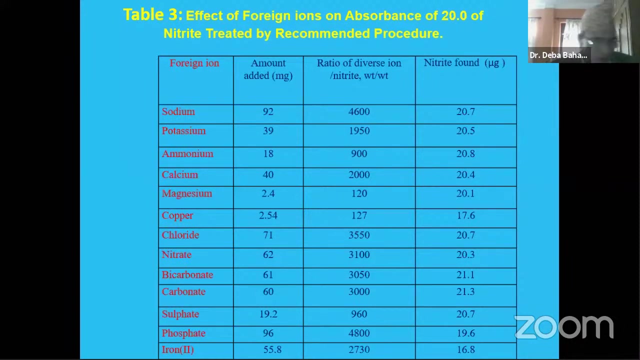 the next mechanism By using the opening region as a giant and based on the orange colors as a die will be pump. and these are the some foreign and has been also investigated, the foreign And that upon a company nitrides are examined by carrying out the determination of 20 micrograms. 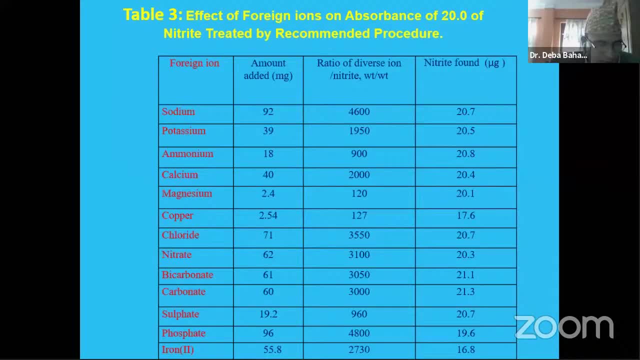 nitride in 25 mol volumetric plus with the foreign ions. following the recommended procedure, It is apparent that interference due to the most of the foreign ions negligibly small and the method seems to be seems to be selective for the determination of nitride. but copper and ferrous ion interfere seriously, while the magnesium ion and phosphate ion. 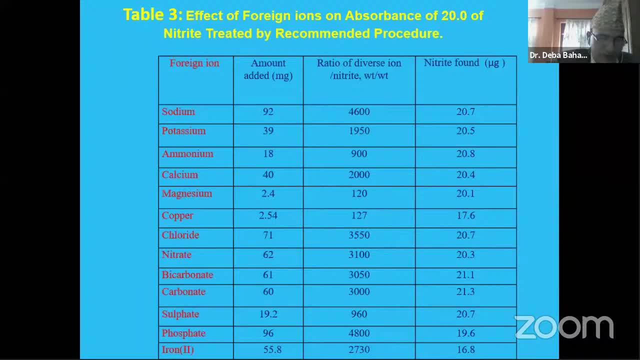 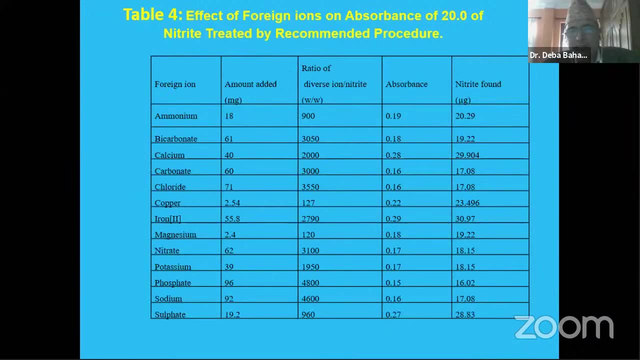 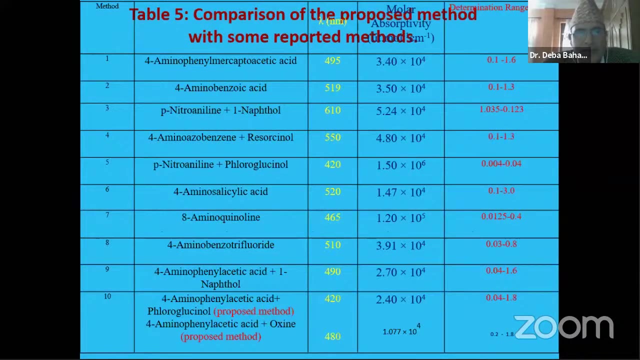 interfere by causing the turbidity of the solution. So this is similarly also tested by taking the obsidian as a coupling region and this is the comparison of the present developed method with the reported results and, as you can see here, the by 4-aminophenyl acetic acid and 4-glucanols and with lambda max molar observability and with this 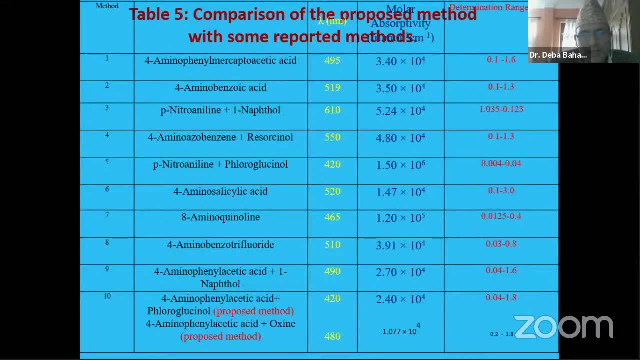 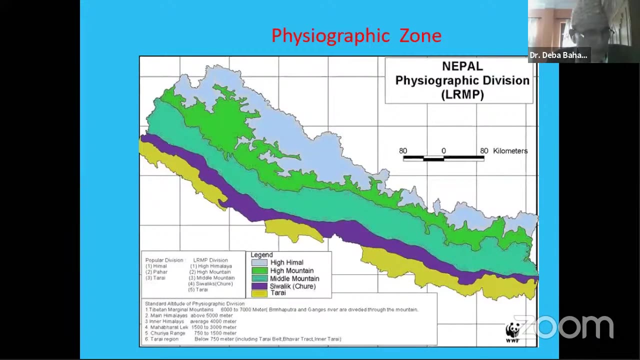 range and with 4-aminophenyl acetic acid obsidian and with lambda max for acting with this molar observability and with this range. So next one I'm going to or discuss about the climate change and its impact. So from the first ones, as I already mentioned, that is based on the 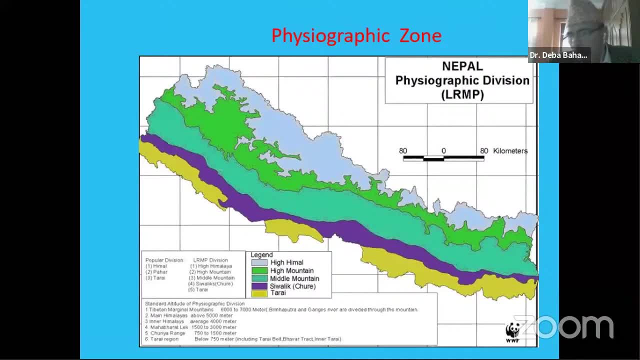 primary data and that is very useful. So in order to manage the biodiversity or to reduce the reduce the pollutions in the waters, also in soil samples. So if you know the fundamental aspect and then based on, we can also by this develop method, we can also apply it and 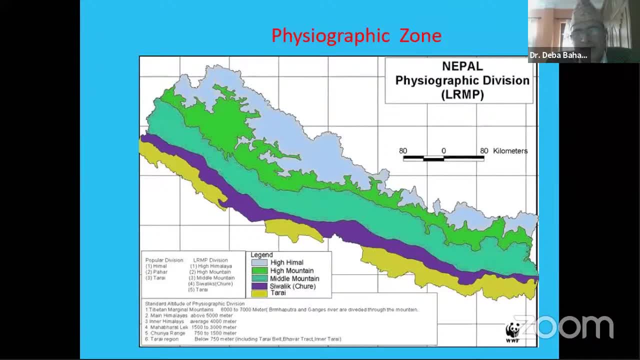 determine the what amount of nitrides is a pollutions or not. and by having this types of idea we can manage the our biodiversity and a good ecosystem and then healthy environment for the human being, for the environment, So the plants, for the earth. So we can kick, save the earth also, weekly clean the our. 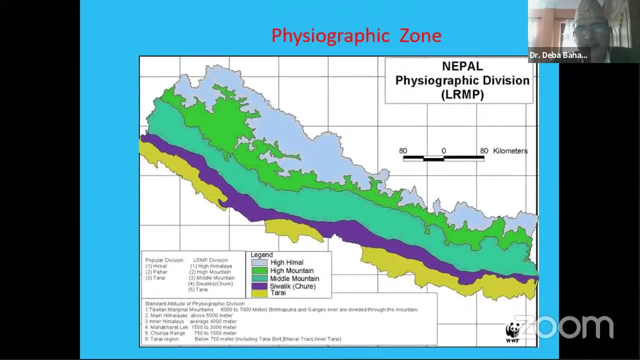 environment. this is the one of the way of the basic and fundamental and applied research And in the another aspect, I am so one of the so participants or organized committee told that. so they are expecting some of the so data from the Nepal. So but I am not experimentalist about the climate change, but I have taken some of the data. 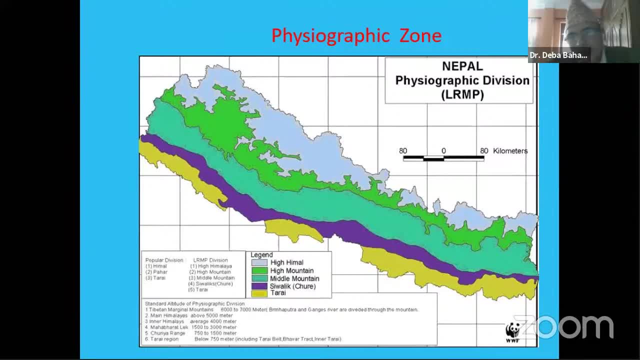 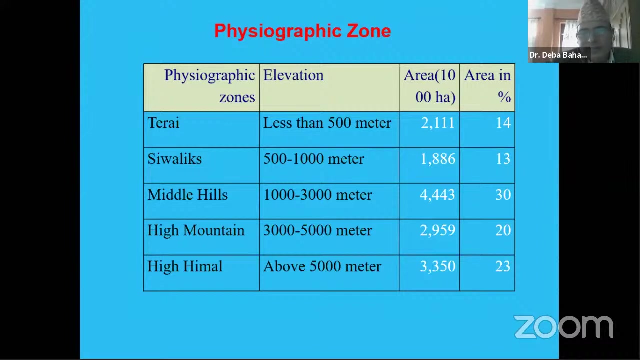 for the presentations in this e-conference, with the limited times, and this is very interesting. You see, it's the map of Nepal, so we have, like Tarai Siwa lake, high mountains, and this is the Himalayas, and then this is the height and this is the percentage. 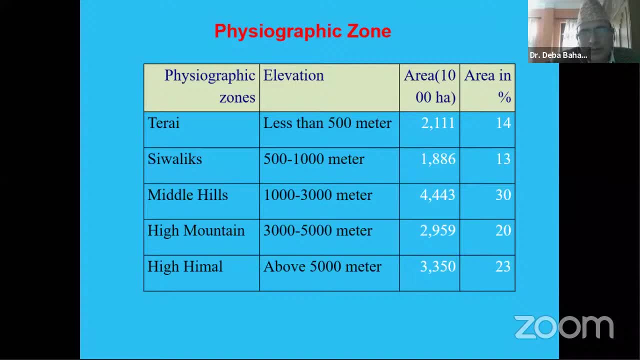 and this is the height and this is the percentage. so that means which area of the land is located in Nepal. so you can see that means from low land to high land. so it is a beautiful. in order to state the biodiversity as a reference, Nepal, and then we can also compare the data around the world. so 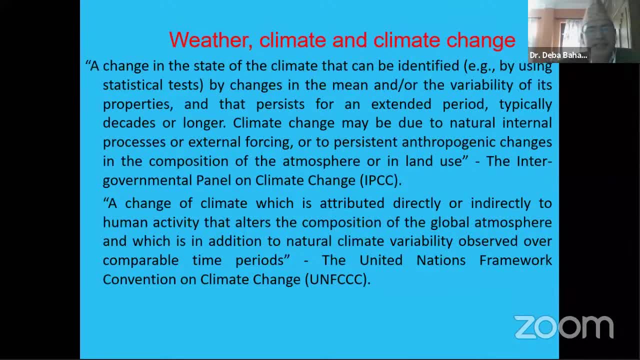 the weather climate and climate change. there are two types of definitions, so that means how the variability of property and the persist for an extended period, type decays or longer climate change may be due to the natural internal process or external focusing, or to persistence. 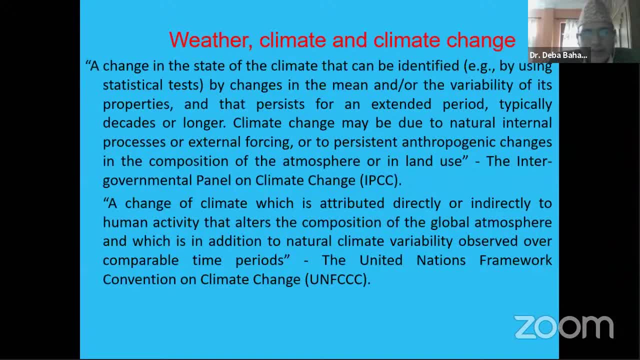 anthrazonic change in the composition of the atmosphere or in the land use by this. this is the, the intergovernmental panel, or climate change, and another definition is change of climate which is attributed directly or indirectly human activity that alter the composition of the global. 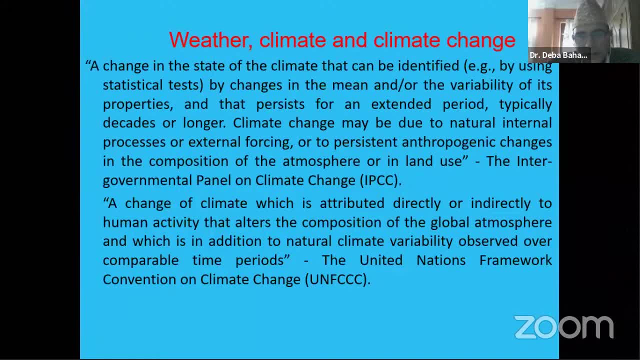 atmosphere and which is addition to natural climate variable observed comparable time period. this United Nations framework conservation climate change information. so it means by the human activity, so different parameter will be affected. so in order to control the, by definition we have to control our human activity. and that is also used only for useful purposes, not for destruction. 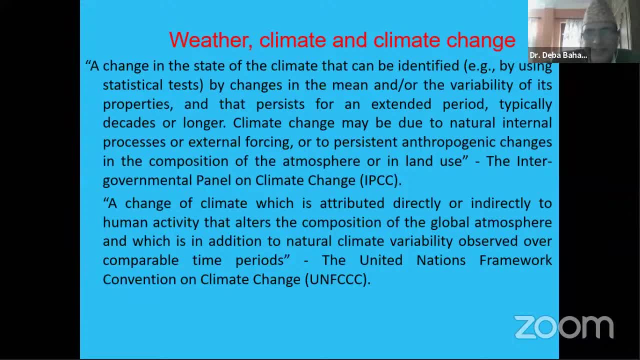 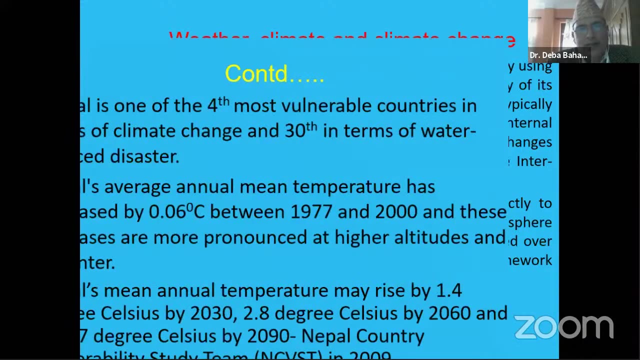 and then our humankind will be safe and our earth will be safe. so in such a way, if we use in the reduce, reuse and recycle, and then we can save the earth, and then we can save the environment, then we will be safe. 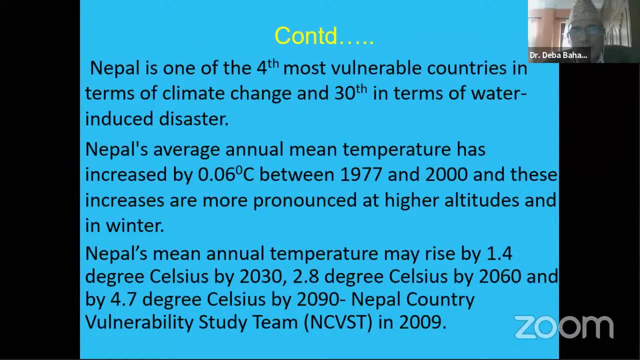 Theothermal energy is a very common resource. it is a very familiar resource, but for the young people it may be a very different technology. It may be a very different source of energy than the renewable energy energy, but it can be a very different resource for the people residents of the community. 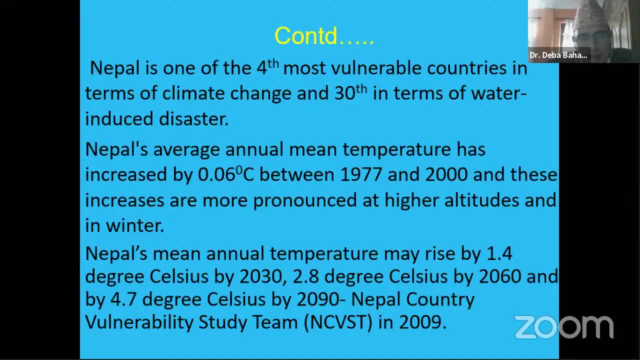 so it is a very, very common resource. In addition to the water, water can be used for waste management and very important for natural airflow. Nepal's mean annual temperature may rise by 1.5°C by 2030,, 2.8°C by 2060, and by 4.7°C. 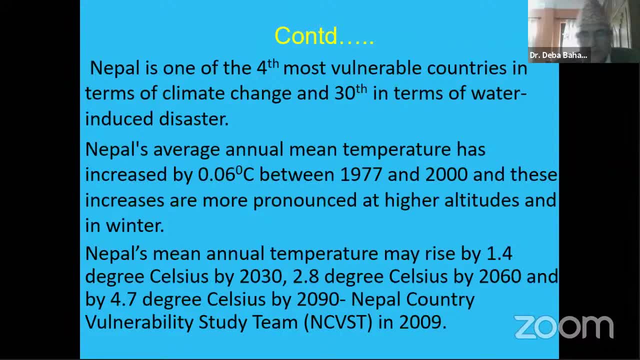 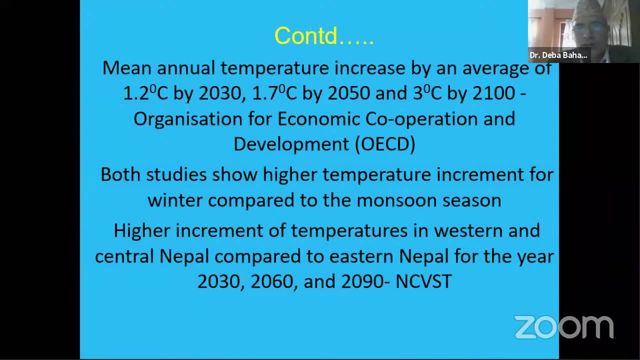 by 2090.. Nepal's country voluntary study teams, abbreviated NCBT, in 2009.. These are some secondary data. Also the temperature, also by organizations for economic cooperation and development. the temperature average temperature: 1.2°C by 2030,, 1.7°C by 2050, and 3°C by 2100.. 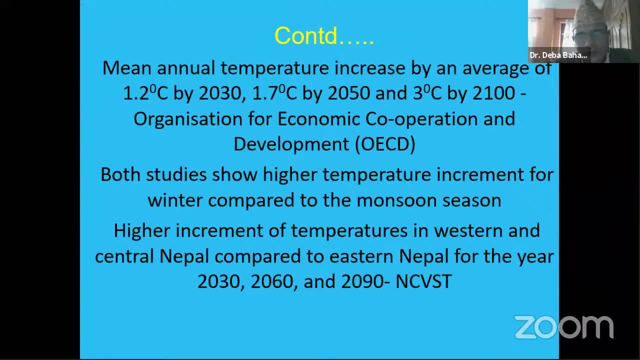 And both studies show higher temperature increment: winter compared to the monsoon season, higher increment of temperature in the western region And the central Nepal compared to the eastern Nepal for and by 2030,, 2060, and 2090,, according to the NCBT. 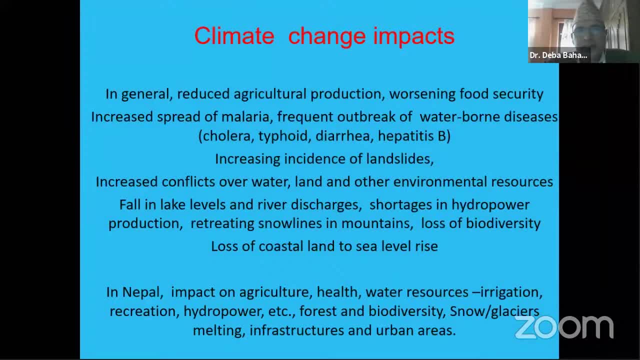 So climate change and impacts in general: reduction of agricultural production, worsening of food security, increasing spread of malaria, frequent outbreak of waterborne disease, different types of diseases Like cholera, typhoid and so on, Increasing incident of landslides, increase of conflict over the water and landslides. 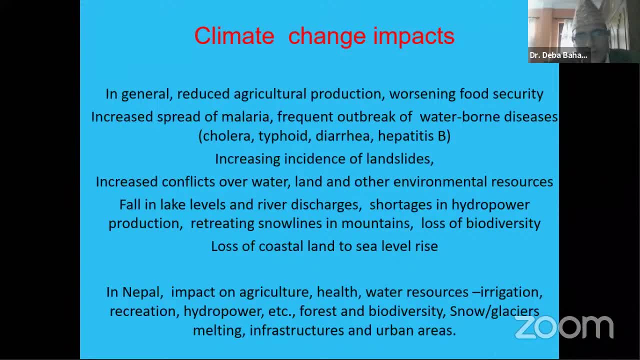 of the environmental resources. hole in lakes levels and the river discharges, shortage in hydropower production, retaining the snow lines in mountain, loss of biodiversity, loss of coastal land to sea level rise In Nepal important. this is the not only Nepal's. around the world's, this type of 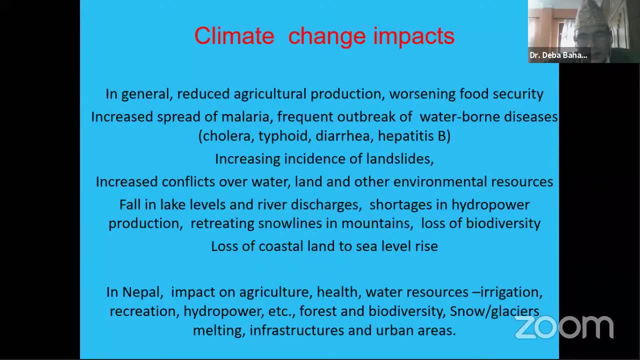 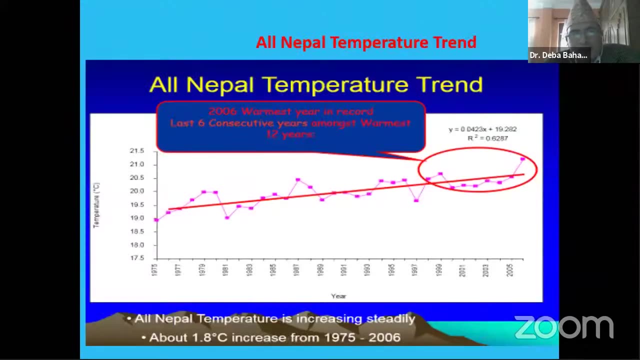 impacts may happen in Nepal: impact of agriculture, health, water resources, irrigations, recreation, hydropower sector, forest biodiversity, snow, glaciers and urban areas, And this is one of the examples. So train about the all temperature. train how changes from 1975 to 2060, that means 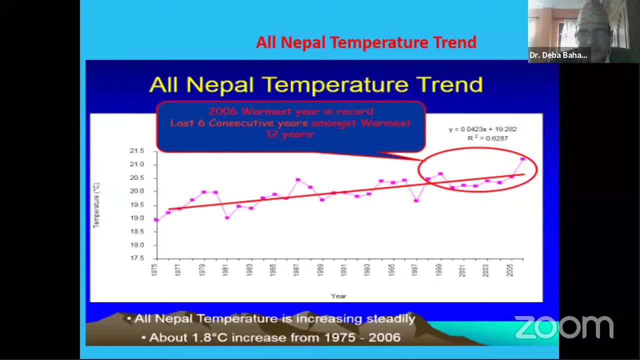 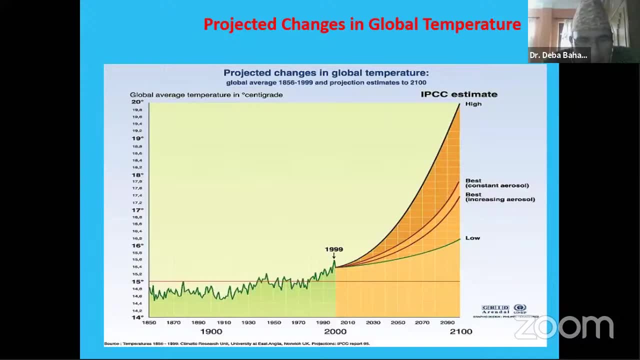 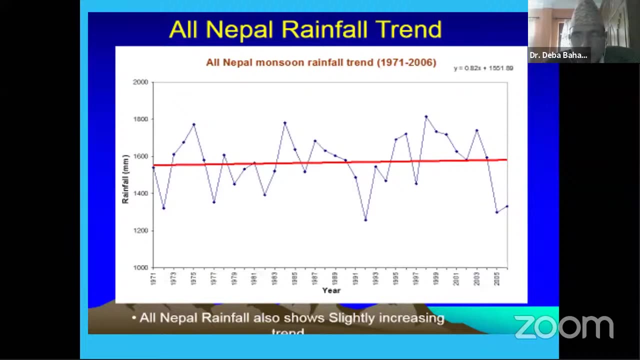 about 1.8°C- And this is not only Nepal's- around the world. So that means 1850, so 1990, also predicted for 2100. Also similarly so in Nepal. rainfall also shows this slightly in Nepal- 2060, also. 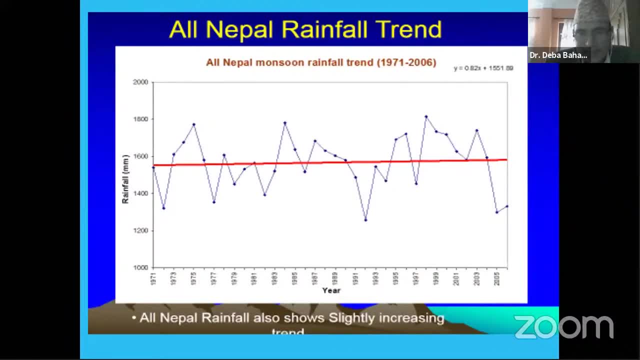 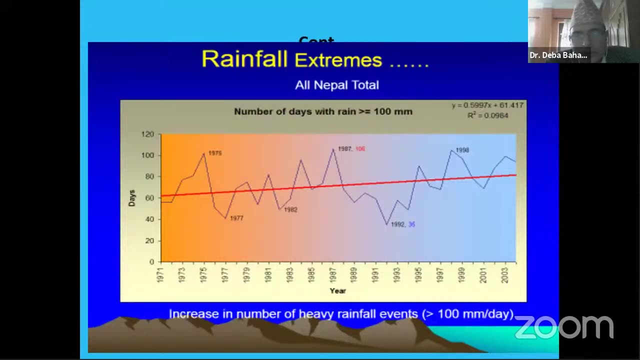 somewhat in Nepal And this also this slightly increasing trends from 1997 to 2006.. Also, increasing number of heavy rainfalls events. so that means greater or equal to 100 millimeters. Also, these years we have very big rainfalls so that means it was almost very high in the last 30 years. So we have 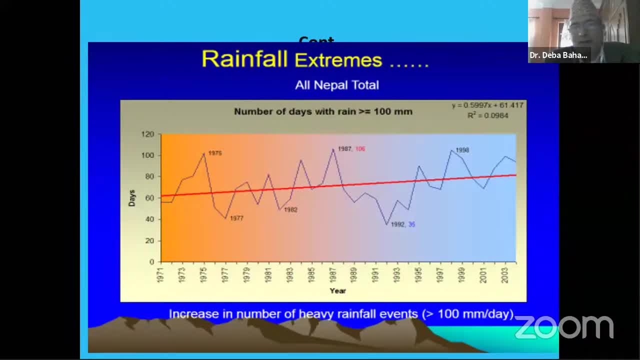 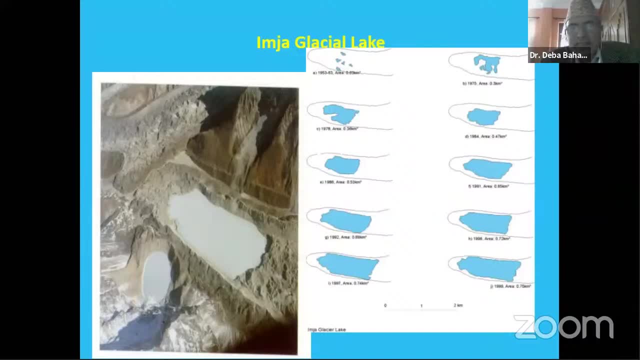 disasters in different locations of Nepal. This is the Imza Lake. As you see, it started from 1953 and it is increasing. In 1975, the area is increasing As you can see. this is the area in 1999, so a lot of increase. Now. that means these types of lakes. 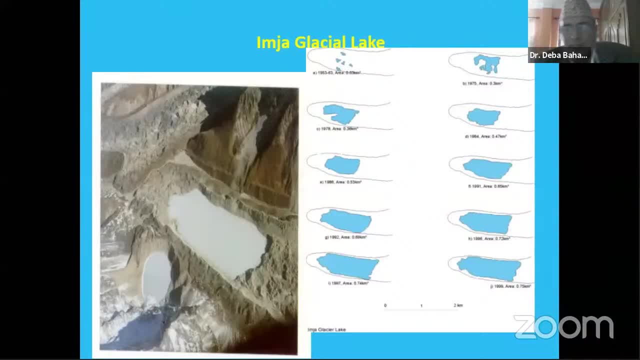 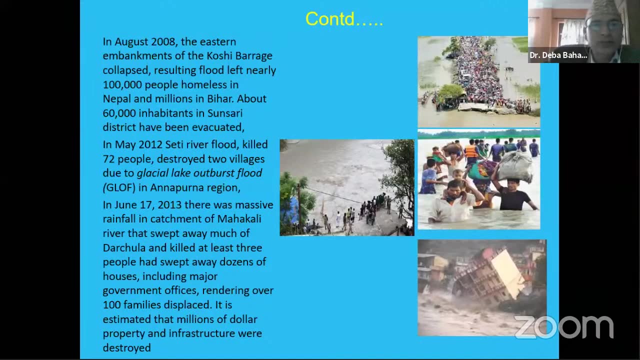 So we have a big problem in the Himalayan regions. These are some of the examples that are shown in some parts of Nepal, also in India and other parts In August 2010,. a strange environment of the overcast has occurred. 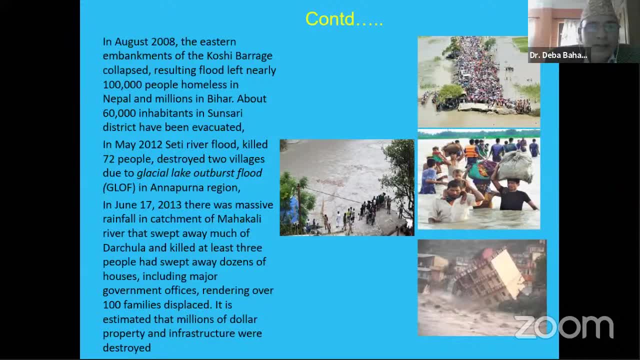 river side. So that means there are problems. Several people- one lakh people- homeless Nepal and millions in Bihar. About 60,000 inhabitants in Shunsari districts have been evacuated to Nepal. In May 2012, Shetty River floods. that means in Nepal killed 72 people, destroyed two villages. 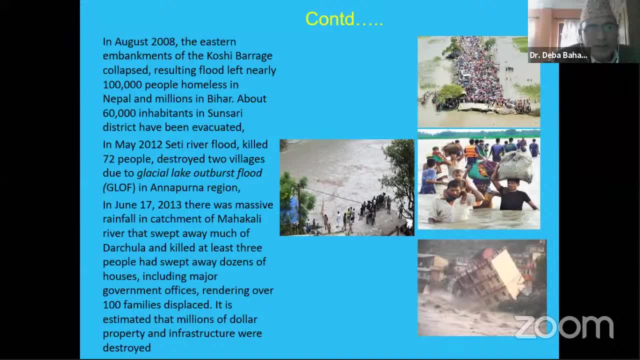 due to a lake of outbursts, floods everywhere In June 2017, 2013,. there was massive rainfall in the catchment of Mahakal River in Nepal that was sifting away most of the darchula and killed 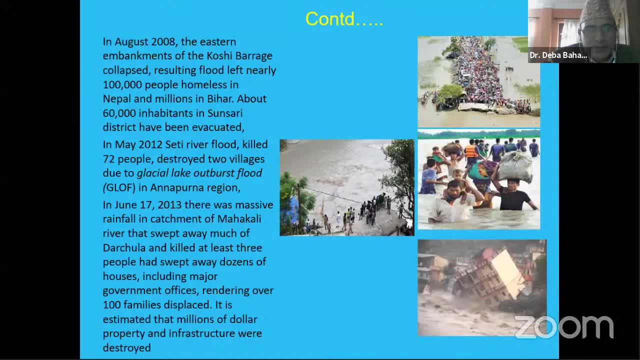 everyone. There was a massive rainfall in the catchment of Mahakal River in Nepal that was at least three people and had swept away a dozen of houses, including major government offices, rendering over the hundreds of families displaced. It is estimated that millions of dollars 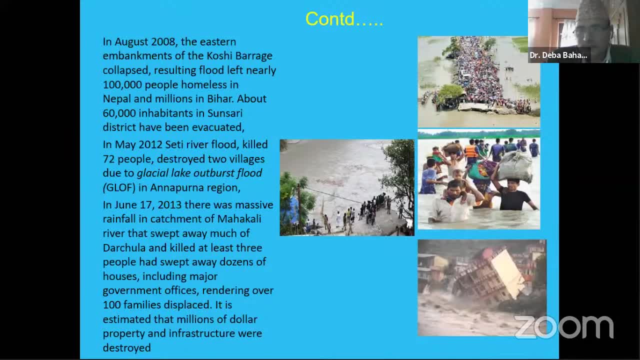 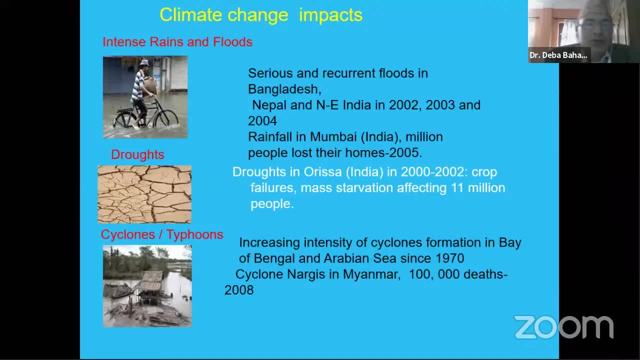 were brought in after this. you see Also the intense rainfall and some like this intense rainfall, some drops and cyclones and typhoons. I can bugger Bangladesh, Nepal in different dates, also in India, like Orissa in India 2000-2002,. 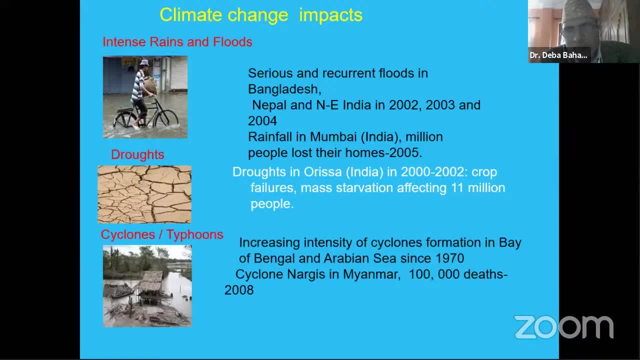 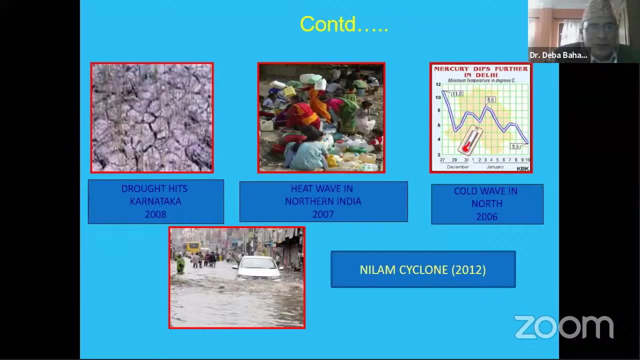 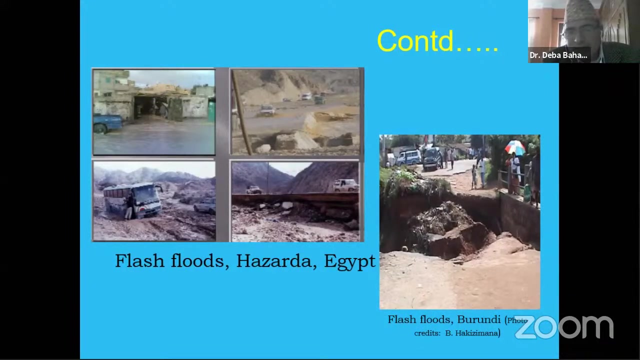 and this old data so increasing in terms of cyclones, Bay of Bengal, also in Myanmar, so that was happened, And also like drop hits in Karnataka, heat up in northern India also in Delhi also Neelam cyclones, so that means floods also hazards in Egypt. also flash floods in Burundi. 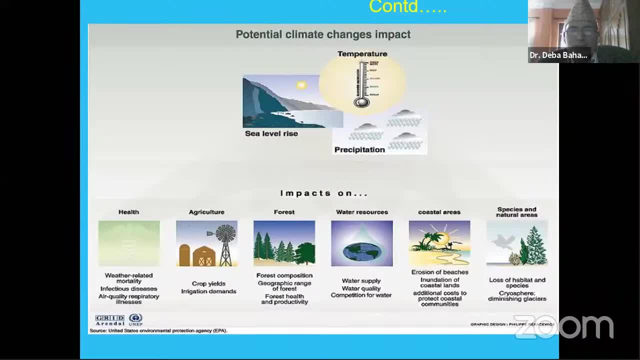 So that means there are some parameters. climate change impacts like temperatures, sea level rise and precipitation Due to these parameters contribute impact On the climate change. so that means in the health, weather-related mortality, infectious diseases as quality and respiratory illness. 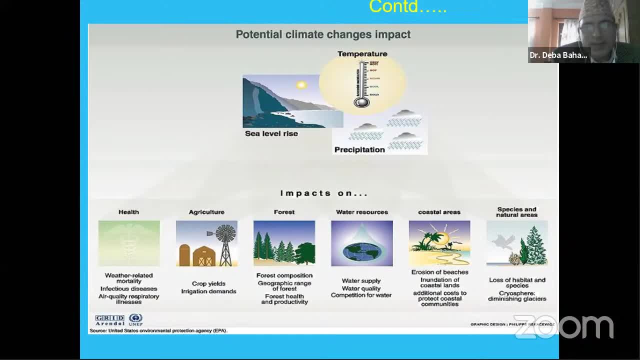 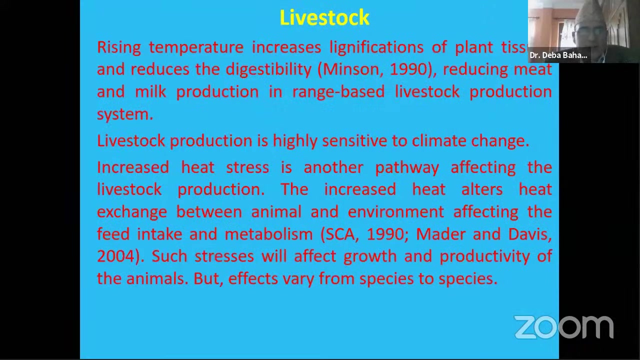 So in the agriculture, crop yields, irrigation demands, in the forest, so also in the water resources, water supply, water quality, competition for waters or coastal areas. also species, different types, lots of different types of species. So also this is for livestock productions. 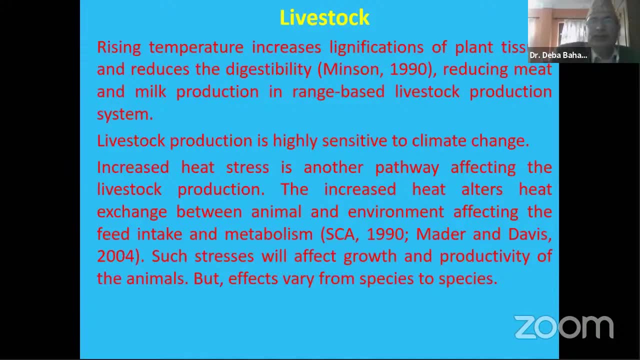 So by rising temperatures. so this is indicated here, so by the reference. So livestock production is highly sensitive to climate change. increased heat stress is another pathway affecting the livestock production. It alters the exchange between the animal and the environment, affecting heat intake. 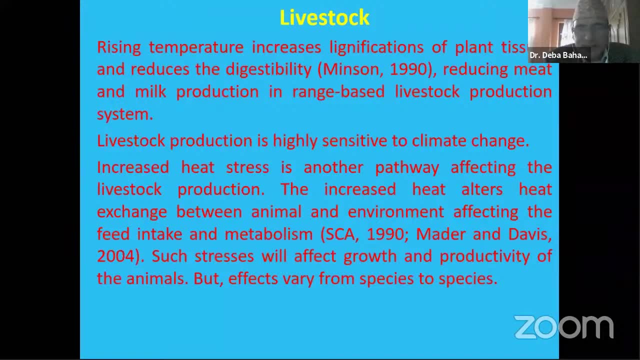 and metabolisms. By this I have taken this one And such issues will affect the growth and productivity of animals, but effects vary from species to species. So that means by climate change, so it will affect so living beings in every aspect. 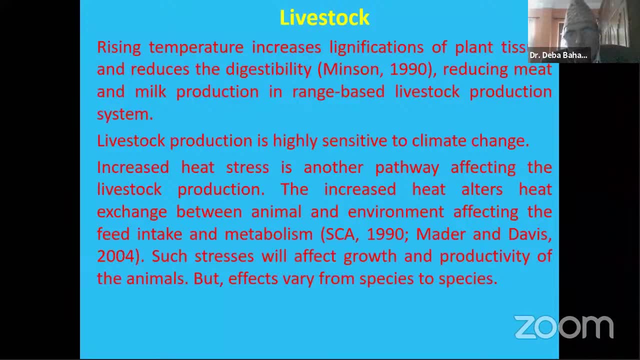 so for like So food production, Food production, Food production, Air quality, as you see, that means the food production. So that means different variety of field. it will affect, That means when it will hinder the our, so human being, that means our humankind will. 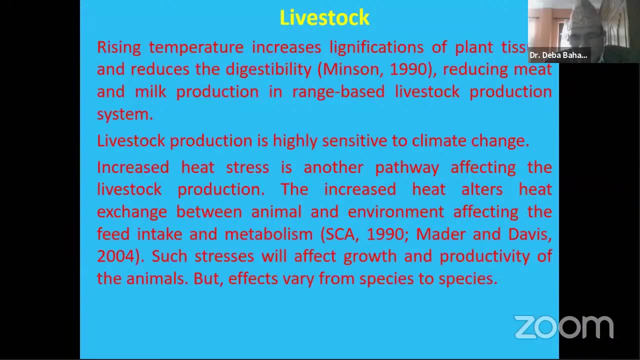 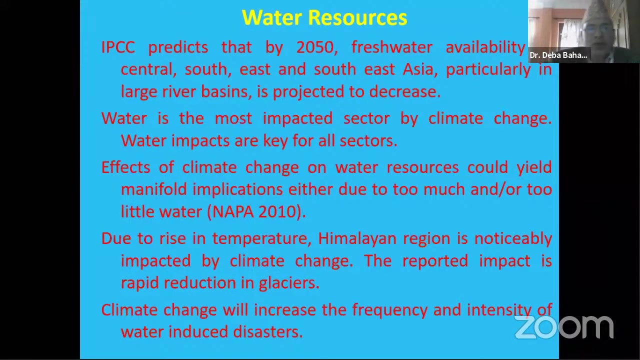 be disturbed, all the biodiversities also disturbed, and then we are out of order. So our system will be collapsed day by day. So this is a very important topic, but also this is the part- the waters. so that means 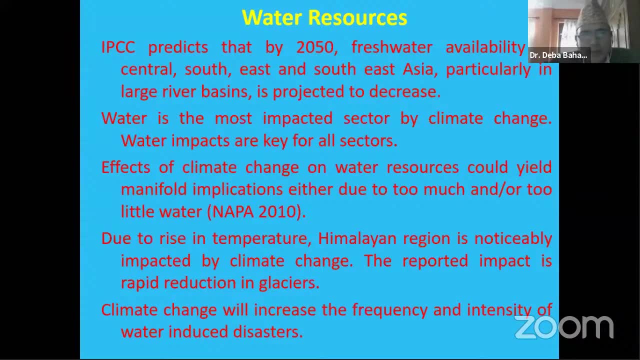 water is the most impacted sectors by climate change. Water impact are key for all our sectors. even climate change on water issues could meaningful implication, either due to the too much or little water, if flood or something, sea level rise And dropped. 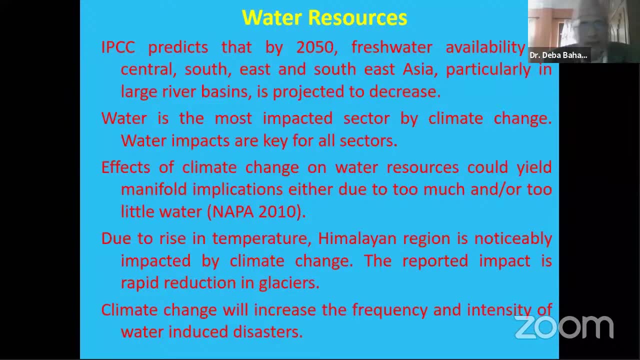 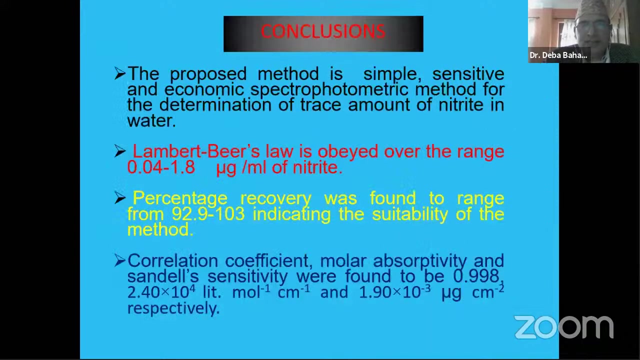 So that means different problems by the water Due to the rising temperature. himalayan region is noticed impacted by climate change. the reported impact repeated reduction in glaciers. Climate change will increase the frequency and intensity of the water-induced disaster. So in the first ones. so some of the so conclusion I have drawn. the purpose is very simple. 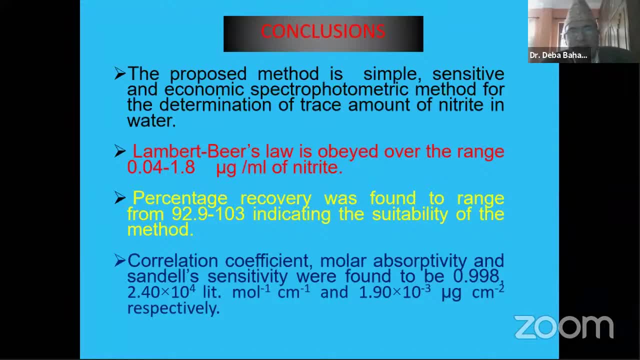 Nothing's the end of the world. Looks like the end of the world. So what is the end of the world? simple, sensitive and economical spectrometric method for the determination of the test amount of nitrate in the water, And Lambert-Baird's law is obeyed over the range 0.04 to 1.8 microns. 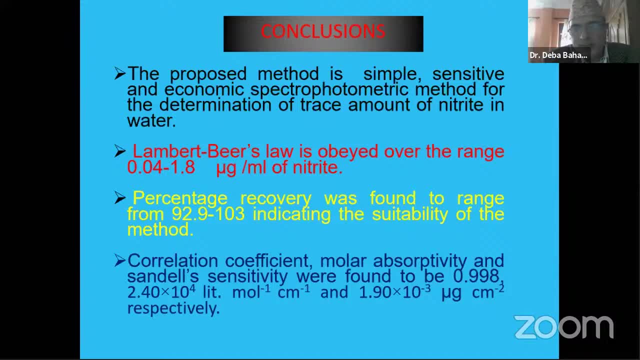 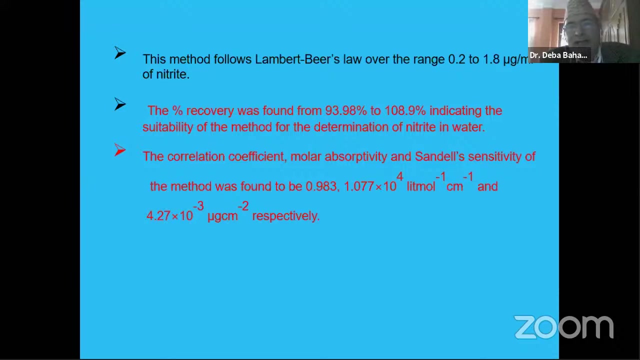 per ml of nitrate, Potential recovery was found to range from 2.9 to 103. indicators of the method, correlation coefficient of molal sensitivity and sensibility of the method was found with these figures. In the same way, when we are using the oxyne as a 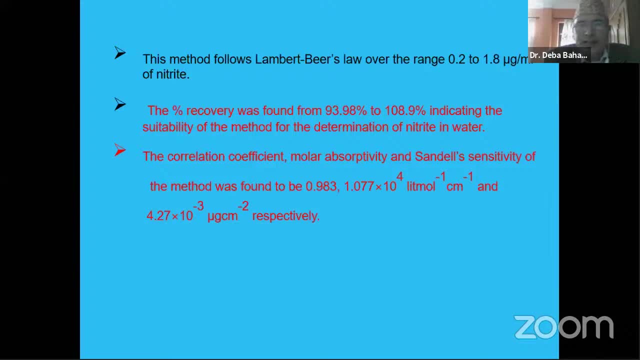 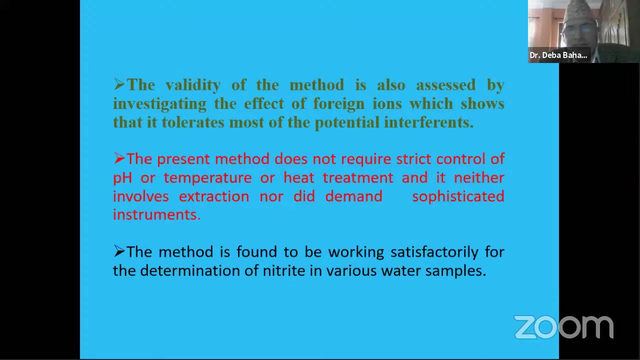 coupling reagent and this is the range. so with this range it is applicable and this is the potential recovery and parameter correlation coefficient of molal sensitivity. sensitivity were found And also the present method doesn't require the strict control of pH. 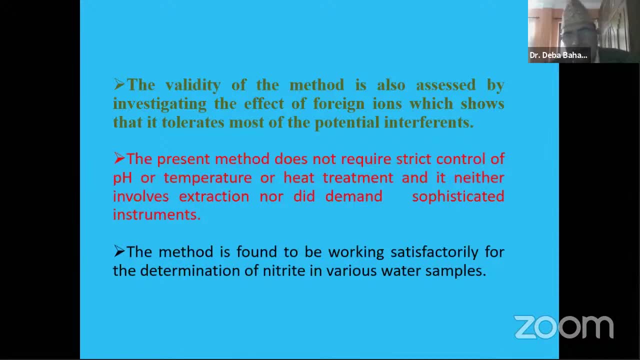 temperature heat treatment. It neither involves extraction nor demand, So physically the method is found to be acceptable for the determination of nitrate in various water samples. Also, some of the reagent has been also tested for the determinations of sweat. 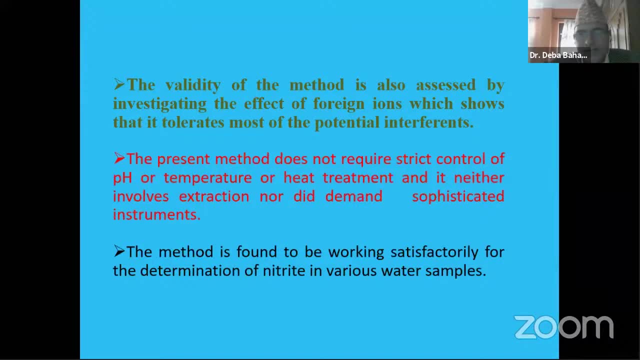 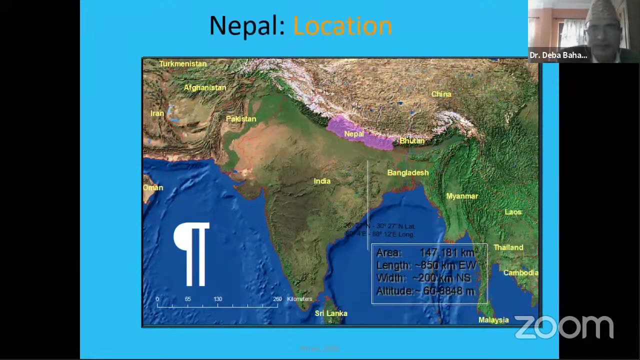 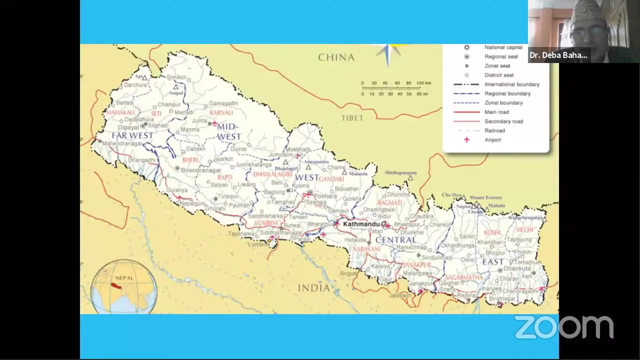 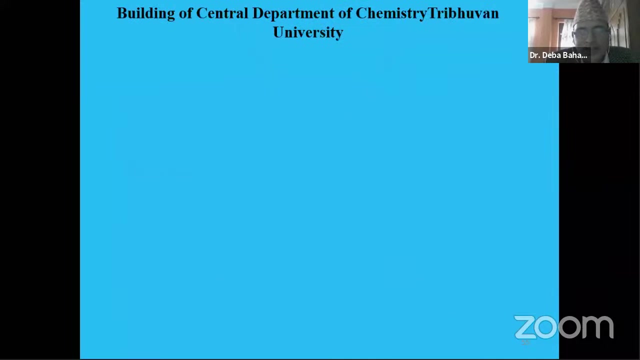 and the temperature of the liquid. So this is the map of the water samples. So we are the so NIORS, So this is the so more detailed maps, And this is the mountain Everest, which is known as so Sagarmatha, head of the sky, And this is the my department central. 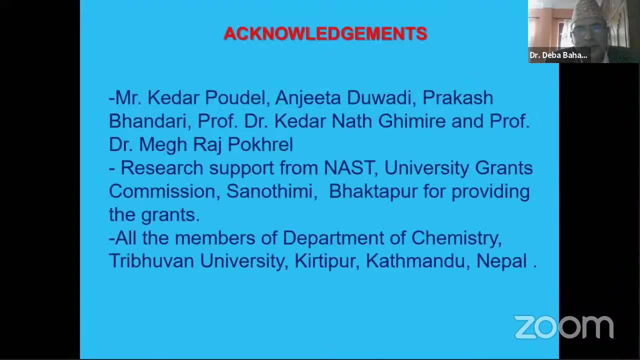 department of chemistry, Pirogan Institute. So this is the map of the university, some of the stars, So acknowledgments. So I would like to thank some of my colleagues, and that means my students, like Kedar Podal Anjitha. 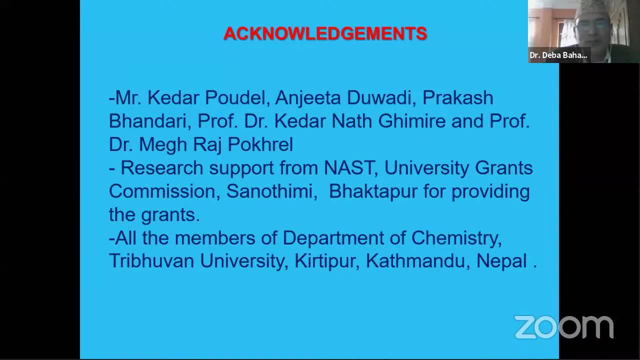 Dwari Prakash Bhandari and some of my colleagues, Dr Kedar Ghimire, Dr Meghraj Pokhrel and the research support from the national. that means Nepal Academy of Science and Technology University Grant Commission, Chanity Bhaktipur Pirogan Grant- all the member of department. 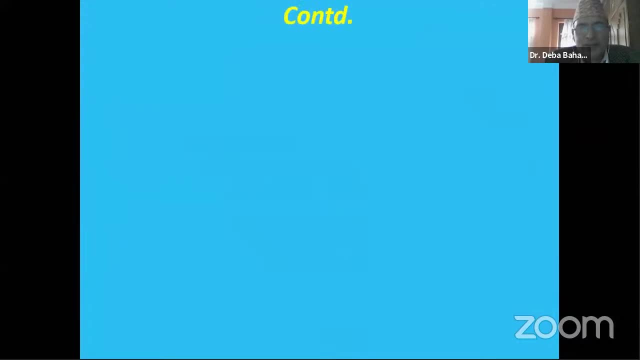 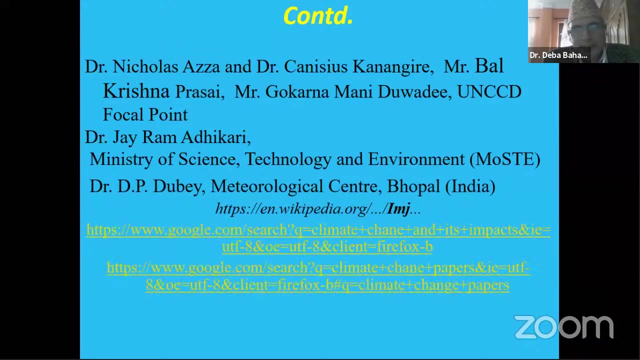 chemistry at the university Kirtipur And for the second data, I have taken some of the references with the this, our scientists and some of the publications, and these are some of the references of the proposed research. Thank you. 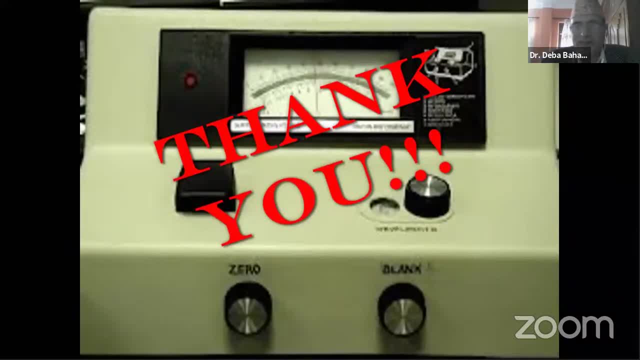 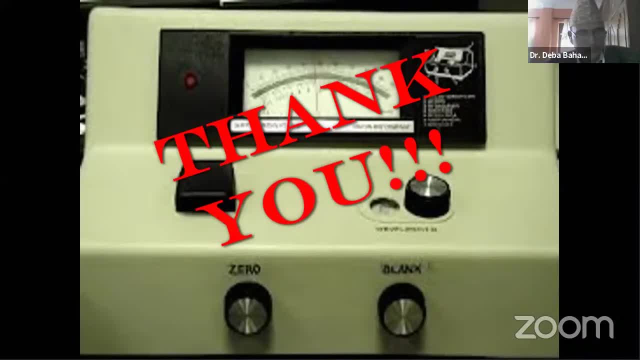 many fold. professor deva in his lecture he said the biodiversity conservation is very important for good ecosystem. he said nitrate determination is essential. he described many methods of nitrate determination through his slides and and. in his lecture he said: how can environmental be protected by monitoring? 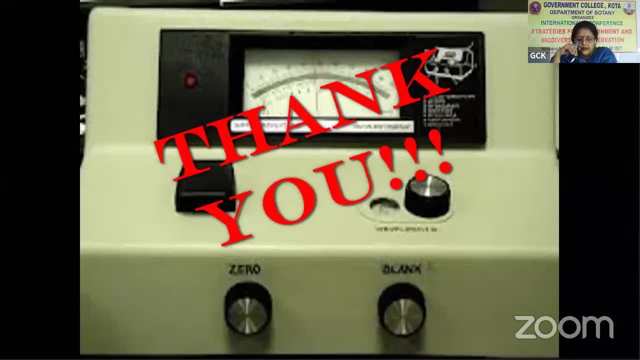 element concentration in environmental and by various methods- he said the- by chemical analytical method. he suggested to make environmental pollution free, for erosion free. thank you, prasadeva. now we'll turn the time over to our next speaker, dr varna andrew wernker, immo state university. all the way from immo state, nigeria. 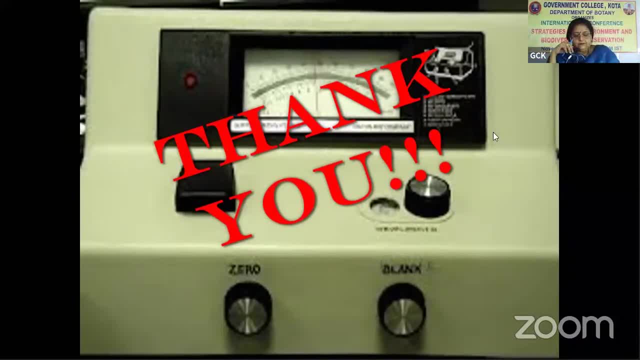 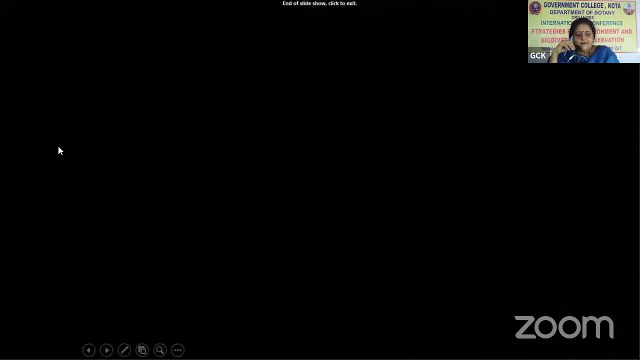 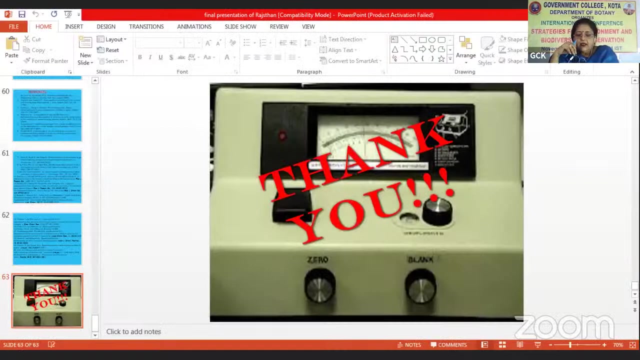 prof varla. yes, sir, is it audible, sir, hello? yes, sir, yes, it's audible, i'm here. yes, welcome sir. yes, uh, professor, his field of interests are environmental pollution studies and analytical chemistry too. it is an honor to have an opportunity of interacting with the remarkable prof wallah. 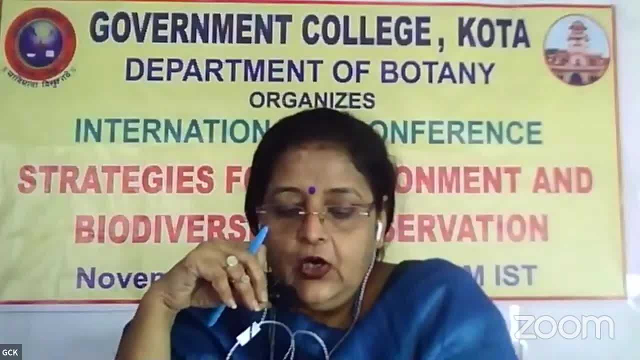 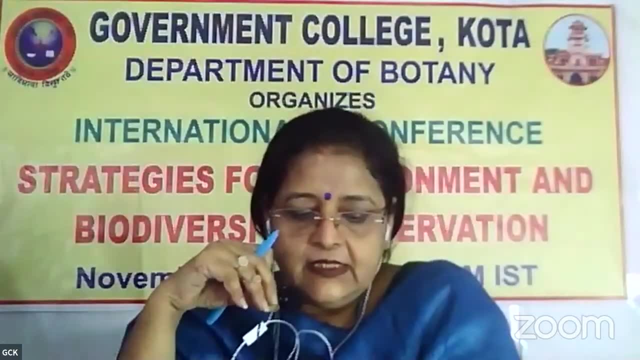 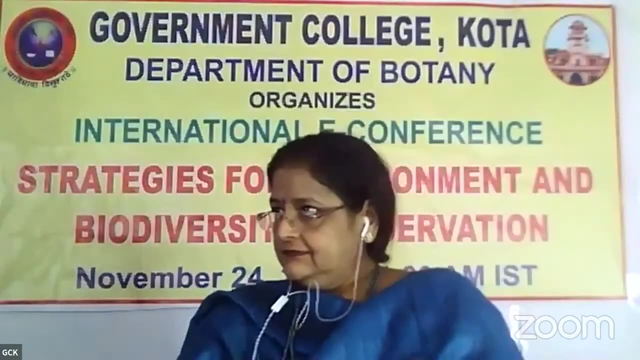 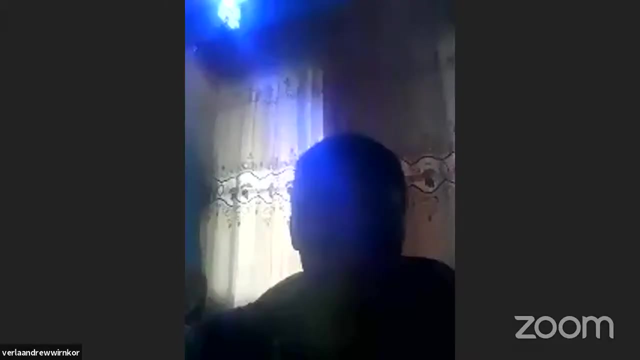 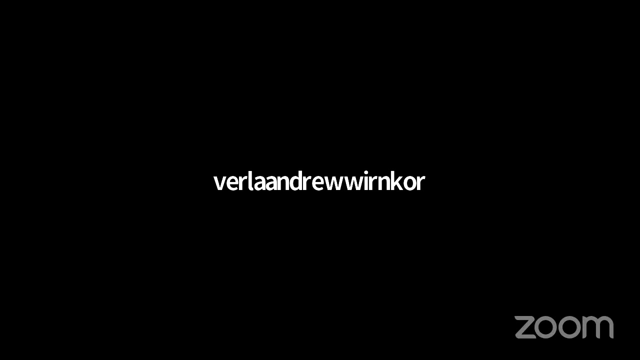 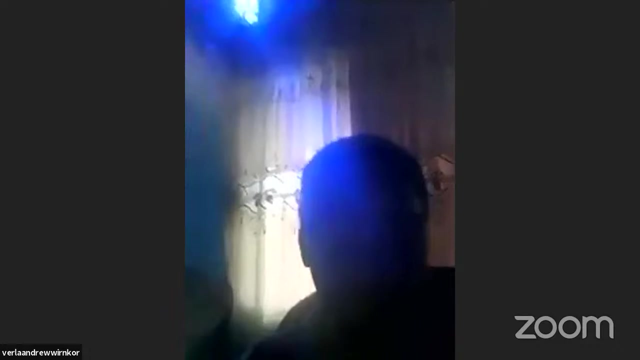 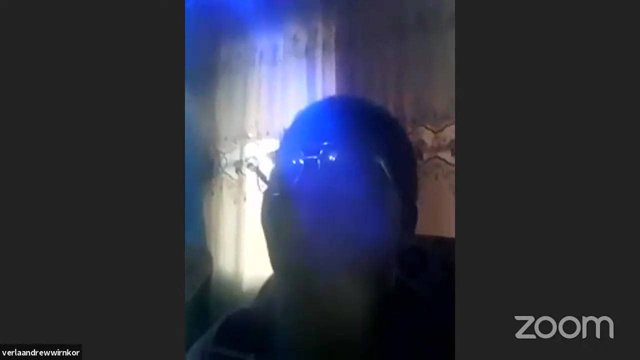 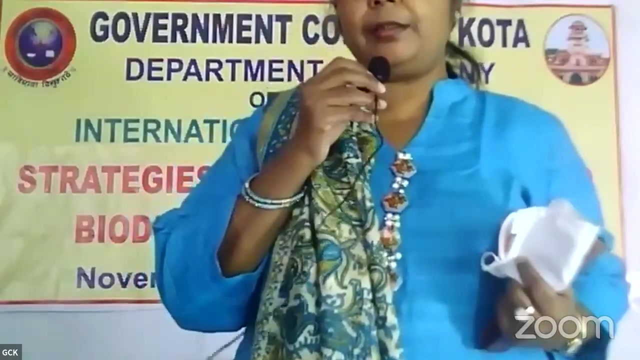 and listening about his works and views on biodiversity conservation, the theme of our international e-seminar today. yes, sir, i request you to join sir. yes, sir, start, sir. okay. so humai is going to JEFF. qué way, hello, hello, hello hi. welcome, dr varla. 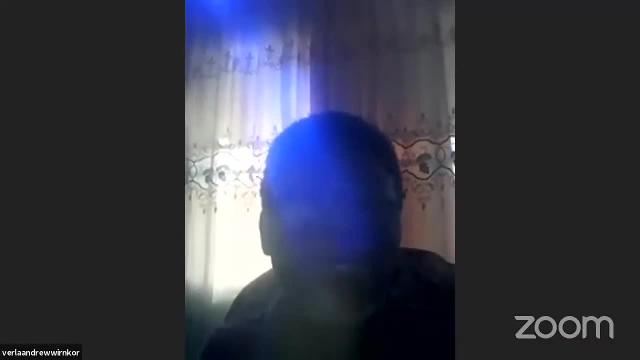 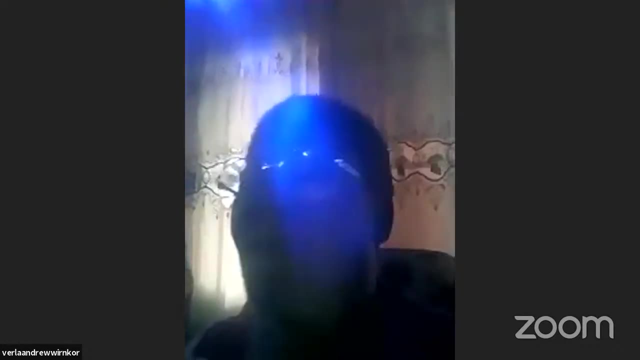 sir, sir, please join namaste, yes, namaste. Dr neji, thanks for this wonderful opportunity, yes, Namaste, to talk to you and your students and to India, about my concept of biodiversity conservation, And I am saying that the topic here is going green as a tool for biodiversity conservation. 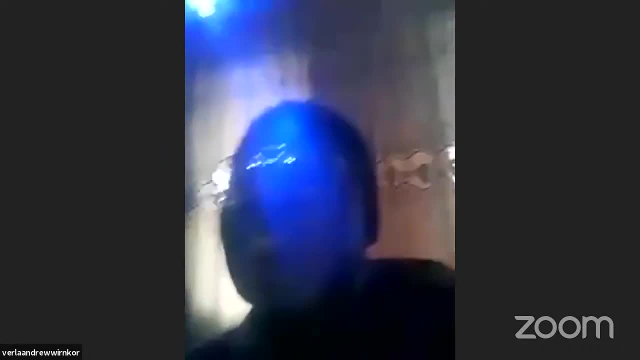 As a way of background, I want to say that man's activities have disrupted the natural balance of the environment and the very nature that is meant to sustain, And here I've listed major causes of biodiversity loss. They include habitat alteration, pollution, over-harvesting of natural resources. and climate change. I equally want to say that human activities future prominently In all of these factors. therefore, to put an end to biodiversity loss and to conserve biodiversity, must be checked and reduced to the barest minimum. As a way of introduction, I want to say that biodiversity 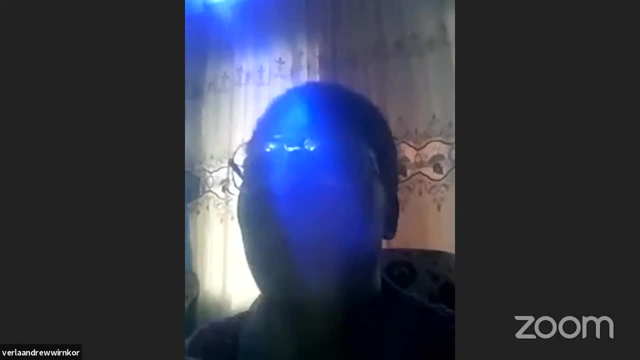 is the life wire of our planet, because man obtains clean air, fresh water, drugs, food, shelter and all the needs from the environment. But within certain limits the environment can sustain humans and biodiversity. Of course, biodiversity is a species, the functions Hence biodiversity makeup must be, of course, very important- of natural resources. Here I have pointed that currently, population growth and the consumption of our natural resources have placed an over demand on the natural resources from man's environment. So what is the statement of my problem? 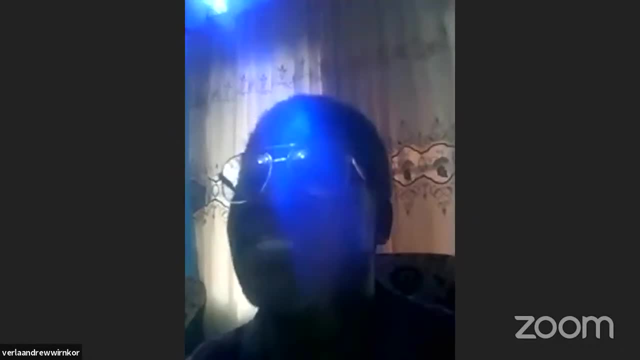 The statement is simply that species are getting extinct and they are being destroyed Again. about 99% of species that once lived are now extinct, While 45% of the forest is lost, 50% of mangroves and 10% of coral reefs. 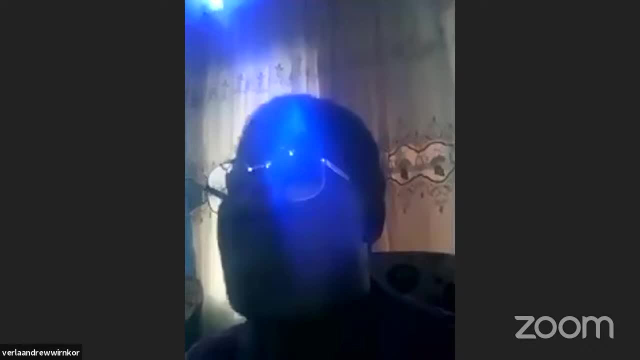 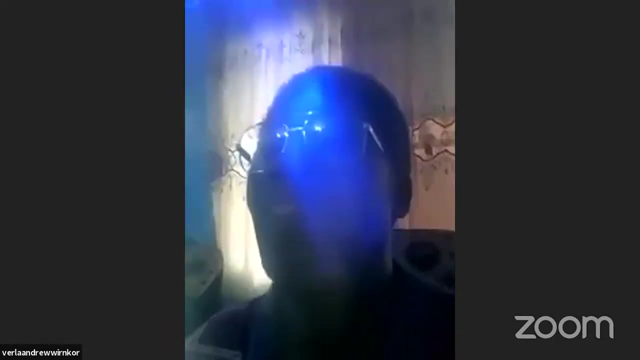 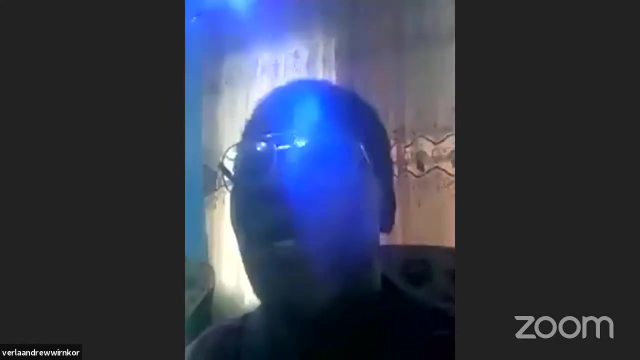 are also being lost. In fact, it is estimated that average on that of most species. A tool is a device or implement, especially one held in their hands and is being used. As a matter of fact, it is proposed here that biodiversity conservation method must be tools in the hands of human beings. 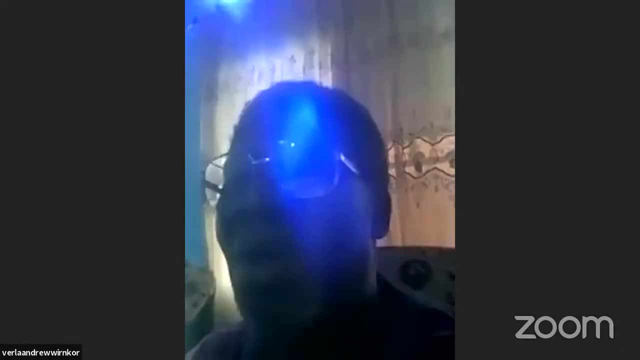 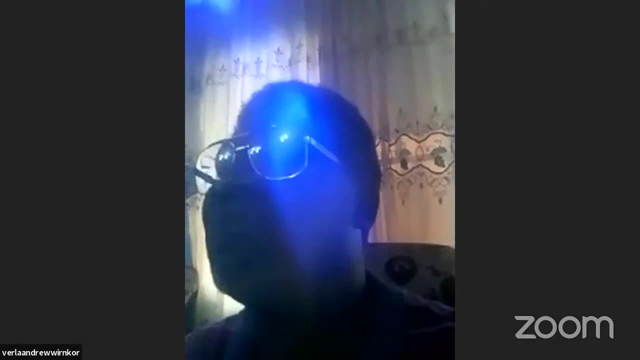 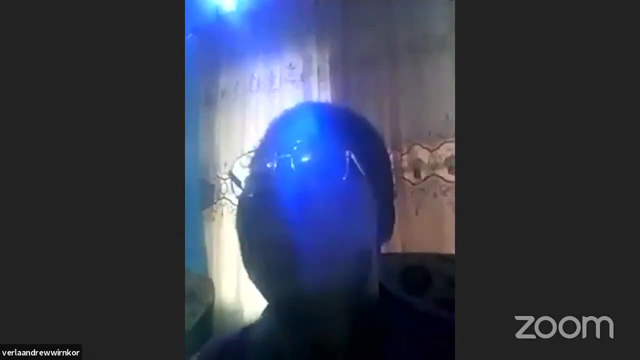 The rule of thumb for the tool is that everyone- regulations forming of zoos, international treaties and many other tools have been put by man to conserve biodiversity, But the question is: are they working? Are they producing the desired results? Therefore, biodiversity conservation. 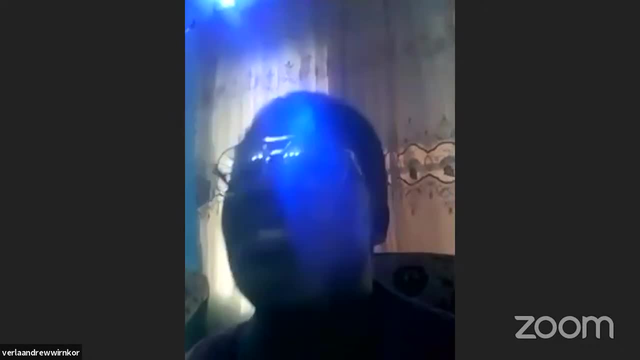 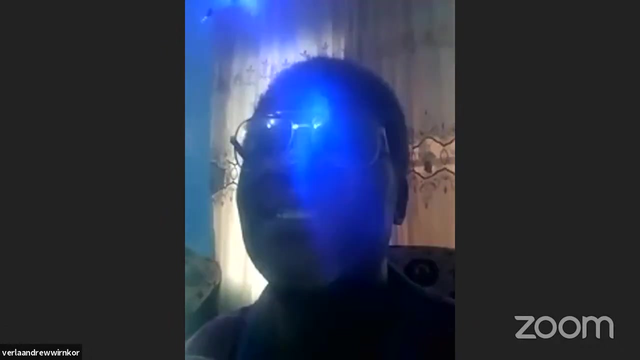 has an underlying concept: to serve species from being extinct and to stop habitats from being destroyed. We take a look at the fact that most developed countries are looking for natural resources from less developed nations. Think of the case of crude oil, The oil from Africa, wood, diamond and gold, et cetera, et cetera. 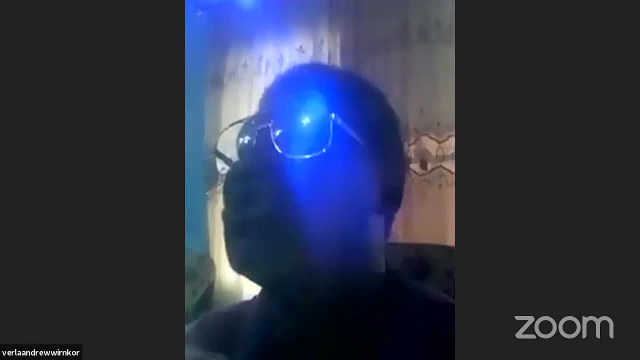 The point is that these activities ensure and cause biodiversity loss. So there is a need to protect species, one to restore biodiversity and to educate the people about the need for the conservation. The objectives of biodiversity conservation are therefore to preserve the diversity of these species, to sustain the utilization of species. 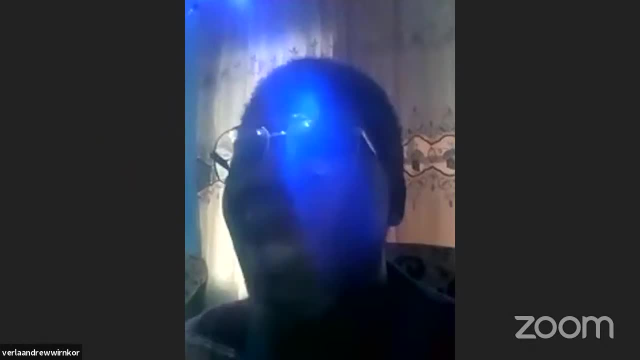 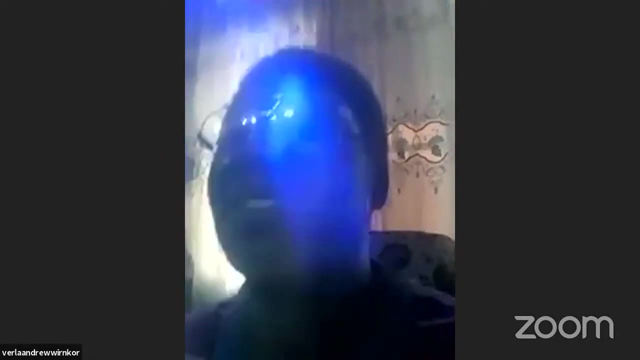 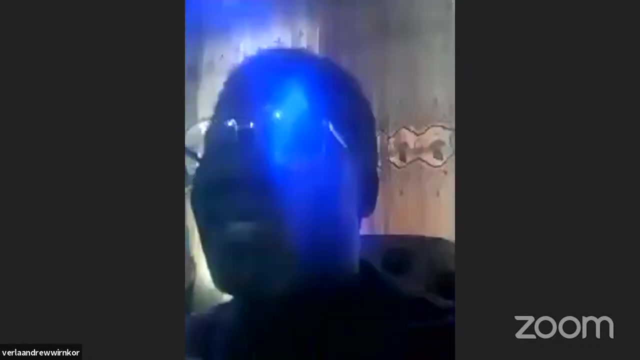 and to maintain life, to maintain life-supporting systems, the ecosystems. When these rules that I mentioned are being taken, the question we ask is: are these objectives, these three major objectives, are they being made? Your answer is yes, And if you are saying, the target species that you are going to be using is as good as mine. or an idea of what biodiversity conservation methods are, want to group them into three basic categories: What I call in-situ approach. That means biodiversity is conserved at that natural environment. This method is cost-effective. it is convenient. then there is the second approach, which is the exit to approach. here endangered species are taken. 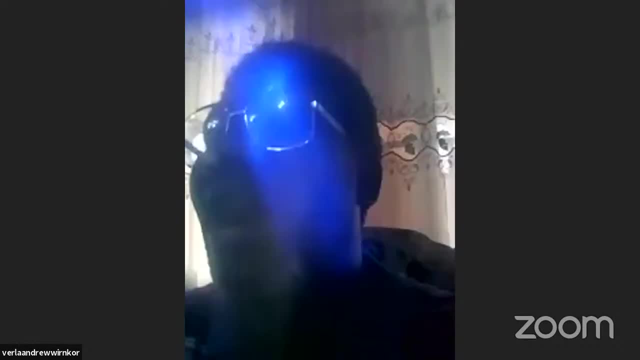 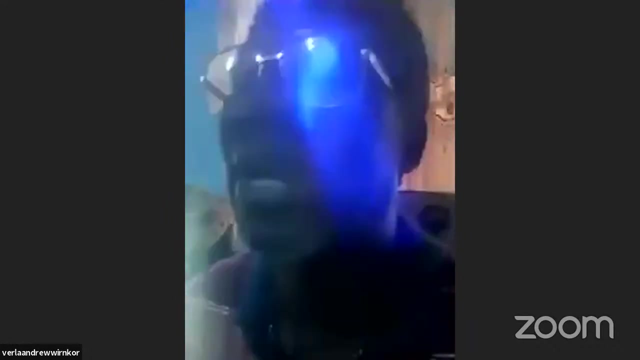 into an artificial area. they are artificially made to grow. in other words, the animal is kept in captivity or the species is kept in captivity, and the single advantage of this method is that there could be genetic techniques or genetic manipulation of these species to suit in their environment. then the third method of conservation is what i call community-based conservation. 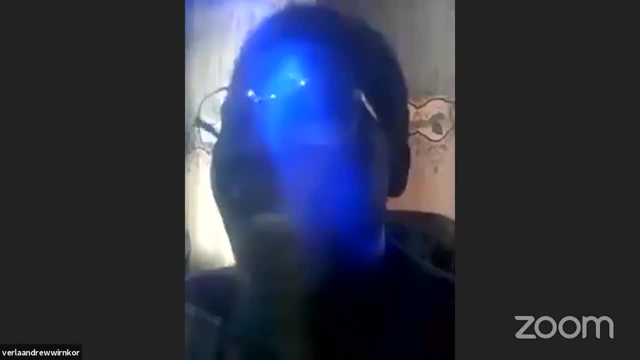 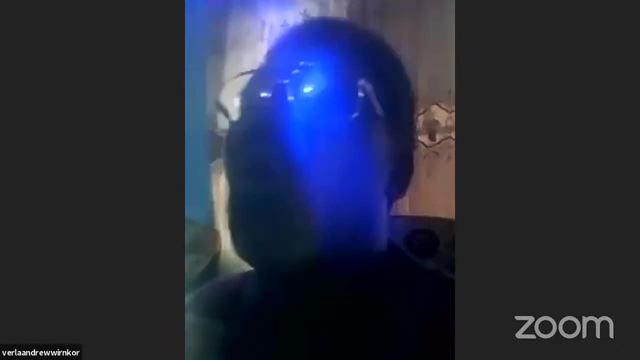 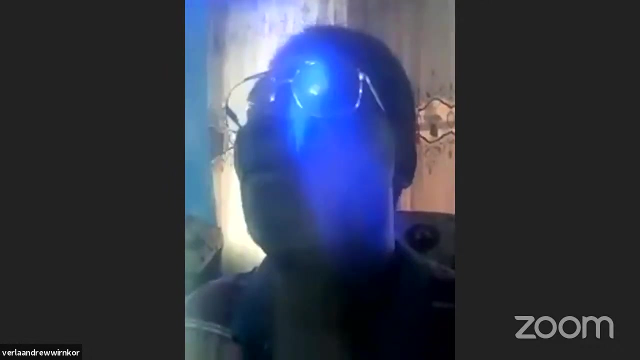 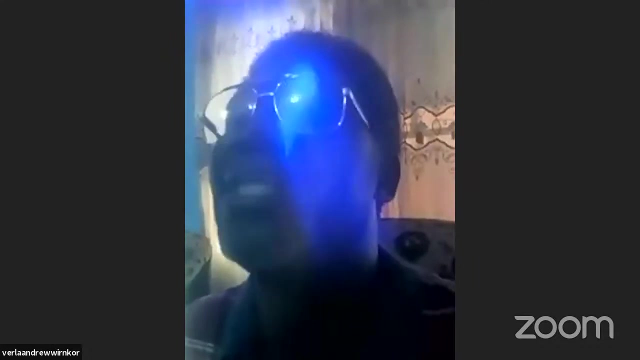 in this conservation, and by so doing, they are part of the success story of conservation. my solution to the problem of conservation is going green. going green simply means pursuing knowledge and practices that satisfy the current human needs, while ensuring that natural resources are managed in such a way that they will satisfy the needs of future generation. of course, what i'm saying here 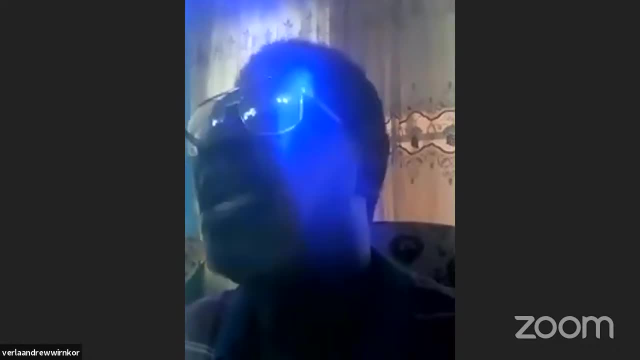 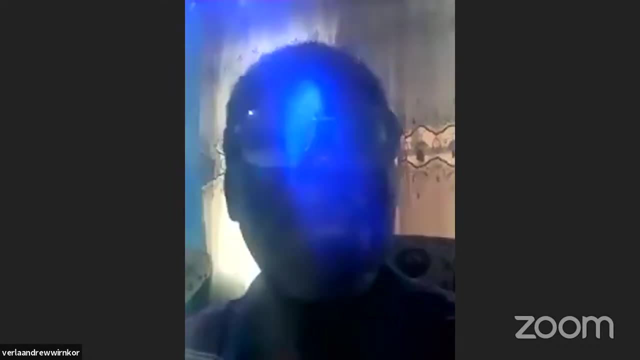 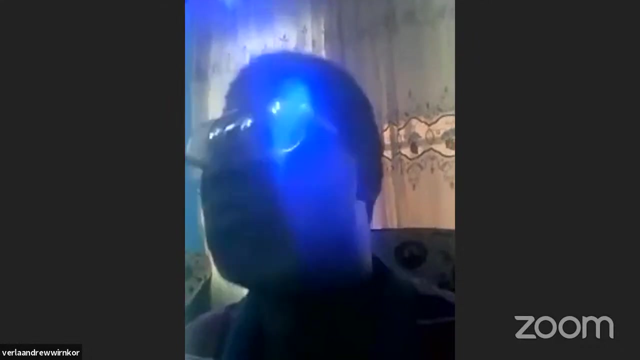 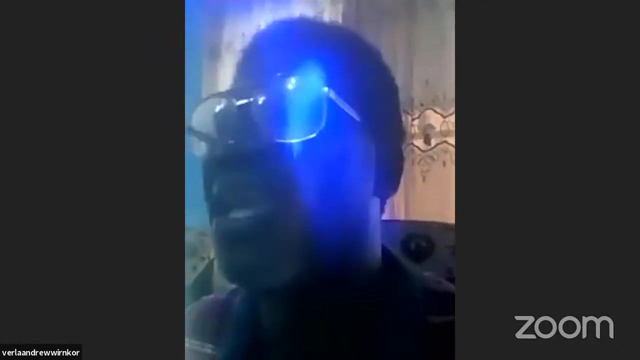 is that if humans turn to nature and begin to live sustainably, the environment can be taken care of, and then biodiversity can be conserved and even restored. in this going green method, in situ conservation method is primarily the major method of conservation, followed by the use of community based conservation methods. 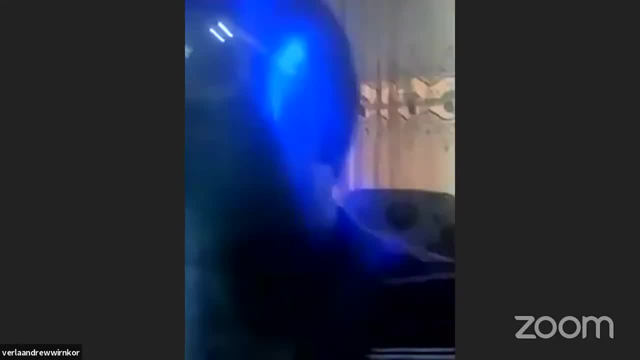 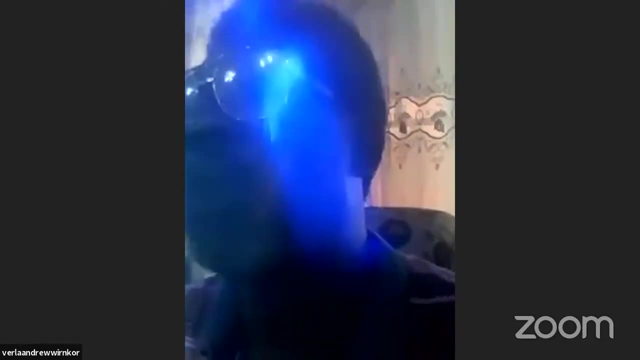 growing green will require some 12 principles which will protect our environment. and when you go green on every aspect of your life, there is a green evaluator. So where do you go if you go green Now, if you, if you want to go green, you は-. 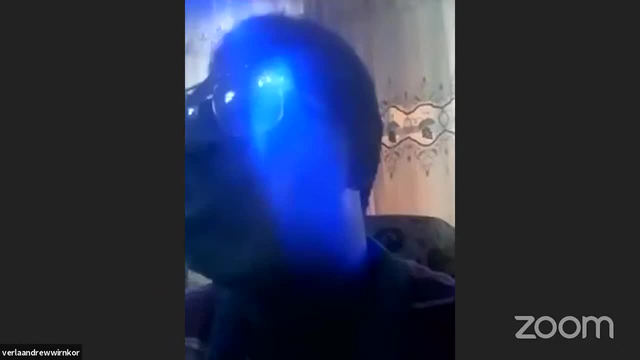 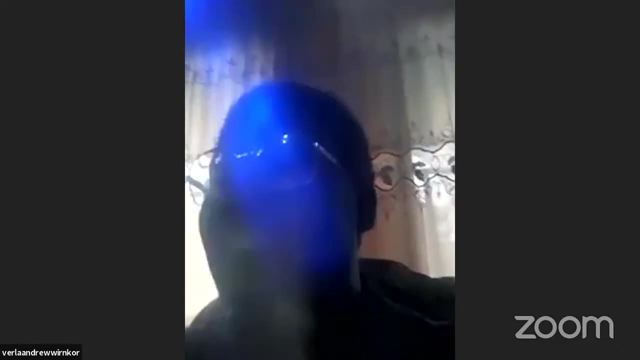 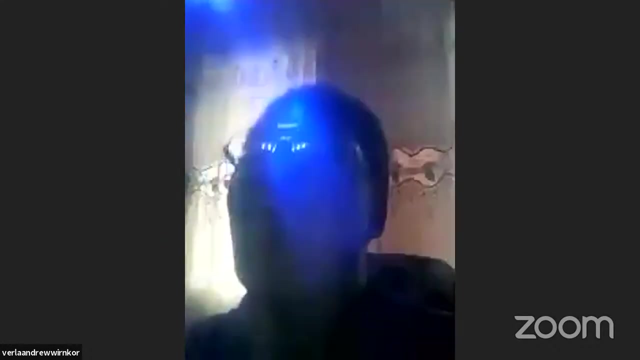 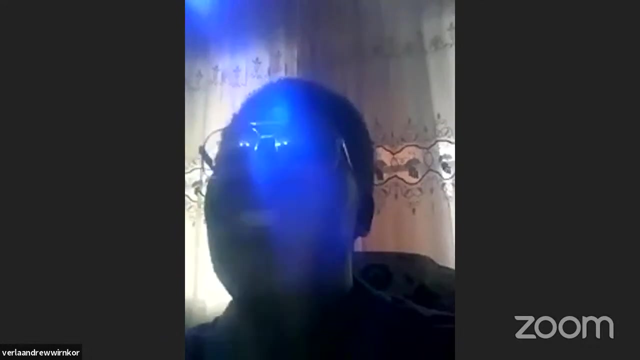 which is just another instrument which will tell you how green is your process, how green is your uh activity, how green is your behavior to the environment. and when we go green, we can obtain knowledge, what i call green knowledge. this is a sustainable living, which describes the lifestyle that reduces individuals or society use of x natural resources. 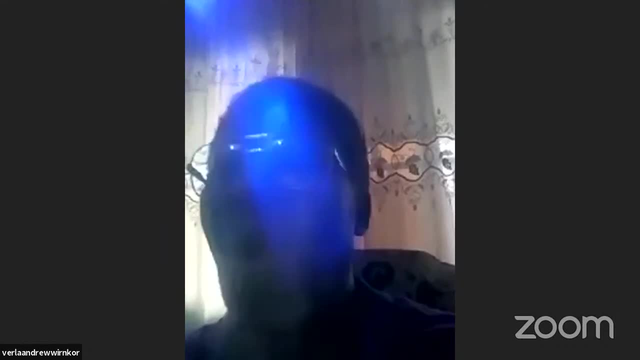 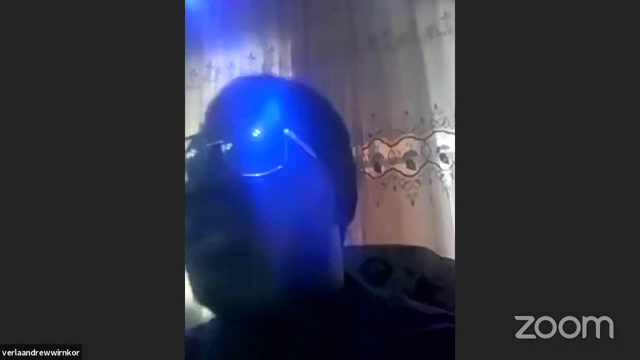 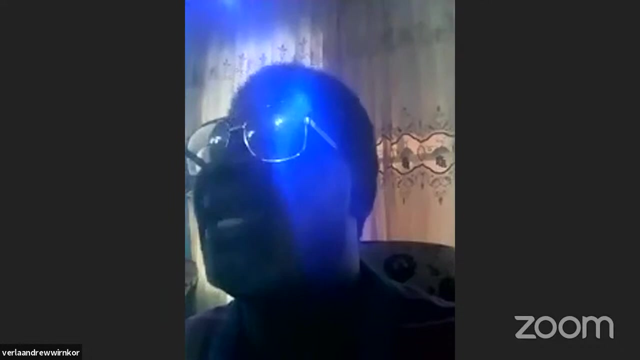 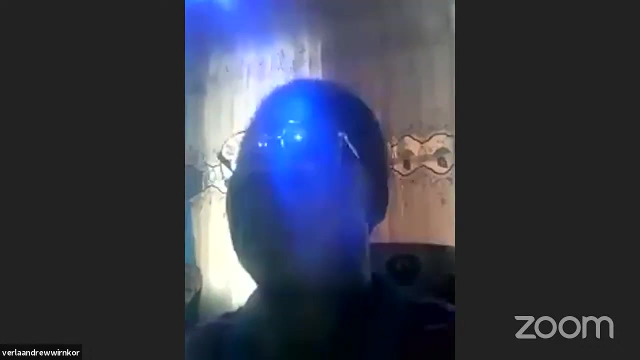 also called health harmony or living of needs, health harmony living or net zero living. when humans go green, living green is that is, a lifestyle that sustain a healthy environment both at home. we realize that biotechnology is at the base of green concept. here i want to mention some green practices and some green technology. 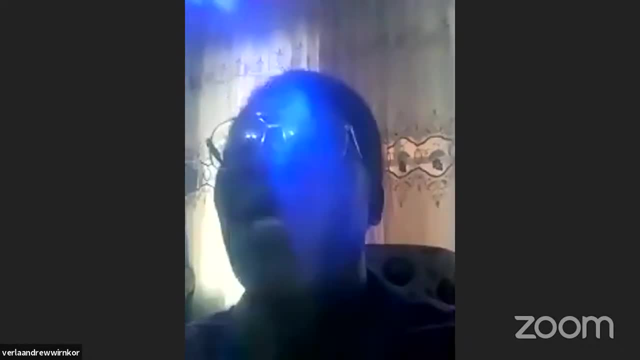 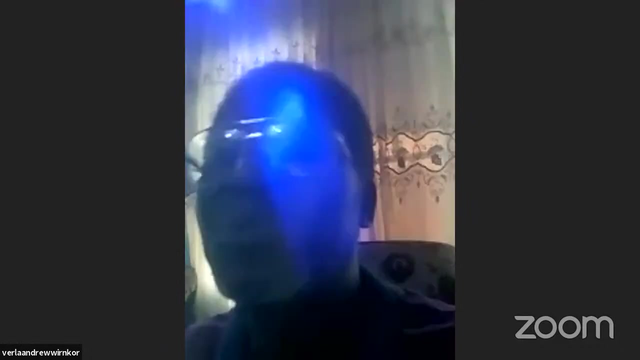 and, like i've said, biotechnology is a very fundamental aspect that should be imbibed in biodiversity conservation. if humans begin to use electric cars with low energy, bulbs, solar energy, the use of e-learning, organic farming, green building, and then they avoid waste generation, humans would have been going green, green technology. 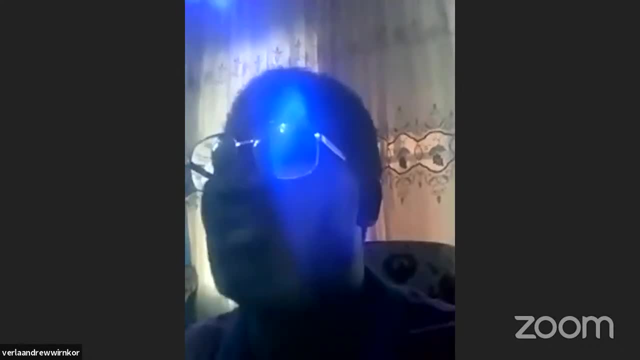 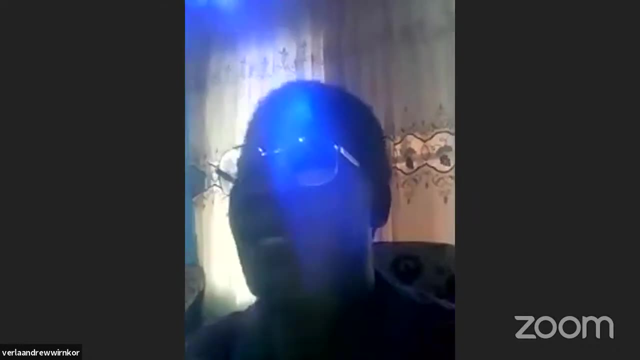 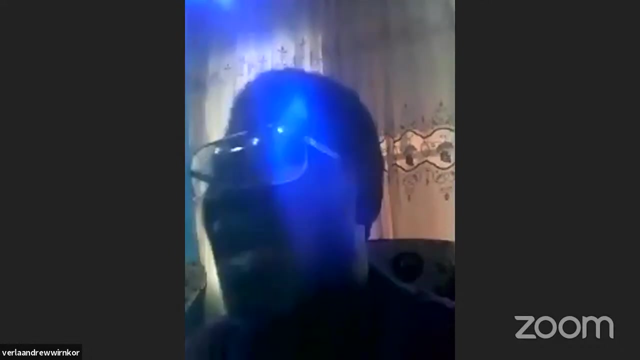 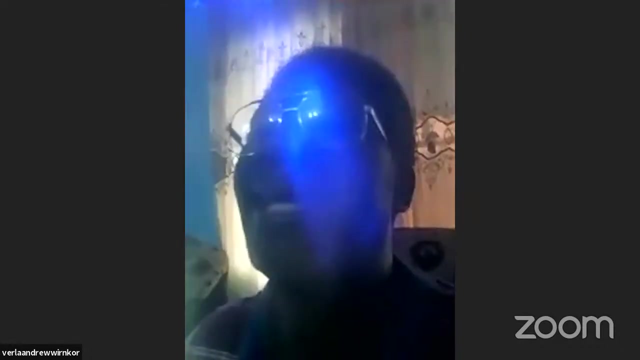 is an umbrella term describing the use of science and technology to create environmentally friendly products and to repair damage done to the environment. america is banding the use of fuel or fossil-based cars by 2030.. In a nutshell, I have said that when humans go green, 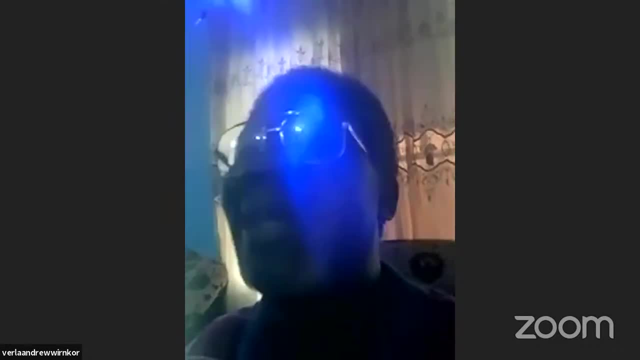 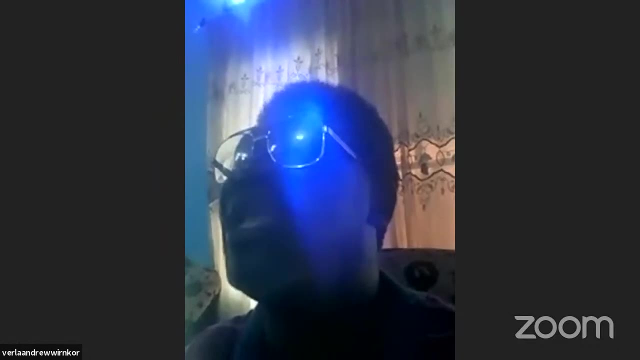 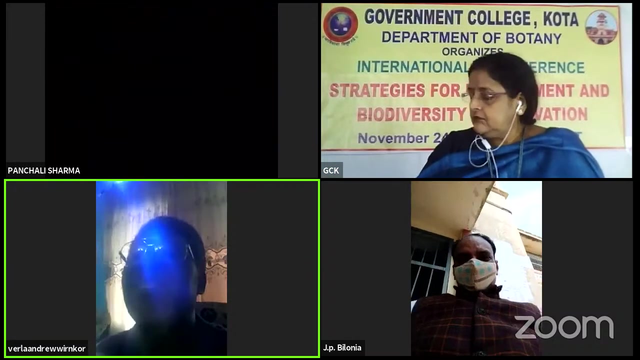 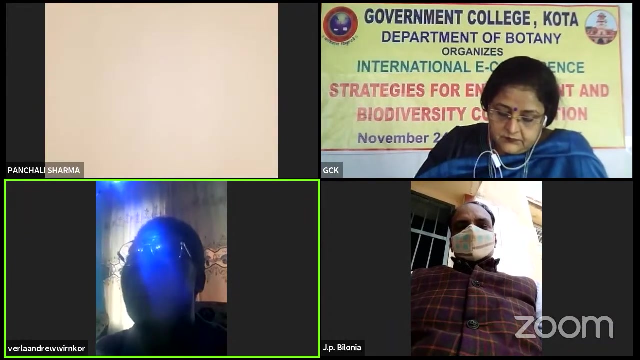 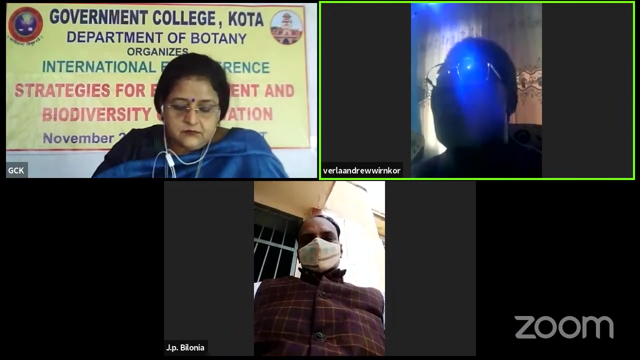 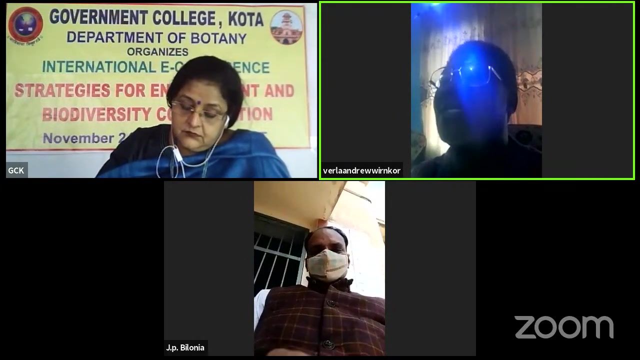 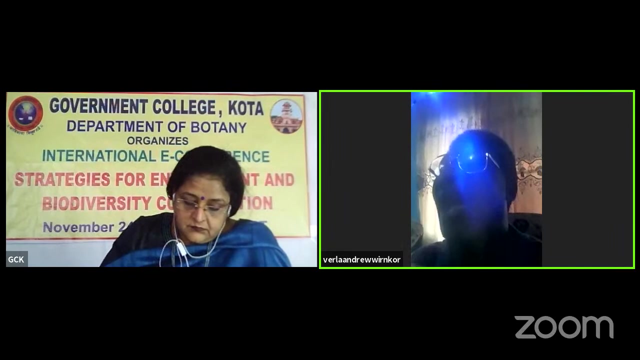 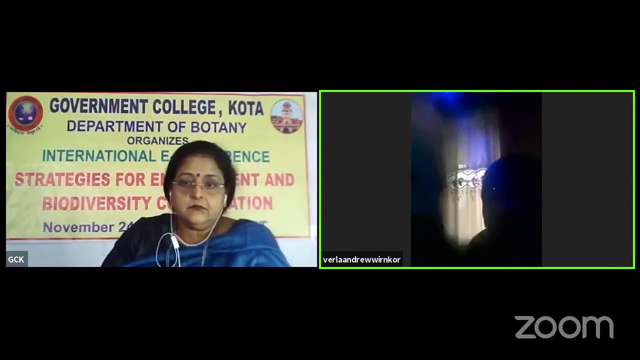 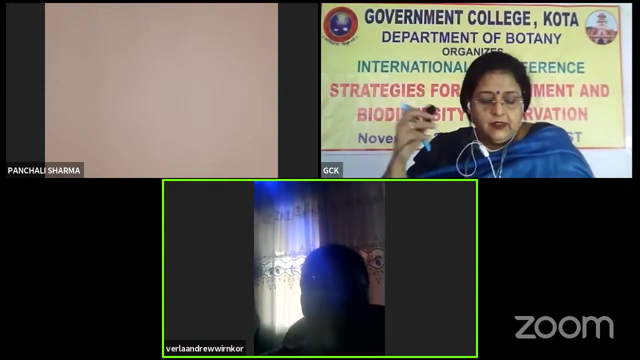 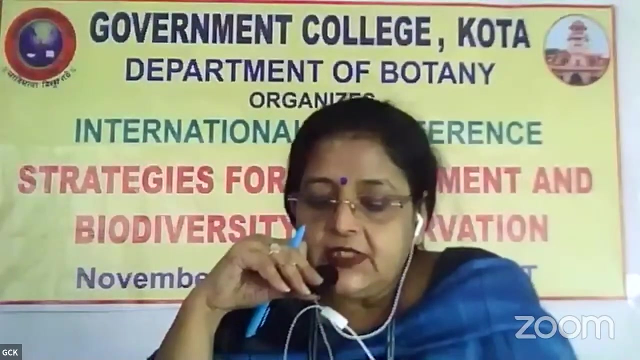 they will imbibe, living closer to nature, and then the biodiversity will be conserved. Researchers now realize that many going green efforts could see more sustainability in the future. Thank you, Thank you. Thank you, Professor Wanker. It was an absolute enriching experience. 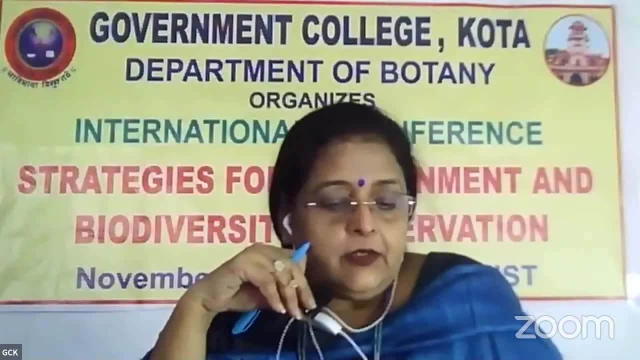 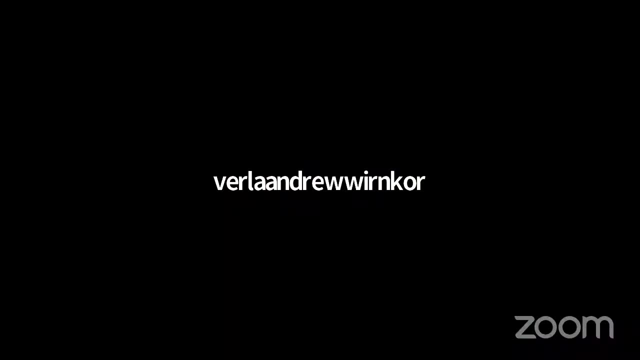 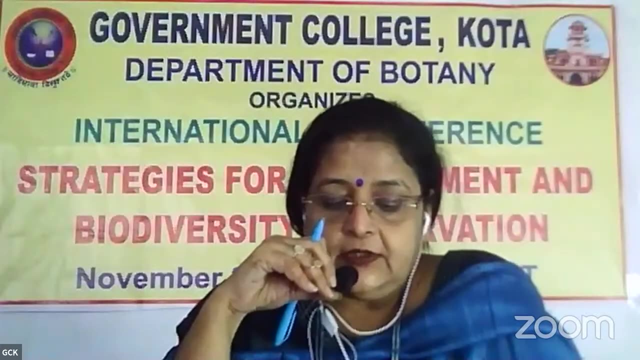 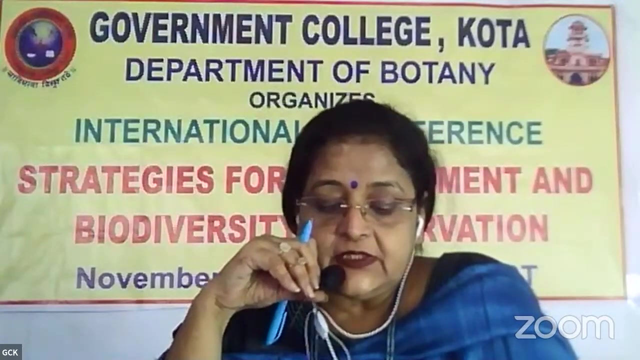 to listen to you and your views on biodiversity. Professor Wanker said biodiversity conservation is very necessary and it should be done to save species from being extinct And to educate people. the will for biodiversity conservation is also very necessary. He suggested many methods like in-situ conservation. 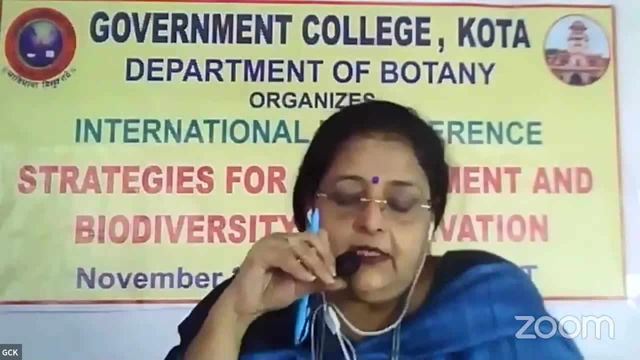 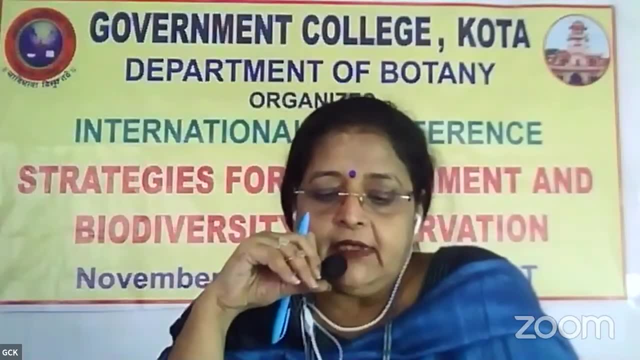 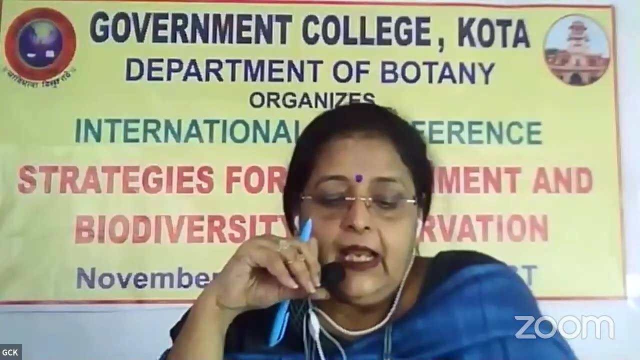 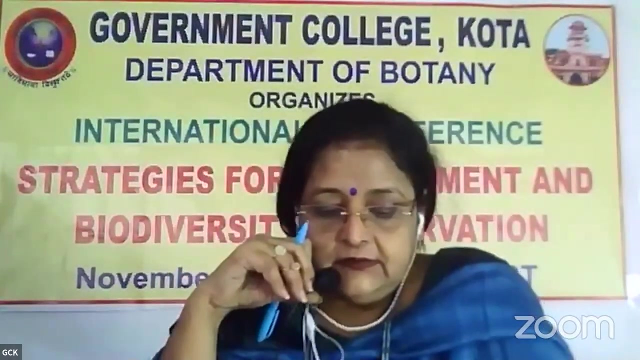 and to conserve the biodiversity. Your lecture on going green has triggered us to pursue knowledge and practices which can lead more environment-friendly and ecologically responsible decisions. Thank you, Professor, We loved it. Thank you so much, Dr Wanker. And this all such, was the grasp. 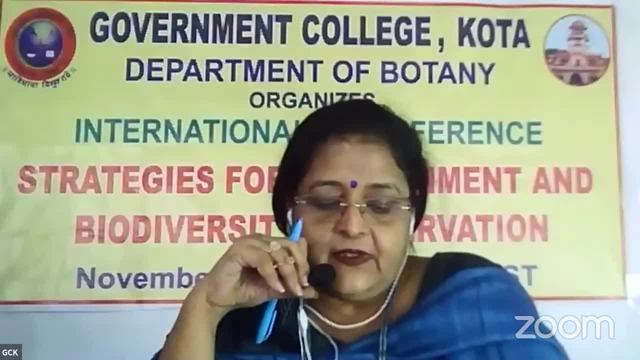 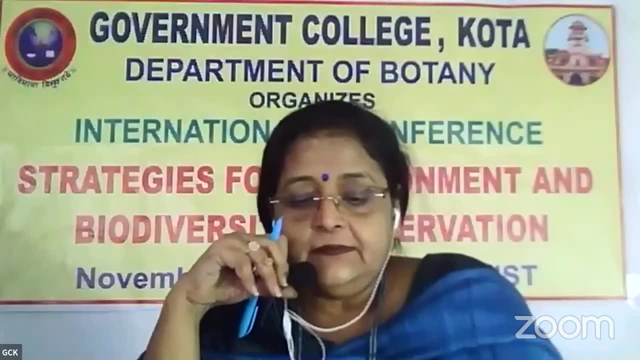 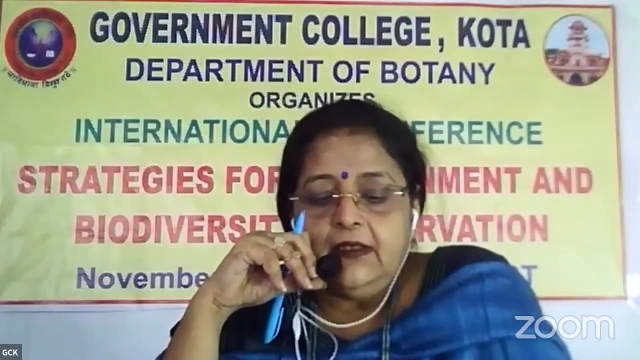 of your lecture And just sitting in thousands of miles in the oceans away from Nigeria, it took us to watch diverse forests of the gifted continent of Africa. Thank you, Sir. Now, son of many other nearby interested people, 돌아 Moment of silence. 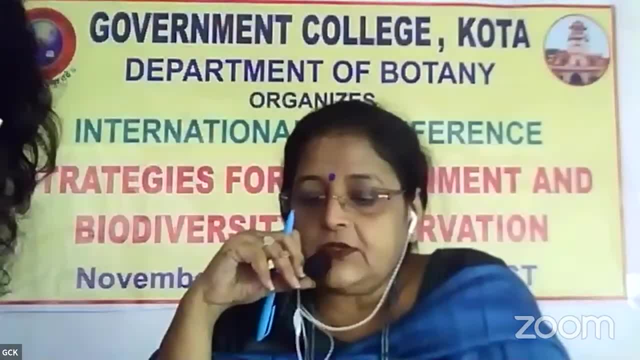 Now I invite our special invitee, Dr Ranjana Sajid. Dr Sanjay Bhagar 対 introduction with open hands. Hi, please, US, Wow, Whew, Aah. Now we will be having Dr Sanjay Bhagir, sir. What is your name, please? article Sadir Sajerabahar Angels. above I made a dispute. 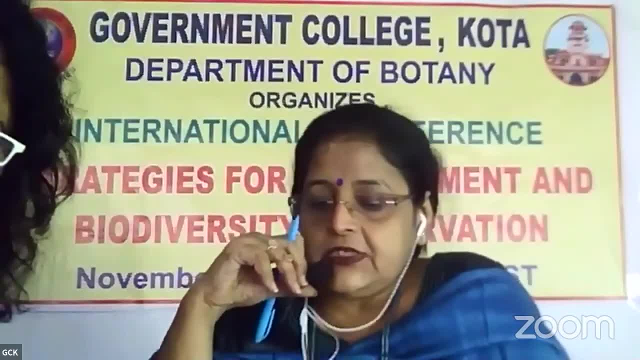 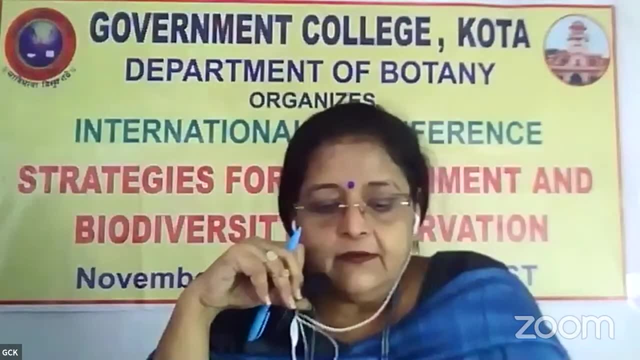 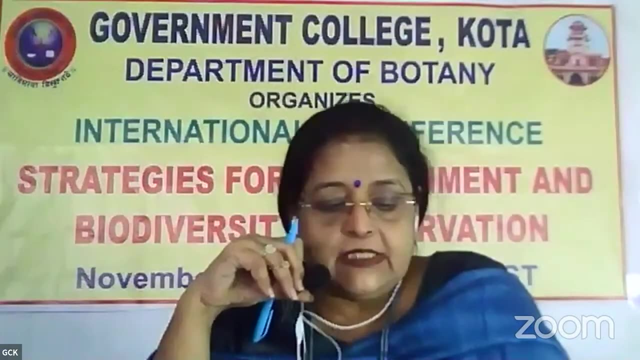 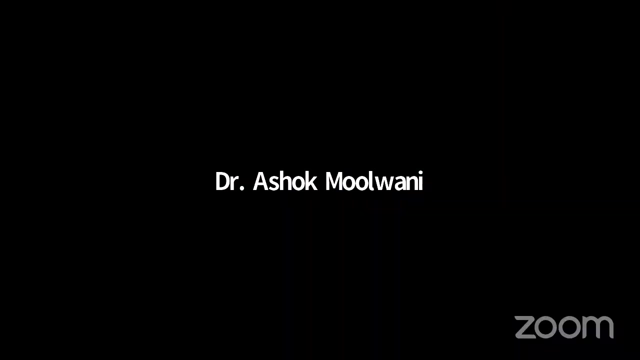 Professor, Regional Student Director, College Education, Jaipur, Rajasthan, India. To say a few words about seminar, Dr Bhargav has been supportive and encouraging in organizing any of the events of the college. A man of few, his dynamic and level-headed personality actually works as the cam in chaos. 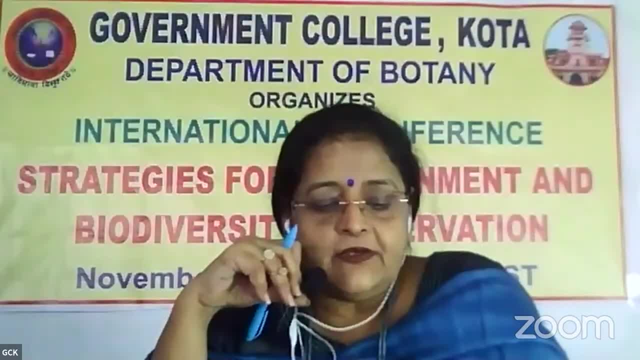 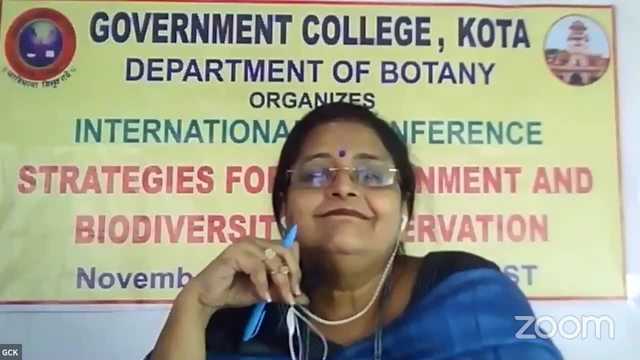 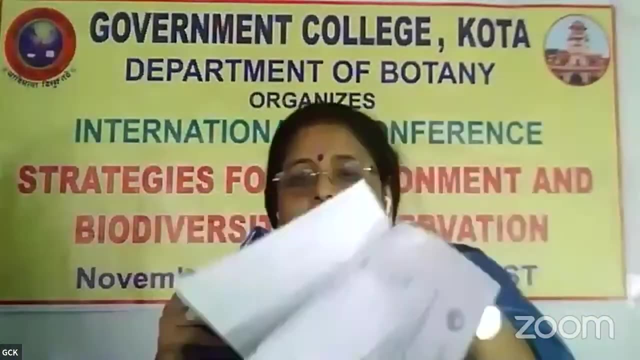 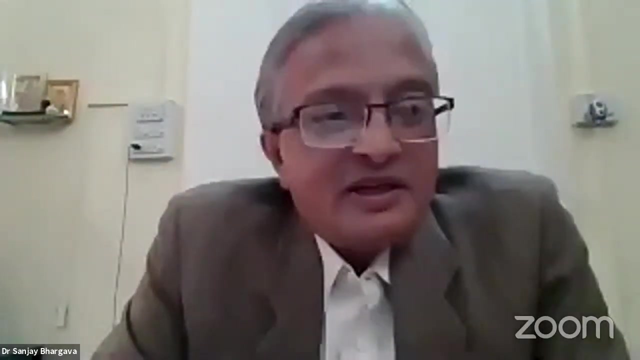 His words of wisdom are a boon to everyone which are close to him. Sir, please join us. Am I audible? Yes, sir, Very much Okay. Thank you Present in the International E-Conference being organized by the Department of Botany. 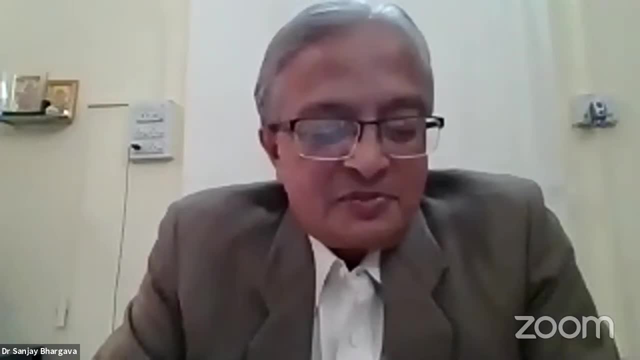 Government College Quota. Respected Principal, Dr Jayant Kumar Vijayavarghia. Eminent Speakers of the Day: Professor Deba Bahadur, Dr Varla Andrew, Dr Prashant Singh, Dr Udhesh Kumar Srivastav. 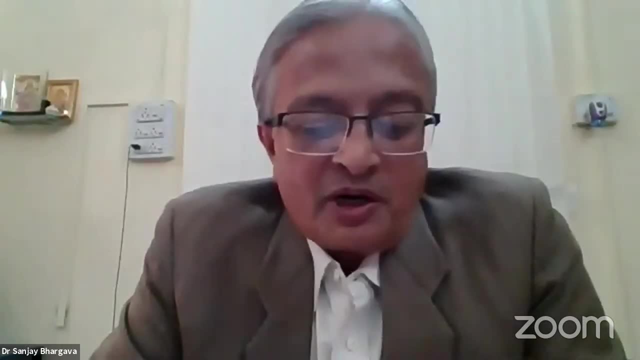 Dr Anju Kapoor. Convener and Head of the Department Botany. Dr Raghu Raj Parihar. Zonal Secretary IFOCTO. Dr Rajan Kumar. Dr Rajan Kumar. Dr Neerja Srivastav. 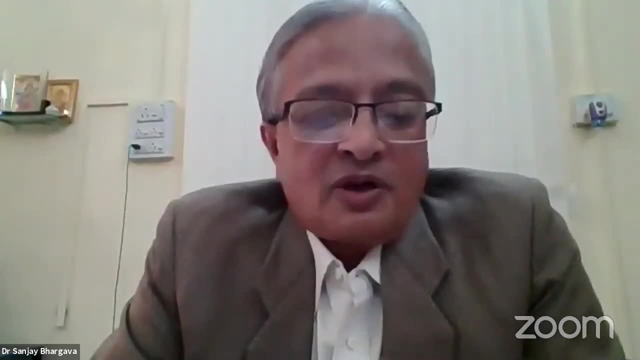 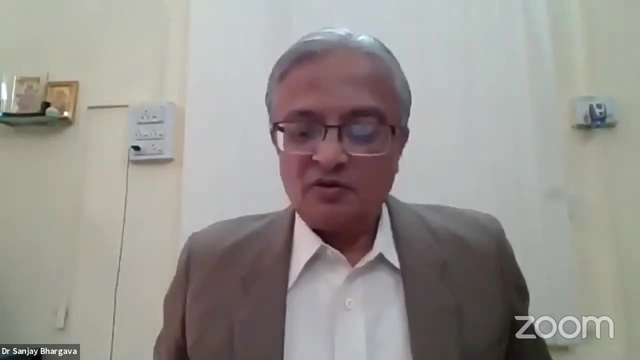 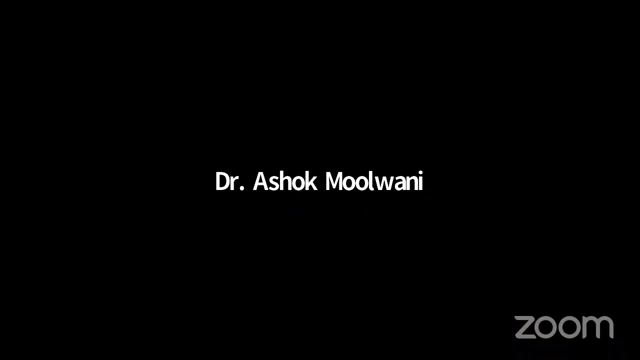 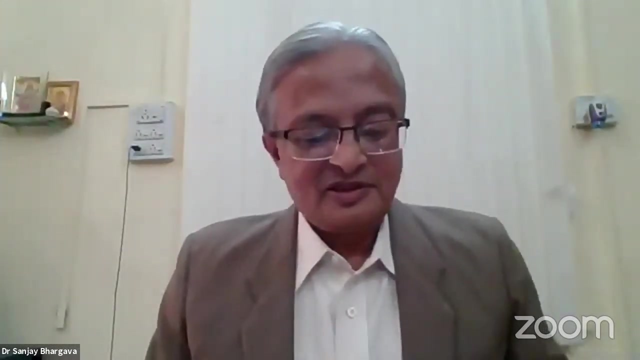 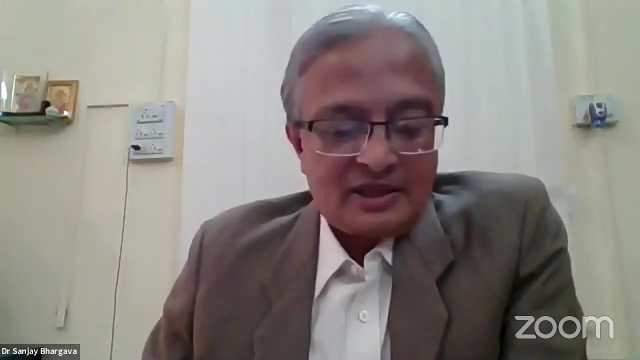 Coordinator of the event, members of the organizing team and the participants of the conference. We had two very high order of technical lectures in the field of an expert sitting abroad. Me, as a student of physics just understands the small broad view about environment and biodiversity conservation. 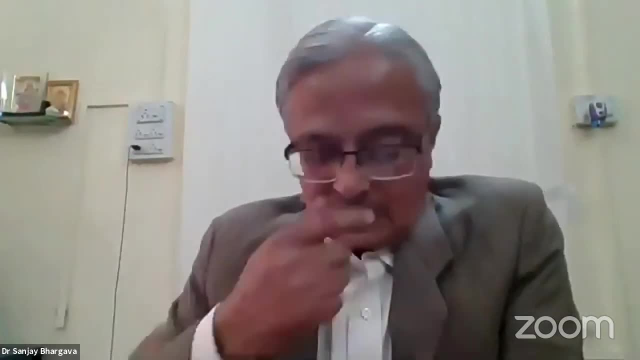 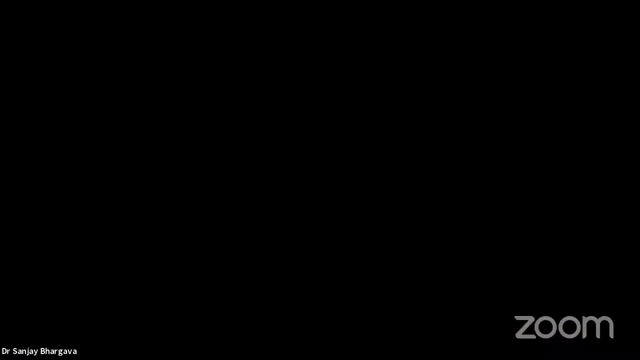 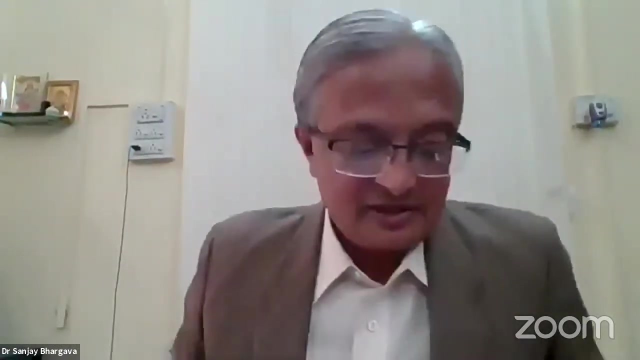 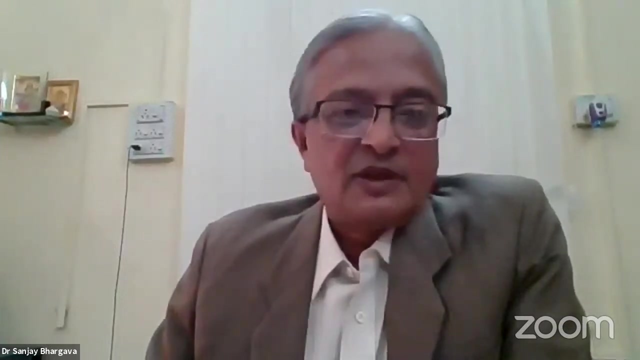 For me, environment and biodiversity conservation forms a very relevant and important topic of deliberation. We only have one planet on which we live, a planet which is full of resources, some renewable and some non-renewable, But unfortunately we have an ever-growing population which poses a huge threat to all these resources. 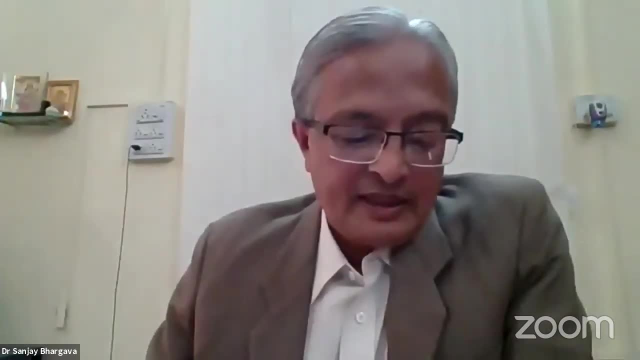 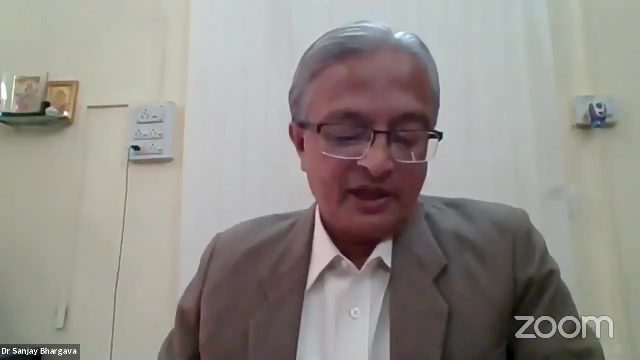 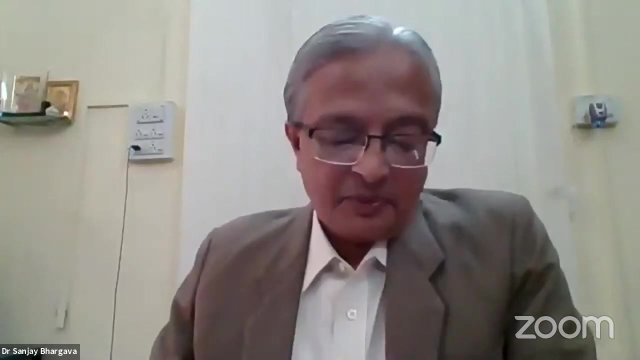 It is therefore unclear what future generations will find and what life will be there for them. if we exploit all the current resources To address this issue and to ensure that we leave some resources for the future, environmental conservation comes into play. Environmental conservation is a practice of humans. 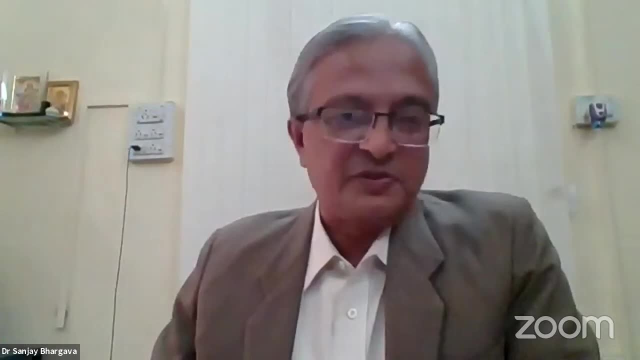 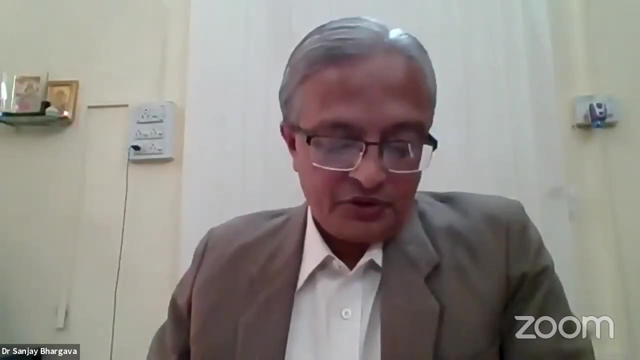 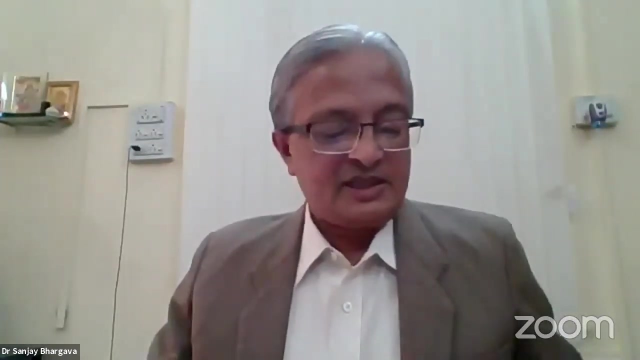 saving the environment from the loss of species and the destruction of ecosystem, primarily due to pollution and human activities. Conservation is important in saving the environment. Conservation is important in saving the environment. Conservation is important in saving the environment and helping both animals and trees. as we are all dependent on one another for survival. Environmental conservation is an umbrella term that defines anything we do to protect our planet and conserve its natural resources so that every living thing can have an improved quality of life. And if natural 다양 sık is taken into consideration, 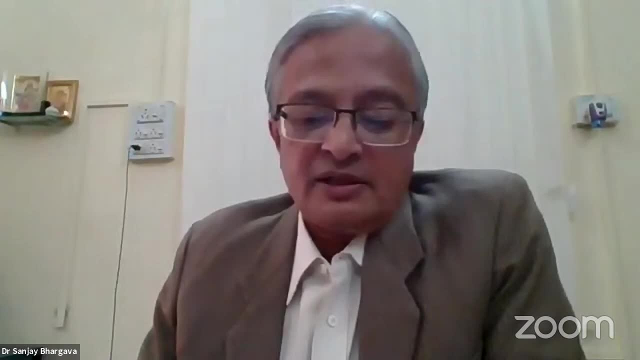 then conservation must be provided. Environmental conservation is the protection, preservation, management or restoration of natural environment and the ecological communities that inhabit them. Conservation is generally held to include the management of human use of natural resources for current public benefit and sustainable social and спасion warmth for ancient tribes and archaeologists. 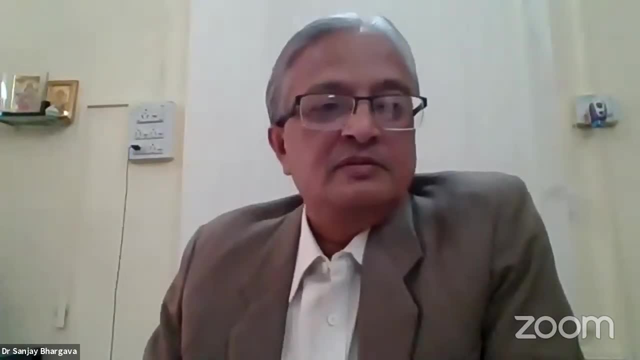 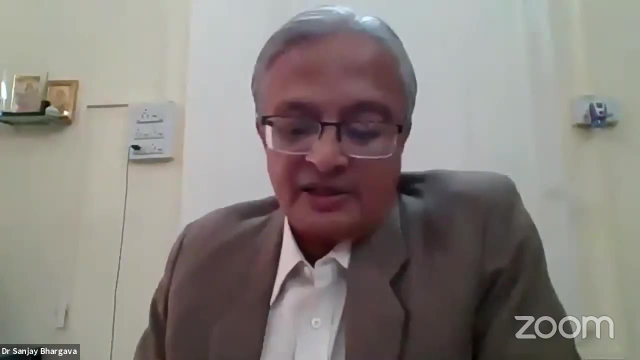 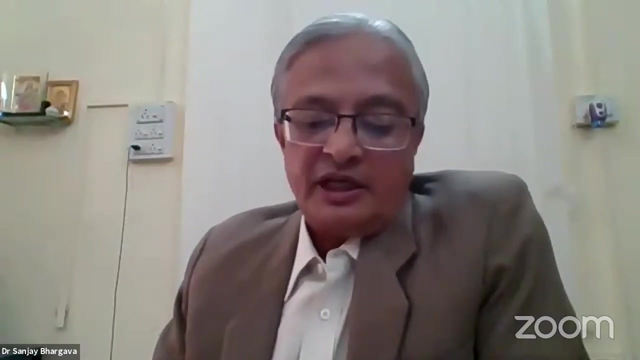 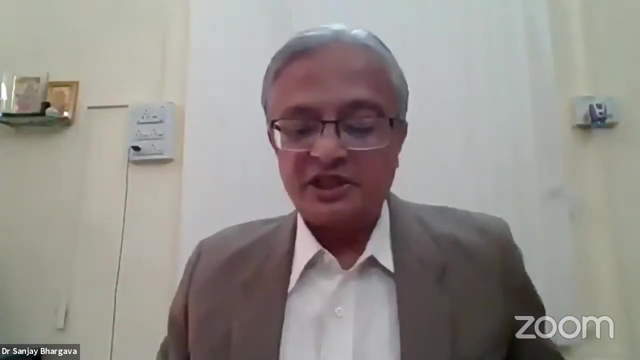 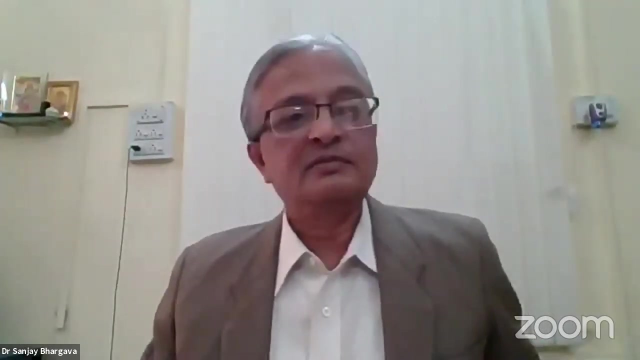 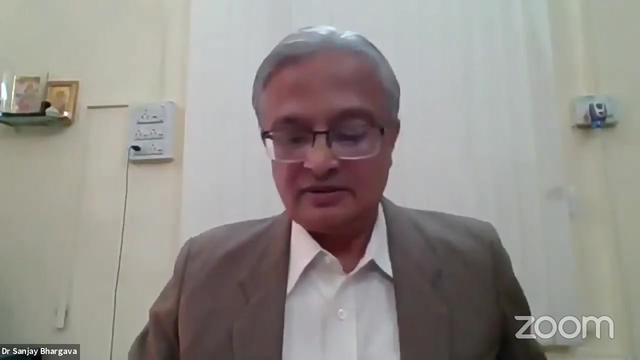 economic utilization. The second term for me, biodiversity, refers to the variety of plants and animals found on earth. It measures the variations at ecosystem, species and genetic level. Biodiversity conservation means protection, conservation and management of biodiversity in order to obtain sustainable benefits for future generations. Biodiversity conservation. is important because it provides certain services and resources which are essential for the life on earth. Biodiversity conservation can have three main objectives: To preserve the diversity of species, sustainable utilization of species and ecosystem. to maintain life supporting systems and essential ecological processes. It can be conserved by preventing 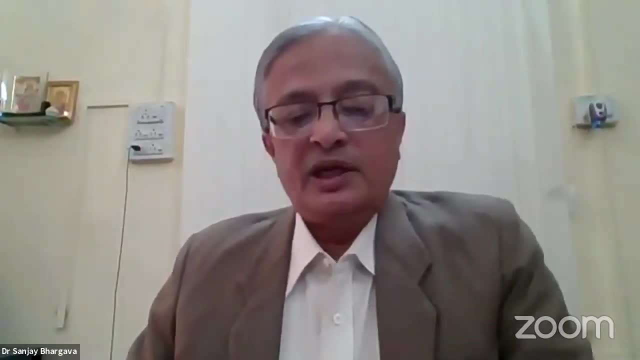 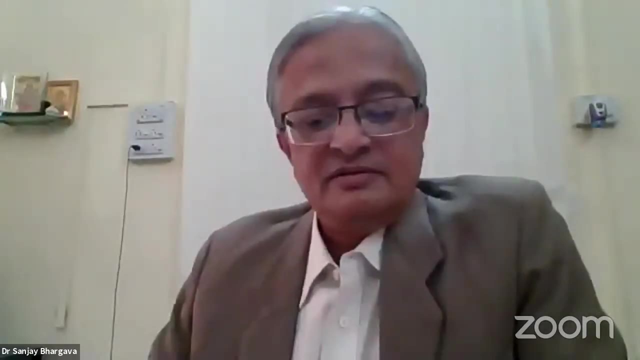 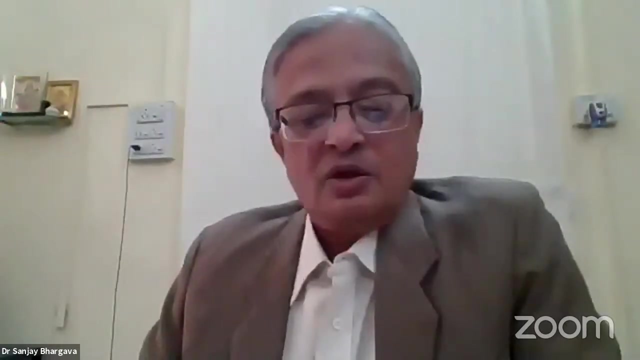 the cutting of trees, putting a ban on hunting of animals. efficient utilization of natural resources. Protected areas should be developed for animals where no human activities are permissible. Biodiversity refers to the variability of life on earth. It is normally conserved by the two different methods of conservation. Biodiversity conservation can be conserved. by the two different methods of conservation. The two methods are in-situ conservation and another ex-situ conservation. In-situ conservation of biodiversity is the conservation of species within their natural habitat. In this method, the natural ecosystem is maintained and protected. The important advantages of in-situ conservation include, for example, the ability to preserve can be. it is a cost-effective and a convenient method of conserving biodiversity. A large number of living organisms can be conserved simultaneously. Since the organisms are in the natural ecosystem, they can evolve better and can easily adjust to different environmental conditions. Certain protected areas where in-situ conservation takes place include the national parks, the wildlife sanctuaries and the biosphere reserves. In the second method, that is, in ex-situ conservation of biodiversity, it involves the breeding and maintenance of endangered species in artificial ecosystems. such as zoos, Nurseries, botanical gardens, gene banks, etc. There is less competition for food, water and space among the organisms. The advantages can be counted, as The animals are provided with a longer time and breeding activity. The species breed in captivity, which can be reintroduced in the wildlife. 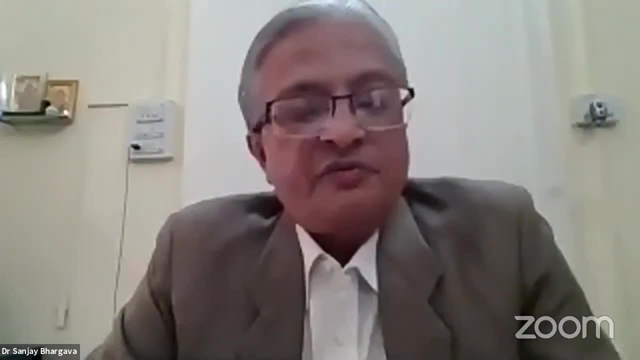 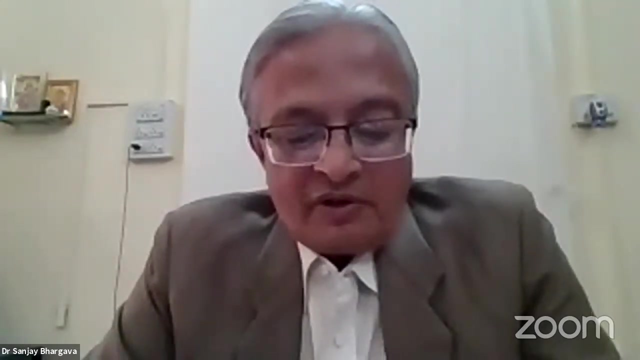 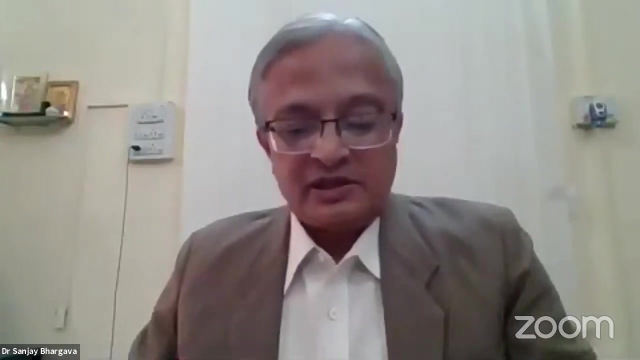 Genetic techniques. Genetic techniques can be used to improve the quality of the wildlife. They can also be used for the preservation of endangered species. What are the different strategies for biodiversity conservation? Among them, the important ones are: All the varieties of foods. timber plants, livestock, microbes and agricultural animals should be conserved. 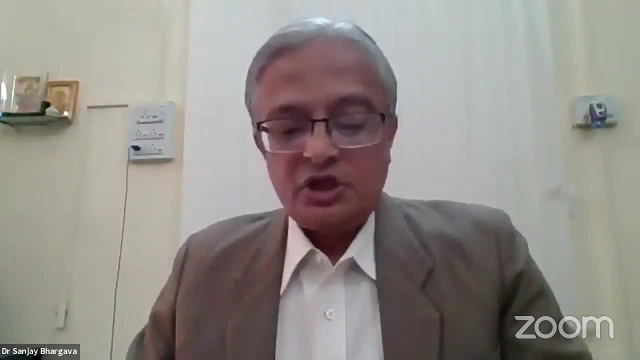 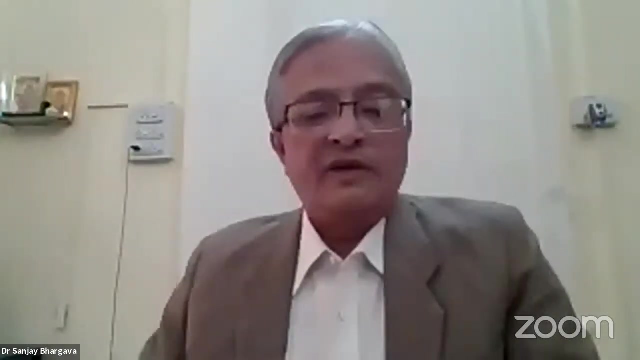 All the economically important organisms should be identified and conserved. Unique ecosystems should be preserved first. The resources available have to be utilized very efficiently. Poaching and hunting of wild animals has to be prevented. The reserves and protected areas should be developed very carefully. The level of pollutants 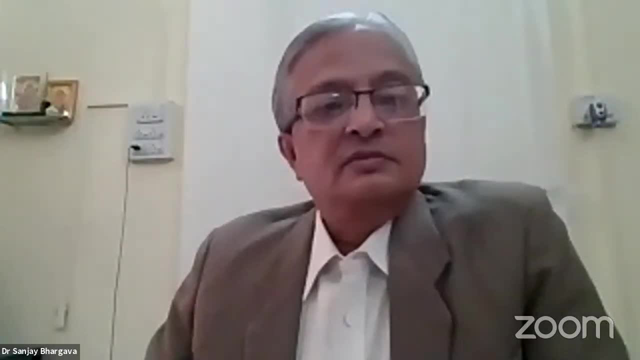 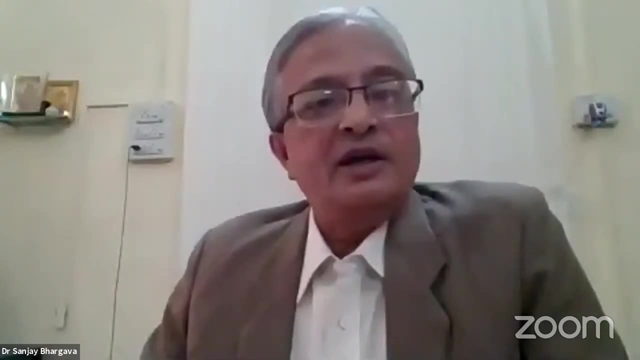 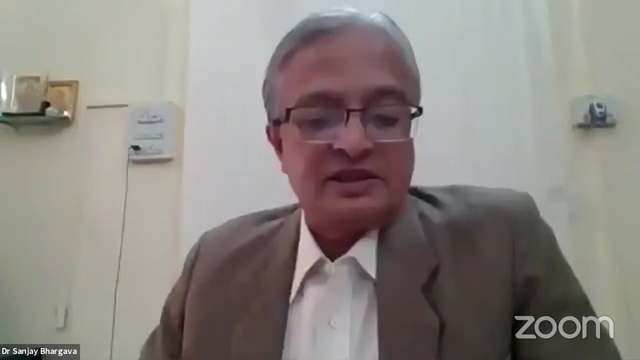 has to be reduced in the environment. Deforestation has to be strictly prohibited. Environmental laws should be strictly followed. The useful and the endangered species of plants and animals should be conserved in the nature, as well as artificial habitats. Public awareness has to be increased and created. by the use of the resources available. The use of the resources available has to be reduced and the use of the resources available has to be reduced. and the use of the resources available. regarding biodiversity conservation and its importance, Why really do we have to conserve biodiversity? Despite our many advances, our environment is. 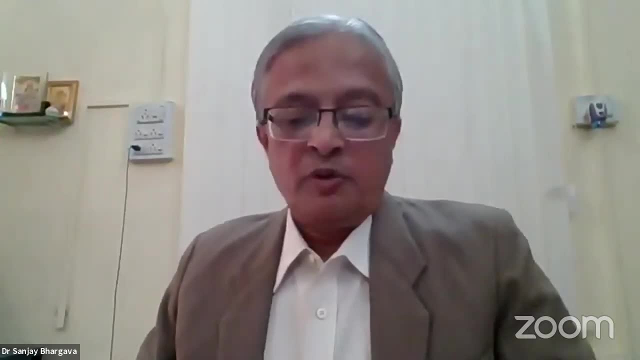 still threatened by a range of problems, including global climate change, energy dependence on unsustainable fossil fuels and loss of biodiversity. Humans have changed ecosystems more rapidly and extensively than in any comparable period of time in the human history, largely to meet rapidly growing demands for food, fresh water, timber, fiber and fuel. 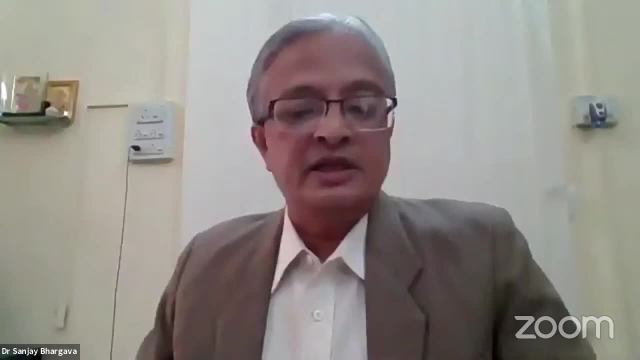 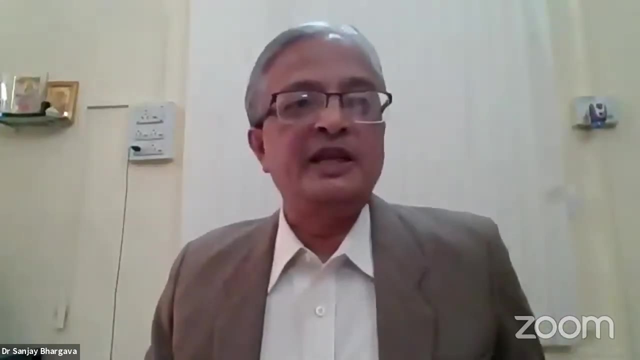 This has resulted in substantial and largely irreversible loss in the diversity of life on earth. It is believed that an area with higher species abundance has a more stable environment compared to an area with lower species abundance. We can further claim the necessity of biodiversity by considering a degree of dependence on the environment. We depend directly on various species of plants for our various needs. Similarly, we depend on various species of animals and microbes for different reasons. Biodiversity is being lost due to loss of habitat, over-exploitation of resources, climatic. 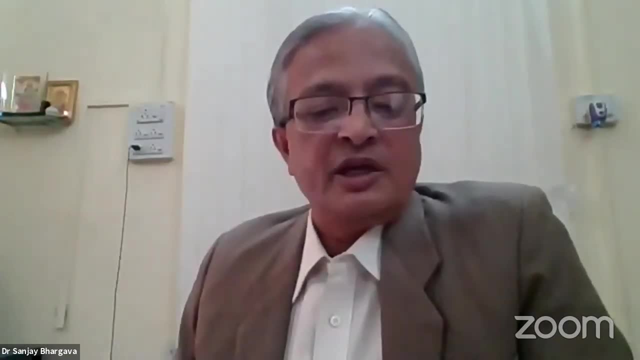 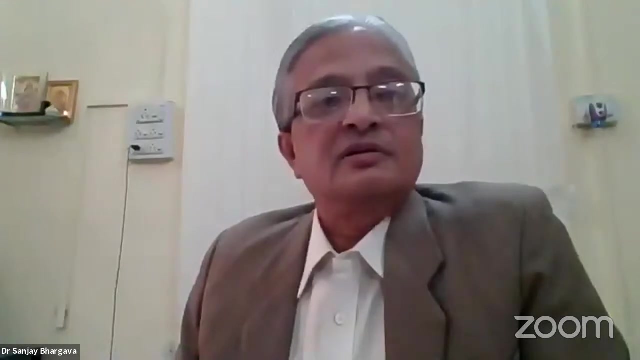 changes, pollution, invasive exotic species, diseases, hunting, etc. Since it provides us with several economic and ethical benefits And adds aesthetic value, it is very important to conserve biodiversity. The diversity of the phenomenon of nature is so great, and the treasures hidden in the 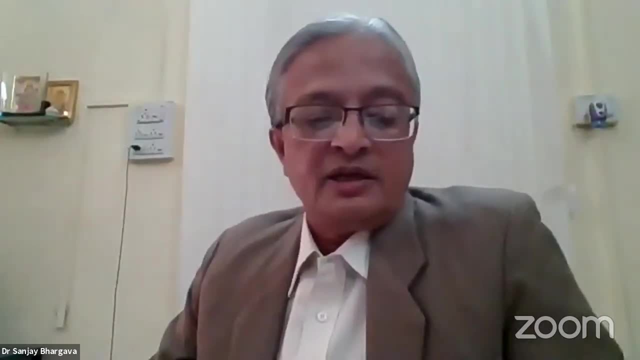 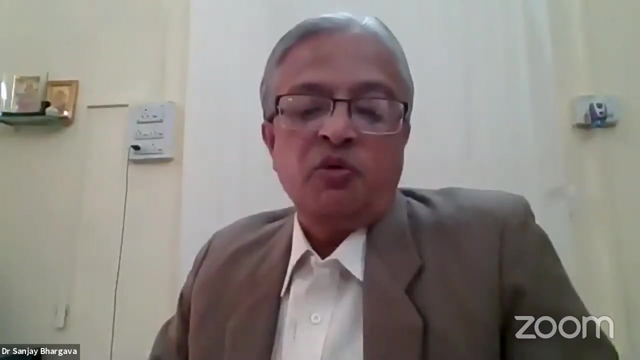 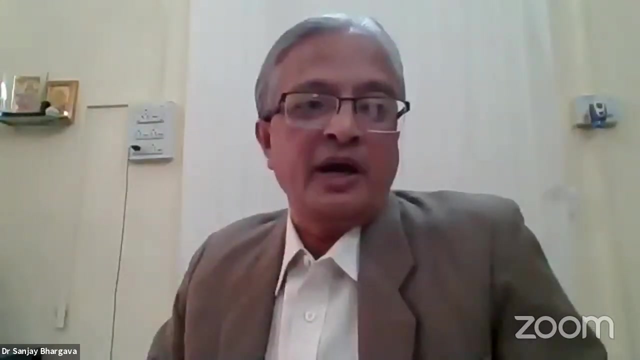 heavens are so rich. precisely in order that human minds shall never be lacking in fresh nourishment, We should preserve every scrape of biodiversity as priceless, while we learn to use it and come to understand what it means to humanity. To underline the importance of conservation of environment and biodiversity, it is very 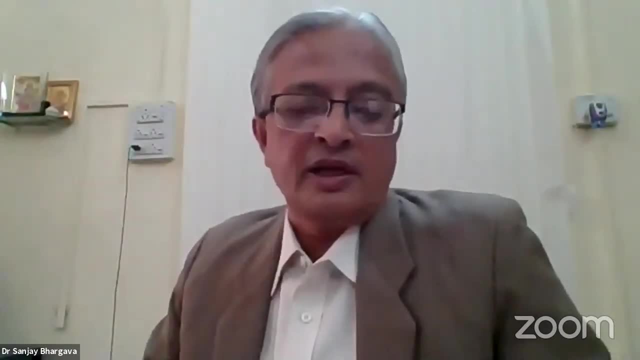 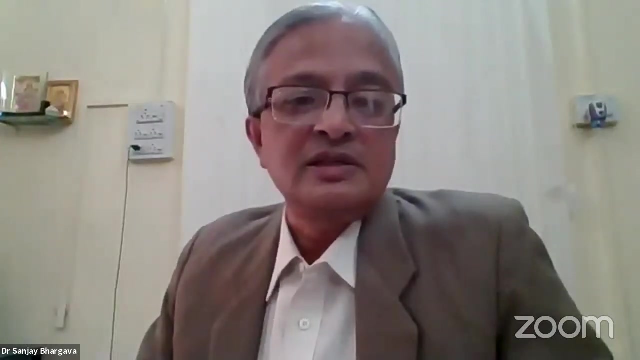 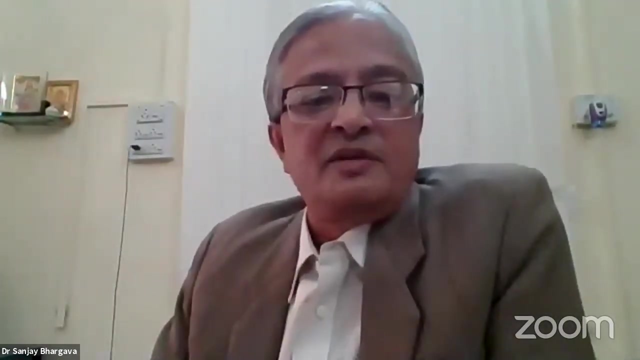 rightly said, if you pollute the air, water and soil that keeps us alive and well and destroy the biodiversity that allows natural systems to function, no amount of money will ever be able to save us. With these words, I wind up As a layman- words from my side- and thank the organizers for providing me an opportunity. 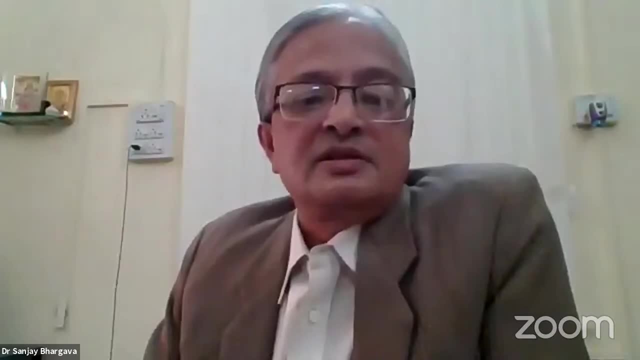 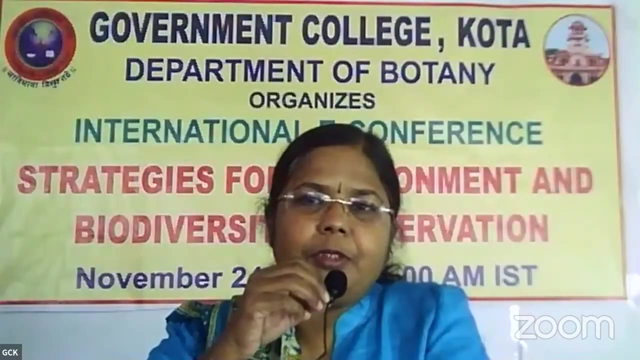 to be a part of this e-conference. Thank you very much. Thank you, sir. On the behalf of Botany Department, I would like to thank Dr Sanjay Bhargava, sir, for giving us a brief introduction about the biodiversity. 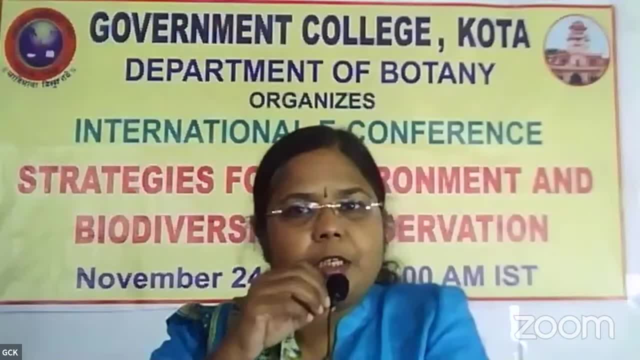 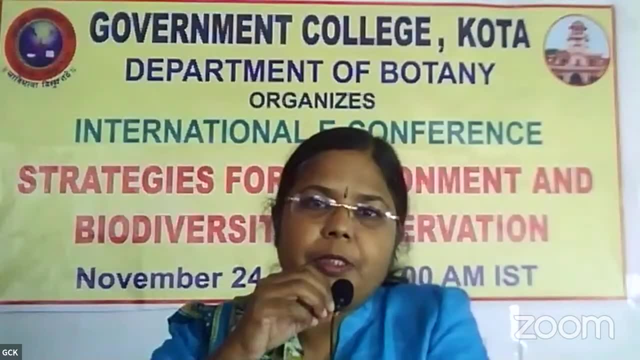 This may inspire all of our students. Thank you, Thank you so much. With this we come at the end of the first session. In the first session we have the two eminent speakers, Dr Varla and Dr Deva, sir who, 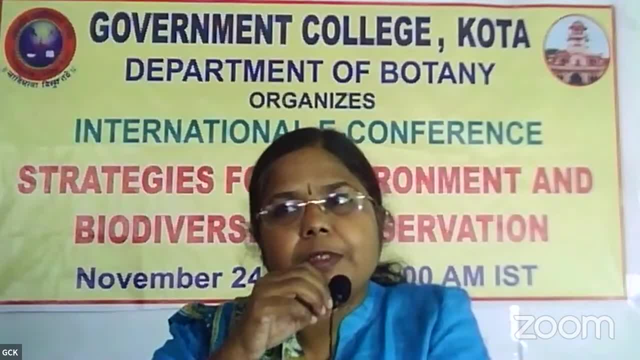 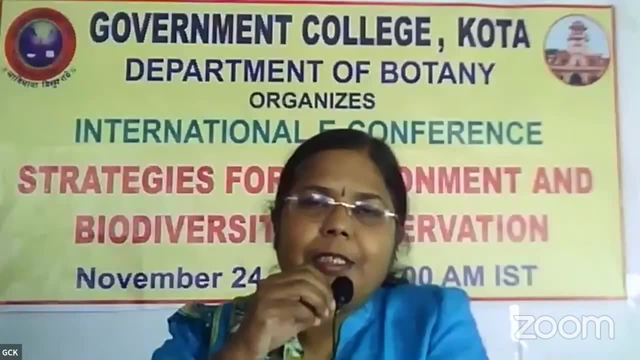 gave us a very informative who delivered a very informative talk on the topic biodiversity as well as environmental conservation. Thank you. I personally thank Dr Deva and Dr Varla to connect with us and give the very useful and attractive information. Thank you. 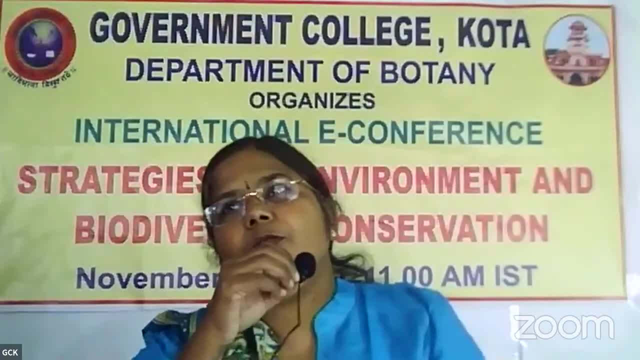 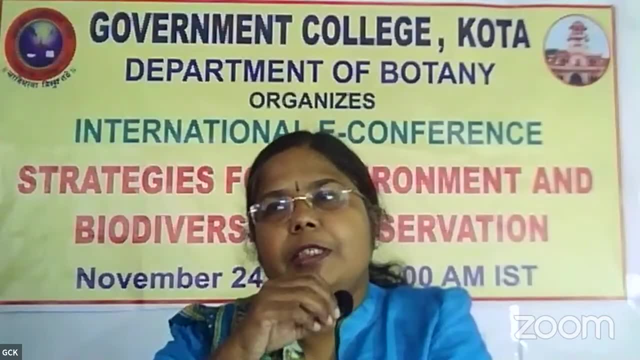 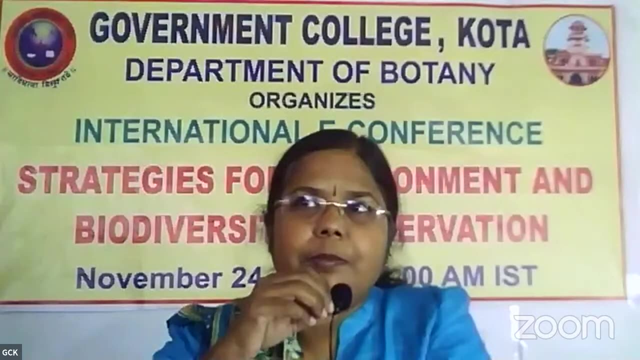 Thank you so much. At this point, I would also like to thank Professor Deepak Sharma sir, President of Indian Science Congress Association, who is always with us, And by this association we are able to come to this webinar. Thank you, Dr Deepak Sharma, sir, for your constant cooperation and support. 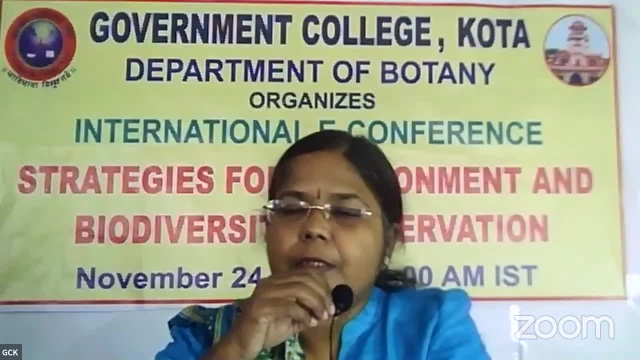 Thank you, sir, For the second session. I would like to invite Dr Sulekha Joshi to conduct second session. Dr Sulekha Joshi, please, Thank you. Thank you, vam shi nishih. 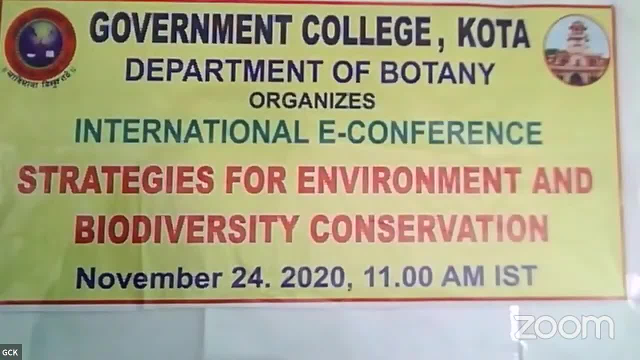 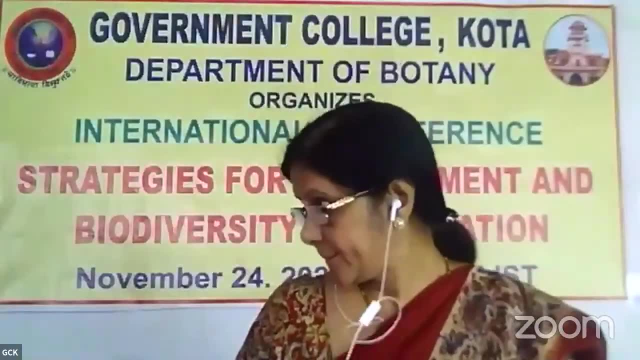 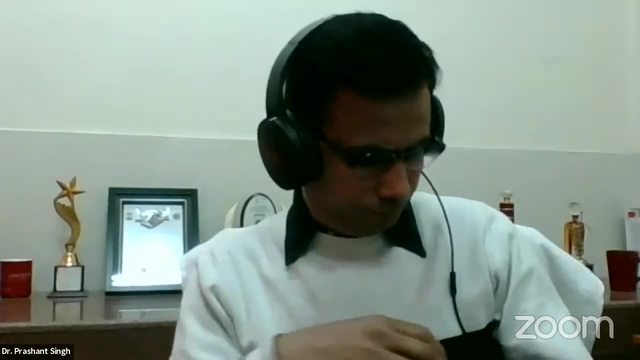 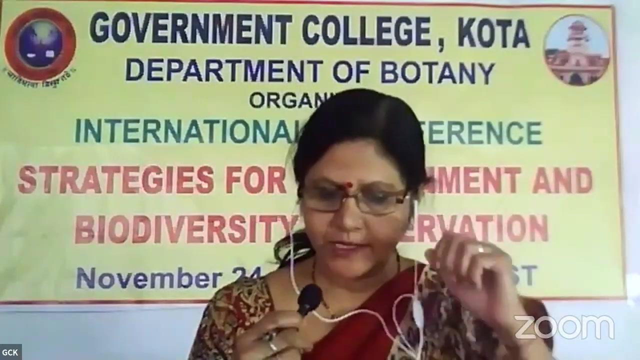 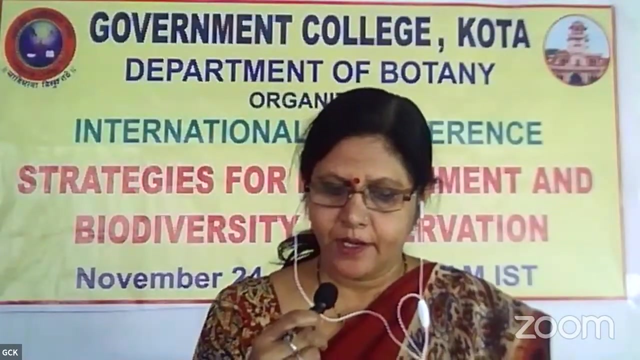 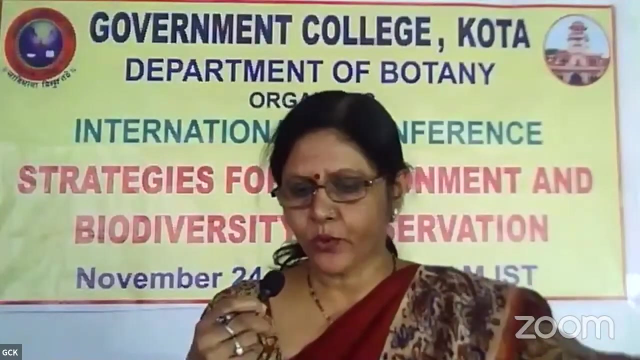 Sulekha Joshi of India, Namaskar. It is detail of Tambren Sikar. Dr Prashant Singh Singh, leader Ganga Ke Teer Par Rehne Wale Dr Prashant Ne Apni Doctorate Ke Upadhi UK Se Prapt Ki Hai. 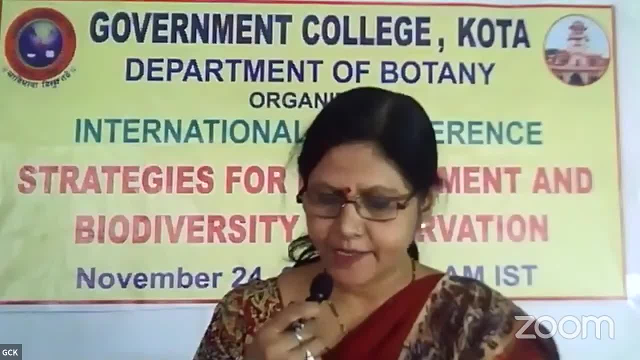 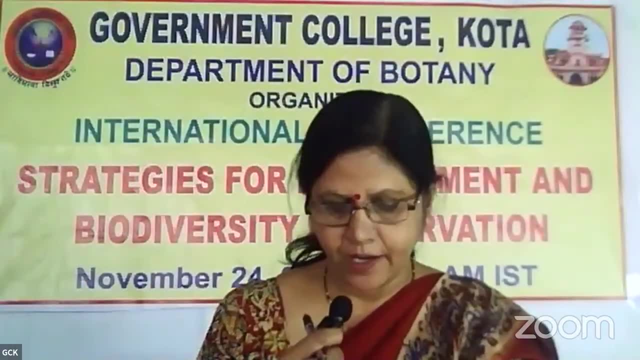 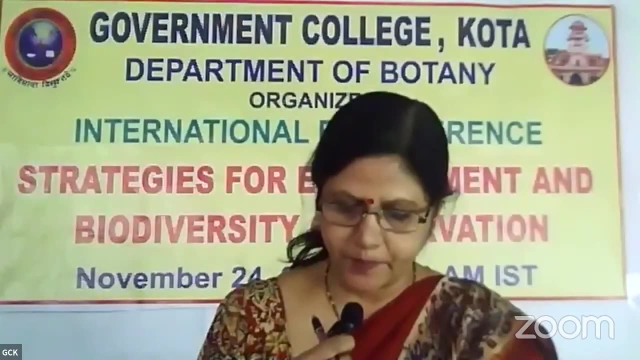 Aap Overseas Research Award, UK and NSC Postdoctoral Fellowship Award Se Nawaze Ja Chukhe Hain, Kayi Rashtri Va Antaraastri Generals Ke Editor Hain. 30 Se Jata Rashtri Va Antaraastri General Mein Aapke Shodh Patra Prakashit Ho Chukhe Hain. 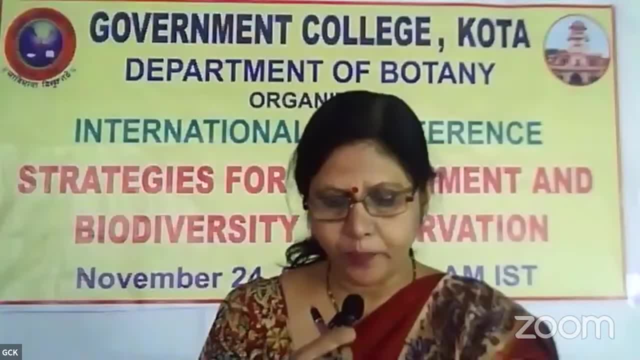 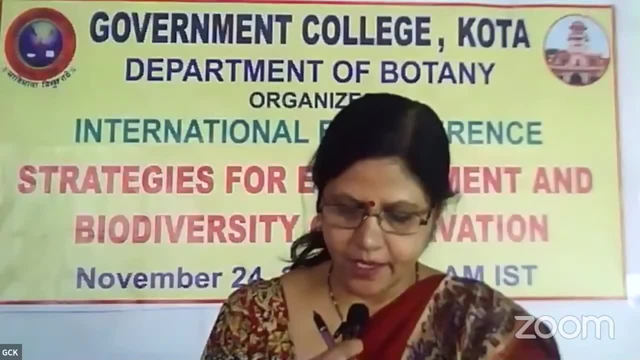 Arradiopsis Resistance Genes Par Aapke Do Patent Hain. Yeh Aapke Shodh Kari, Ki Bahut Badi Uplabdi Hai Aapke Is Gyan Ganga Se Hamare Sabhi Pratibhagi Labhanvit Ho. 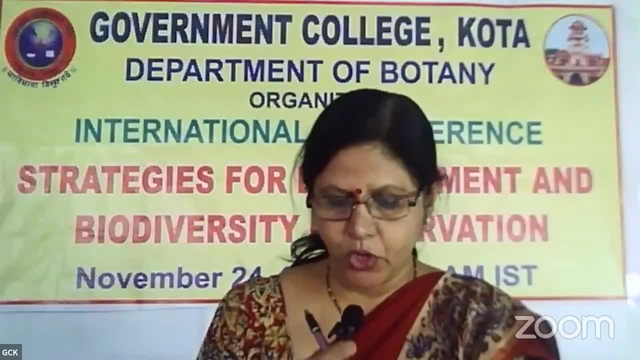 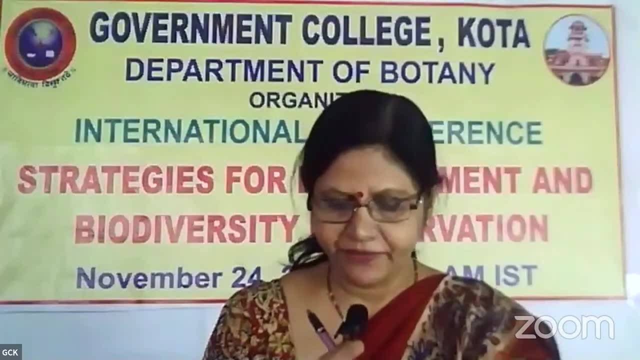 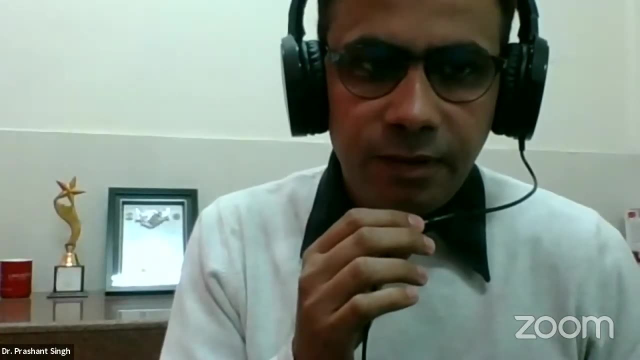 So, Sir, I cordially invite to Dr Prashant from Varanasi for sharing their knowledge on Green Vaccination for Human Welfare. Dr Prashant Sir, Welcome. I mean you're audible. can you hear me, Dr Prashant Sir, Can you hear me? Am I audible? 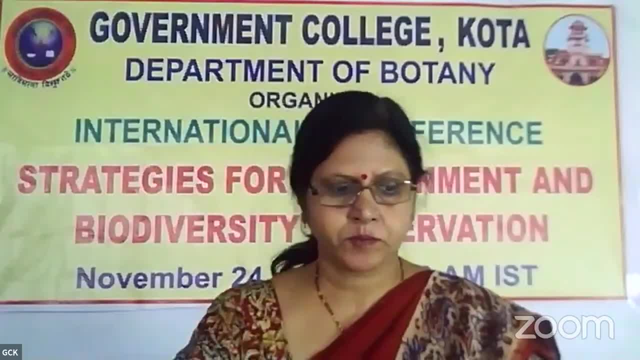 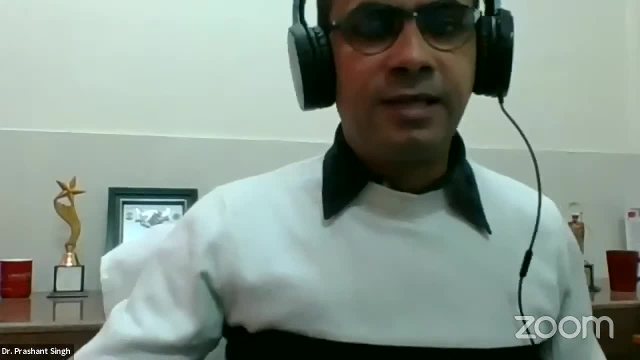 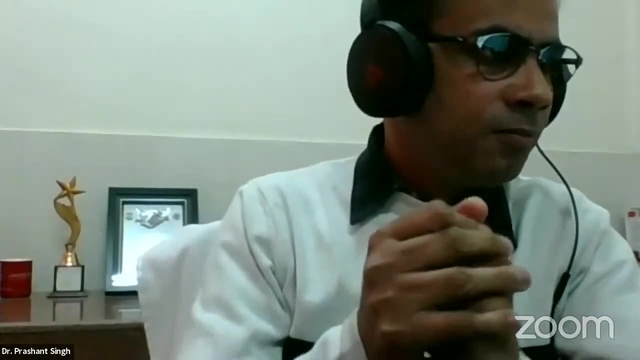 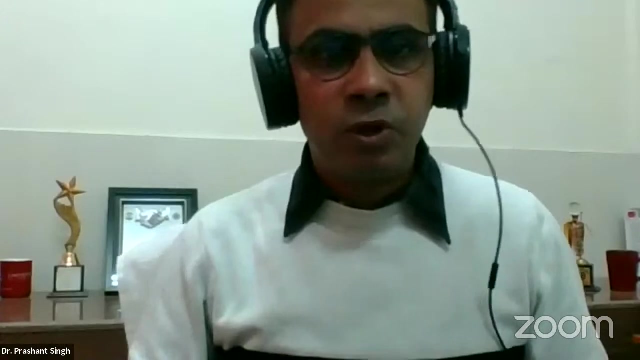 Dr Prashant Sir. Yes, Sir, Dr Prashant, Sir, Alright. So thank you very much for all these organizers in committee and your principal Vijay Vargi, leaders in Austria, Himlata Gupta, and all these coordinators for organizing a very nice international event. 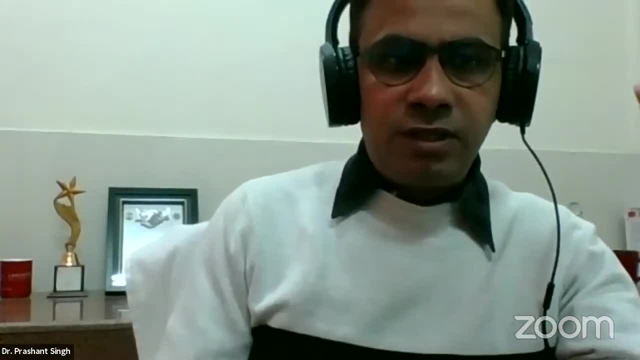 Dr Prashant Sir. Thank you, Dr Prashant Sir. Thank you. thank you, Dr Prashant Sir. Thank you very much, Dr Prashant Sir. Thank you very much for the panel and the involvement in the Bayan University conservation. 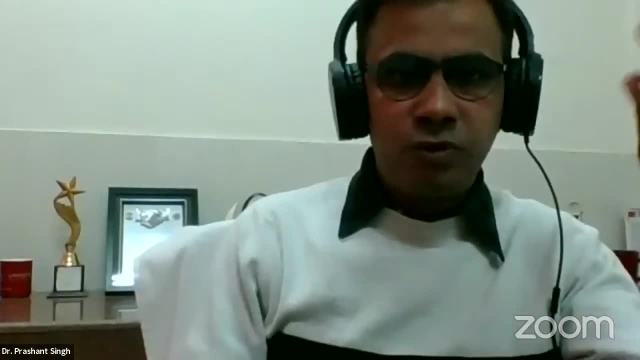 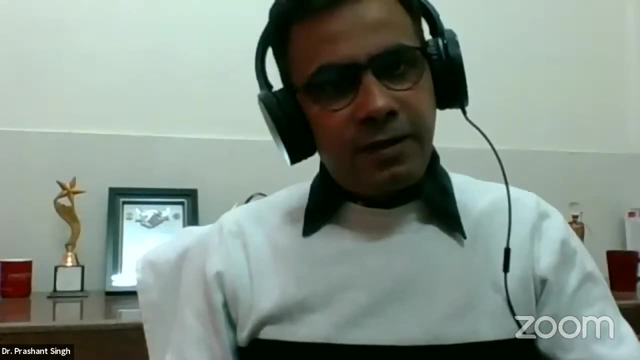 Dr Prashant, Sir, Thank you. So I'm really thankful and I will try to share my some views in my research work on the field that I was doing for the past eight to ten years and I try to connect in terms of the conservation as well as the analysis. 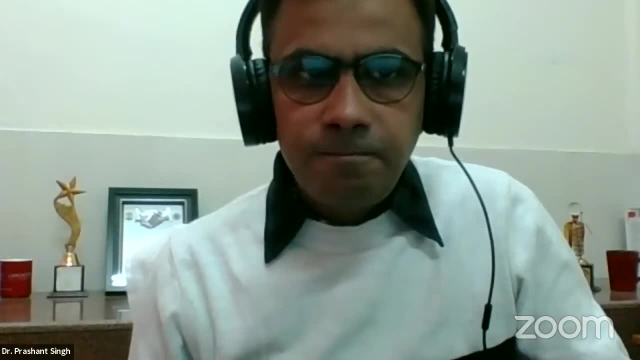 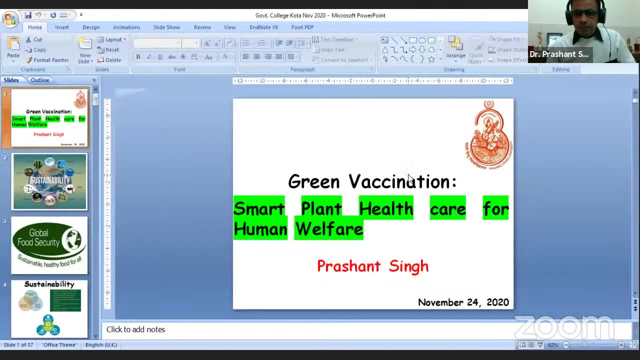 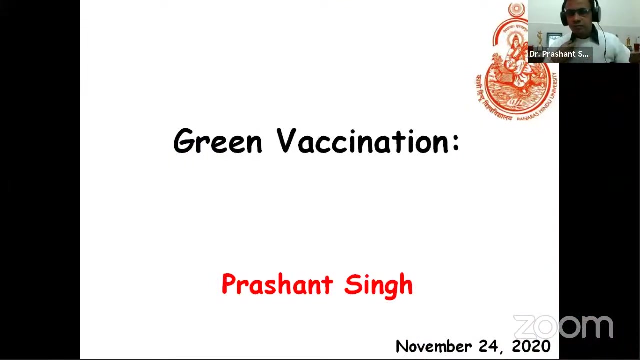 So let me share my screen first and then we can proceed. is the screen is visible? just let me know once so that I can move forward. is my screen is visible? is my screen is visible? yes, sir, visible, all right. so now we are in the 21st century and now you can see there is a. 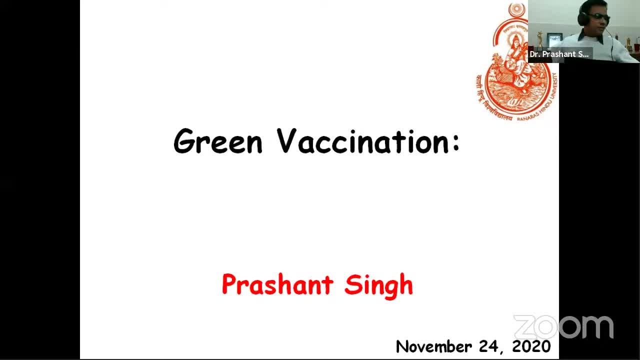 the word written here is like green vaccination. so you know, among the COVID pandemic, so I'm not going to talk about that vaccination, but what we talk in terms of the biodiversity, the data conservation- and it was really nicely touched with doctor. you know the different type of conservation strategies, but now what we need to do, I mean 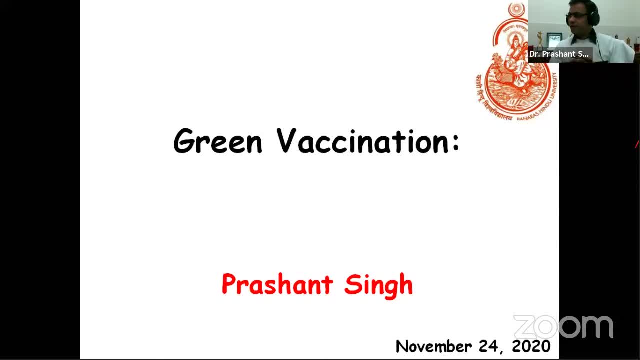 there are the different ways for these conservation and the one way we need to really understand to protect our the crops or to protect our the plants. and there is a different ways you can protect these plants to increase the bear diversity. but what I'm going to touch today a very novel way that you can protect your crop, and that's the 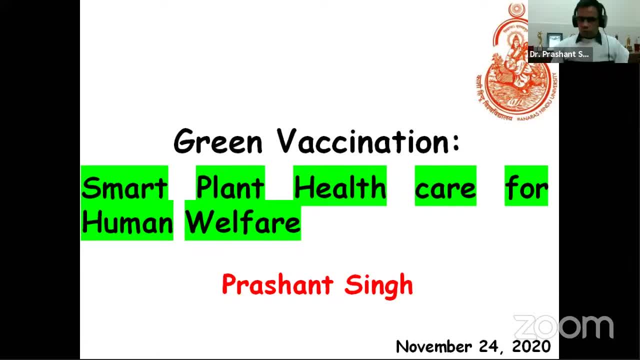 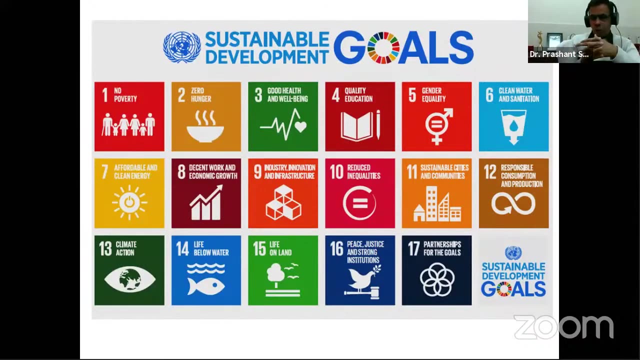 reason I have given the name, the smart plant: health care for human welfare. we know there are different SDGs, started with the UN long ago and we have to figure out these SDGs for the bear diversity as well as the bioconservation you can see here the parity, the 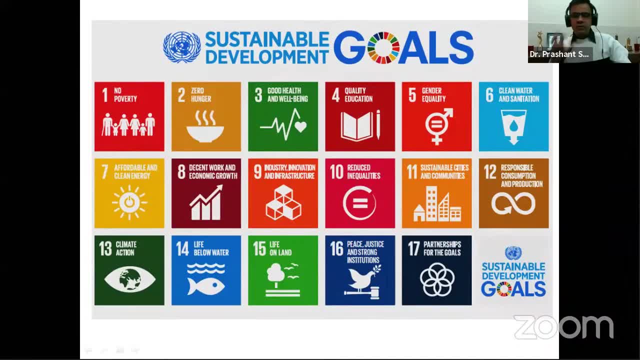 good health, quality education and, out of this, SDGs. one of the important SDGs is zero hunger. it means we need to feed billion of people, but it has to be sustainable. that I will touch later on. so this is one of the important goal of SDGs that also include this. 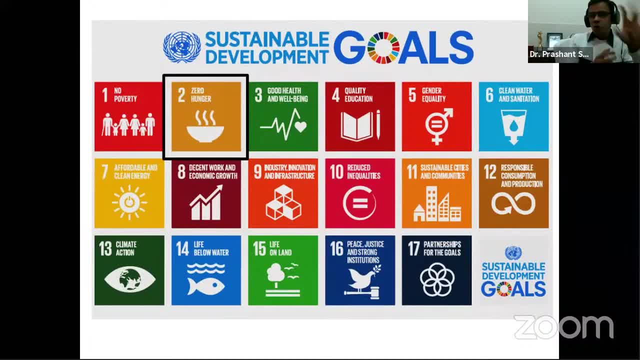 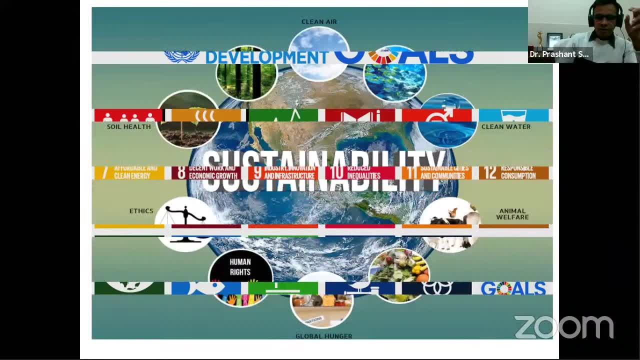 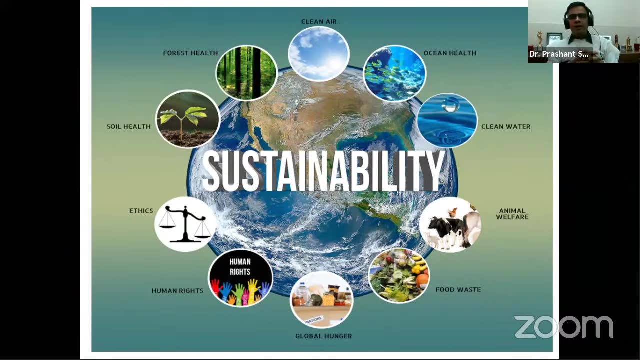 conservation, the bear diversity, that is the zero hunger that nobody should die because of the calorie and because of non-healthy food. more precisely, if we try to connect here sustainable agriculture or the sustainability, so you can see here these are forest health- a lot of people have already touched these- the clean air. 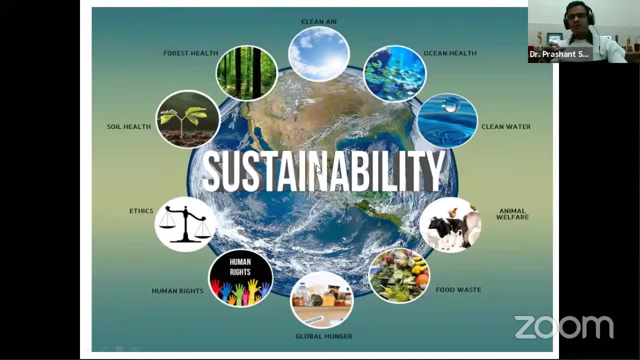 the ocean, health, the water, the food waste. so if we are going to bring all together and if it is sustainable, then in the real scenario we are going to protect our environment and we need to increase over the barracks. and what I'm going to touch today is the global hunger in the case of sustainable agriculture and nowadays, 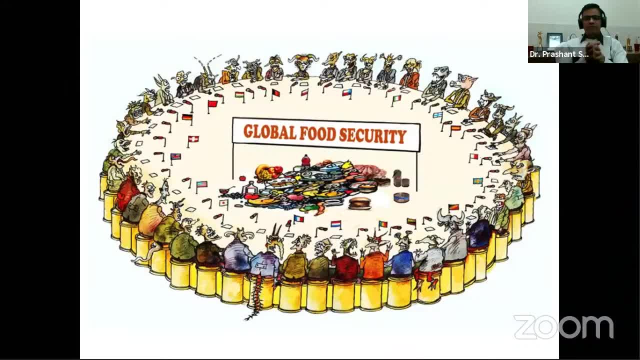 we talk every day about GFS, that is, the global food security. so I was the member of number of the panels overseas back home in states in London, Virginia, Paris, Germany- and gave a number of talk in the global food security. but the guys I never satisfied that if we solve even the problem of global food security, 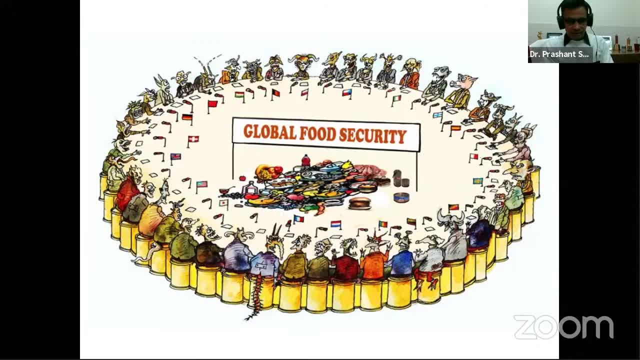 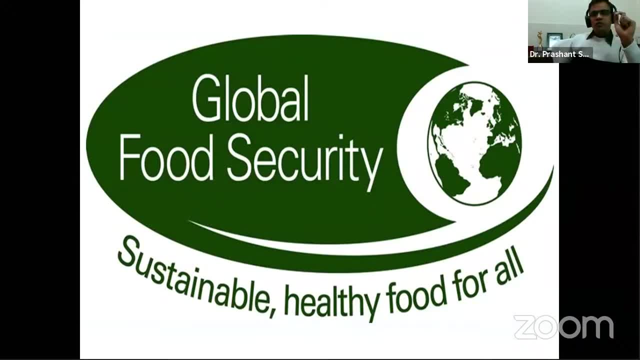 we can bring the sustainability. so in my head, the global food security has to be sustainable, no risk to the environment and the healthy food, for then we really solve the global food security. if we simply bring the enough food to feed the people, it is not going to solve the problem because we need to consider number of parameters. so for me, 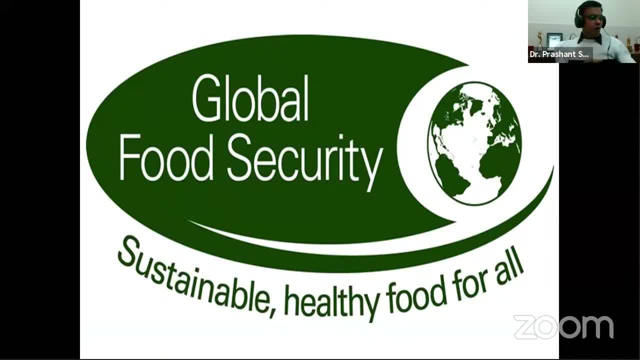 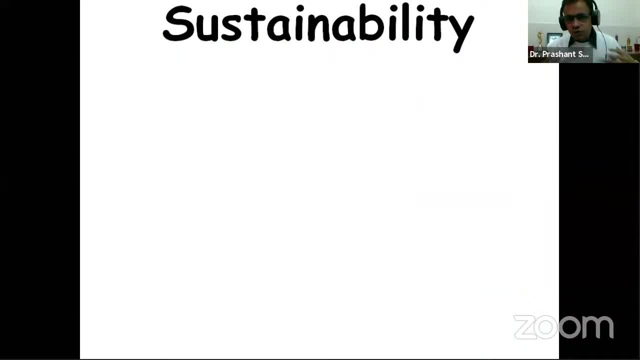 the only global food security is successful if it is sustainable. and we really need to understand, as a scientist, as a plant immunologist, as a conservatist, what exactly is sustainable. in a very simplified way, when we talk about the conservation, they are the three pillar for the sustainability. first is the environmental, health, profit and economic increase. 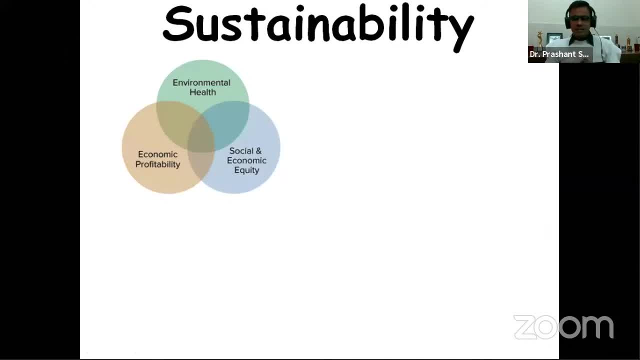 If we are missing any of these and even we bring the solution to the global food security, it is not going to work. So imagine you can bring a very nice resistant cultivar and you can bring into the system. Yes, you will increase the productivity, but there is a detrimental impact to the environment, to the soil. 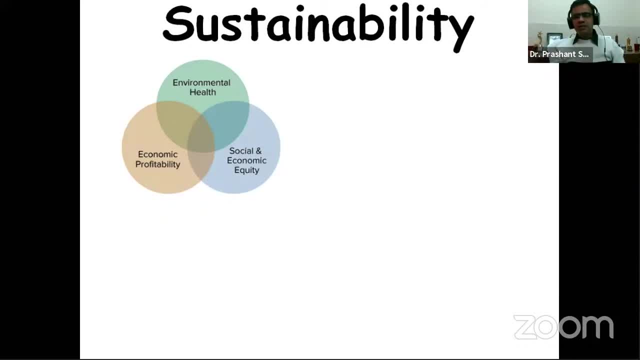 And we heard there is a lot of cases of the GMOs. So again there is a risk to the environmental health. Definitely it is not going to be sustainable. Second, even if there is no impact to the environment and it can feed the billion of people, and if there is no profit, again it is not sustainable. 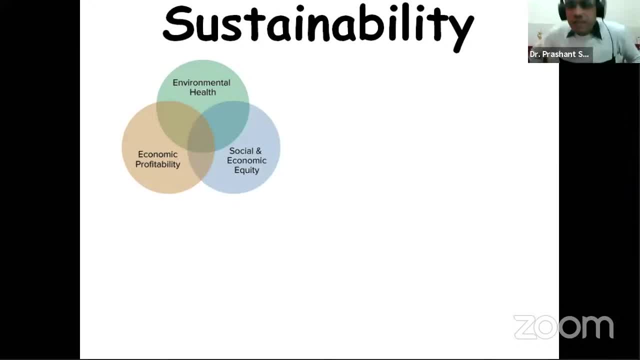 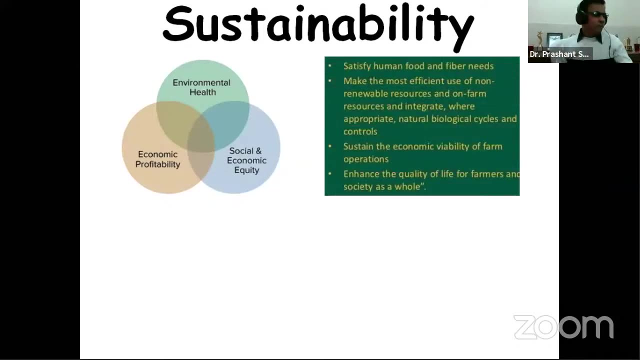 So we need to think and we need to bring any innovative tools to think in terms of sustainability And if we click all these boxes then it is sustainable. Otherwise it is not. In a very simplified manner, I can say that it should be safety for the human food, sustain the economic viability and definitely increase the quality of the farmers. 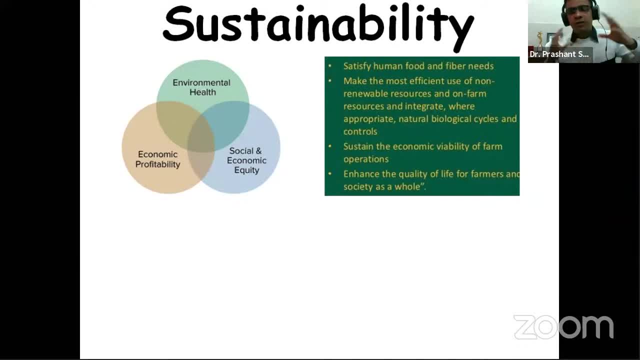 If you bring the very nice variety, there is no impact to the environment, But if you can't change the quality of farmer again, it is not sustainable and it is not considered as a sustainable. So in my head, as my name, Prashant, there are the three P's that are important: people, planet and profit. 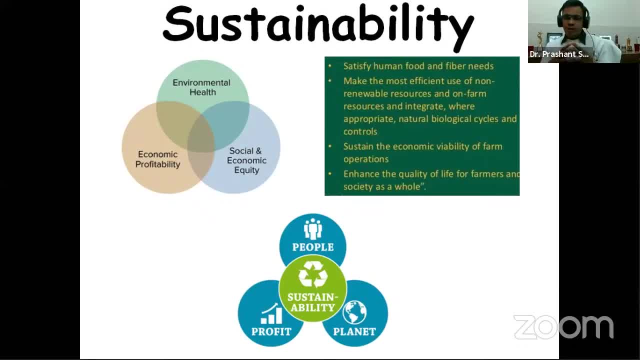 If we bring any new ideas, any new innovation that we can tick all three boxes- people it means definitely can feed the billion of people planet. there should be no impact to the environmental health. And thirdly, that once you have the profits, if you bring all the three pillars, then it will be sustained. 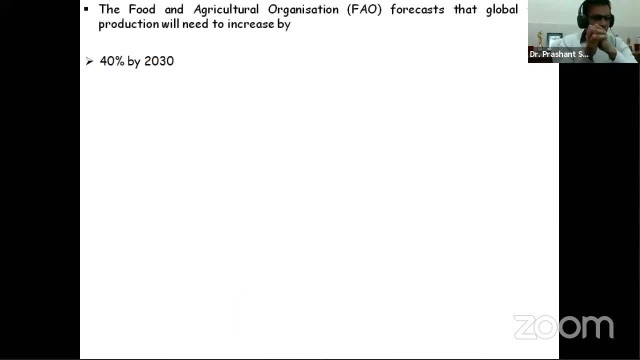 And we know that FOI already forecast that we need to increase this global food production, In fact, the sustainable global food production, almost 40% by 2030 and almost like 70,, more than 70% by 2050, because there is a population growth. 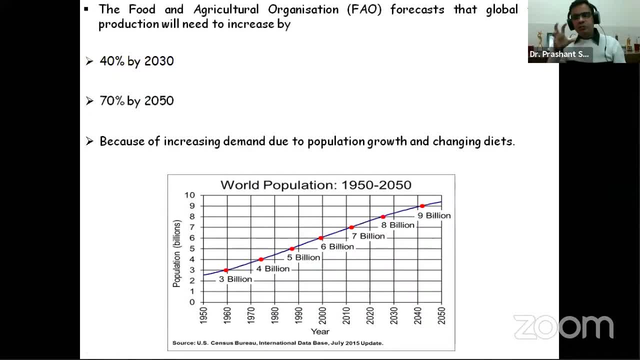 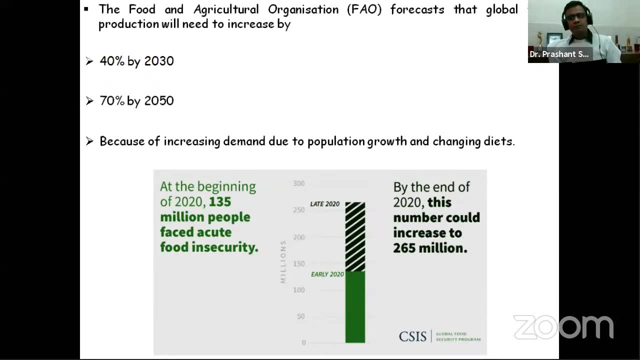 The population is increasing exponentially, so we need to protect our biodiversity, we need to protect our crops because there is a big problem of the population growth And it was recently said- at the beginning of 2020, it's almost like 130 million people were facing acute food insecurity. 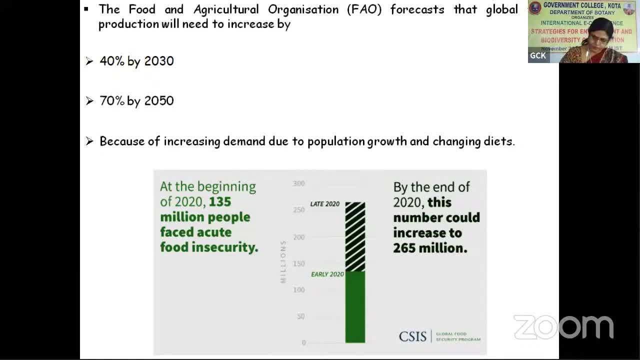 And we are not going to bring any innovation. But if we have an innovative solution, this number is going to increase by 264 million. So look the guy, the scientist and the student. we need to think in that perspective to bring some new ideas. 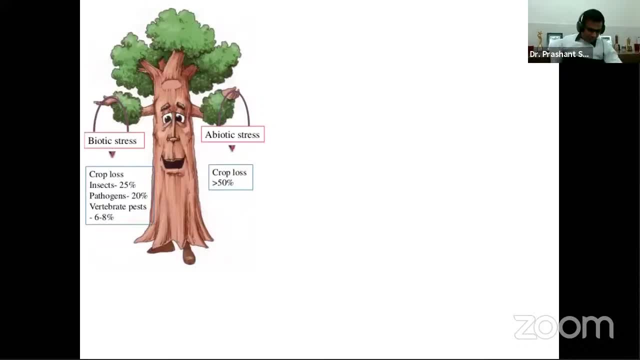 What to do. I really love this guy. I mean, whether you can consider him as my boyfriend, girlfriend, whatever, I really love this guy. I really admire him. The reason behind that you can see. In fact, he's suffering from different kind of stress, whether it's the bearing stress, whether it's the aviary stress. this guy is still smiling. 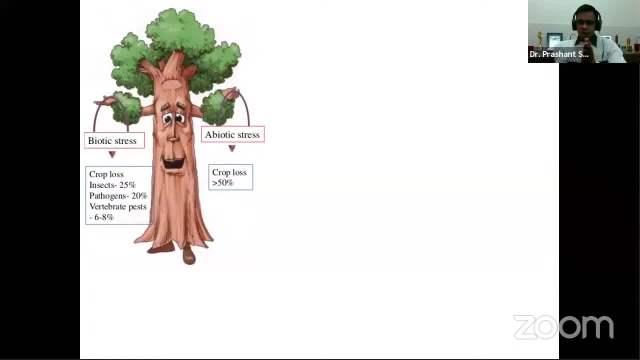 So it's our duty to protect our plants, to protect our crops, to conserve our biodiversity, And there are a number of ways you could do this, And I'm not here counter saying that these methods were not good. They are, But now we need to bring some more innovative method. 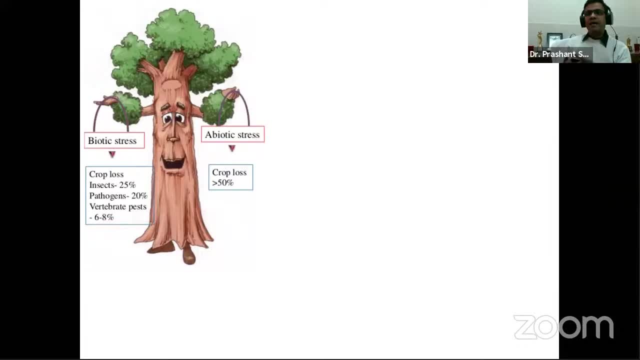 To bring sustainable agriculture production. We know that they can eat the plant and you can create this resistant cultivar, But, yes, it takes a bit of time to bring this cultivar to the society. Moreover, we can go for the transgenics. 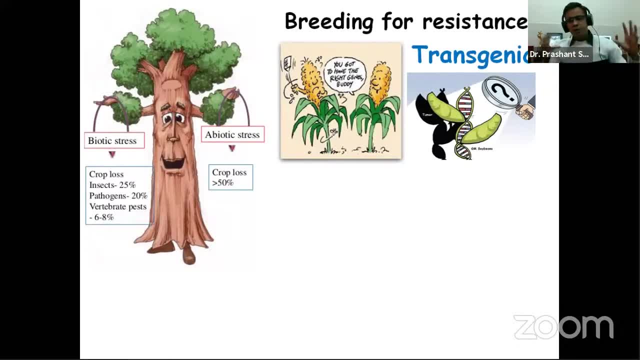 You can create this genetic engineering. You can transfer the gene from the bacteria to the crop and the vice versa. You can create the number of transgenics, But, guys, still this is not acceptable Because we have the problem of these GMOs. 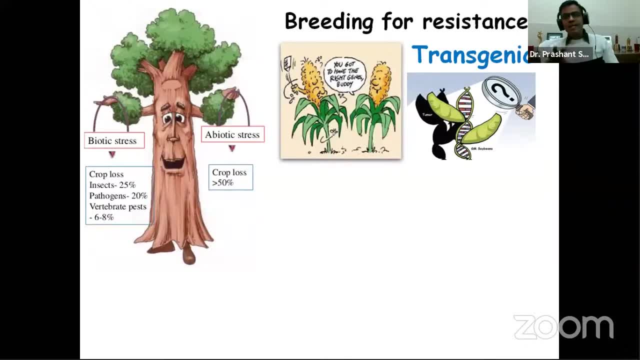 And once I was in Switzerland, the people are very offended if you talk about GMOs. Now we have switched to CRISPR-Cas as a very new technology And we said that it is not GMO, but it is genetically engineered crop. 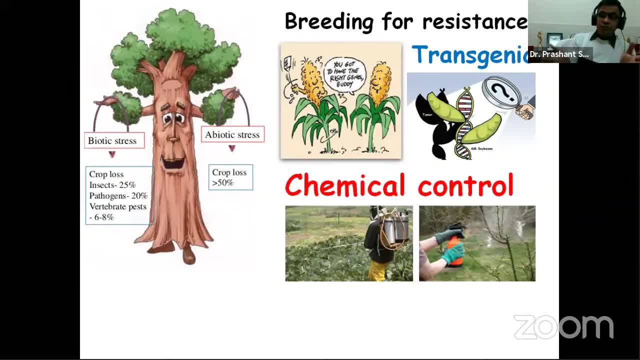 But again there is a problem. However, we are using insecticide and the pesticides, But again I told you, there is a protection, But there is a risk to the environment. So definitely this is not sustainable. So what to do? 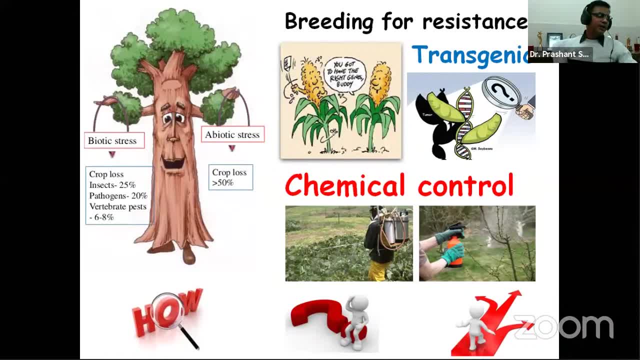 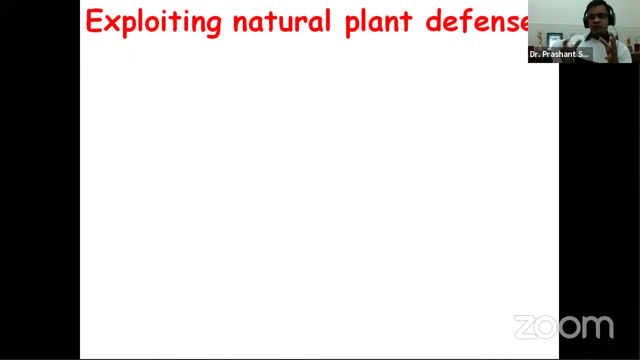 There is a lot of way of thinking And we need to bring some novel strategies to protect our crops. And I can tell you, guys, These plants are very smart, You don't need to do anything. In fact, they are smarter than us. 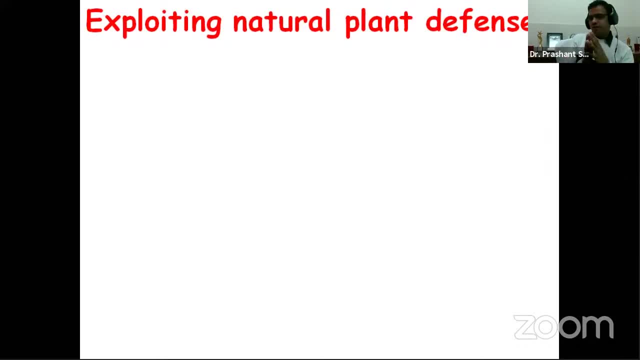 In a very layman language: what do you need to do? You need to simply aware them that they have their defense response And after that you don't need to do anything. Then there was a question. was there for these guys? 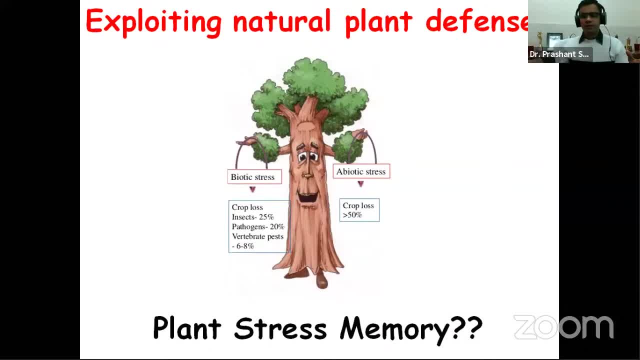 Do these guys have the stress memory? Because now, as a human, when we face any kind of pathogen or any kind of stress, We have different kind of cells in our body like T-cells, B-cells, helper cells, memory cells. 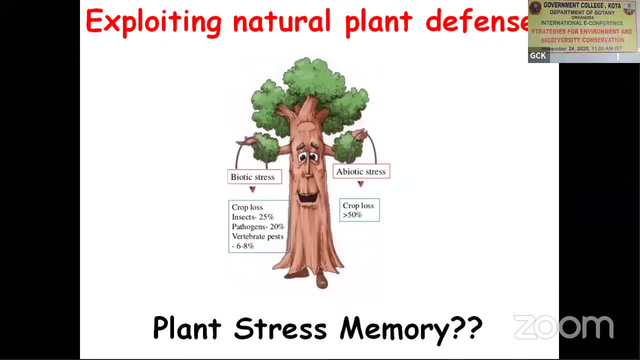 They can record the information. Yes, you are going to face with the bacteria or the viral disease and they can store this information, But unfortunately the plant doesn't have any well-defined immune system. What to do? The thing is that they are very smart. 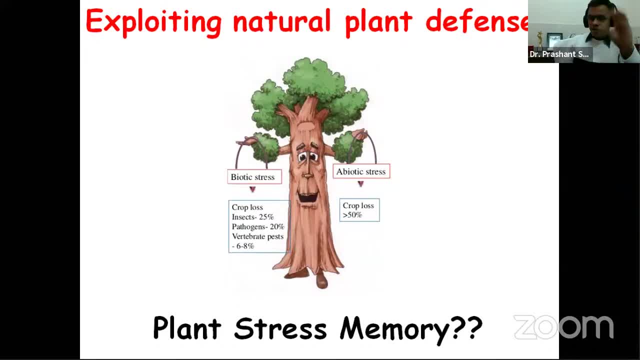 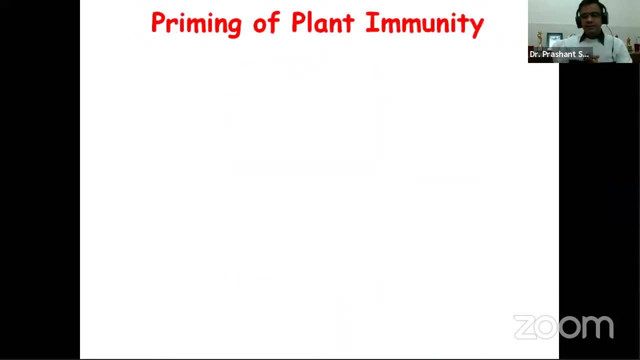 Every plant cell, in the case of the crop, acts as an immune cell. So for me another big question was that: could the plant have a memory if they face one challenge and they can remember, And we call this as a priming? 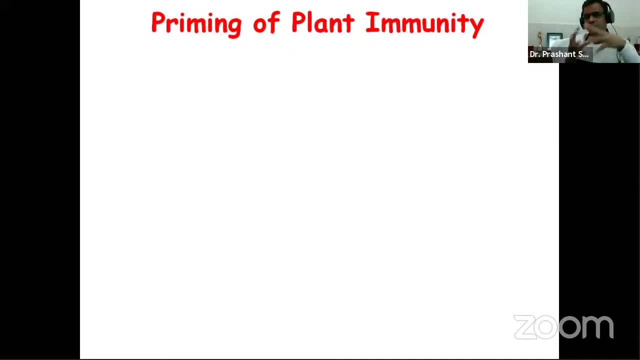 Just try to focus on this slide, because this is the main G-stop. This is the story and this is the main selling point of the talk in terms of conservation, in terms of sustainability, in terms of environment, in terms of balance. Just focus on this slide carefully. 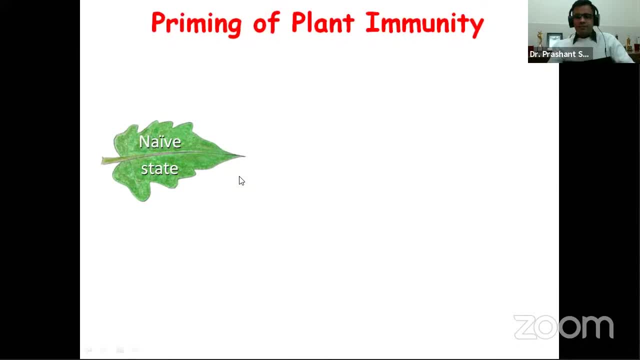 So imagine this is your normal plant. We know that if the plant is going to face the biotic attack, there is a response And we call it an induced response. But what happens during this induced response? Imagine this is the plant leaf, and if this plant is attacked here by the pathogen, then there is an activated response and that is called an induced response. 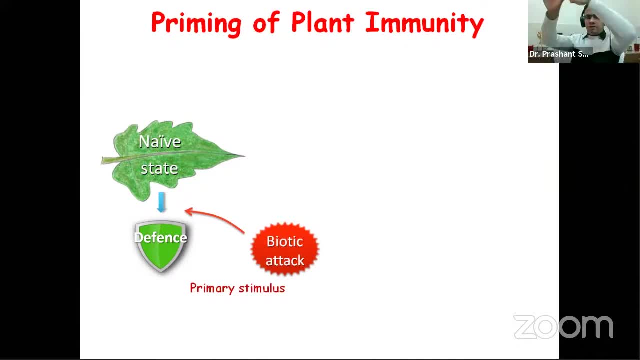 As the signal is perceived here. now the signal is translocated to the other parts of the body And plants feel that they have faced the challenge And once they've felt it, they are in the alarmed state, They are in the vigilant state. 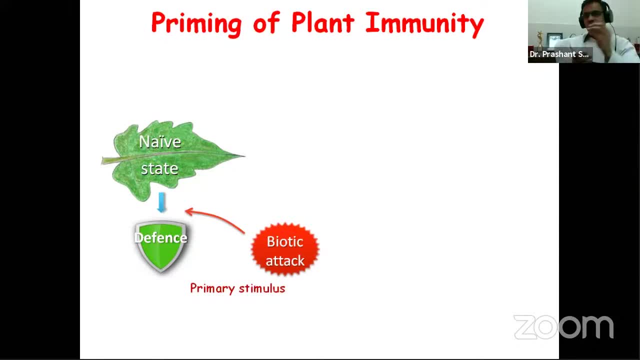 You know, like a very simple example I always give this analogy: Imagine that in your school, if you think that there could be a visitor of your vice chancellor or the principal in your classroom who are very vigilant, and imagine there is one more guy. he doesn't know that there could be a visitor of vice chancellor. 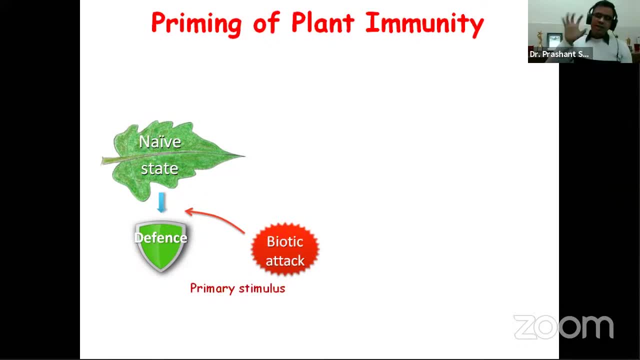 He should not be very active. What will happen if the vice chancellor will visit the guy who was vigilant? He feel that, wow, you know his desk is clean, He's doing his work because you knew that there could be a visitor of vice chancellor the other guy, he doesn't know. 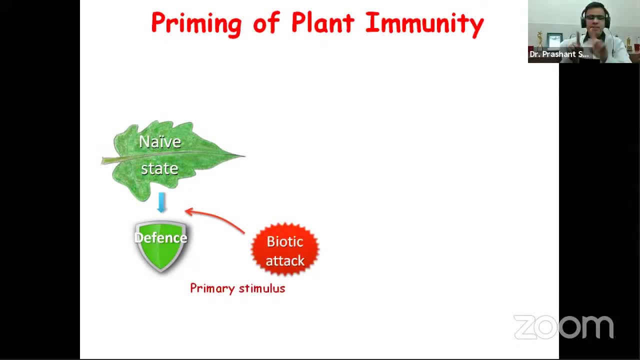 And then he could be in the problem. But it doesn't mean that there is a big difference in terms of these two guys. The only difference was that the one guy was vigilant because he sensed that. Similarly, in the case of Karn, when it is attacked by any pathogen, during this induced resistance. 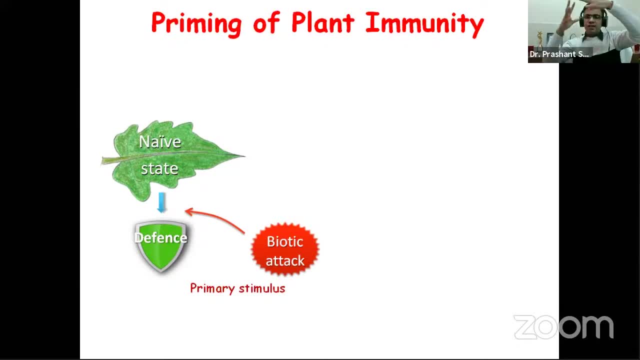 they can sense the signal. and once they sense the signal, they can transfer to the different distal part of the body. And this sensitization of stress responsiveness during induced resistance is what we call as the crime. You know, it's just like a vaccination. 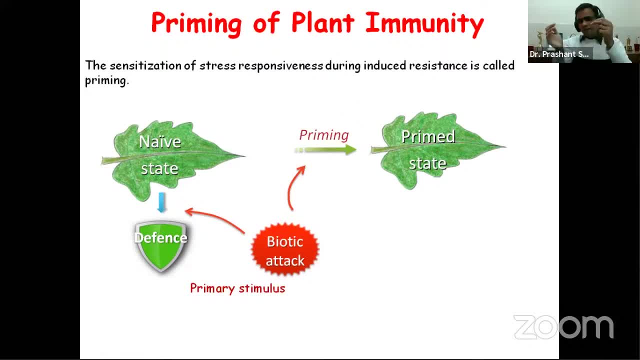 You know what is In terms of vaccination: you get an antigen of the same pathogen that caused the disease and then the body itself develops antibodies. And in the case of the plant, what we do? we use the same pathogen to bring the plant into the alarmed state or the activated state. 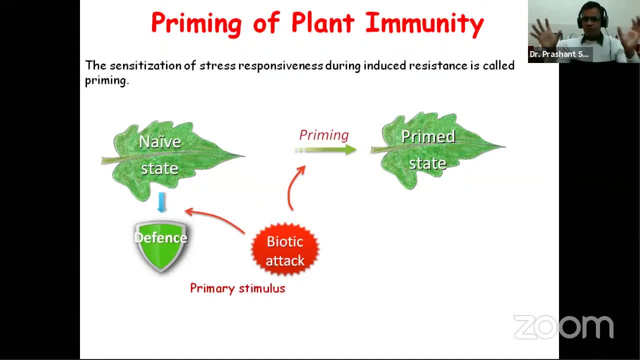 And this activated state is called as the priming. That is the very important term. I try to draw a line. So In the priming the plant is only in the vigilant state. There is no activated defense response, Because if the plant will activate its defense response, most of the time there is a yield penalty. 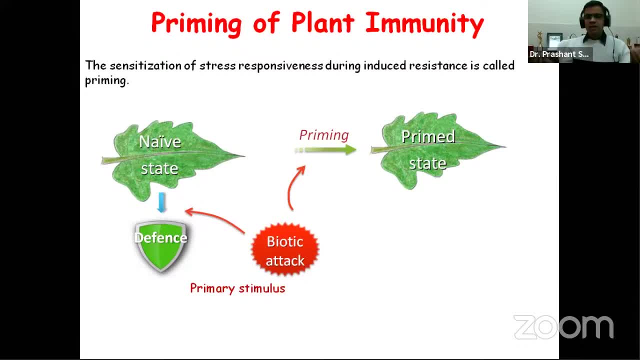 As a farmer, as an agriculturist, you don't want a super resistant plant with the reduced yield. But here the beauty is that the plant doesn't Increase the defense capacity. yet They are only in the alarmed state because they have faced the first challenge. 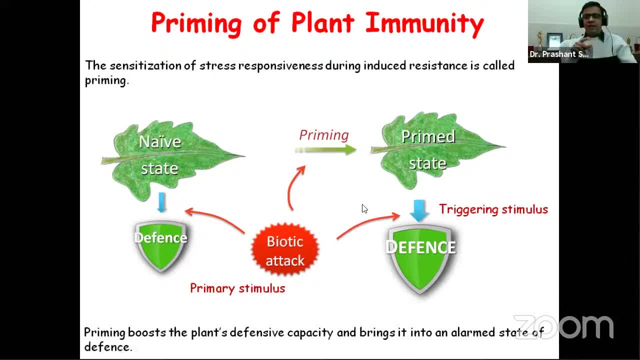 And what happens When they face the challenge again. you can see that there is an increased defense response. It means defense response is unsteady, And that's why this priming brings the plant into the alarmed state And increases The defensive capacity. 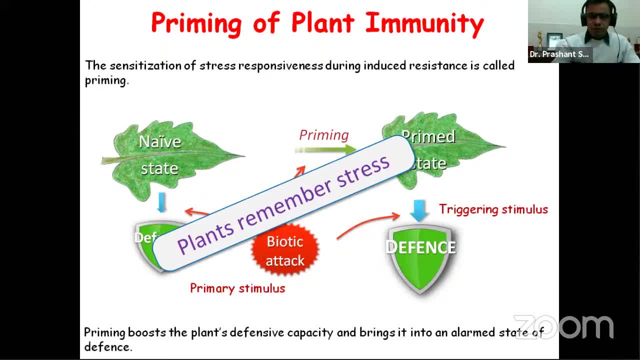 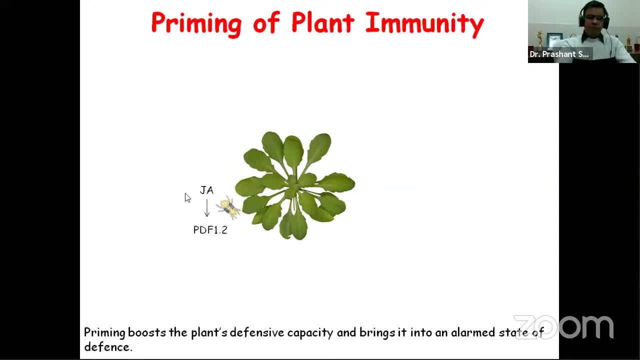 See here. So indeed, the plant remembers stress. Now see here. This is the one of the plant, The other plant we call the rabidopsis. If this guy has faced any challenge, you can see that this is. I think you must be knowing these are the defense hormone, the jasmonic acid. 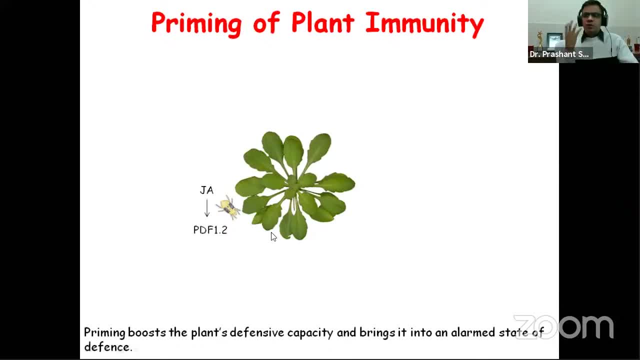 And then there is an activated defense response, The activation of: Okay, What happened Once they are attacked? now the signal is translocated to these digital parts of the plant. And what happened here? They are in the activated state, They are in the vigilant state. 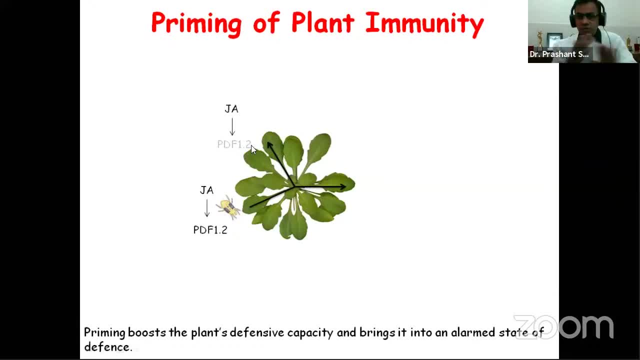 They are in the alarmed state But still there is no activated defense response. It means the plant is not retranslocating its photosynthetic for the defense response Once it faced the challenge again. now you can see that then there is an activated defense response. 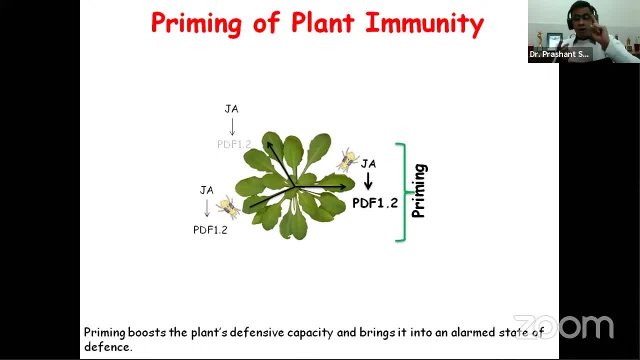 And that's what I said. This phenomenon is very important because what We are not using any insecticide, We are not using any pesticide, We are not creating any transgenic, We are simply bringing the plant into the alarmed state or the vigilant, or 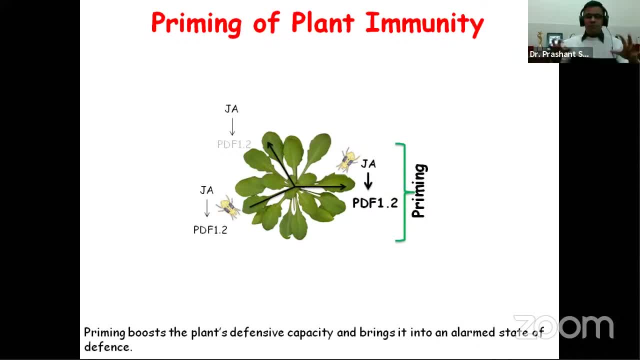 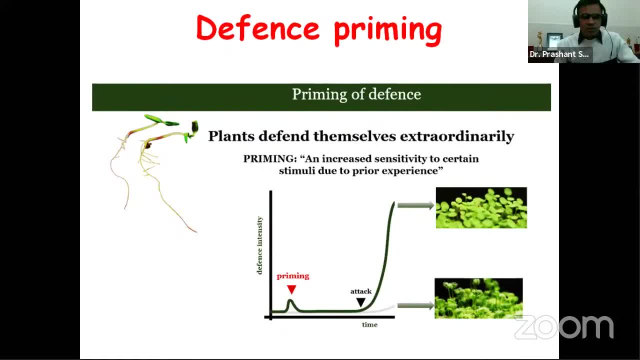 And I can clearly see here. this is the defensive capacity Once the plant is primed. you can see here, And when they are going to face, that there's a huge difference between the prime plant and the prime plant. The prime plant can defend themselves extraordinarily. 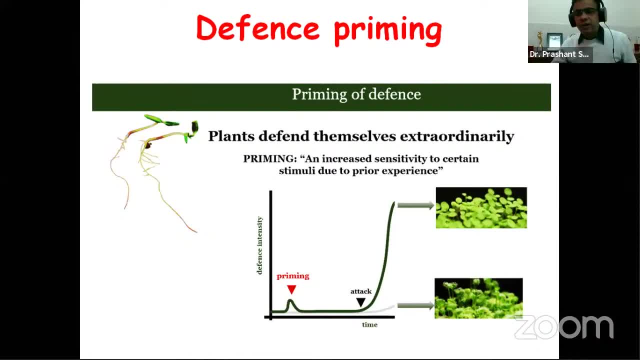 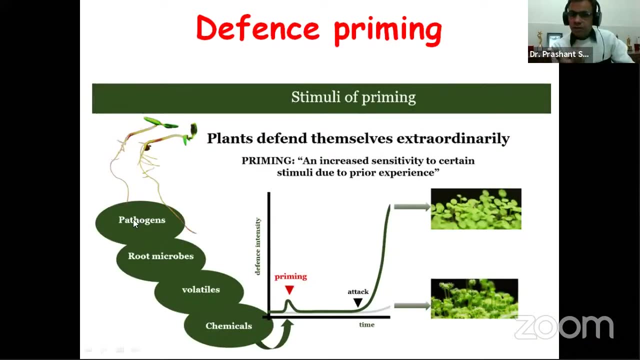 Now the question is that what could be the way that we can do this defense priming? So I gave you an example. You can use the same pathogen bacteria virus that cause the diseases. You can use the pathogen to bring the plant into the primary state. 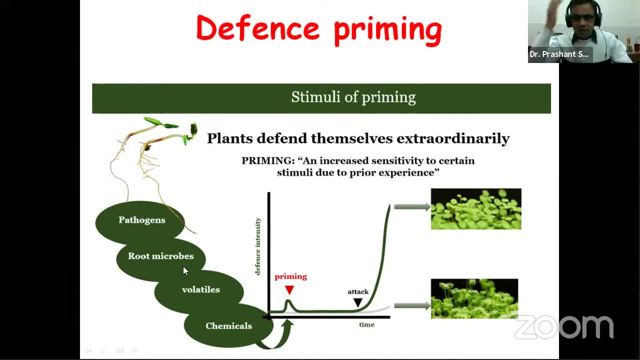 You can use the root microbes. in the next talk He can talk about the PGPR. yes, This could be also one of the candidates to bring the plant into the alarm state. You can use the volatiles. You can use the certain chemicals, elixirs that could bring the plant into the alarm state. 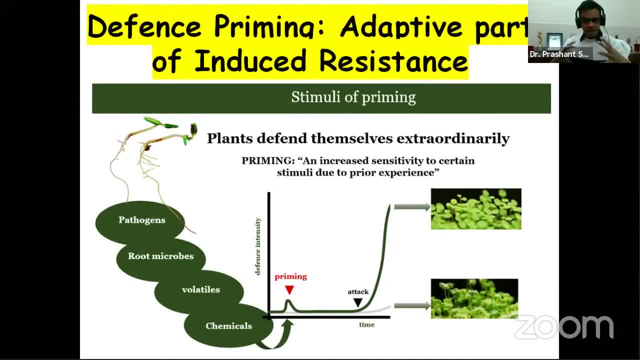 And that's why it's very simple. What is that? It is a. It means during the induced resistance, the plant has sensed the stimulus, and that's why it is an adaptive part of induced resistance. And now the biggest question is that. 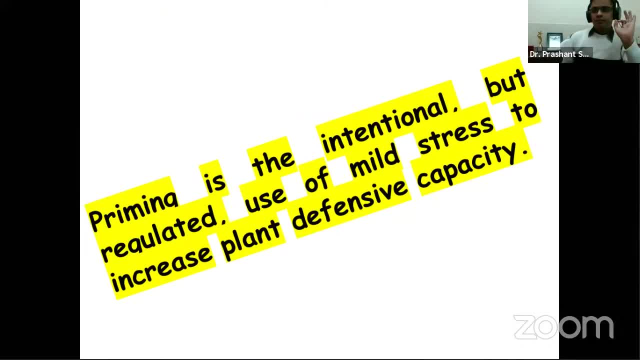 So that's why I said here that it is the intentional. We are bringing the plant into the primed state to protect the crop or to conserve over the diversity. So priming is the intentional, but regulated It means you can easily regulate. 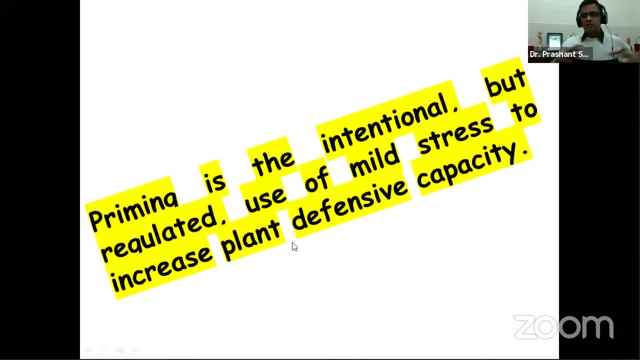 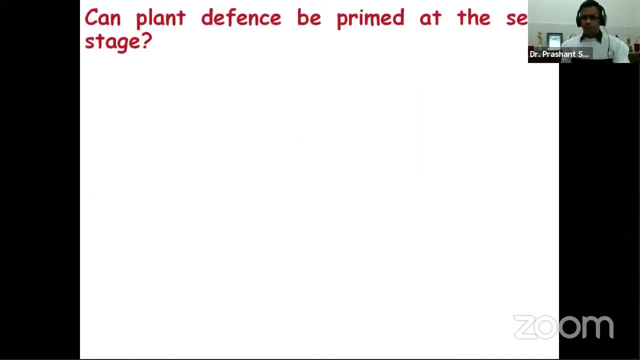 Use of mild stress to increase the plant's defensive capacity. The second point is that what could be the best stage to prime the plant, Because of shortage of time, it can't soak so much. Yes, you can simply prime the plant even at the seed stage. 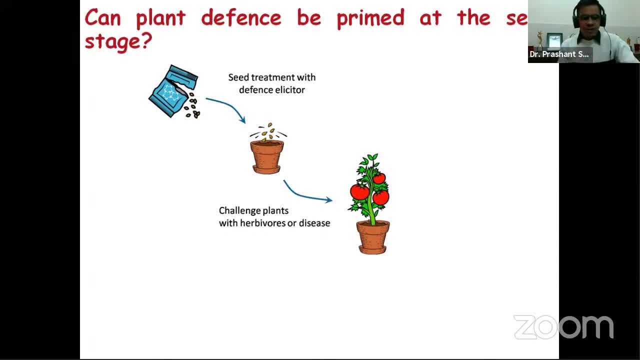 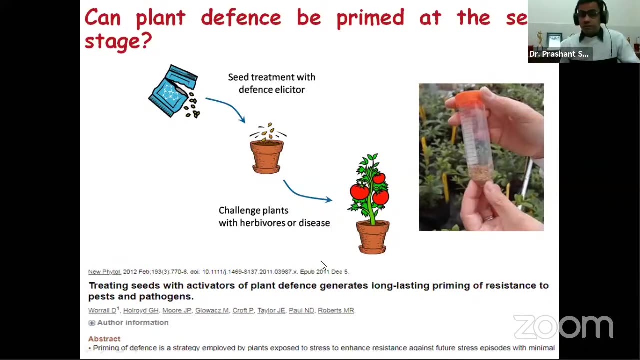 If you have the seed, you can bring the seed into the prime state, like here. I mean, this is the tomatoes. They are treated with certain licitors, Hot And now these tomatoes were super protective And we already published this word in one of the reputed long journals, in the Neophytol, long ago. 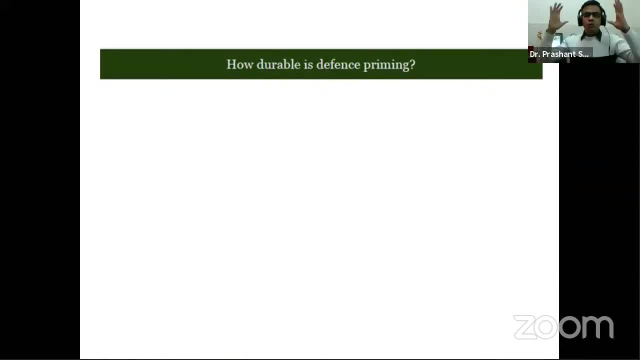 Now the question is that: how durable is priming? So imagine you bring the plant into the alarmed state. you know, because in the human cell they have the memory cell. they can remember forever. But in the case of the plant cell, if they are primed, how long? 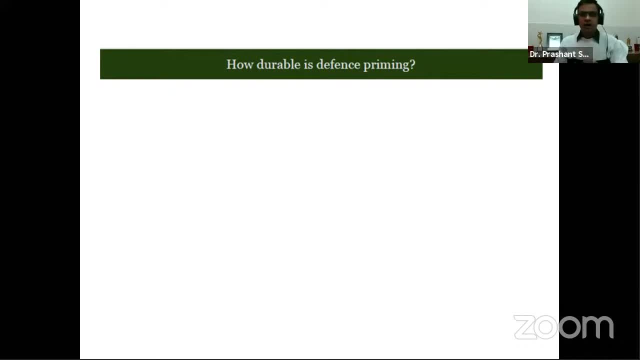 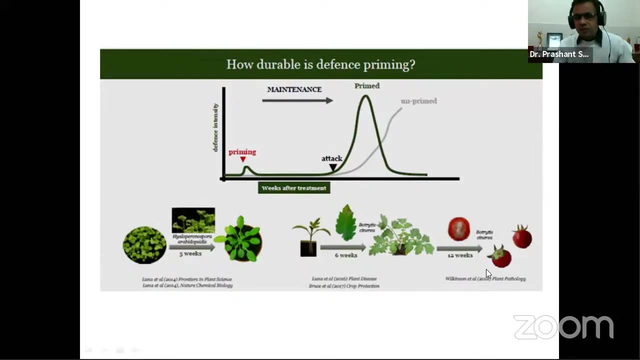 They can remember. That was the biggest question that you could ask And you can see here, even after five weeks, six weeks, 12 weeks, it clearly suggests that the priming could be maintained even after two months, even after four to six weeks after treatments. 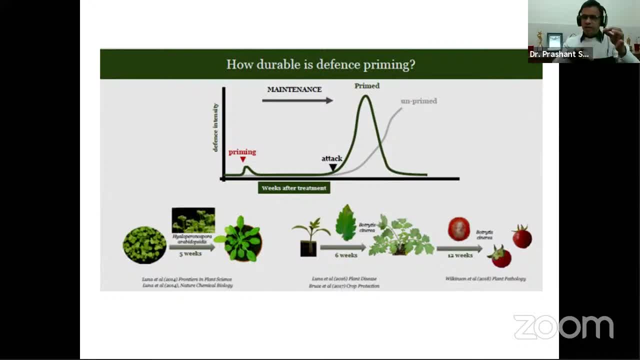 Imagine if we treat the plant today and you can leave the plant you know grow like that normally And then you can challenge again after two months. Still they have this kind of memory or the sensitization. So that was a very burdening discovery. 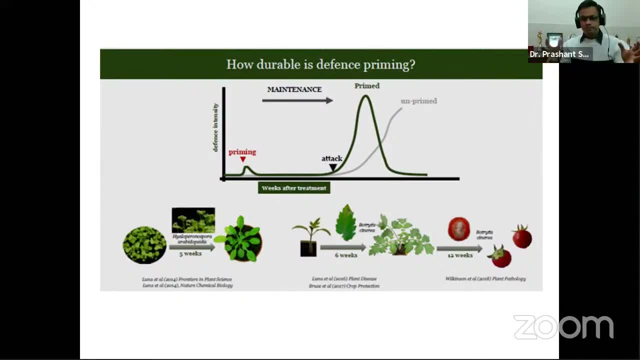 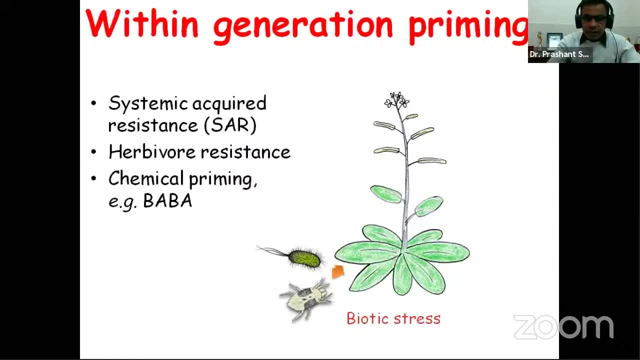 What we found, that this priming is durable. It means this could be maintained for a pretty longer period. So we call that. if the plant is primed within the same generation, it's the part of SAR. So imagine, here it is the stress, if it is challenge. 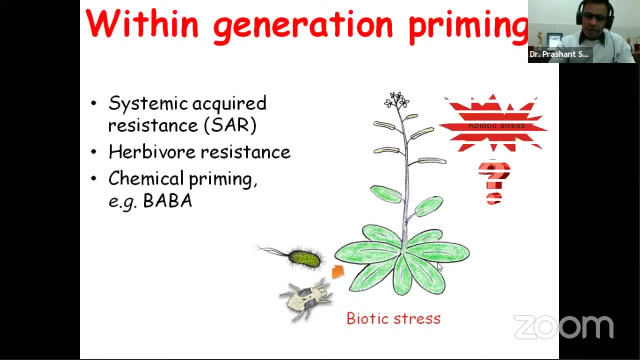 The plant is the problem. The third important question was that if we use the A barrier stress to bring the plant into the prime state, could the plants are primed again? the barrier stress It is not really the cross tolerance, because in the cross tolerance there is the interaction here. 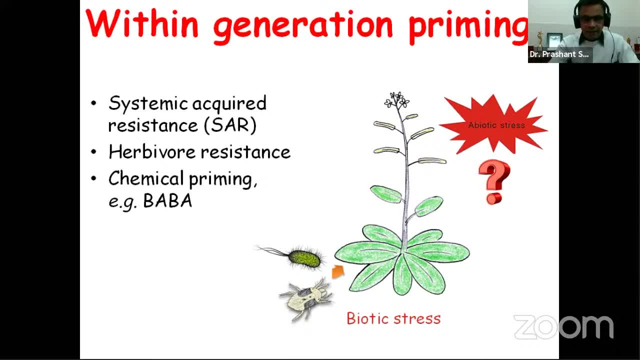 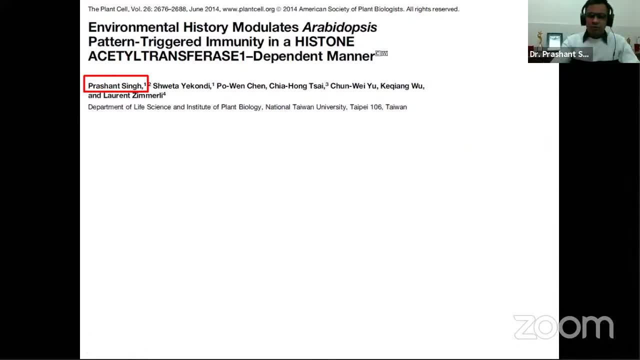 You are simply bringing the plant into the long state. And again, it was published in the Plantswell. it's one of the very reputed journals in the plant science And what we found here you can see here. we didn't do anything extraordinary. 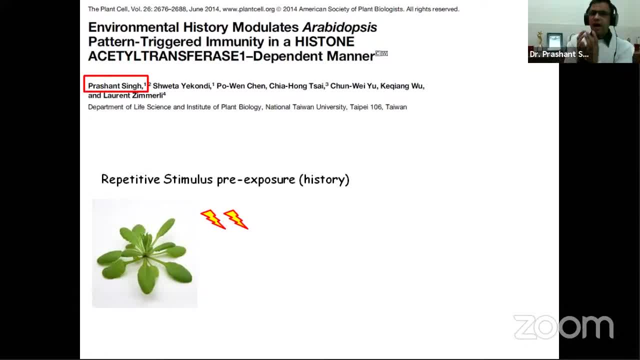 So that's a good point In some time in science the idea has to be novel. You don't need to do a lot of work, but you need to think beyond the black box and you have to have an innovative approach to bring the solution to any problem. rather than you can do the repetition. 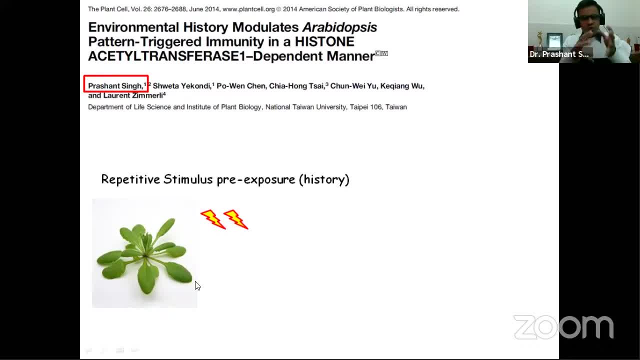 What we have done here, simply here. So this is a normal plant. We kept the plant at 26 degrees just for 10 minutes And we have used the cold He saw, but I'm just showing you here the heat, And after that we did it for seven days. 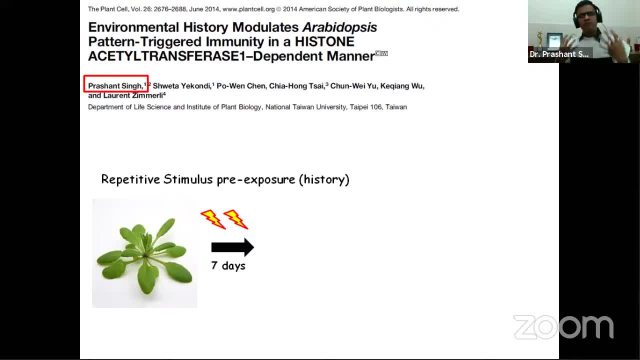 And the hypothesis behind that. maybe after seven, five, three days the plant can remember that they're going to face the smiley stress again And this could bring the plant into the prime state. I can clearly see here: after the priming there is no big change in terms of the morphology, which means there is no genetics here. 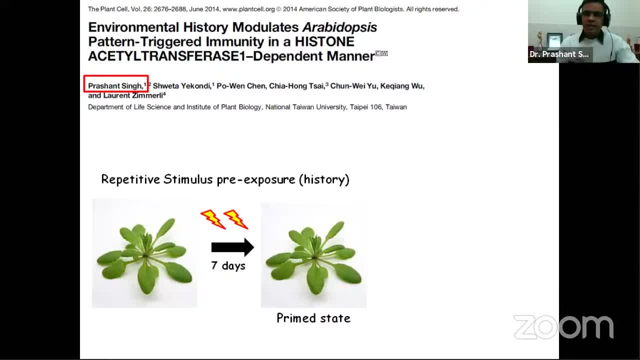 I can't talk, but I can tell you the mechanism is totally epigenetics And after that they were faced with stress. is that? see here, These are Zero means no heat stress. Five and seven. You can really see, after seven days of the mild heat stress, bring the plant into the prime state and when they face the challenge, 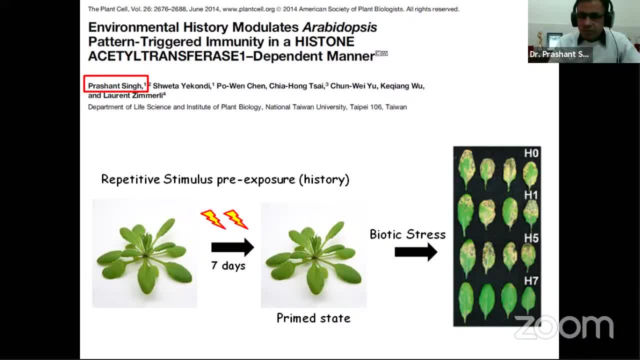 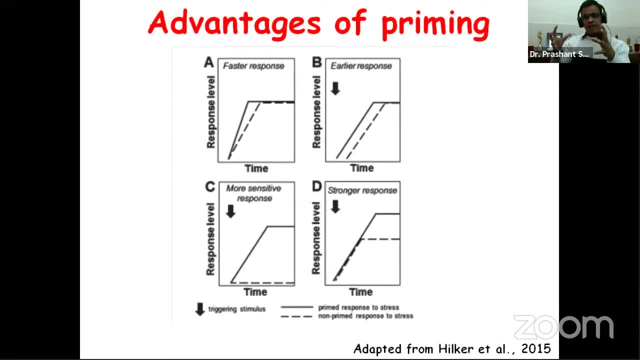 That's every day, Same thing happens challenge. they are super protective, so this is a real beauty. i think i have already explained you what is that. what is so? if the plants are, the prime response is faster. you know it is, you know, like a cctv camera. imagine in your house if there is a cctv camera is there? your response is quicker. 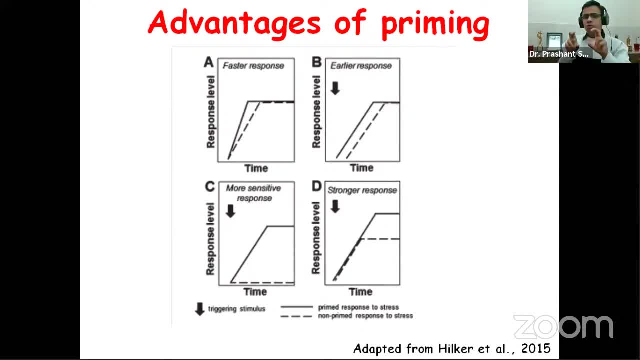 you can easily see who is coming to your house, so earlier, more sensitive. then you will be ready with the different bullets, but you will be fired the bullets only if somebody will break the door. if somebody is not breaking the door, you will not fire the bullets. in other scenario- imagine there. 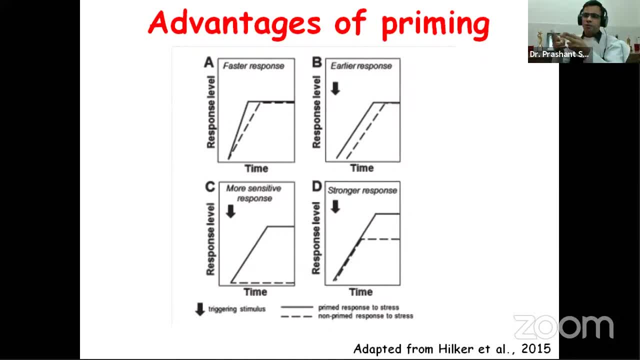 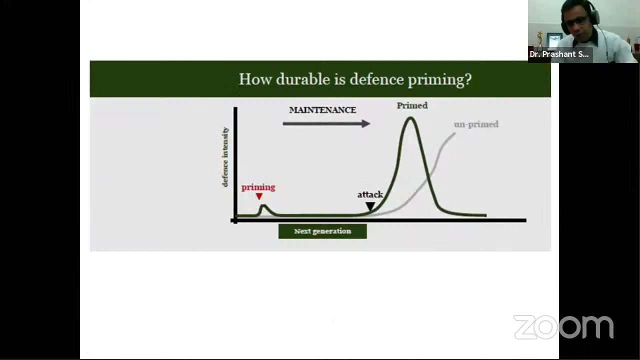 is a guy who is on the roof and he is just firing the bullet that nobody will come. so there is always the cost and the benefit. so in the case of the priming, the cost is very less and the benefit is more, and that's why the response is faster earlier, more sensitive and more strong. now this is a billion dollar. 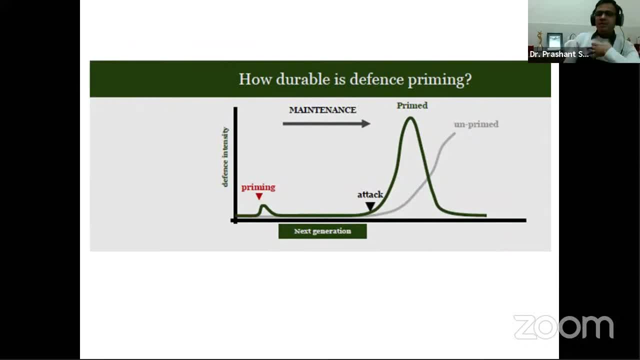 question we asked almost like three years ago in the case of vaccination. if i'm vaccinated, my kid need to be vaccinated again. it will not pass into from one generation to the next generation. so imagine if we need to conserve the certain plant which are endangered and they are very prone to certain diseases. this could be one of the 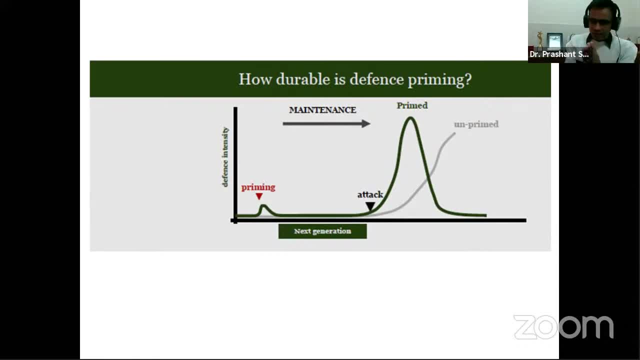 way that we could do this. now the biggest question was that we thought- we thought just now- that the priming is durable. it can maintain within the generation. now the question was that: could it is maintained to the next generation if we have primed the plant, if we collect the seed and if we sow the 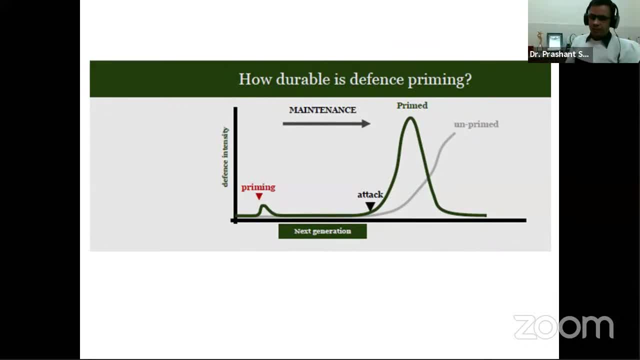 seed in the next generation is still. they are the prime and imagine for the poor farmers if they have their own seed stock of the prime seed stock- and they can, if the seed stock could be also protected in the next generation. that is the real sustainability, that is the profit, that is the social economic equity. 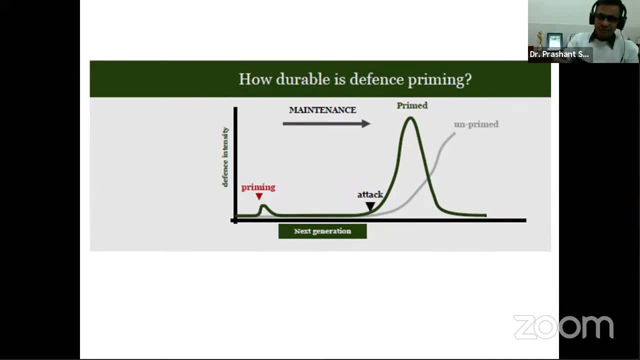 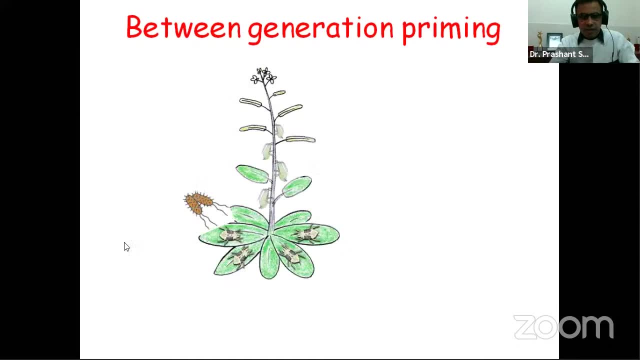 for the poor farmers, and that is the real scenario of sustainability. so what we call that between generation to prime. so see here, this is the plant which is attacked by any kind of the bearing stress. just parental stress increases offspring resistance and we call, as as TGIP, transgenerational. 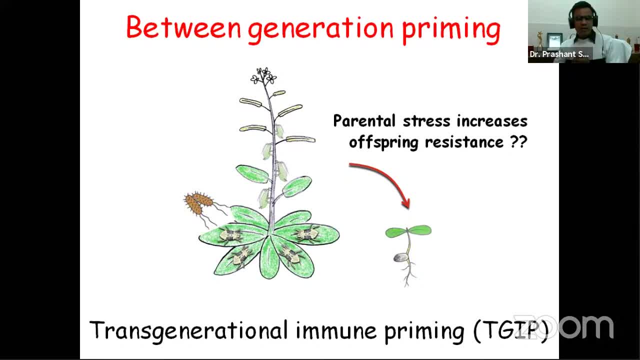 immune prime. it means good priming go to the next generation. so it means if the parent is primed, if you collect the seed, you sow the seed, whether the seed is the prime. so that was the biggest question and you will be surprised that we were happy. we were very happy. the answer is yes, see here. 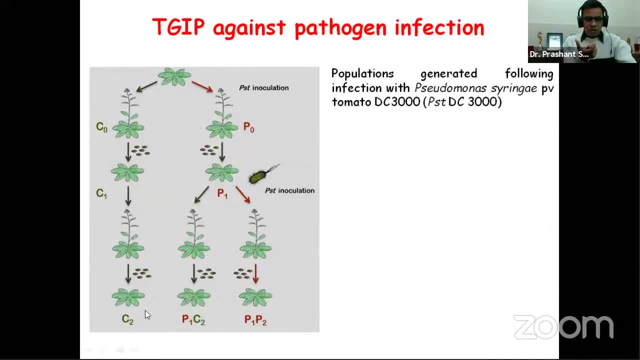 this is the plant, this is the control plant. imagine this is your grandparent, this is you and this is your case. so I'm just giving an example of three generation: grandparent, parent and the kids. in this case, the grandparent was challenged with one of the bacteria that we 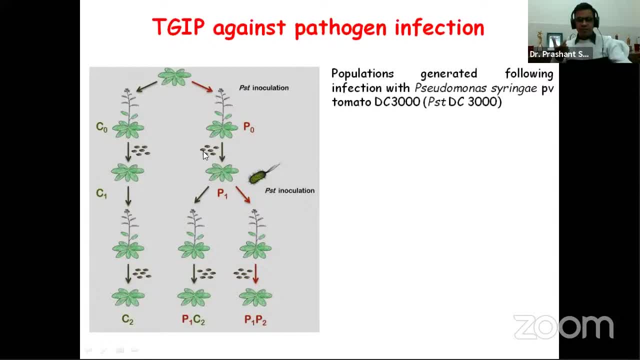 called as Pseudomonas ringe and challenged with this bacteria. and now we collect the seed. and it was primed. and now we have the parent. in the first case, we collect the seed from the parent, which was unchallenged, and then we collect the seed again. that is, the child or the offspring. 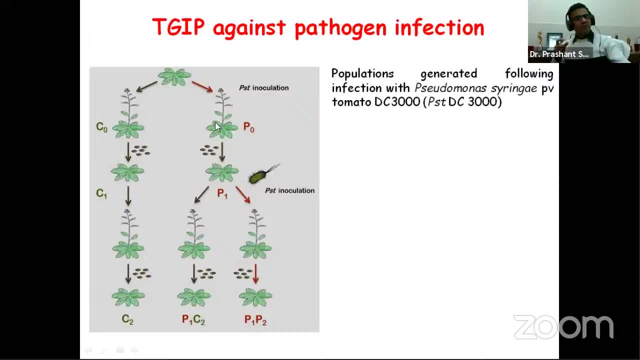 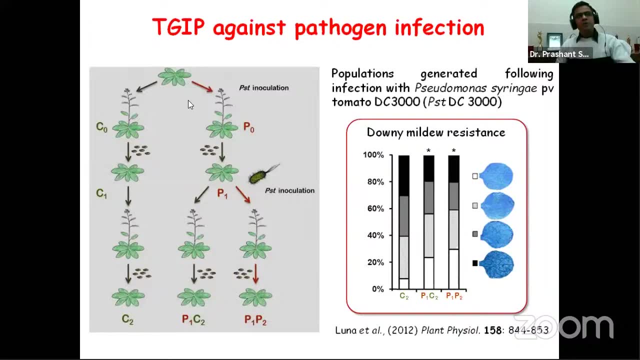 in the second case the grandparent was primed. but again we collect the seed and again we prime the parent. and the beauty is that if simply grandparent is primed, the offspring is primed, so it means you don't need to prime the parent again, and that further suggests this priming can grow into the 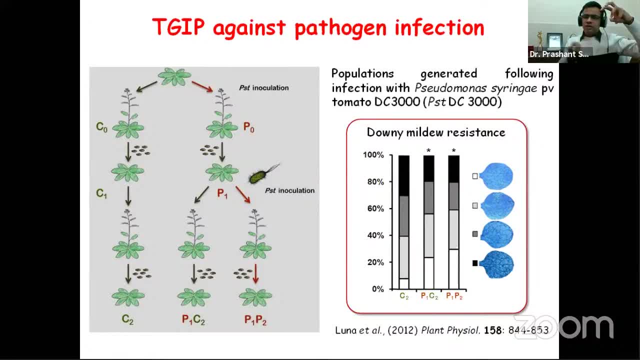 next generation. so if your grandparent is primed, you collect the seed, grow the seed. parent is still priming, is there. collect the seed, grow the seed is still the kids. that is the real, the beauty of this. you know the novel way of this, sustainable the conservation or the agriculture practices and 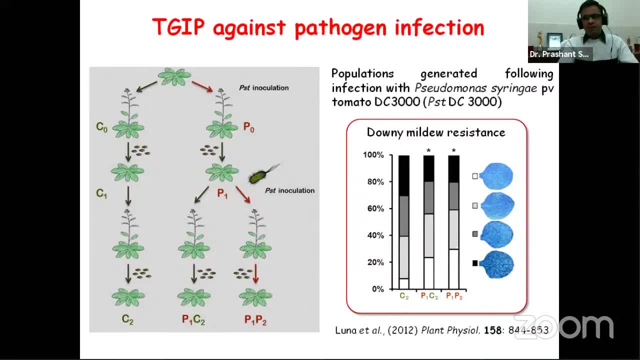 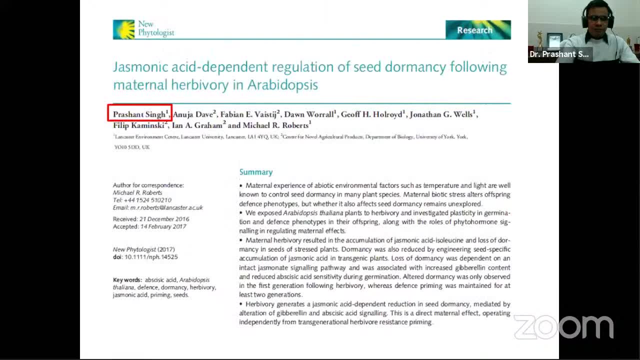 there are a lot of data I can show you, unfortunately because of time constraint, but just to make the story can go to the next generation. there are the few more examples. we have tested number of pathogens with the number of uh elicitors and in all the cases we found just the priming. so I can. 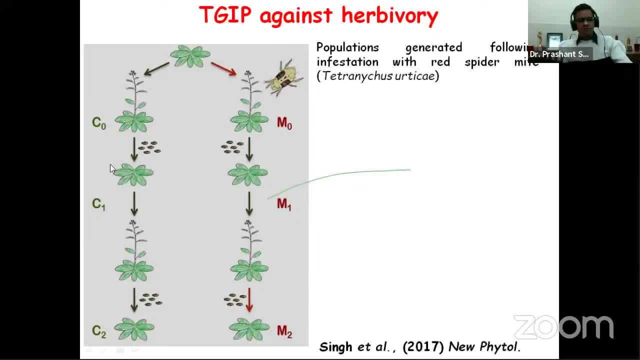 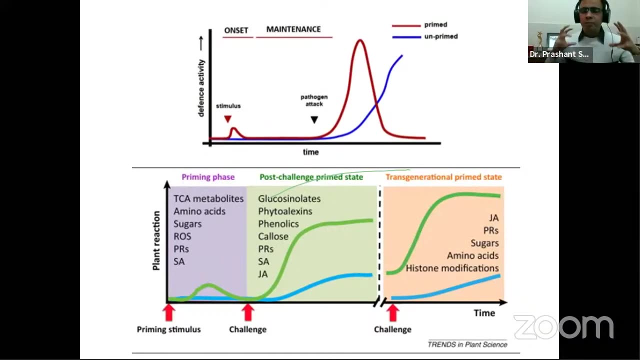 clearly see here. this is some other oxygen and again in the same case, they were super protected, and again, just for foreign knowledge, I can't talk so much. so there is a lot of changes takes place. so there's a big omics: transcriptomics, metabolomics and the proteomics- there's a lot of change. 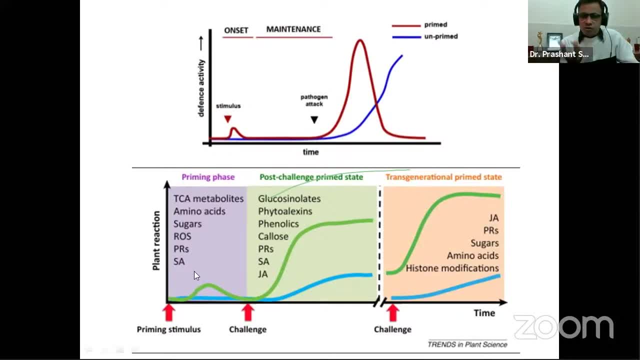 that can give priming stimulus. there's a change in amino acid sugar and the Ross- and they are in the post-challenge prime state- is addition of phenolics. that was the pure and then they are in the transnational primary state again. then there's activation of some uh defense responsive. 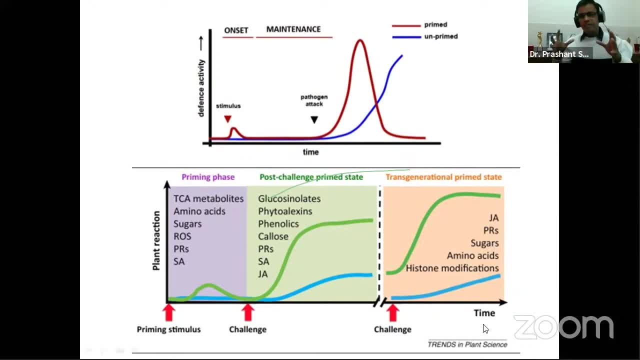 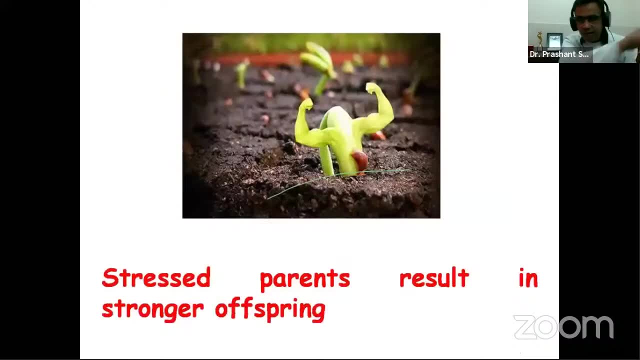 gene or the histone. this is very important. the mechanism of this, the priming, is simply epigenetic. I have two, three more slides and I really love it. if the plant are distressed, the they are resulting the offspring, and it's a very simple analogy. again, imagine your first day. 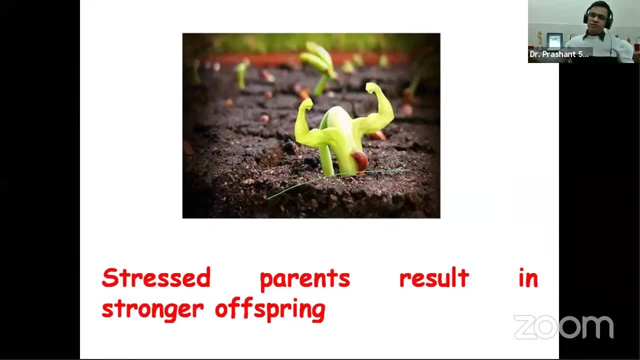 in the class, imagine a night before in the examination. so when a week before in the examination you are a little bit distressed and this stress makes your efficiency stronger and your production is more, you are very good in that. so similarly in the case of the plant: again they have the K time. 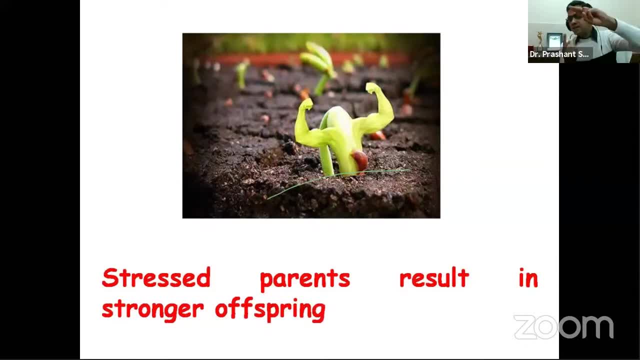 of strength. so now we have picked two point. first, the people. so definitely we can protect the crops and we can feed the billion of people so that that box is thick. so people planet. there is no impact to the environment, there is no detrimental impact to the environmental health, there is no use of. 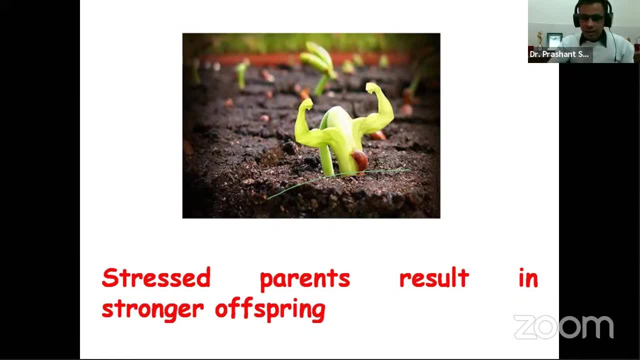 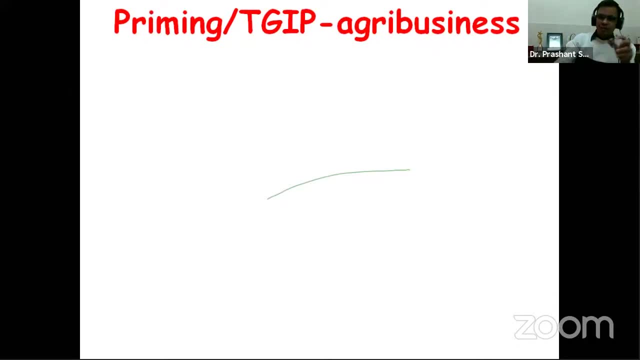 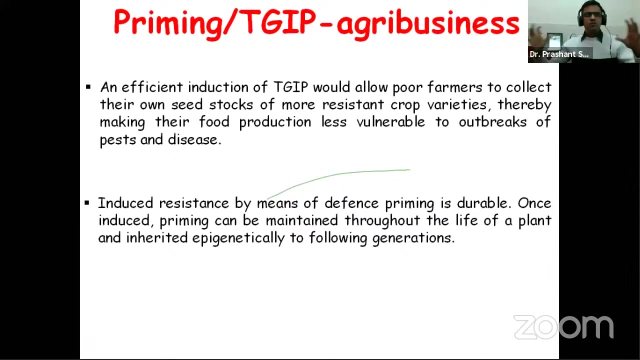 insecticide and the pesticide. now the third point is the perfect indeed, if we include this, the priming is unstable and if patterns are, they can maintain throughout the life of the plant and it can go into the number of generations. and in my debater also, however, do type GIP in this business? I think I have already explained you, because the priming is stable and if this pgat make the farmers, You have your own CD stock and their food production is that will的 elementos. Because of this, they will not be able to produce them into the. There are several kinds of best diseases. Moreover, once it is induced, it is OK, laver, and it will maintain in this business. However, moreover, long-term, 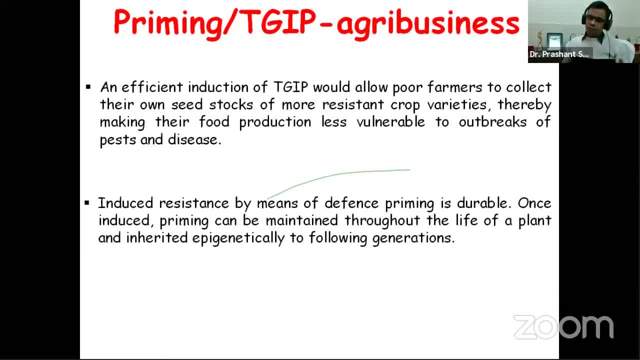 year it is induced. it's durable, it can maintain throughout the life of the plant and it can go into the number of generations and in my river plant, life of the plant and it can go into the number of generations and in myye hand i have tested 10 generation and the plants were primed and the tgip was intact and the plants. 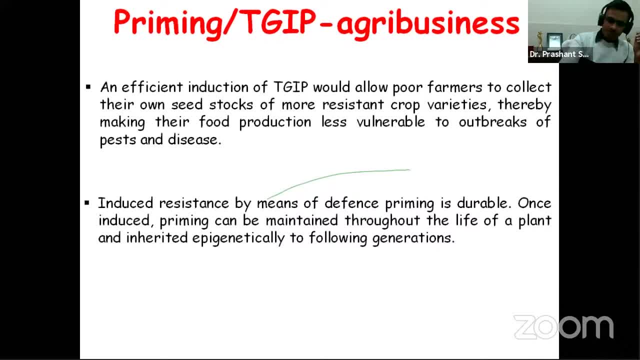 were protected with no yield penalty and again, this is very important. so what i'm saying? that i'm not here preaching that you should not use the insecticide and pesticide. what i'm saying you can minimize. so imagine if you are using one liter of insecticide now. you can use. 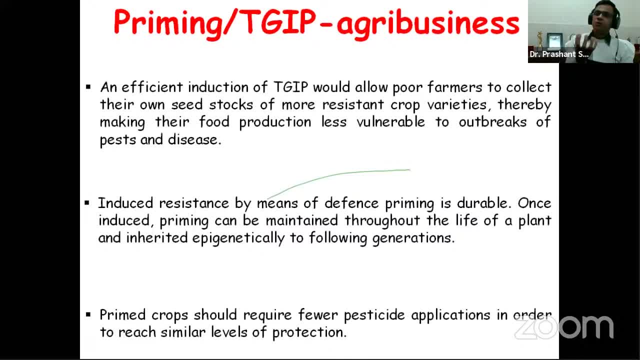 one milliliter of insecticide along with the prime crops and slowly, slowly. if you do this, definitely your environment will be healthy. so again, it could be part of the ipm and you can get the same protection. so we know that there are the different ways. 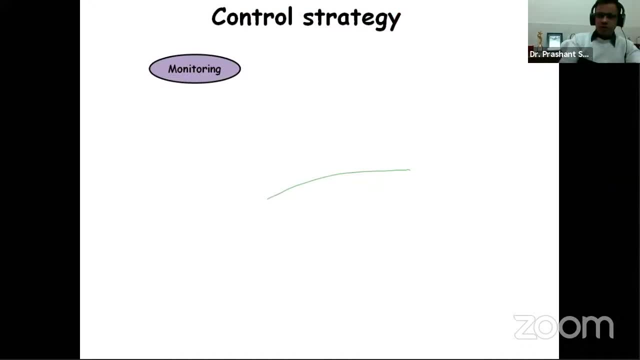 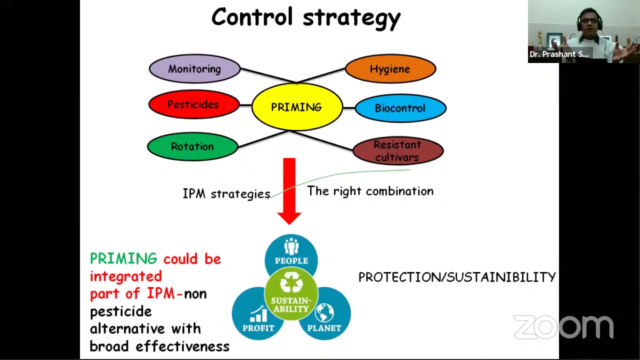 of different strategies for the uh, the crop protection, like the monitoring, pesticide hygiene control. if this guy sits nicely in somewhere here and if we have a very right combination with the prime crops, what will happen? non-alternative, non-pesticide with the broad effectiveness. because if we have the right combination with the prime crops, what will happen? 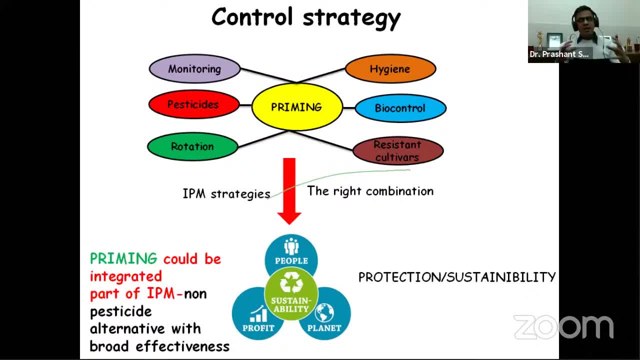 then this could be a non-alternative, non-pesticide with the broad effectiveness, because once the crop is, or the plant is primed, they are protected against various pathogens. simple answer is very simple, because the plant is vigilant. once you are vigilant, it doesn't matter. 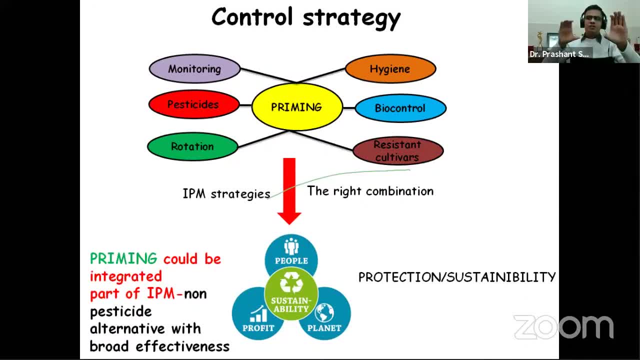 your head is coming, your vice chancellor is coming, anybody is coming, your response will be very quicker in response. so imagine you bring the plant into the long state by bacteria, one particular bacteria. if you are going to face the another bacteria is still. plants are protected. they look very good. they would have to hide it if they want to. 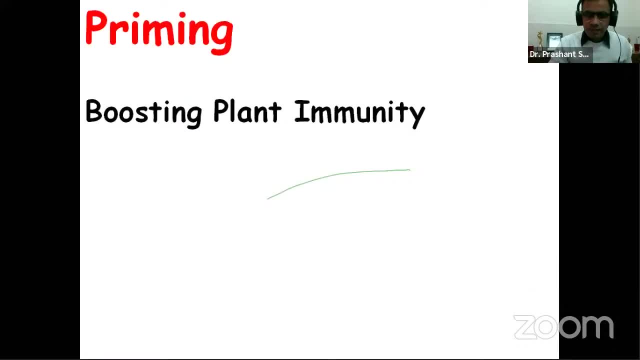 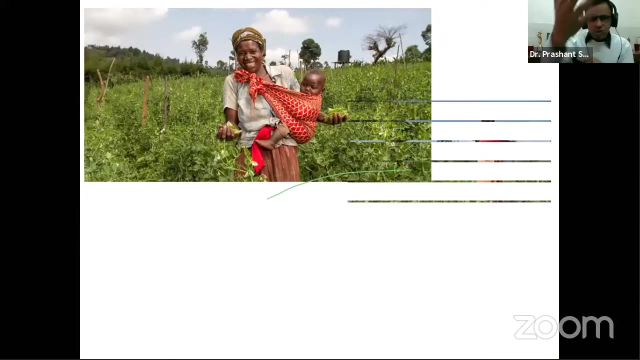 um is so you can't. and you know it's like an action and the plants are protected and the green stands for the plant and, yes, indeed, is the sustainable approach for the crop protection. and that could be also utilized for the, the conservation, the ecosystem, the management, as well as sustainability. and finally, i mean these are. we have a number of the stations. 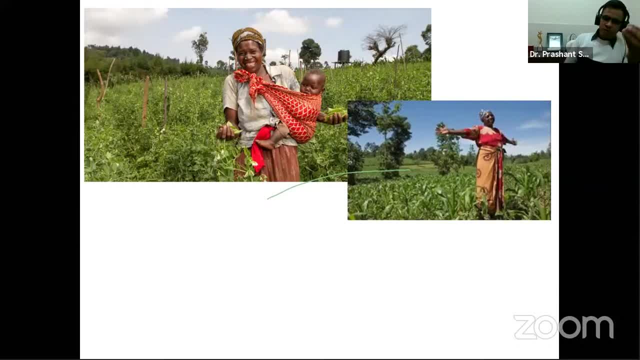 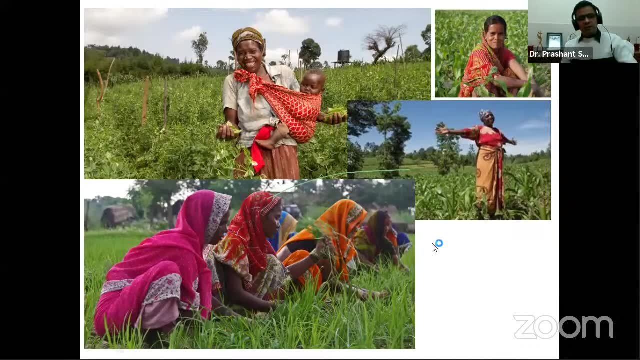 when i was in london it was in edinburgh and some of the stations in the south africa where these the crops were grown, the major you can clearly and you can see here. you know this is my hometown and this is my own field. just for, like a small trial, you know i have used this one in the priming. 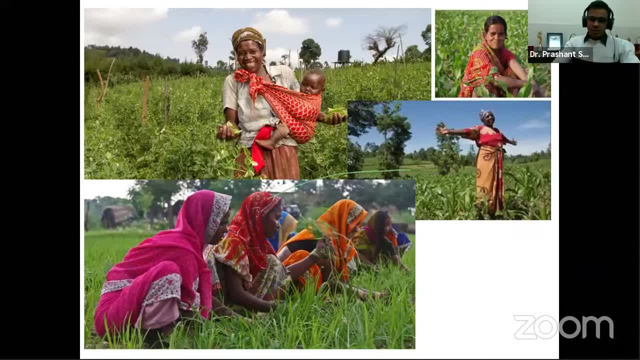 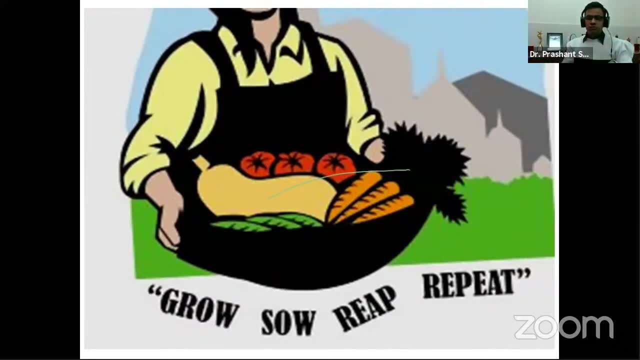 and still we get a very nice impact of these. uh, the priming phenomenon. what is that? grow, sow, reap and repeat. so that is the message here. so, if the plants are the prime, you can grow the seed, you can bring the plant, you can cut the plant, collect the seed and you can repeat into the. 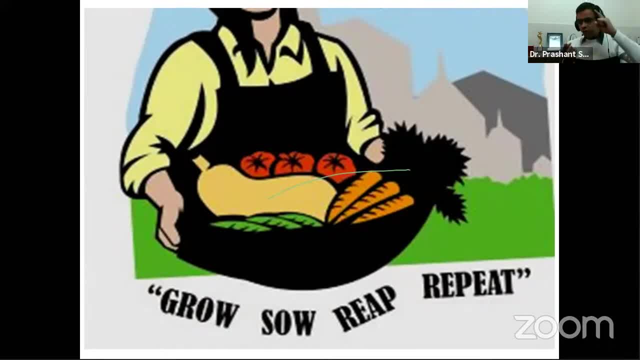 number of generation and there should also increase, because you are not using any transgenic, so there should be no impact to the biodiversity. it still can conserve the biodiversity. there should be no resistant to the different kind of microbes that you want, that we see against the gmos, so still you can bypass these things if the plants are the prime. 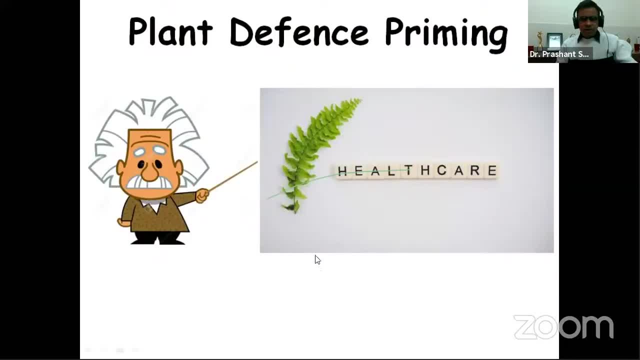 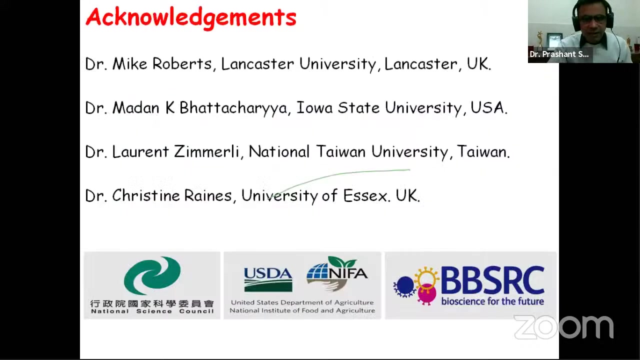 and i like this slide again. so we are talking about this, the health care. so this is the plant, this is the health care. you know that einstein was smart and that's why i say this: the plant defense, priming green vaccination or the tgib as a smart plant, health care and finally, a lot of people. 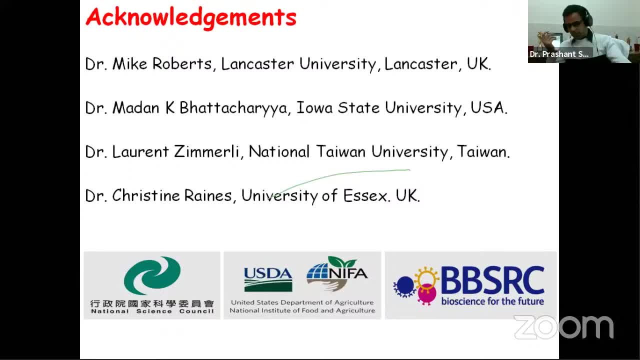 i would like to acknowledge the number of people that are involved in this kind of work and the mike from london, the mother from our state bag in the straits, the lauren generally was in taiwan. the christine was in essex since i moved to bernardo's hindu university in. 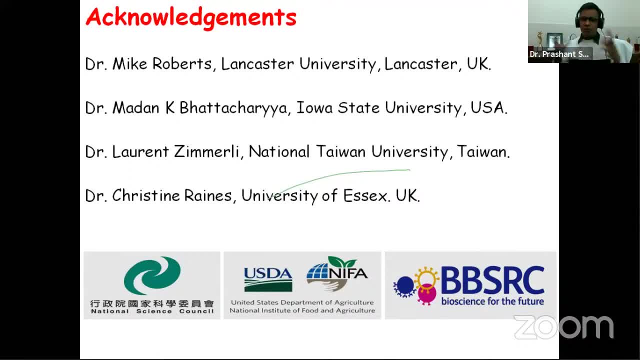 fact, i also worked for a year or so at department of university of ratistan, so i was also there when i moved from london. and these are the different fund agencies back home. here we have the funding from ugc, bsu, in shoot, of ambulance funding and also from dbt and 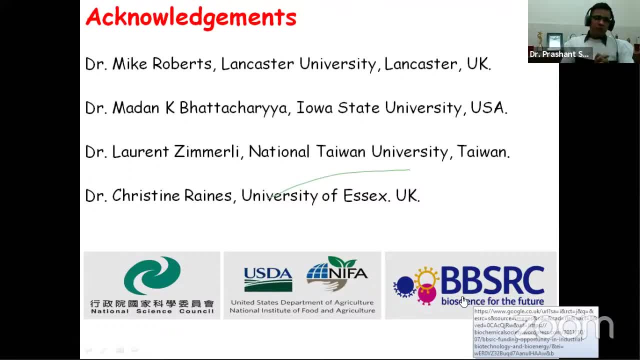 dst to take this work further. so thank you very much for a very lovely listening and thank you again for this organization to giving me an opportunity to talk a bit of my work and to translate my work to the wider audience, and that's the end of my presentation. thank you very much. 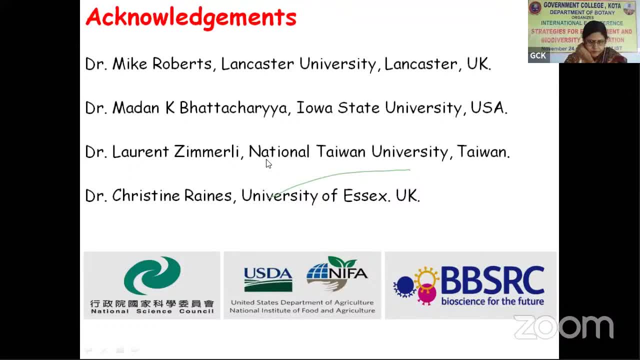 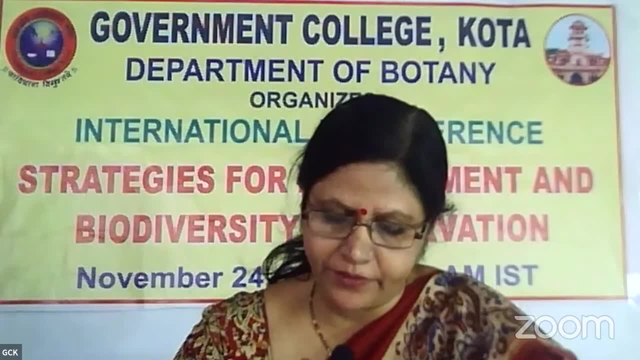 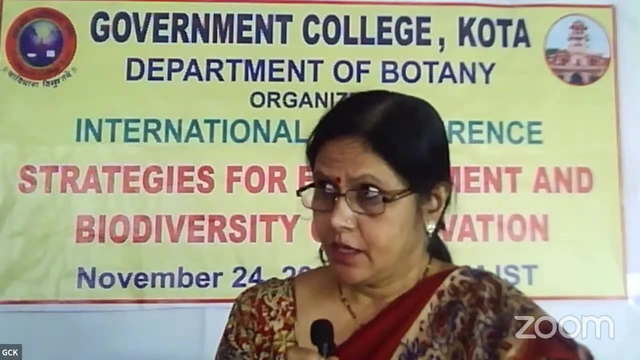 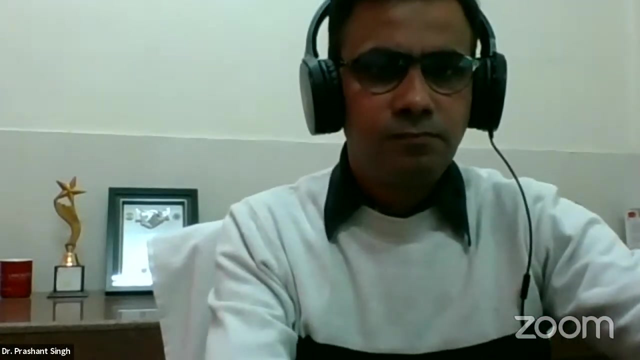 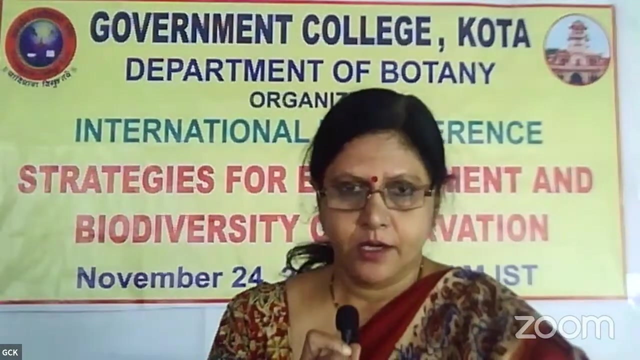 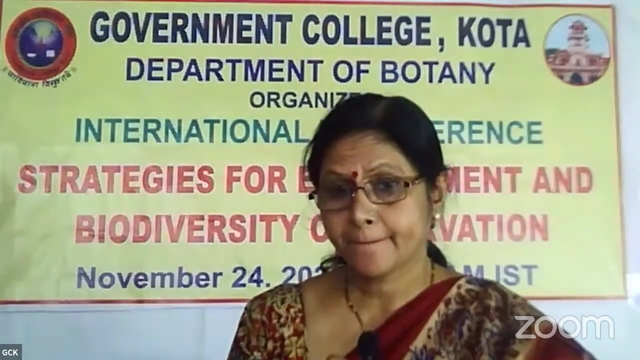 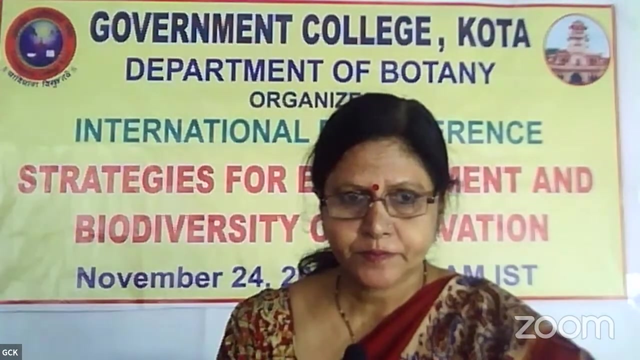 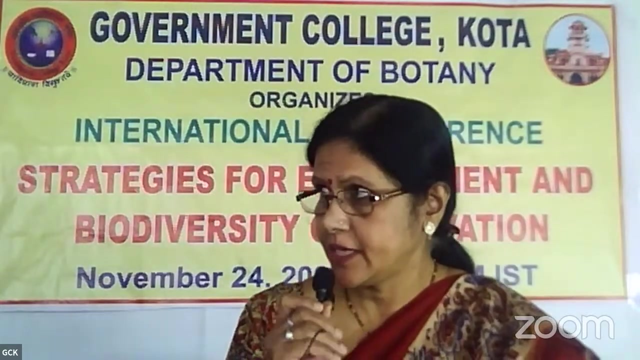 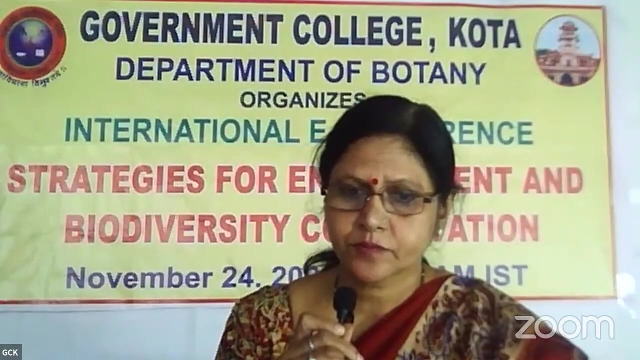 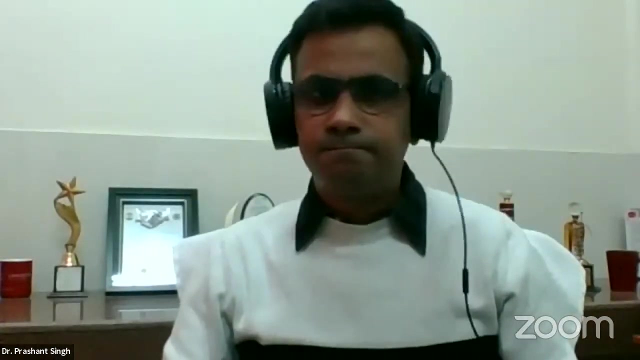 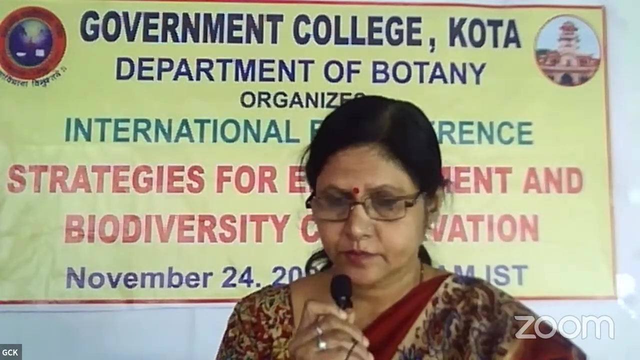 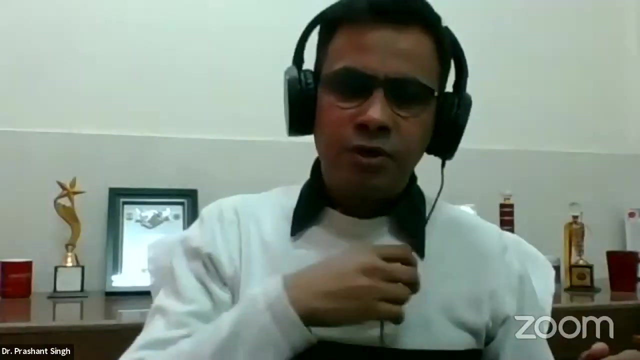 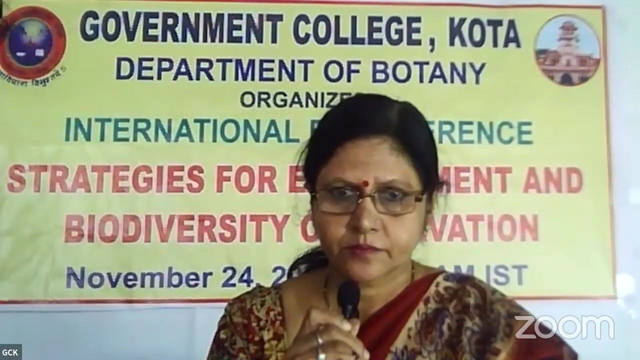 indeed, if there is any question, i would be very happy to answer that. thank you so much. i can't hear hello uh eres do. i'm not sure you can ask other people, but i can't hear you very well. There's a lot of disturbance in the background noise, so I'm not sure where it's. 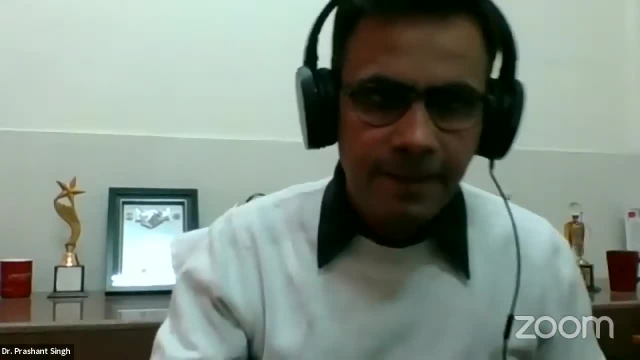 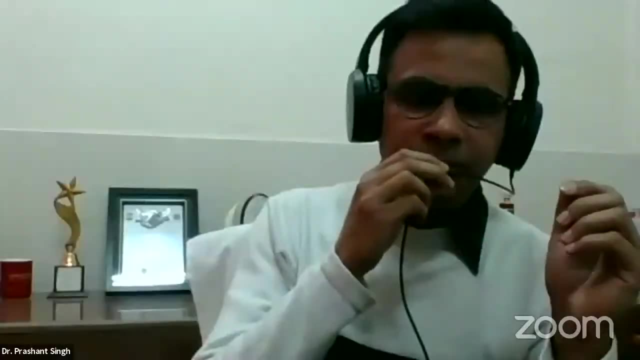 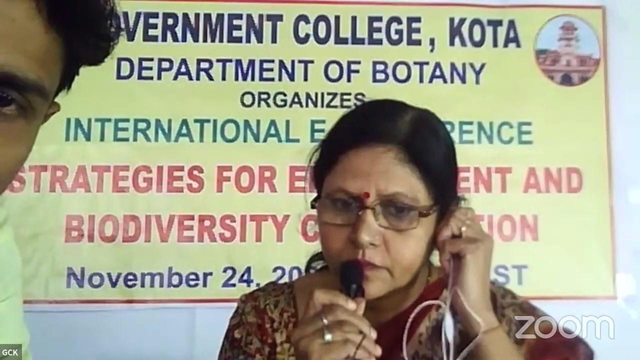 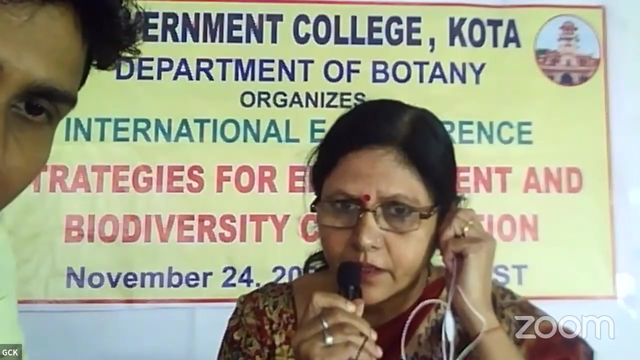 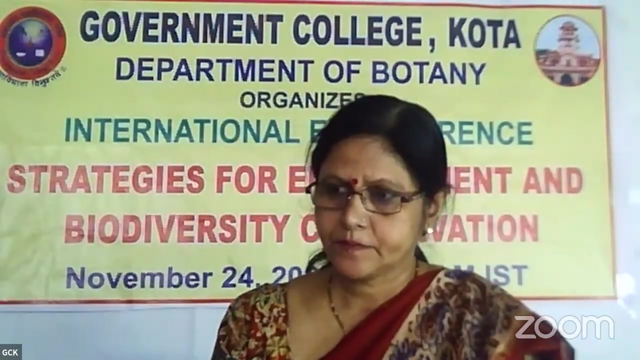 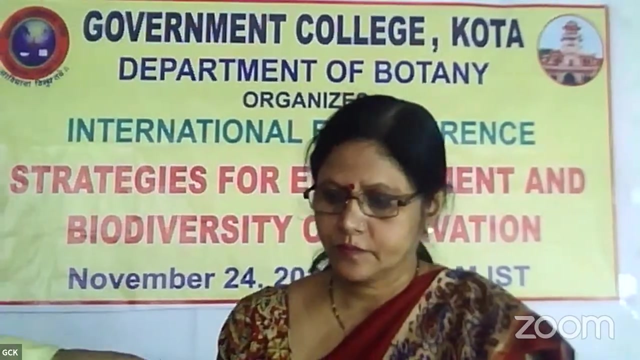 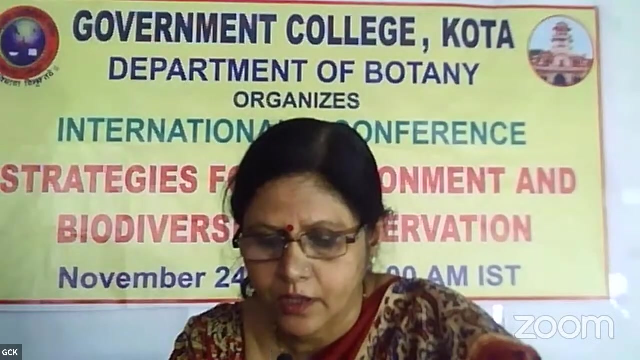 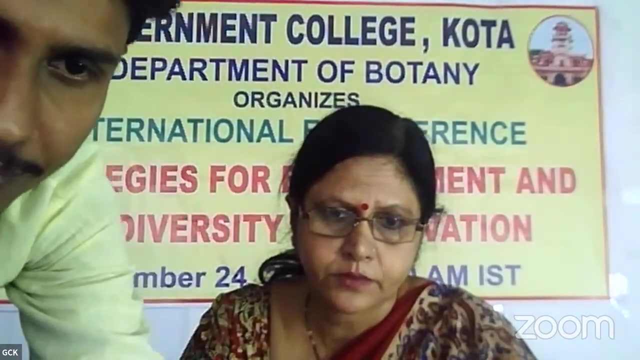 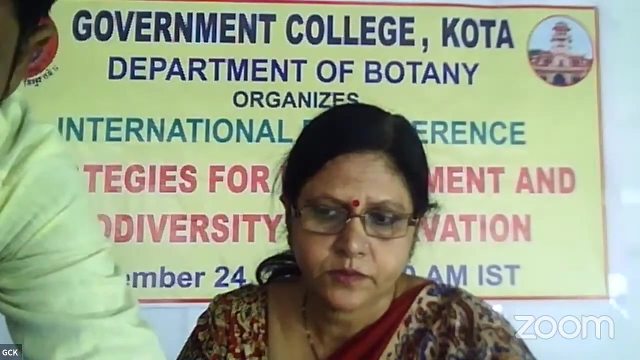 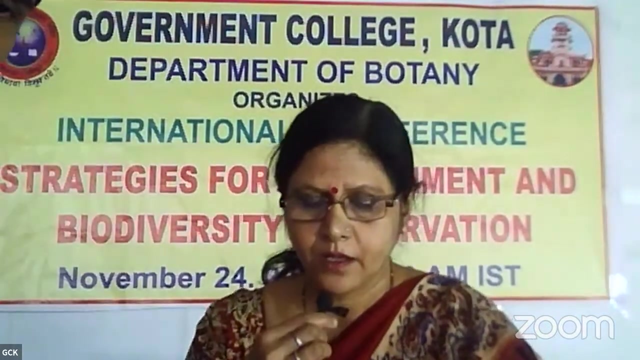 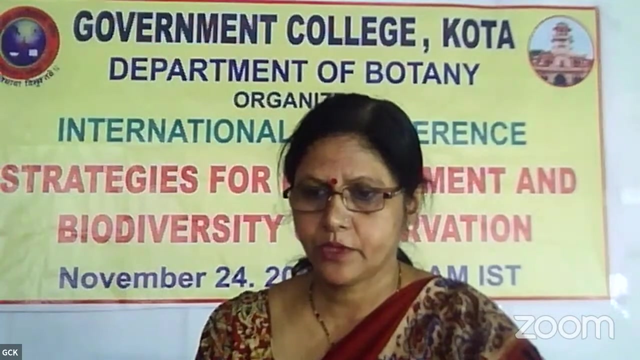 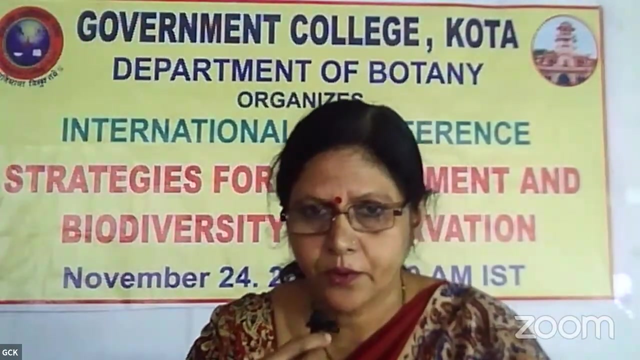 coming from. I can't hear you. Maybe please tell everybody can switch off their mic, because there's a lot of background noise coming. There's a lot of noise coming. There's a lot of noise coming. There's a lot of noise coming. 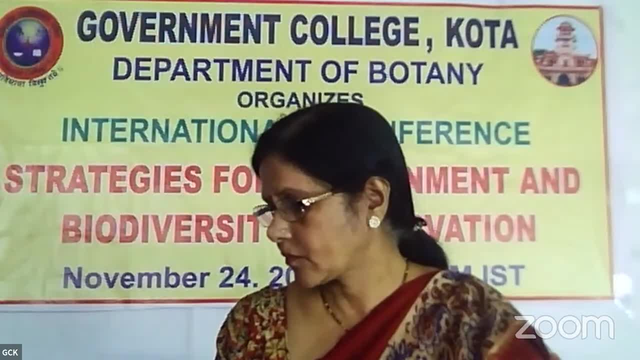 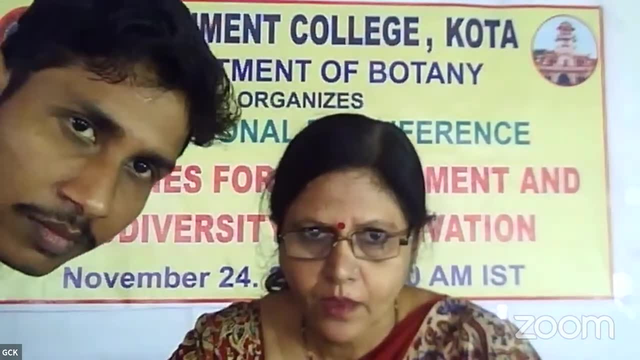 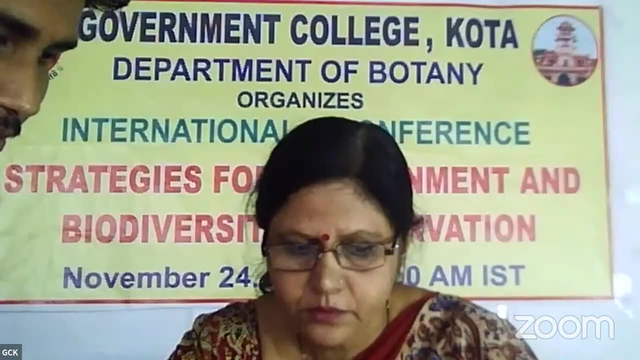 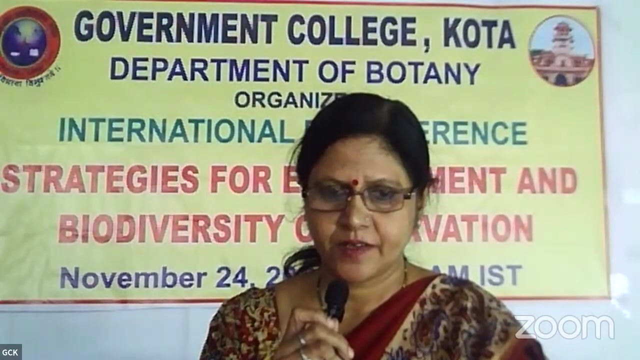 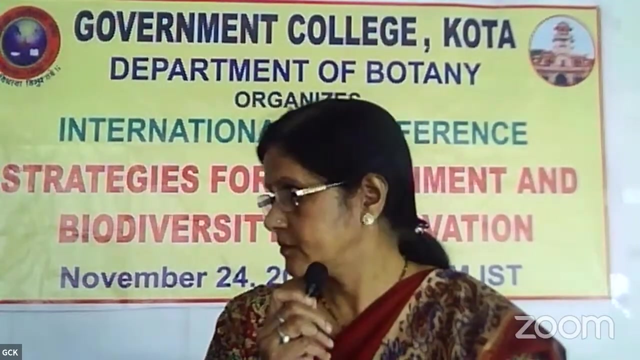 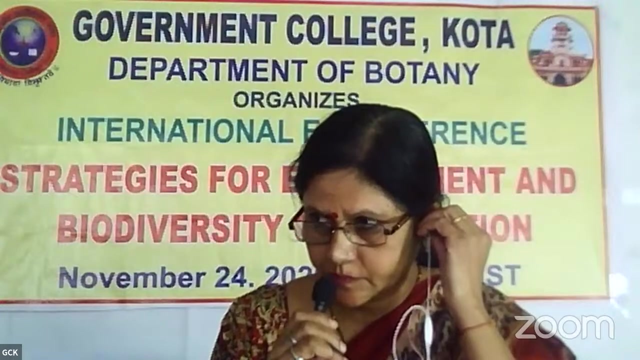 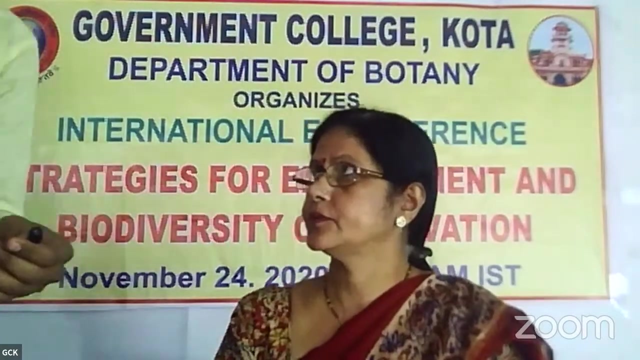 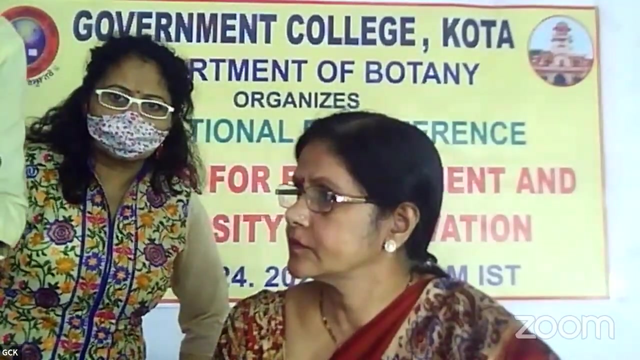 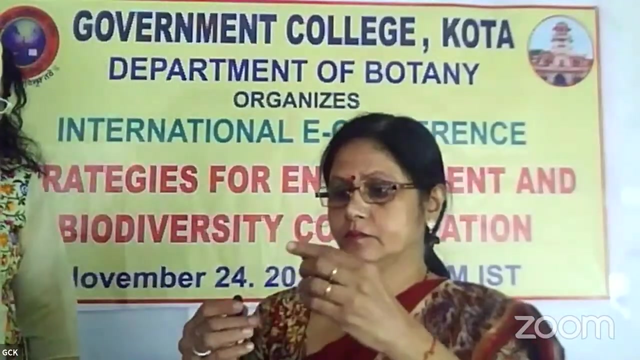 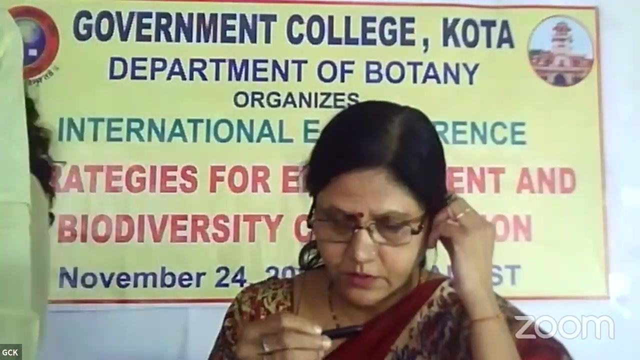 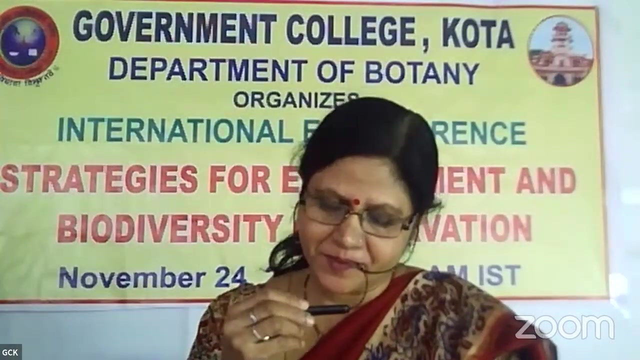 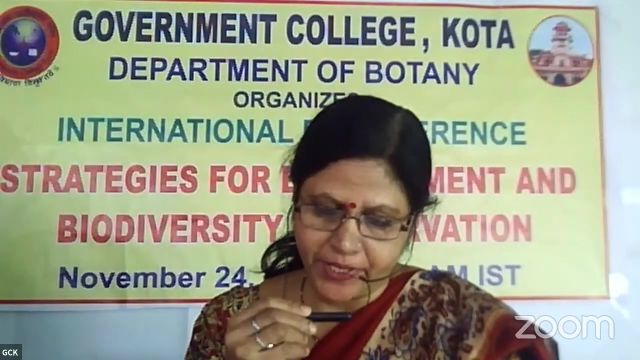 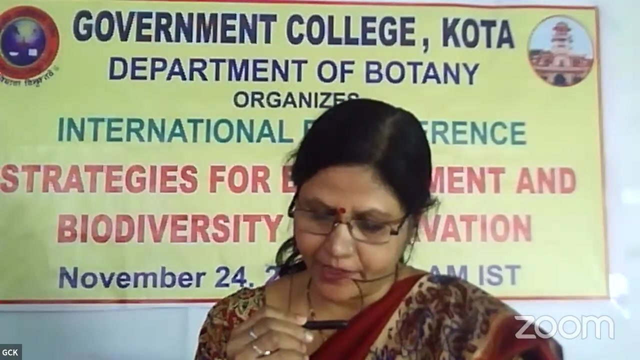 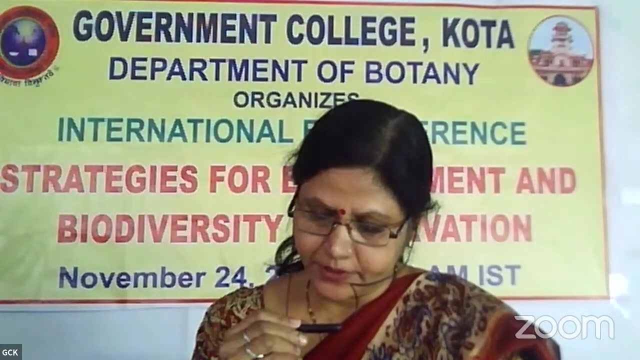 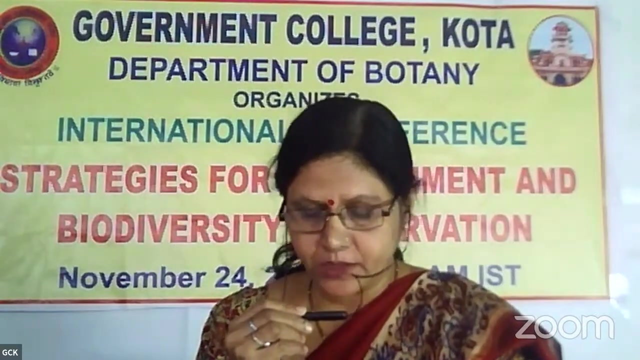 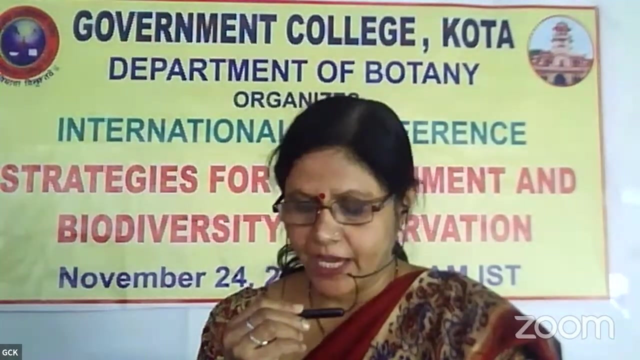 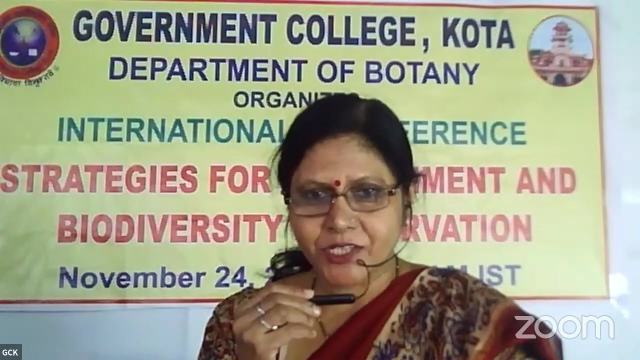 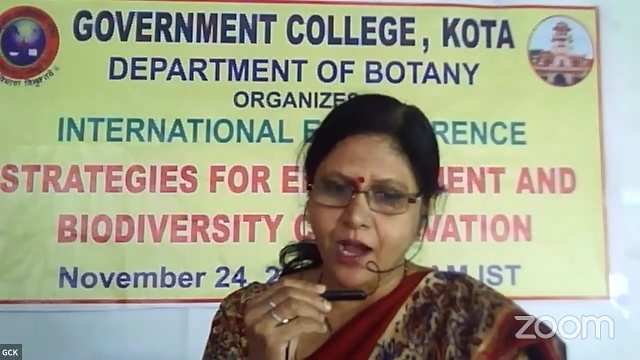 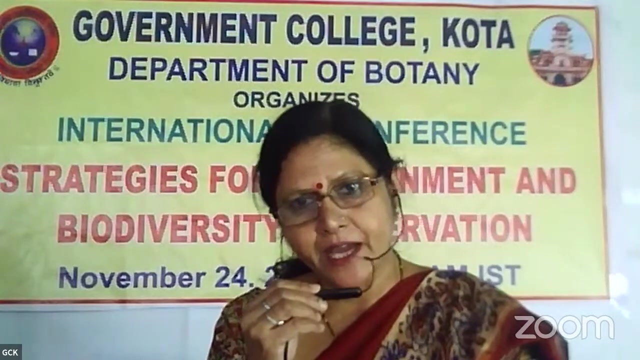 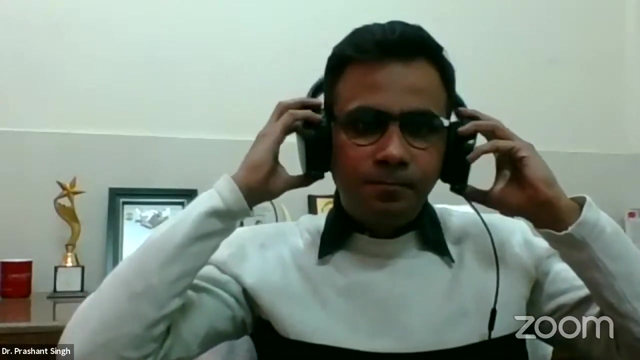 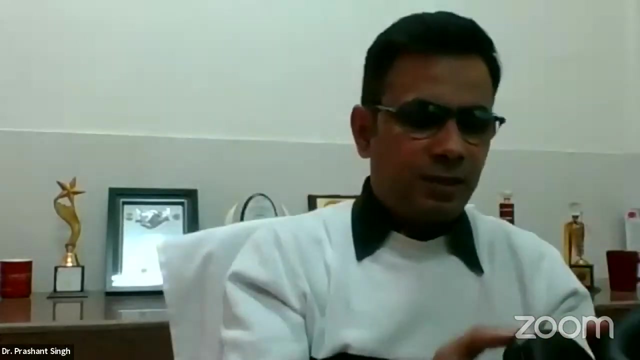 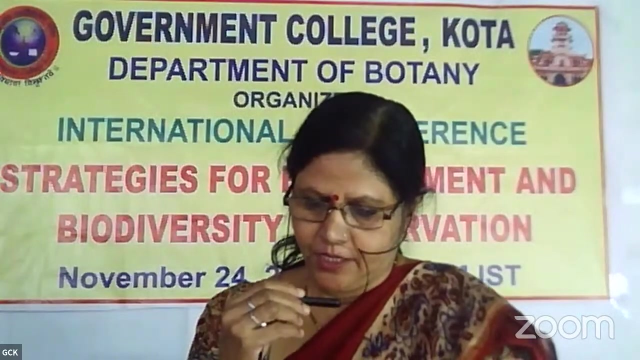 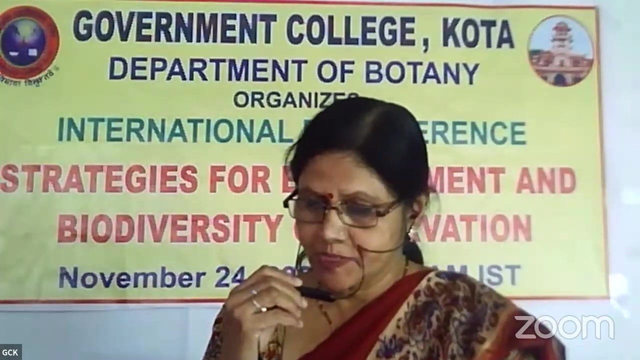 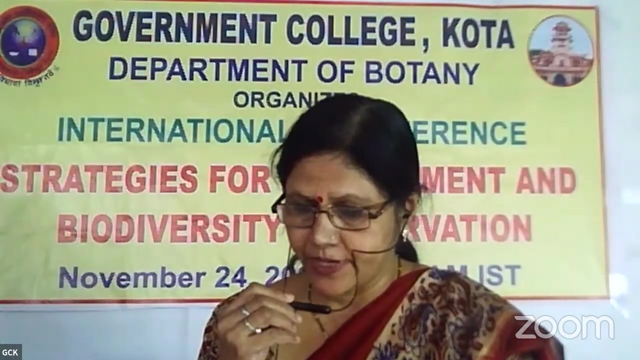 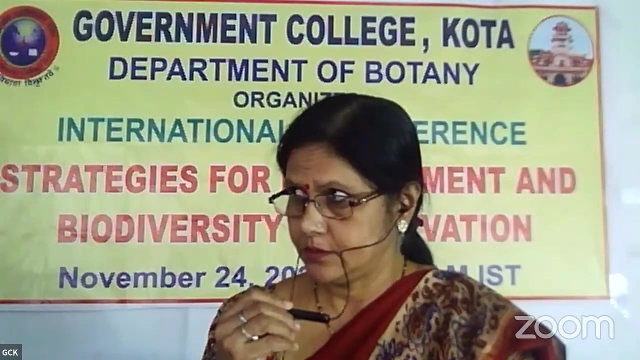 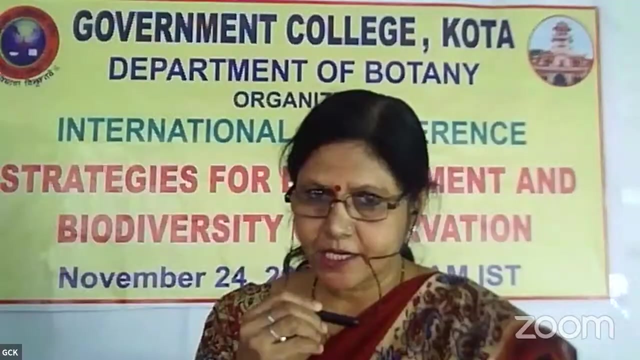 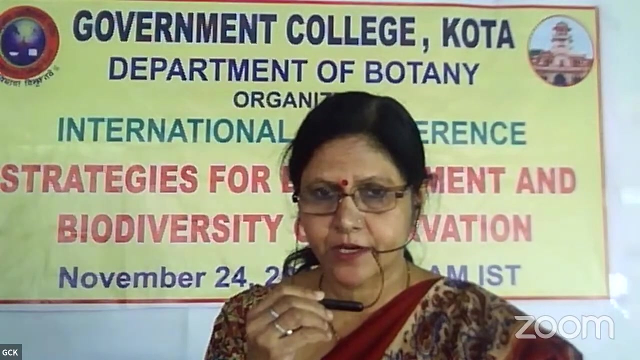 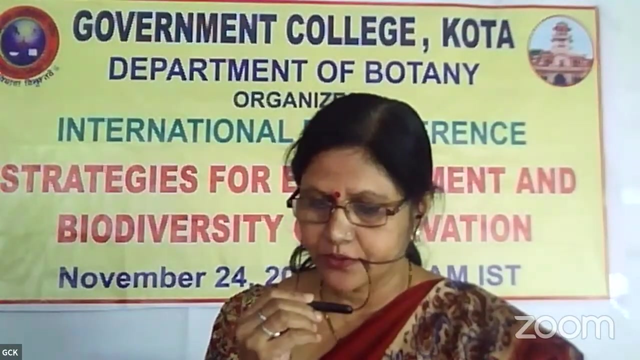 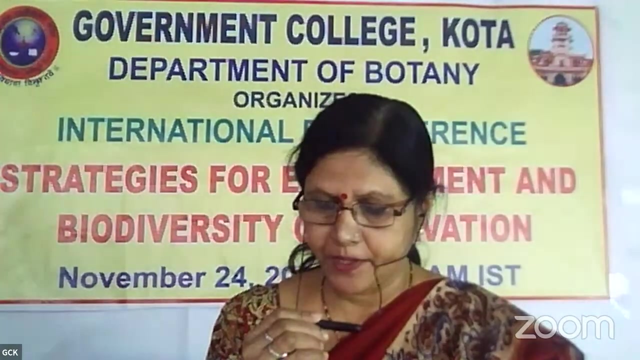 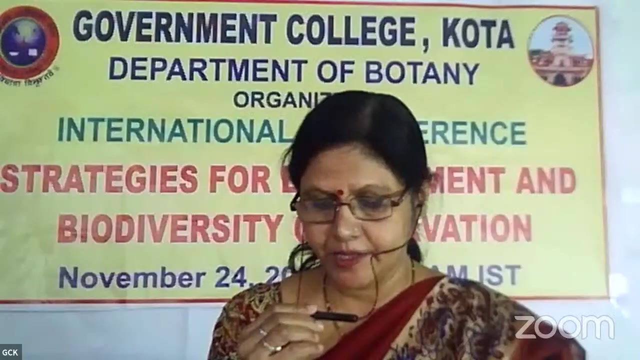 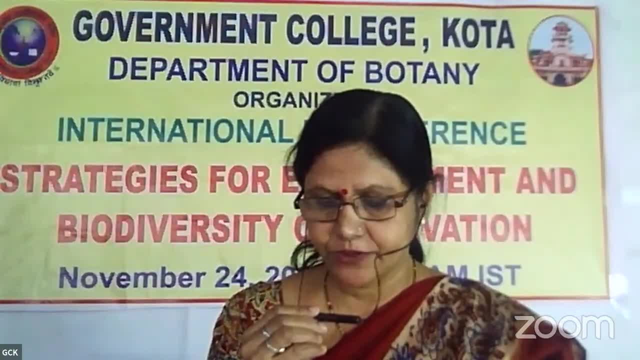 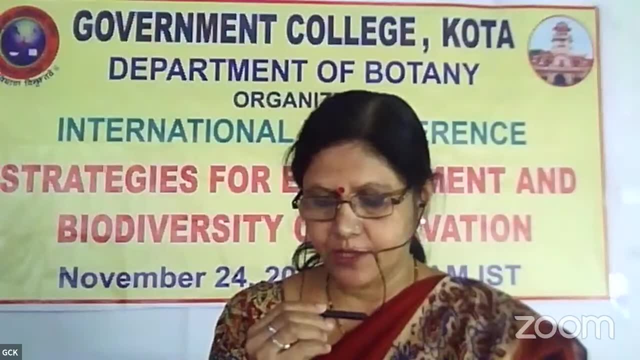 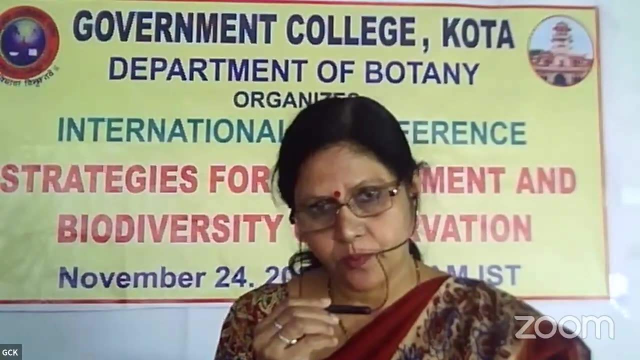 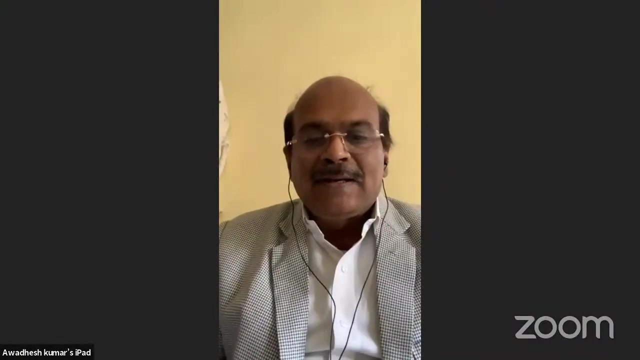 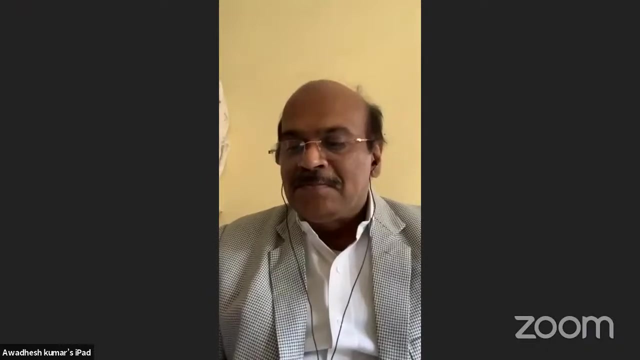 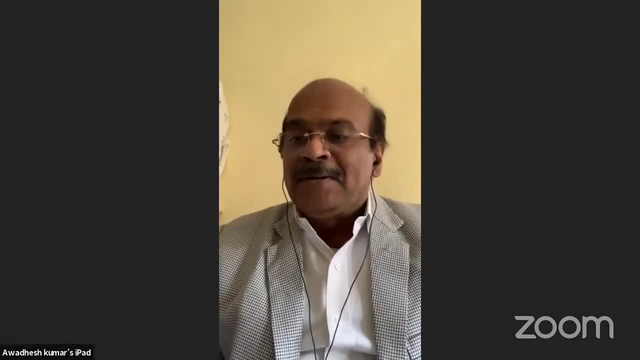 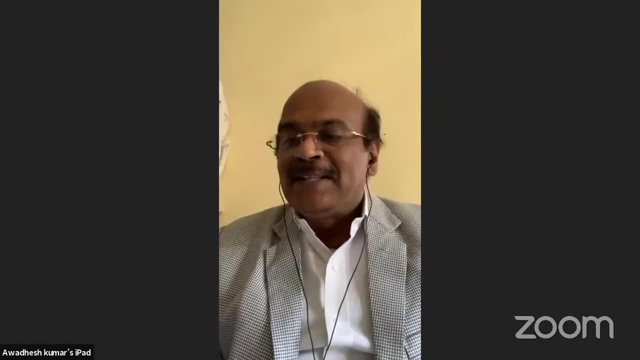 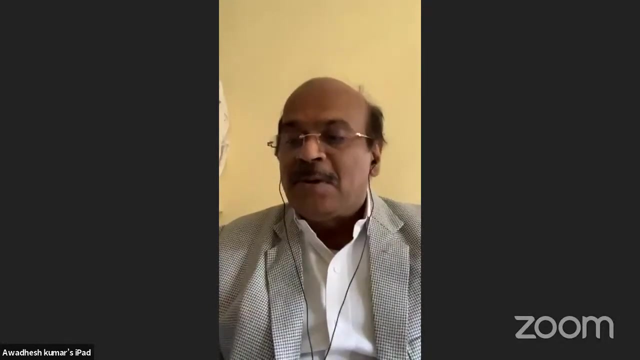 Tomorrow night is going to be so beautiful, It's breaking. That's what I want to talked about. So guidelines, That's what I want to talk about. That's what I've talked about. That's what I've talked about. 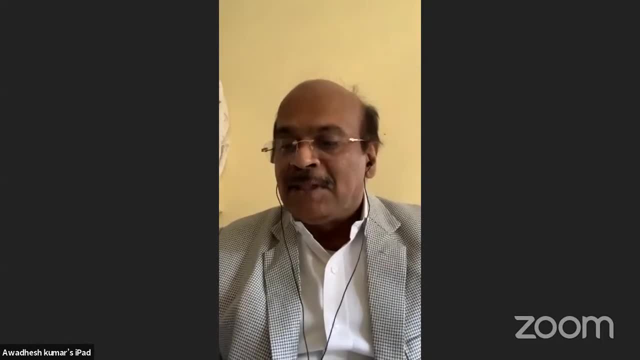 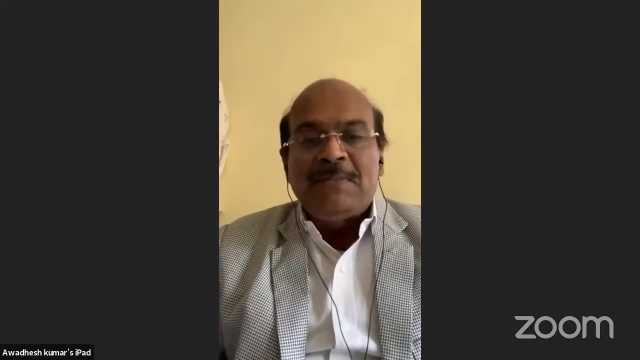 Hope you enjoy. Mirja Srivastava, ma'am, Meera Bhatnagar, ma'am, Hemlata Gupta, ma'am and Raghu Das, who is a special invitee. So, without wasting my time, I'm coming to my presentation. 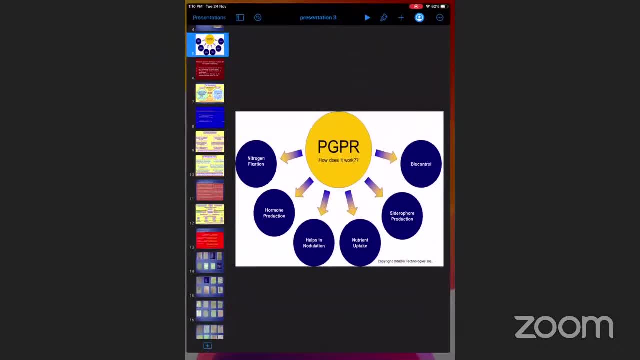 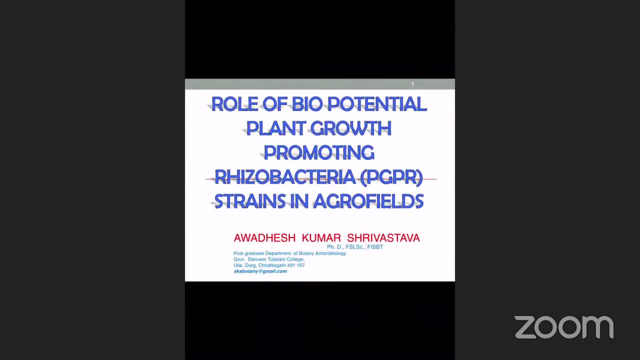 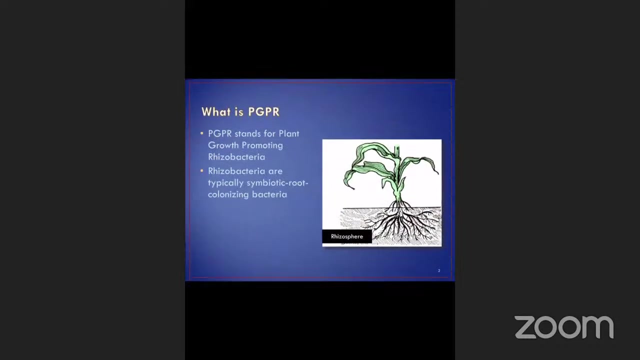 So I have taken my topic as role of biopotential plant growth-promoting rhizobacteria, commonly known as PGPR strains, in agrofield. First question arises: what are PGPRs Actually? PGPR stands for plant growth-promoting rhizobacteria. 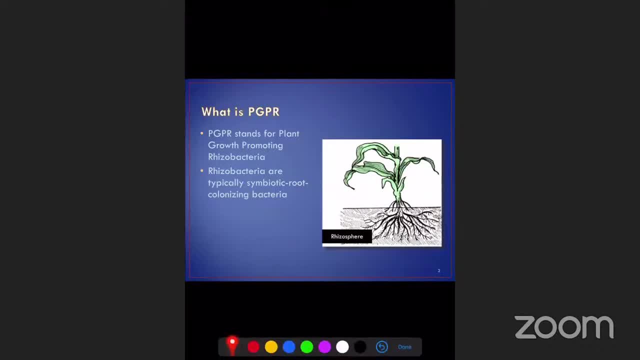 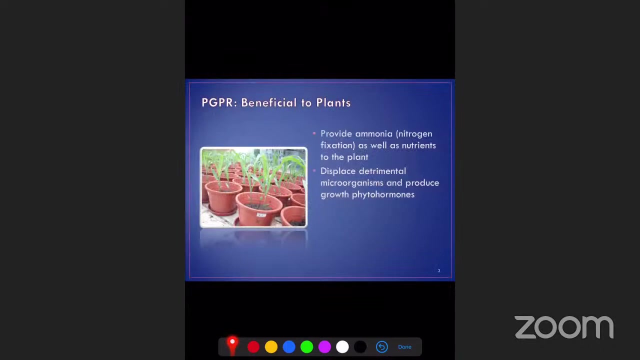 Because whenever you take about this rhizospheric region, this rhizosphere has typically so many types of symbiotic root-colonizing bacteria And the role of PGPR to the plant is they provide ammonia as nitrogen fixture, as a nutrient to the plant And microorganisms. 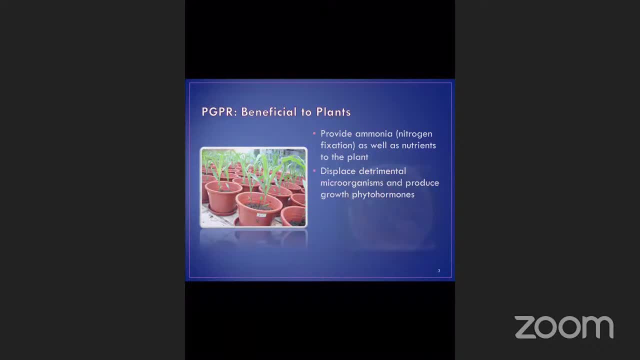 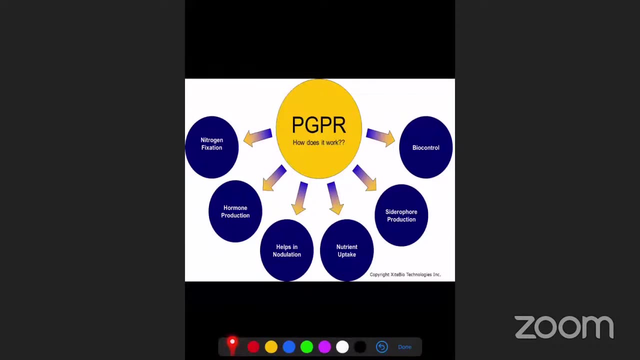 which are also produced so many things within this. So PGPR actually performs nitrogen fixation, hormone production, helps in nodulation, nutrient uptake, cytopherol production and so many types of biocontrol. And how it works. this is our main target to discuss with you. So, first of, 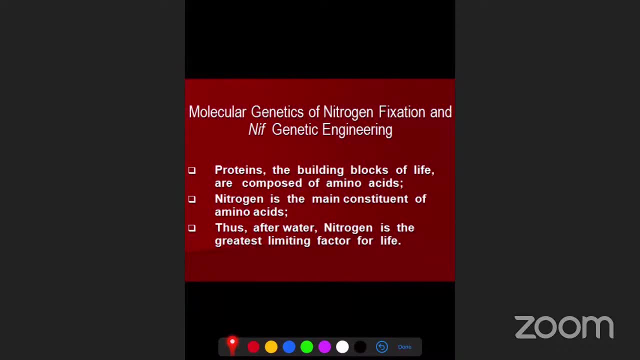 all. I want to give you a little idea about nitrogen fixation. We know that protein is the building block of life and composed of amino acids And in amino acids nitrogen is the main constituents. Because we have heard since morning Dr Deba has told a lot of things about amines and nitrogen metabolism. Even 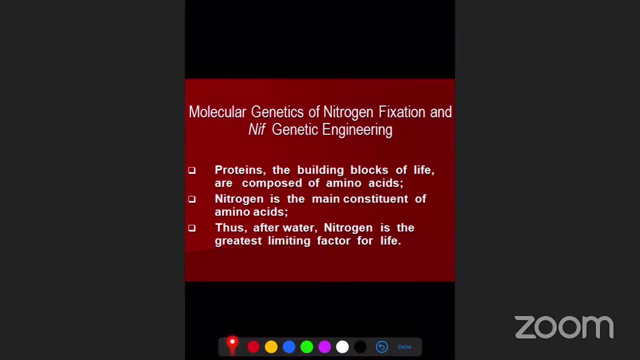 Dr Wad chemicals and потому因为将有 Mlet Dann noch過去. Dr Vargal has also concluded in his part, and above all Mr Vargal has also maintained that we should conserve all the plants. 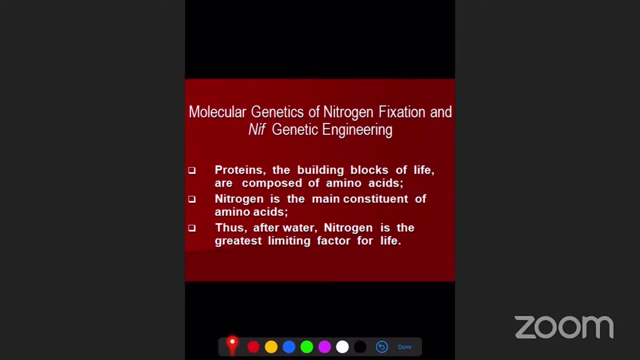 Dr Deba and co also decided to conserve all the plants, and you know that nitrogen is the main cause of life, So we is the main constituent of the amino acid. Thus, after water, nitrogen is considered as the most limiting factor for the life. See, in atmosphere, 0.03% is the only carbon dioxide. 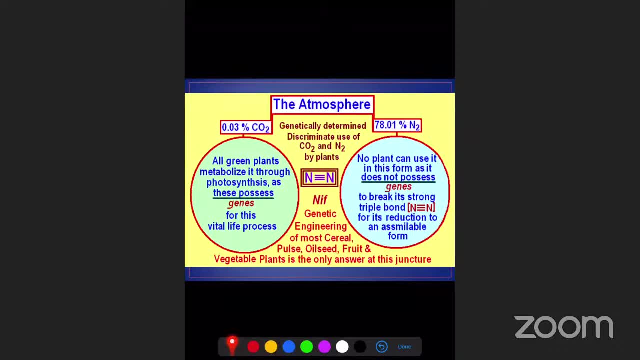 And all green plants, starting from algae, graphite, tetraphite, gymnosperm. if you talk about micro plant as well as macrophytes, everyone has green capacity, that is chlorophyll, and they metabolize it by photosynthesis. And why they go for photosynthesis? Because they have 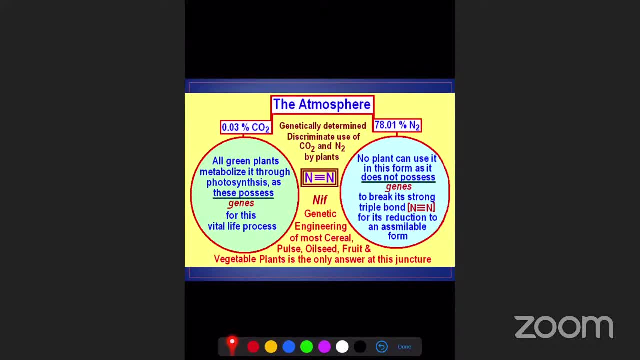 genes for this life process, And we know that most abundant gas in the atmosphere is nitrogen, which constitutes 78.01.. But this is a drawback for the plant as well as all the animals, that no plant can use it in this form, as it does not possess gene which can break the triazide bond. 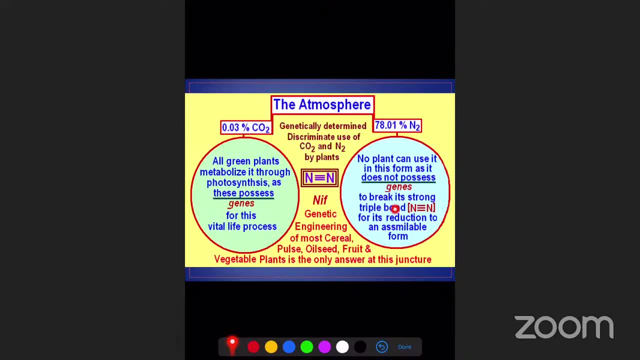 in between two nitrogen, So this strong bond is not easily breakable And because we have no such type of genes and genetically determined discriminated use of carbon dioxide and nitrogen for the plant, So this bond is actually broken by this leaf Nitrogen fixing or genetic engineering of the most cereal, like pearls and seed fruits. 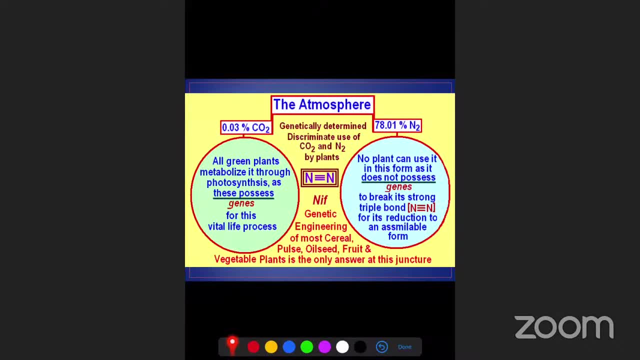 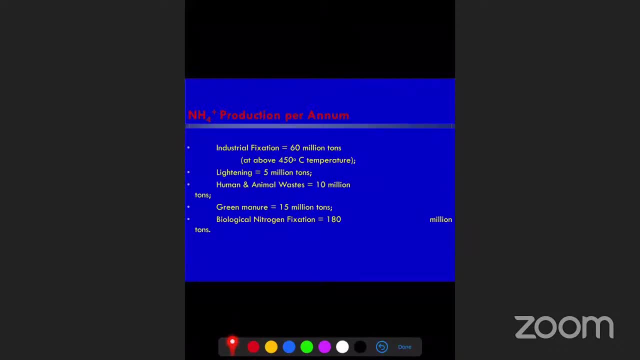 vegetable plants has only answer at this junction. If you talk about fertilizers, we are talking about sustainable development, sustainable farming, sustainable agriculture, sustainable forestry. So, ammonium production per annum. as for the industrial fixation, 60 million churn, which require 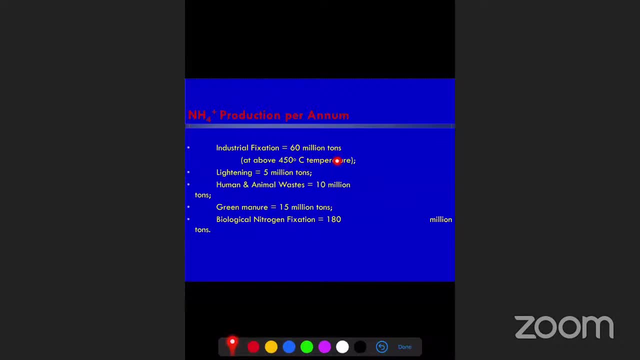 above 400- 150 degrees Celsius temperature By the lighting and thundering of the natural biological fixation. only 5 million tons of the nitrogen is being fixed For animal and human waste products excreta. about 10 million tons of the nitro ammonium is being fixed per year. As for the green 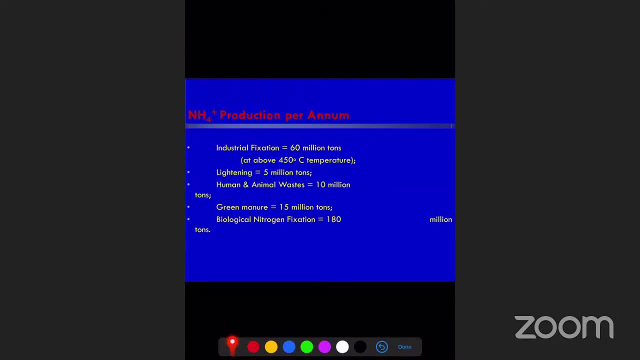 manure is considered, it is 515 million tons And by the biological nitrogen fixation it is about 180.. So from this data it is very clear that only agent is the biological nitrogen fixation. If we talk about synthetic nitrogen fixation, they require up 450 degrees Celsius temperature, which 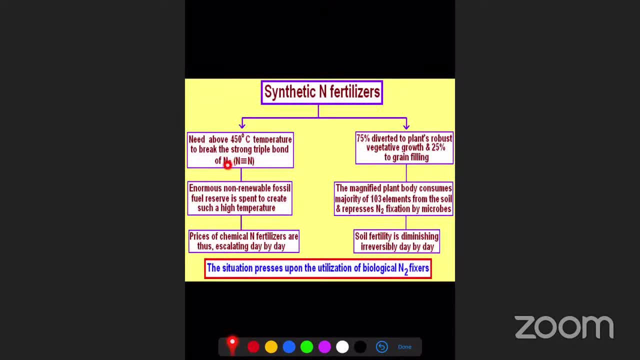 can break this triple as I bond between which is present in diet, your compound, and this needs enormous non-renewable fuel, fossil fuel which have made, which are present in our reserve, and it, If it is expanded, it creates such type of high temperature. 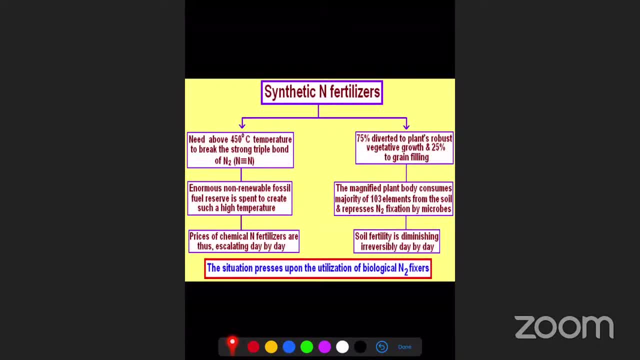 So for providing this high temperature, you also require a lot of energy and a lot of our non-renewable fossil fuel, And simultaneously, in return, we are getting pollution. As for the prices of the chemical nitrogen fertilizers, this way is escalating day by day. 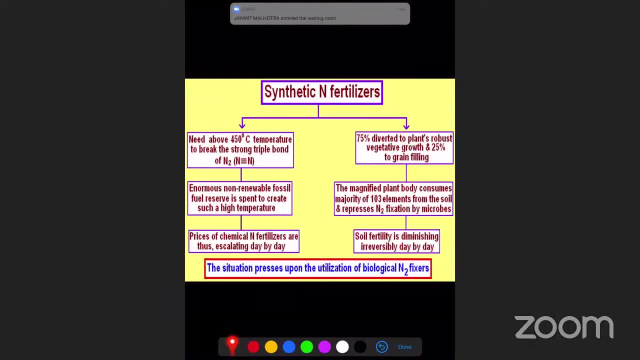 If you think about it, 75% diverted to plant-reduced vegetative growth and 25% is only responsible for grain filling. So 75% of the nitrogen is reboosted for the vegetative growth and only 25% is coming in the form of food grain. 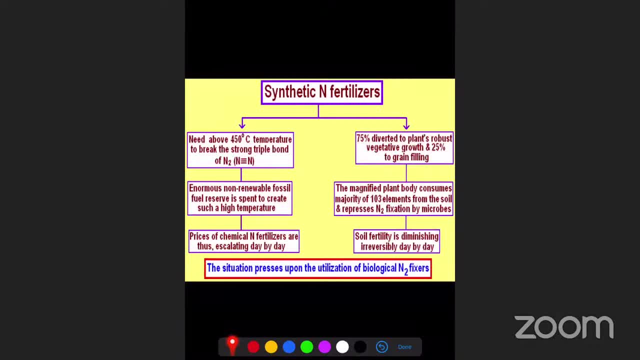 And this magnified plant body consumes majority of 103 elements from the soil And represent nitrogen fixation by the microbe, So soil fertility is also depleting irreversibly day by day. Dr Deba has shown about such drastic changes even in the Himalaya, which is considered as biodiversity reservoir. 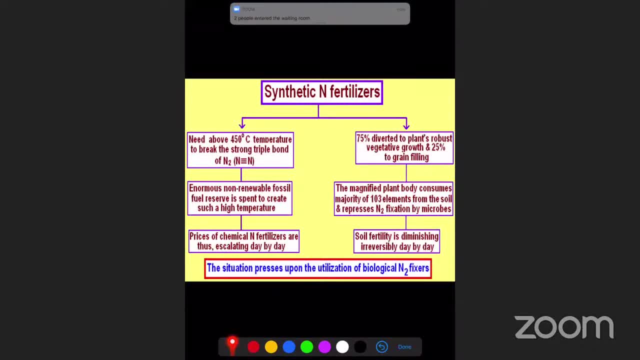 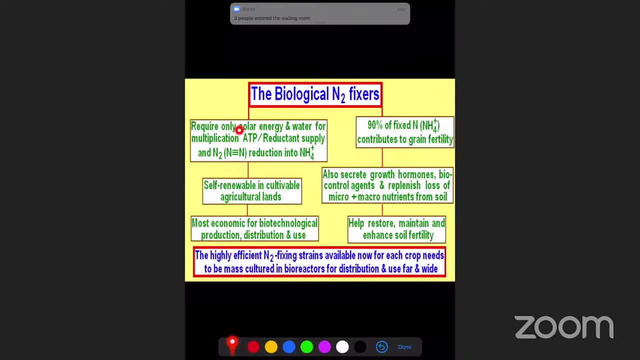 So situation pauses upon utilization of biological nitrogen fixation. As for the biological nitrogen fixation, It requires only solar energy and water for multiplication, that is, ATP and reductant supply. So this nitrogen is reduced into ammonium and this ammonium creates self-renewable in cultivation for the cultivation of the agriculture land. 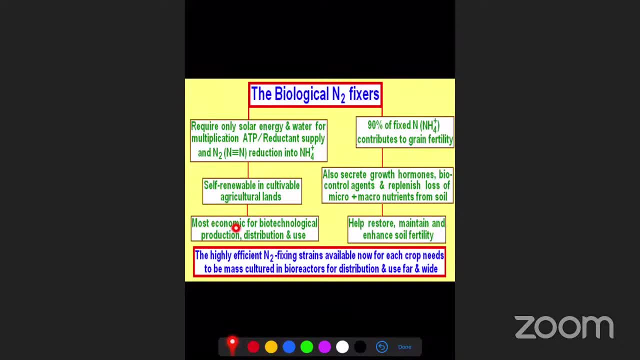 And it is most economic for biotechnological production, distribution and use. As per 90% of the fixed nitrogen contribute to the grain fertility, So it also secretes some growth hormone, which also control bio-agents and replacing loss of micro and macronutrients from the soil. 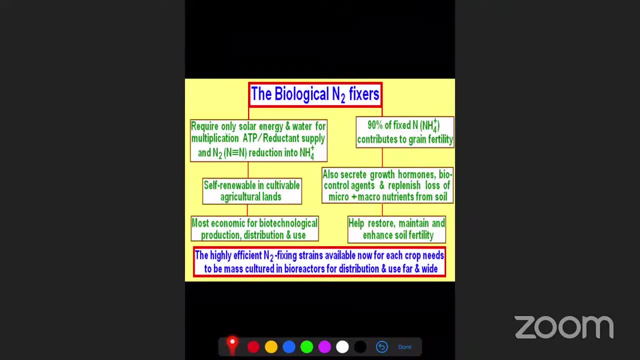 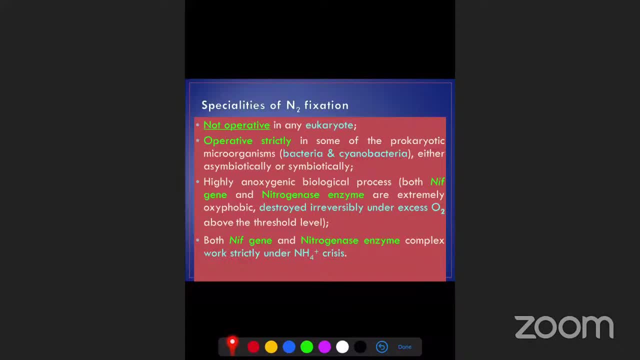 Thus it helps in restoring and maintain and enhance the soil fertility. As for the specialty in the nitrogen fixation is concerned, It is not only the nitrogen fixation. It is not only the nitrogen fixation. It is not operating in any eukaryote. 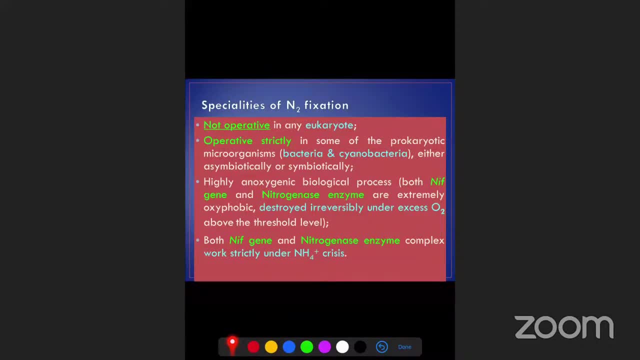 It is operating strictly in prokaryotic microorganism, Few bacteria and almost so many cyanobacteria, Because all cyanobacteria also do not possess this capacity. This is why my work of PhD either is symbiotically or symbiotically. 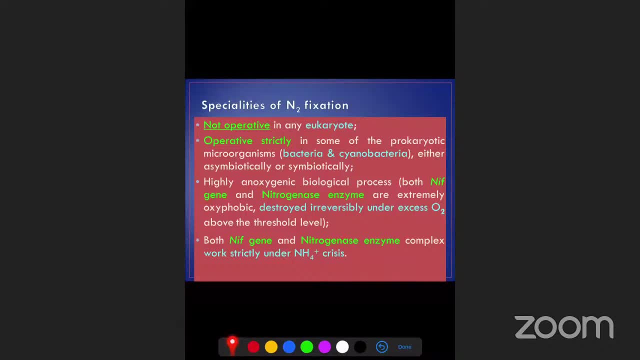 And they have a very good chemistry And they have a very good chemistry And they have a very good chemistry. important type of enzyme which are highly N-oxygenic for this nitrogen fixing gene and nitrogenase gene. They are highly oxyphobic. They're destroyed irreversibly under excess of. 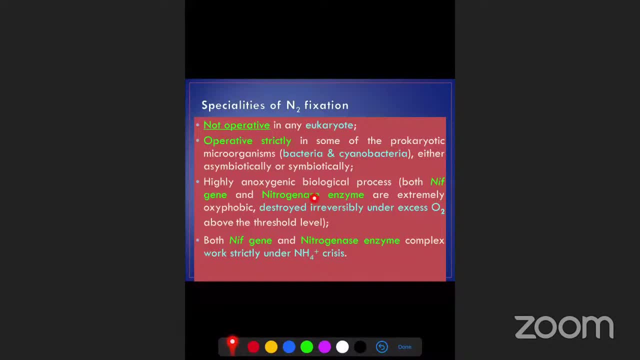 oxygen. So they are present in the type of special packages that is known as leg hemoglobin. So this nitrogen fixing gene and nitrogen enzyme complex work strictly under ammonium crisis Because during this work we have isolated so many strains of the cyanobacteria. 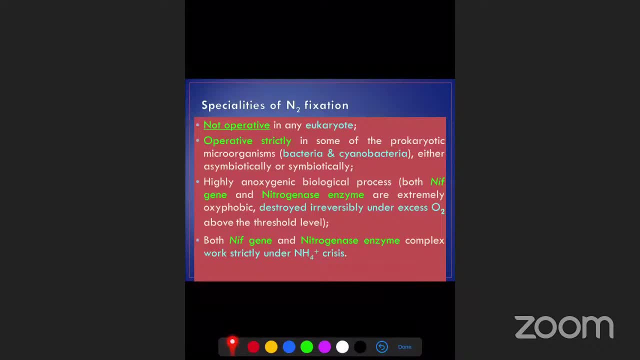 In our nutrient culture. we have provided nitrogen in the form of different nutrients And most of the cyanobacteria will survive. But when we are not given nitrogen as the nutrient, we are not able to provide nitrogen as the nutrient. So this nitrogen fixing gene, 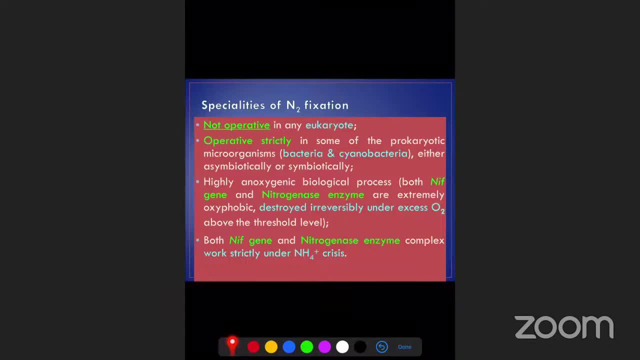 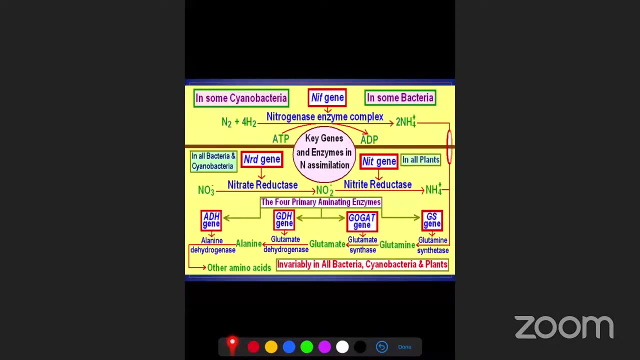 is a nutrient and it fixes that atmospheric nitrogen into nitrogenase compounds. Then we can isolate how they are nitrogen fixing or non-nitrogen fixing. See this: NEF gene is responsible for nitrogenase enzyme complex production. So whenever nitrogen comes in contact with the hydrogen they form ammonium And this is present. These are the key genes and 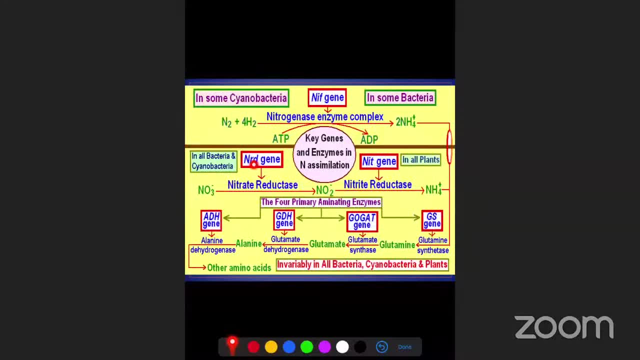 enzymes that are present in the nitrogen. So this is the key genes and enzymes that are present in nitrogen assimilation, because which needs NRD genes and NIT genes And four primary emanating enzyme, that is ADH gene, GDH gene, GOGAT gene, GS gene, and they convert them into glutamine. 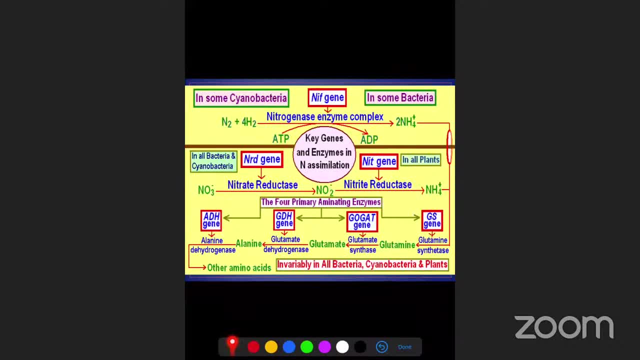 And for conversion of this ammonium into glutamine, glutamine synthetase is required. When glutamine is converted to glutamate, it required glutamine When glutamate is converted to glutamate synthetase. when glutamate is converted to. 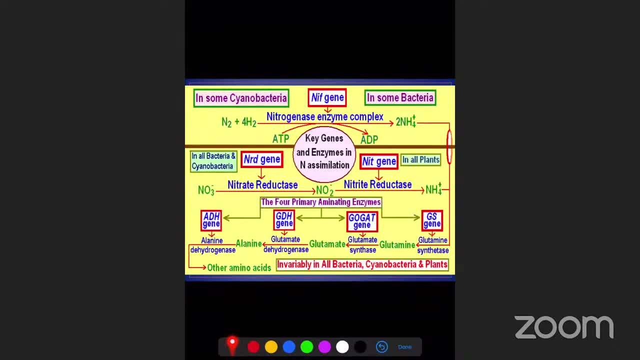 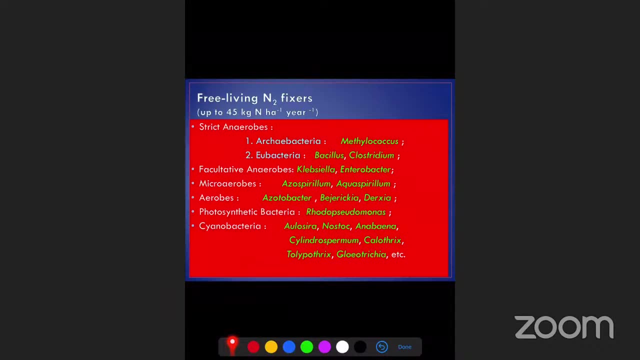 alanine, it is given by glutamate dehydrogenase And when alanine is converted to other amino acid. so this enzyme or this gene is required. So this is about some nitrogen fixing process. And this is a list of strict N-aerob, facultative N-aerob. So these are the 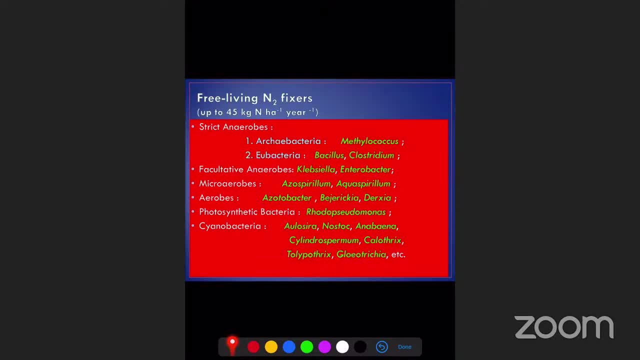 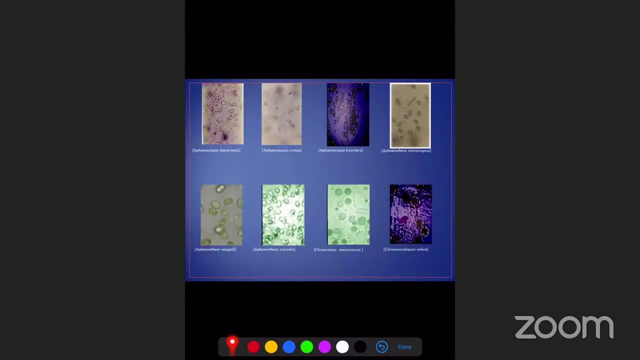 different strains of the cyanobacteria which we have collected from the agrofield, of the agrofield, as well as some pasture land and ponds of different area of the Blaspur which is present in Chhattisgarh And simultaneously our team has worked throughout the Chhattisgarh And FNO CAPs. 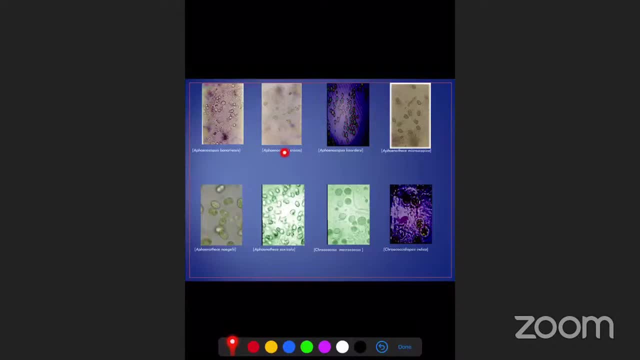 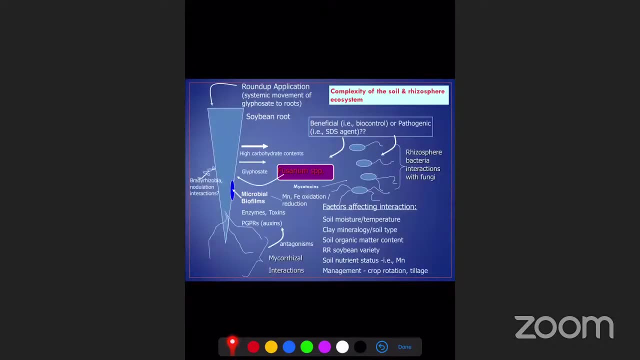 they have different varieties. So these are the different cyanobacteria strains which we have collected from the different fields And by the process of isolation, pouring, plating and sootane media and B11 media they were, are considered for their growth And if you think about this rhizospheric ecosystem, this 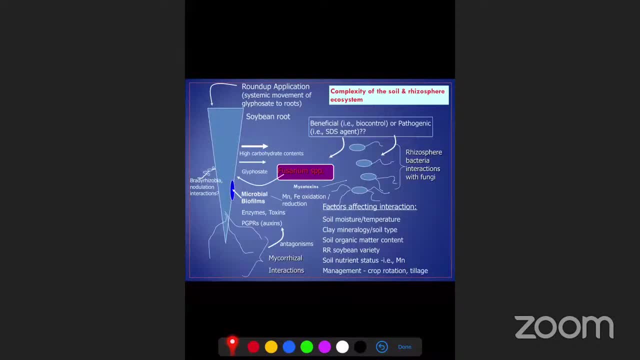 is very wonderful because if we think about this roundup application of systemic movement of glyphosate to the root- suppose this is soya bean root- and there are some microbes like Brandy rhizobia, Aero rhizobia rhizobium, So they have high carbohydrate content as 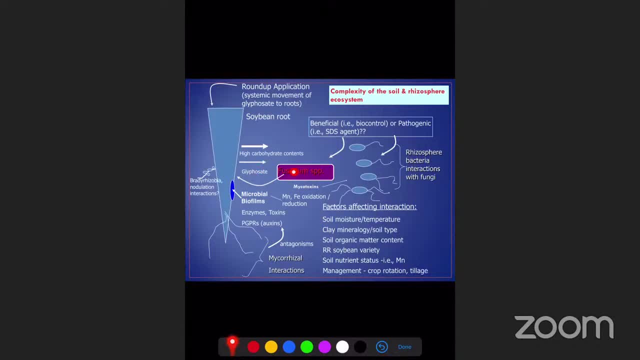 well as glyphosate, And when fusarium type of species comes in their contact they form a type of microbial biofilm which secretes enzyme toxin PGPR, and they secrete such type of mycotoxins which inhibit the growth of other microbes inside them. That's why 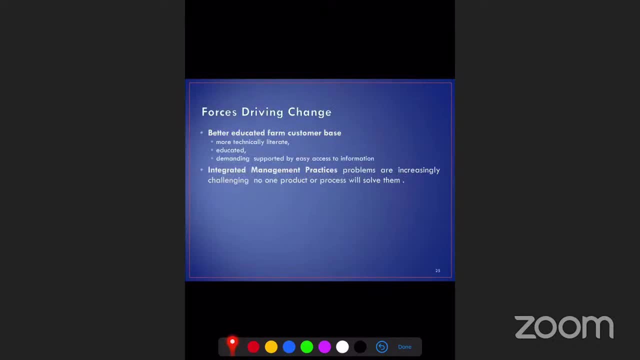 we can say that plant growth promoting rhizobacteria plays a very important role in maintaining the sustainability of the plant. We can say that plant growth promoting rhizobacteria plays a very important role in maintaining the fertility of the soil field And we have just studied, beside that, auxin production. 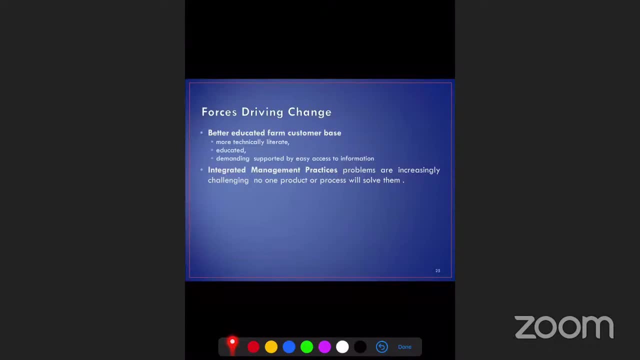 cytopher production and so many other functions is also being carried by them. So what are the forces driving this change? Better educated from customer base, if we are aware, because now it is a time to discuss these things on this international conference and it is not. 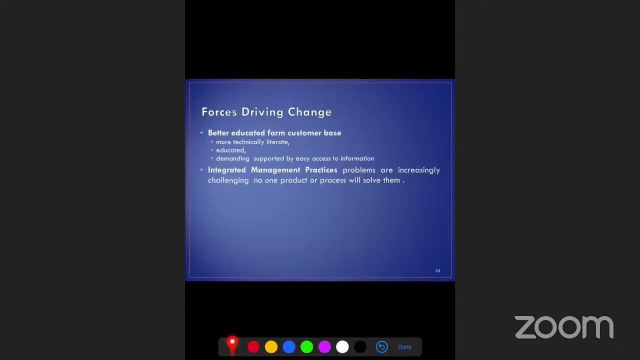 international. It is international. It is international conference That is known as e-conference. The people from Nigeria, the people from Nepal, the people from Banaras- in the university I am present, in the heart of India, that is, in Chhattisgarh. So many people were organizing this event from Rajasthan. 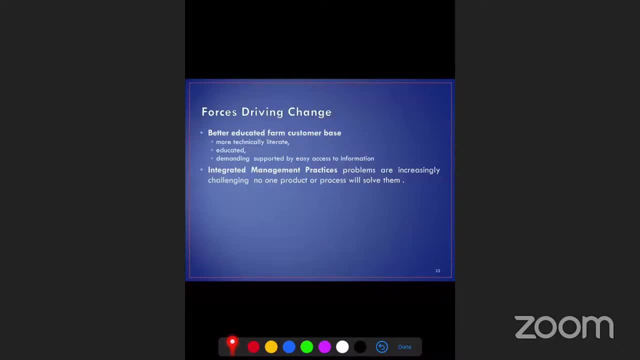 We are aware that we are joined on a Zoom platform and all over we are listening or hearing this program on YouTube type of media. So we have not imagined this before COVID-19.. So this COVID-19 has taught us how to deal with such type of tough situation. Of course, it is a pandemic, but I think this. 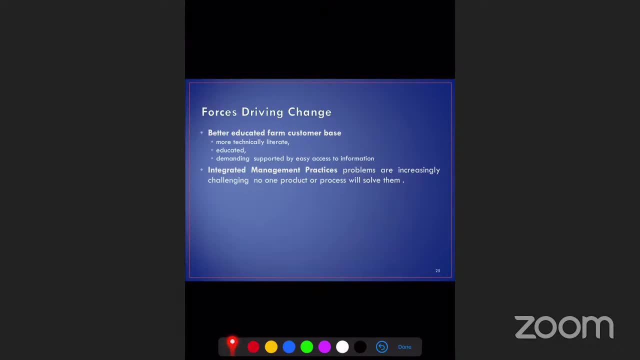 simultaneously it also give a type of boom, for we like people that if you call me at quota, I'm not sure I've come cam or not come. but by this virtual platform we are gathering together, we are talking together. So if we are educated and we are performing such type of farming, 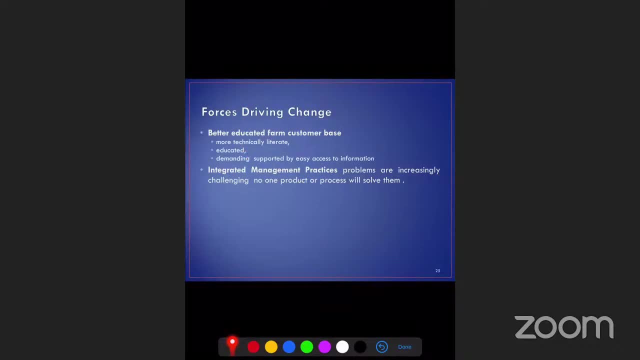 so technically literate, educated, demanding support if such type of things are being used in our agro field. so what will happen? Integrated management practices: problems are increasingly challenged because no one product will prosper In the process. we'll solve them. We simultaneously like that. we are using one thing and on reverse. 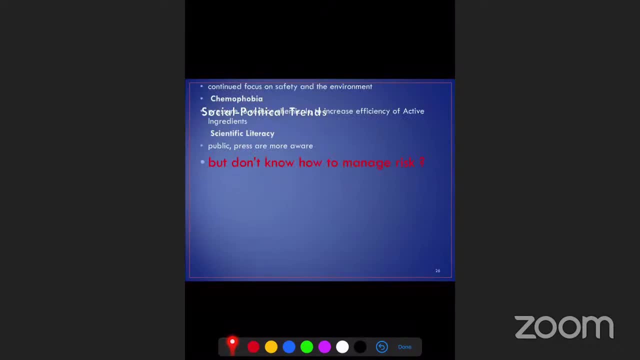 we are getting so many other things. So how we can manage this risk? Because normally we are using fertilizers, and fertilizer- take plant nitrogen, phosphorus, sulfur- all are causing so many type of collateral damage on targeted plants- are also being cu- uh. 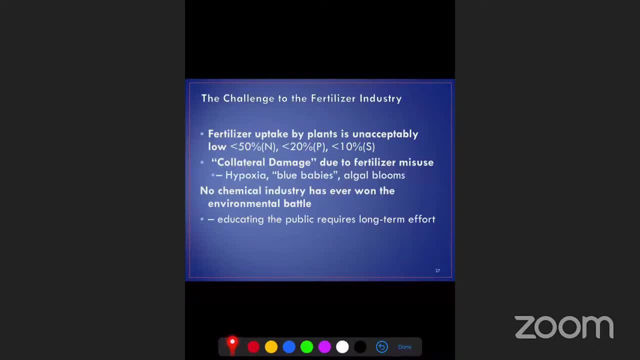 I mean dead, and they are being killed. and hypoxia, blue blebes, algal blooms- all are creating a very dangerous state in our country as well as all other countries. So no chemical industry has even won this environmental battle. If you are using pesticide herbicide. 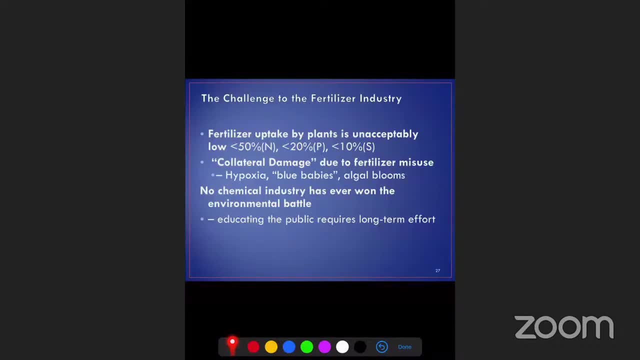 So we cannot say that this is that just now, Prashant Singh sir has told that transgenics- And if you're using transgenic, what will be the side effect is still unknown. Terminating gene technology has come, but how will this solve the problem? 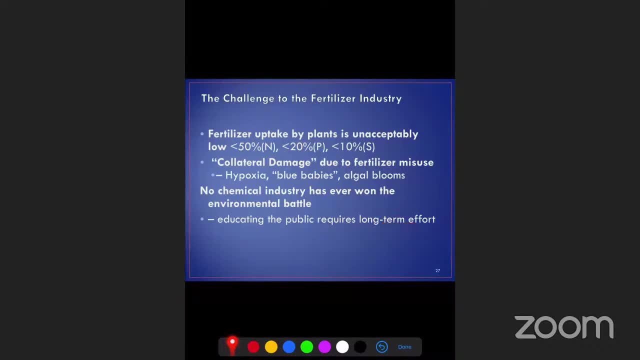 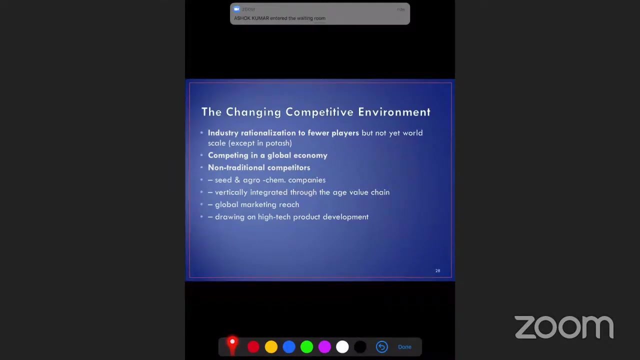 So educating the public, require a long term report. It is not very ordinary process. So in this competitive changing environment we have to develop industry rationalization, compilation of global economy because profit non-traditional competitiveness, Seed and agrochemical companies, vertical integrated and age value chain, global marketing reach, drawing on high tech product development. 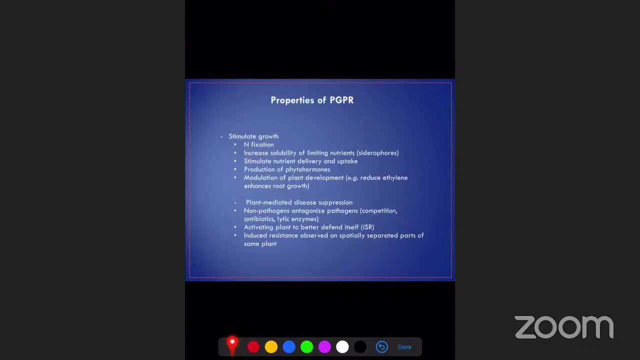 So these things are required and all the solution is given by this plant growth promoting the rise of bacteria because they stimulate the growth. But how? By nitrogen fixation Increases the stability of the plant, Limiting nutrient that is, cytopher, stimulate nutrient delivery and uptake, production of phytohormone modulation and plant development like reduce ethylene in enhances root growth and plant mediated disease separation, non pathogenic antagonism of the pathogen and activate activating plants for better defense itself. 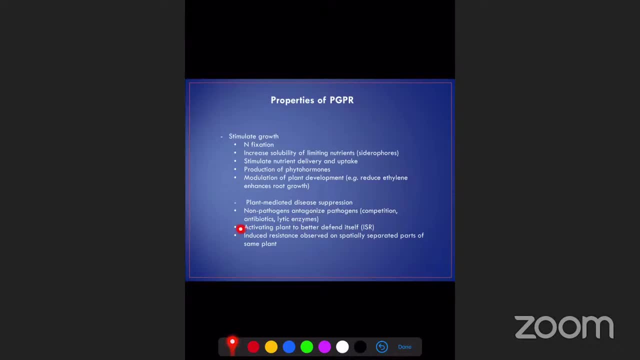 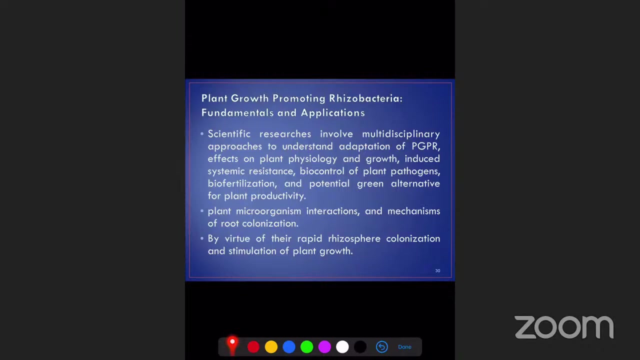 That is ISR And we have just discussed a very important topic by Dr Prashant Singh, sir- And Induced resistance observed on especially separated plant parts and some other plants. So Plant growth promoting rhizobacteria. What are their fundamental and applications? 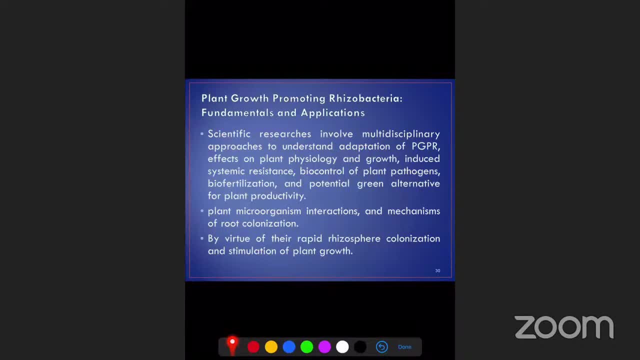 The scientific researches involve multi-disciplinary approaches to understand adaptation of PGPR and they affect the plant physiology and growth, induced systemic resistance, bio control of plant pathogen, bio fertilization and potential green and alternative for the plant productivity. The plant microorganisms interactions and mechanism of root colonization by virtue of their rapid rhizosphere colonization and stimulation of the plant growth, because we know that the most important part of the plant is the root and the colony which is present around them. 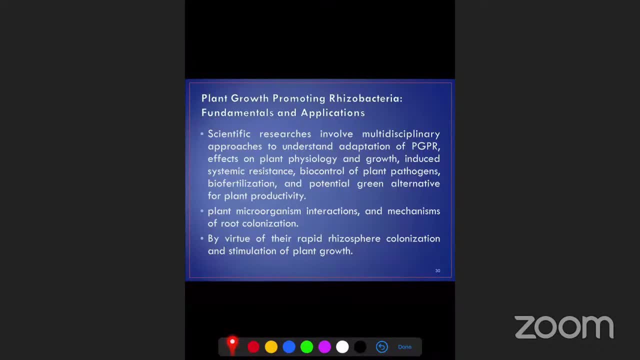 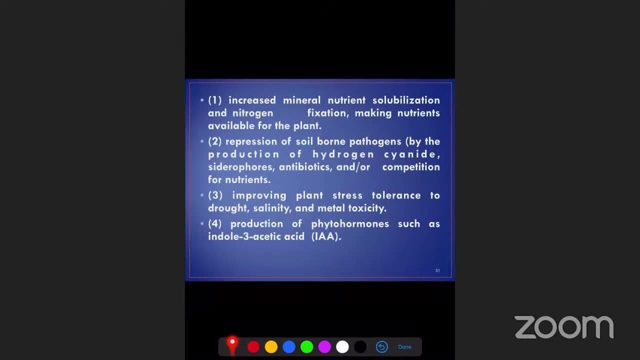 If they provide all the nutrient to the plant, whether it is micro plant or mega plant, a macro fight or micro fight, All are requiring this thing. So it in these mineral nutrients or liberalization like phosphate solubilization, nitrogen fixation and that made the nutrient available to the plant, and the depression of the soil bond, pathogen by production, hydrogen, cyanide, side of force, antibiotics and competition for the nutrient. 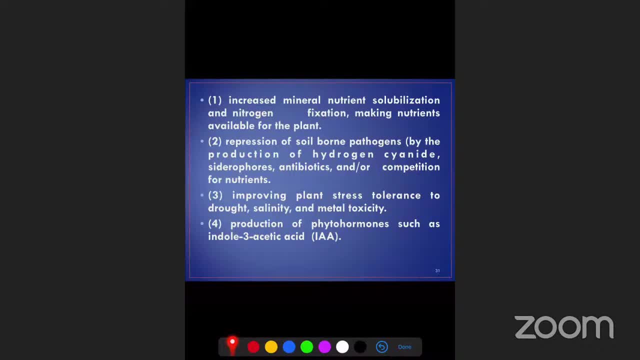 It improves the priority stress tolerance, like drought, like salinity, like materials, metal toxicity and production of phyto-hormones such as indole-lastic acid. and we have seen, because I have completed my two research project of UGC, in which about 16 plant growth promoting 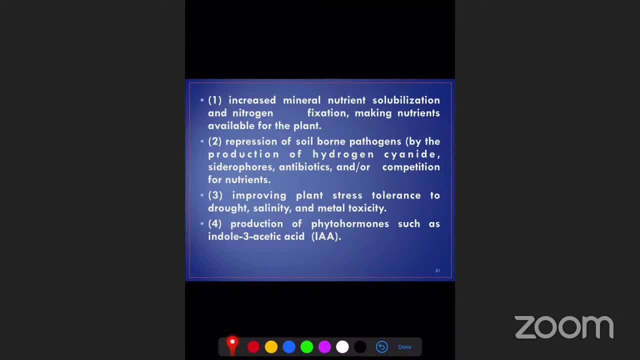 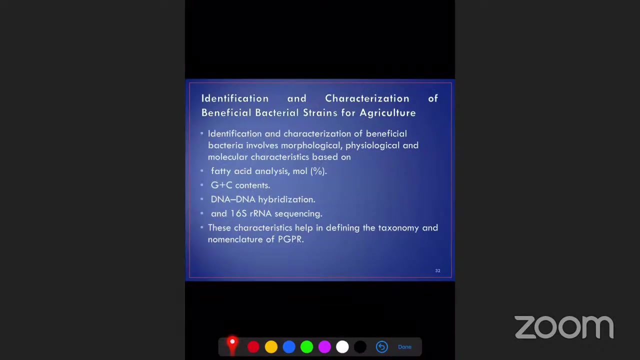 another stress: besides, cyanobacteria is present in my laboratory which is responsible for production of this auxin, which is present or which are synthesized in the green plant at their shoot tips. So how we can identify this bacterial strains which is useful for our agriculture production? So, identification and characterization of beneficial bacteria. 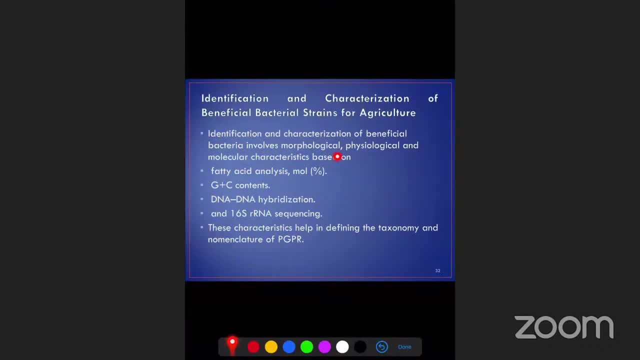 involves morphological, physiological and molecular characterization that is based on these important parameter, like fatty acid analysis by their molecular weight, like we have studied in our first this study delegate. Dr Deba has suggested spectrophotometer and BS Lampert's law, So by this method we can 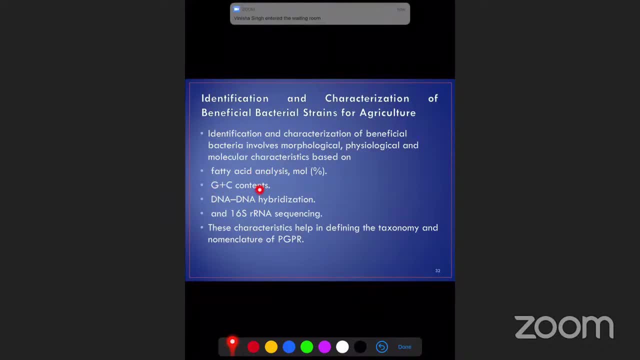 analyze the fatty acid analysis, Guanine cytosine content, DNA-DNA hybridization in situ, GIST-GIS and 16S RNA sequencing, and these characteristics help to defining the taxonomy and nomenclature of the PZPR. As far as the taxonomy is concerned, various approaches has. 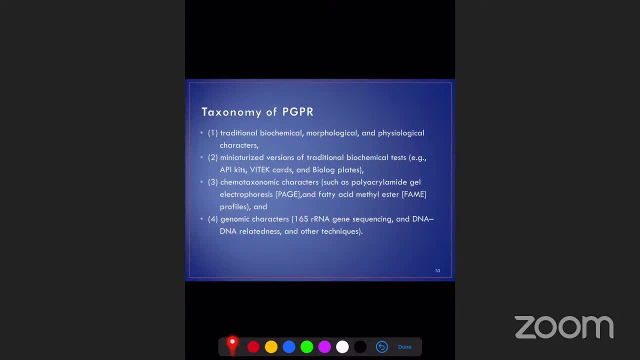 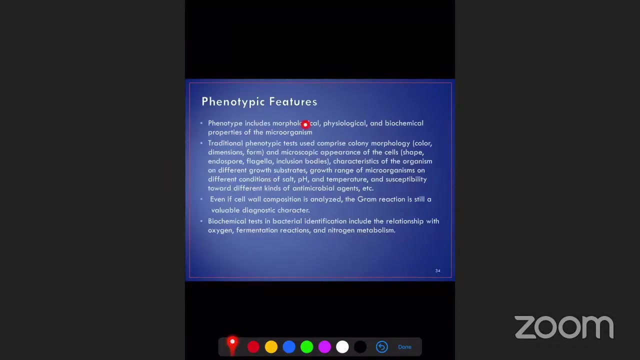 been given throughout the world, even in China, even in Vietnam, even in India. A lot of our worker, even in BHU, Dr Vesampayan sir, Dr RP Sinha sir, is working in this direction. And as far as the phenotype is concerned, phenotype includes their morphological 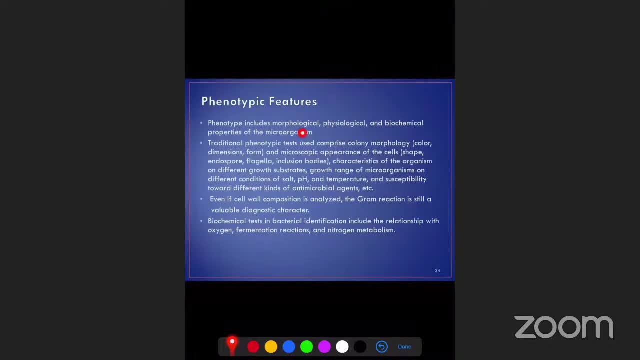 physiological, biochemical properties of the microorganism. The traditional phenotype test used comprises colony morphology, microscopic appearance of the cell and even cell wall composition is also very much analyzed because gram-positive, gram-negative, such type of gram reaction is also available. diagnostic character We are taking 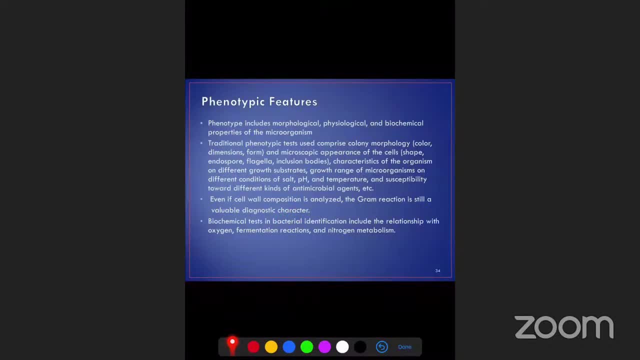 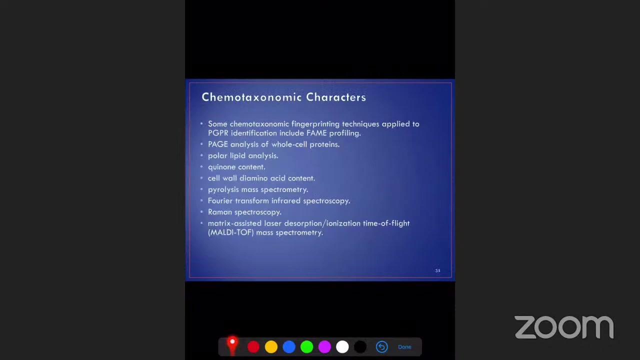 13-15 parameters for this. how to biochemical analyze. So biochemical test is also being performed for their relation with oxygen fermentation reaction and nitrogen. So there are many different approaches to this type of metabolism As per the chemotaxonomic character is being concerned. some chemotaxonomic fingerprinting. 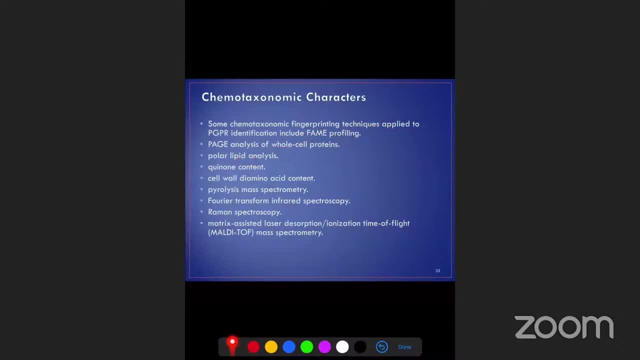 technique applied to PGPR include FEM profiling, pH analysis, polar lipid analysis, O9 content, cell wall di amino acid content, paralysis, mass spectrophotometry, fourier transform infrared spectroscopy, Raman spectroscopy and above all this MALDI or TOF. 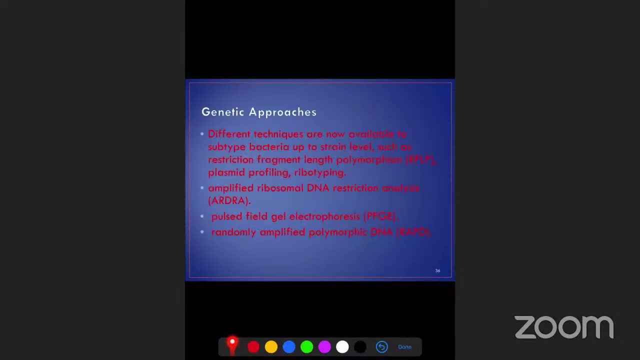 is also being used. As far as their genetic approach is being concerned, different techniques are now available to subtype bacteria up to strain level, such as RFLP, that is, restriction fragment length, polymer polymorphism plus bead profiling and ribotyping. That's why we have talked about this 16S ribonucleotide sequencing and ADRDA, that is. 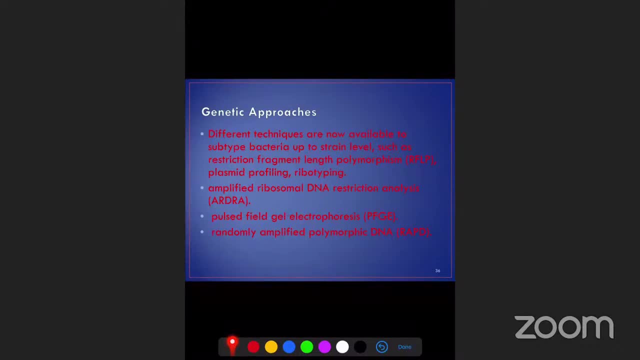 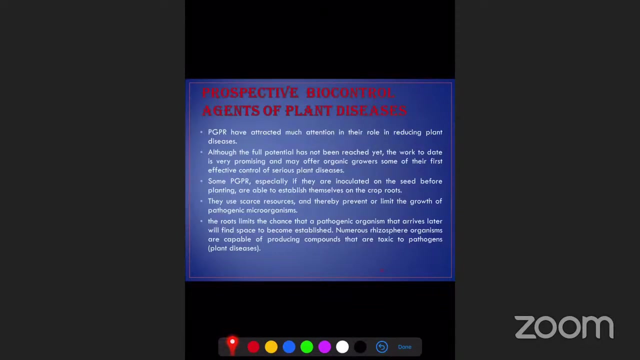 Amplified Ribosomal DNA Restriction Analysis, Pulse Filled Gel Electrophoresis, that is PFGE, Randomly Amplified Polymorphic DNA, R8PD, So the prospective biocontrol agent, because these natural microbes which are growing in. 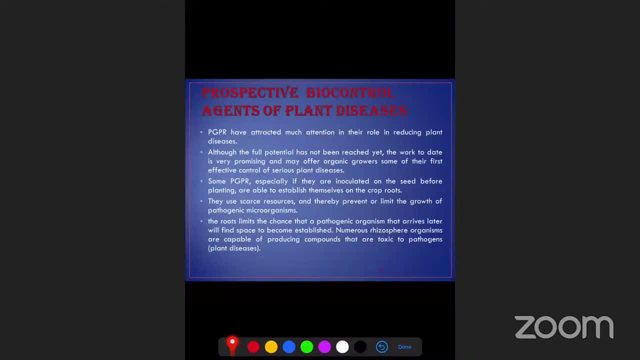 the nature automatically. we are not responsible to sow, harvest and cut and re-harvest. They are present naturally in our soil, They are present with but we are treating by untargeted chemical phobia type of agent, like fertilizers, like pesticides. 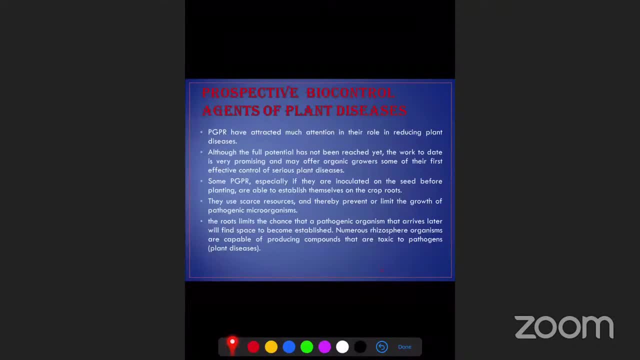 So they're innocent, they're prokaryotic creature. They are situated for giving benefit to you type of people, we type of people, But we are giving them such type of doge untargeted. they will be killed And the most important soil profile is being changed. 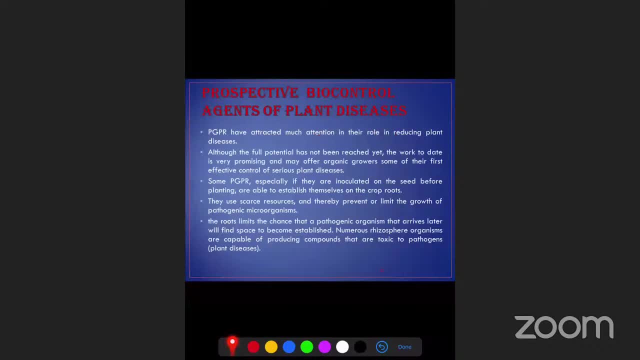 And so This PGPR- have attracted much attention in their reducing plant diseases because, just in case of Fugirium- and I'm giving you a long list in which peoples are working and they have given a list so that so many diseases can be controlled by the help of this PGPR- 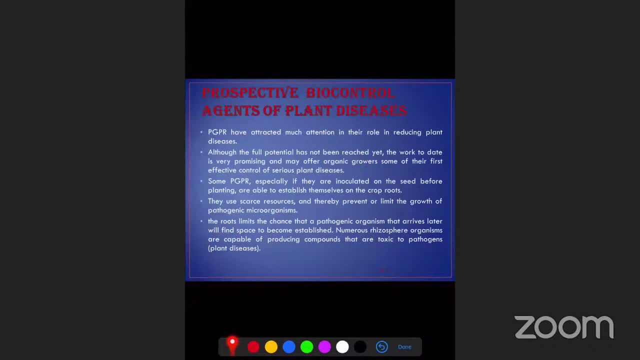 Although the full potential has been reached it and not reached it, the work to date is very promising and very offer organic growers, Some of the first, effective control serious plant diseases, Some PGPR, especially if they are inculcated on the seed before planting, because they 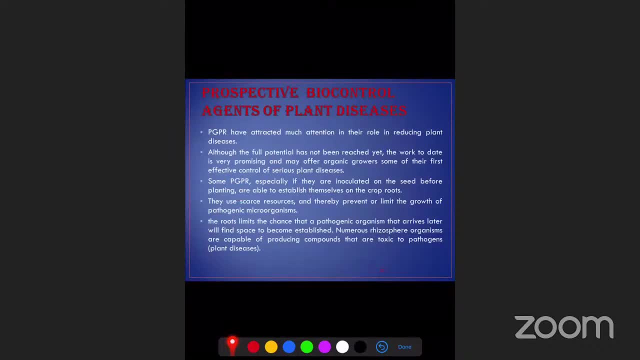 also enhance germinating capacity And we know that the there are few hormones which are responsible for seed germination, So they also perform such type of things. So use of source resource, thereby prevent, limit and growth of the pathogenic microorganism. 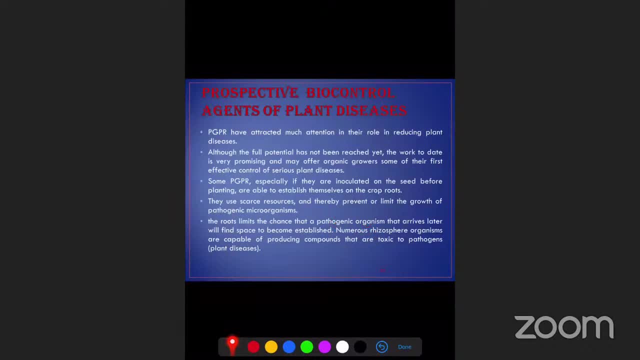 the root limit the chance, the pathogenic organism that arrive later We'll find a space to become established. Numerous organisms are capable for producing such type of compound, which is toxic to pathogen, So they can inhibit the plant disease, As, for example, bacillus sub stylists is one of the commercialized PGPR organism and it 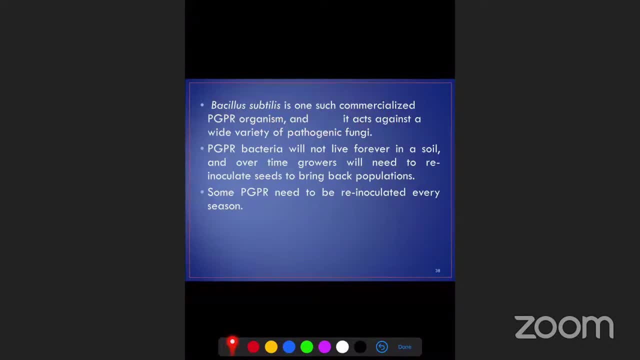 acts against a wide variety of pathogenic fungi, So you can use this even by culturing, even in your laboratory and PGPR. bacteria will not leave forever In a soil and over time grower will need to re-inoculate seeds to bring back population. 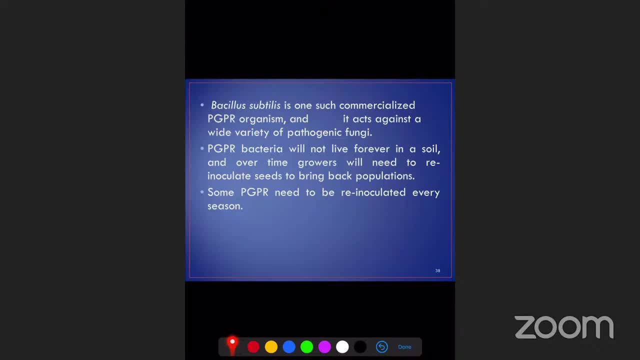 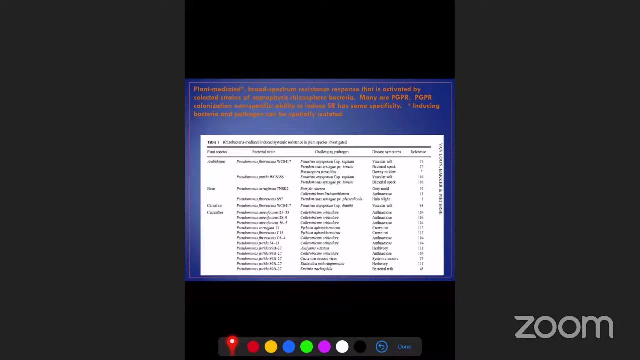 Some PGPR need to be re-inoculated in every season, Because in our Chhattisgarh the chief minister has put a slogan: we should conserve our body and by conserving our body or our farmland we should use such type of few strains and 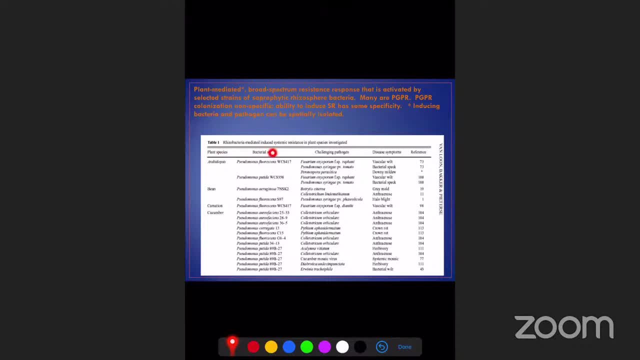 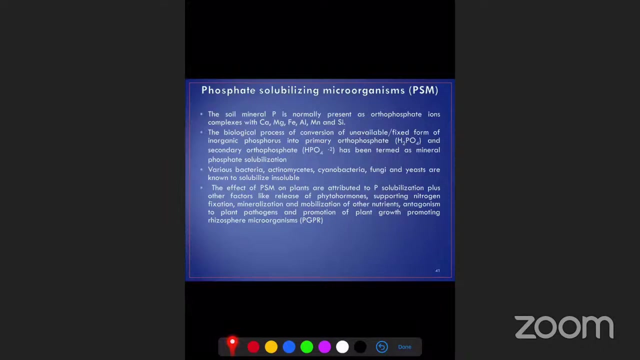 see, they are the plant species, They are the bacterial strains, they are the challenging pathogen. These are the disease symptoms and these are the different races reference which controls such type of diseases. Okay, Next is phosphate solubilization. 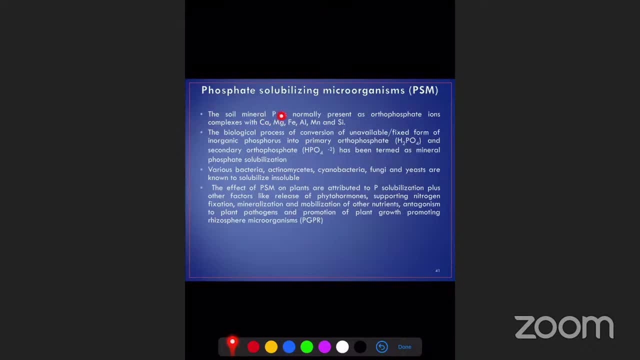 Phosphate is a very important mineral and usually present in the form of orthophosphate, iron and combined with calcium, magnesium, iron, albumin, magnesium, silica, And they are responsible for solubilization of this phosphate. So we have not put too many fertilizers within our farmland. rather, we can use such type. 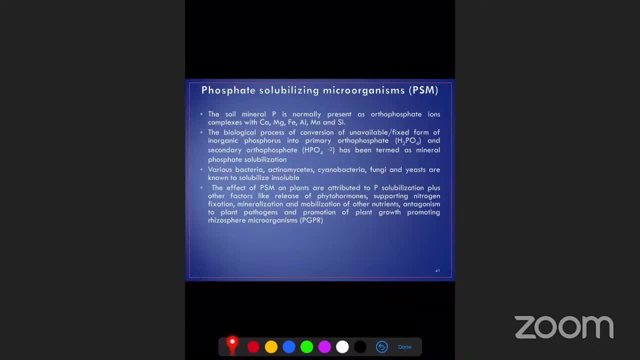 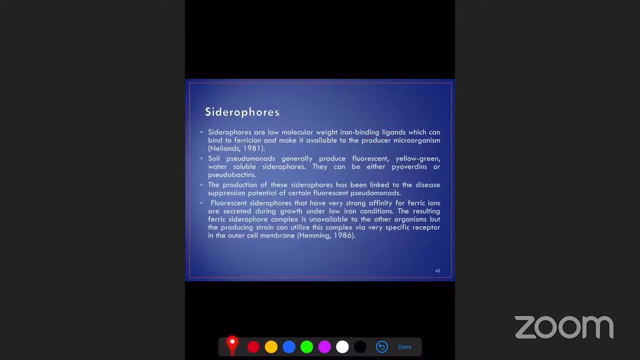 of PGPR and they perform this work. Similarly, cytophor. cytophor are low molecular weight iron binding lesions which can bind ferricione and available to the producer of them. This was a very important And Pseudomonas. 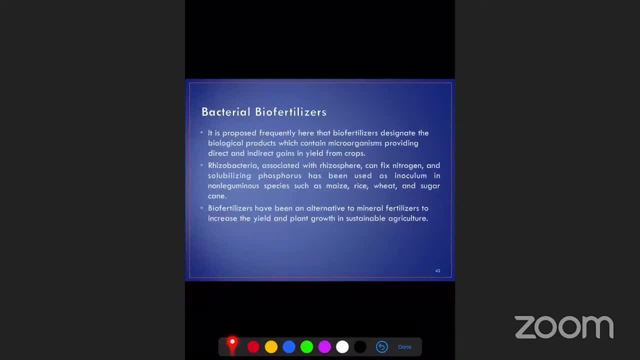 That's type of agents were responsible for such production: Bacterial biofertilizers, because these biofertilizers can be also used- this rhizobacteria, brandy rhizobium and so many other types of rhizobacteria which are present in soil, and they give a type 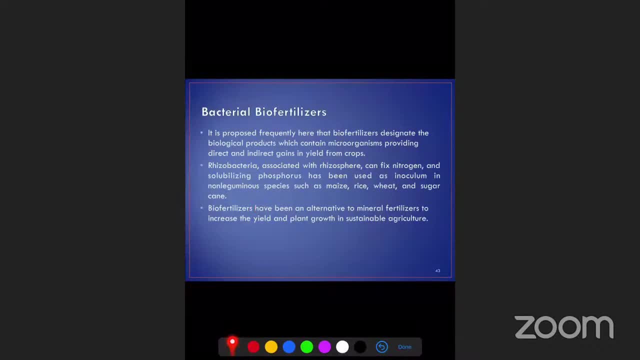 of biofertilizers type of effect, So this will enhance our fertility and they will create sustainable development to our agro field- organic farming. So one of the challenges of using PGPR is natural variation because, due to rapid industrialization, modernization and chemical use, chemophobia type of things, their natural variation is. 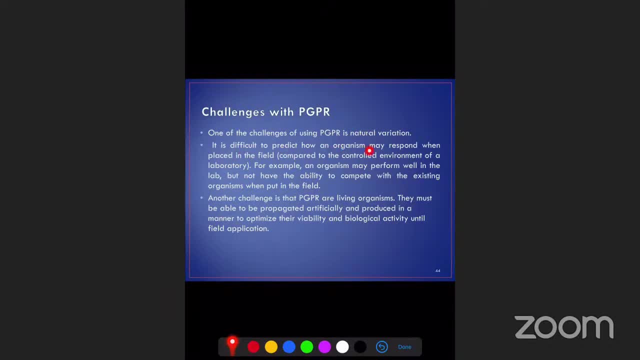 also being seen. So it is difficult to predict how an organism may respond. And if we are not in position, we have to say that an organism may perform well in life lab but not in the agriculture field, because we have also seen some student who is performing. 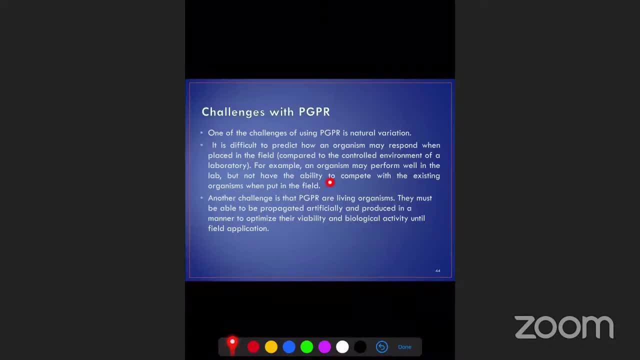 very excellent in the class, do not perform very well in examination. Similarly the laboratory and field report. they should not coincide with each other. so we have to perform this experiment repeatedly, repeatedly. and another challenge for PGPR living organism: they must be able to propagate artificially so their for viability, their biological activity and for their field. 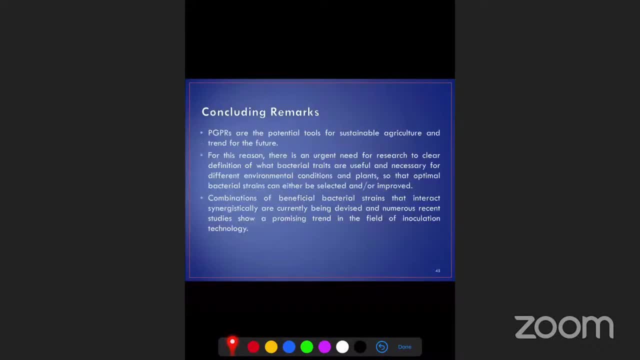 habit. we should be very aware and, as per the PGPR, as biopotential tool for sustainable agriculture and for it is a train for the future. that's why I have taken this topic: biopotential PGPR, because those microbes which are not visible power, ie naked eyes. 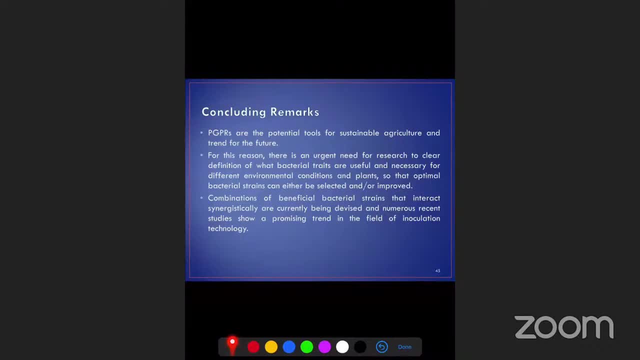 the macrophages which are not visible. power- ie naked eyes, macrophages which are not visible. power- ie naked eyes, macrophages which are not visible. power- ie: naked eyes, macrophages, everything, everything is going for them, but we should conserve our some limit, some knowledge, such as saving methodology. 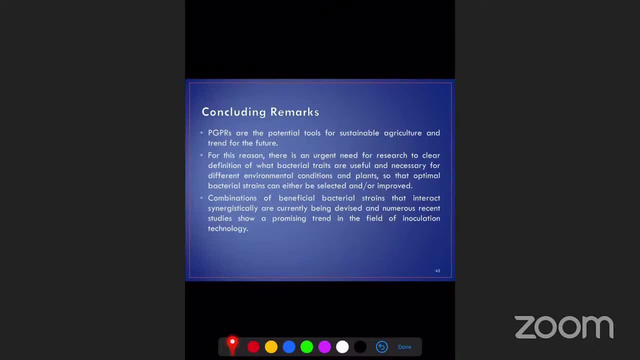 for preserving them, So they're the potential tool for our sustainable agriculture. For this reason, there is a urgent need for research to clear definition to what bacterial is useful and necessary for different environmental condition and and plants, so that optimal bacterial strain can either be selected and can be improved, like 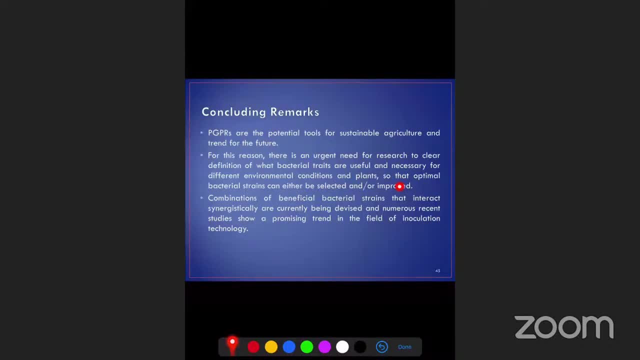 bioremediation, because so many cyanobacteria strain even I mean responsible for I mean reducing the concentration of mercury and so many heavy metals. So, if you are using such type of things, because even our Deba Bahadur sir has told so many heavy metal contamination in the water, 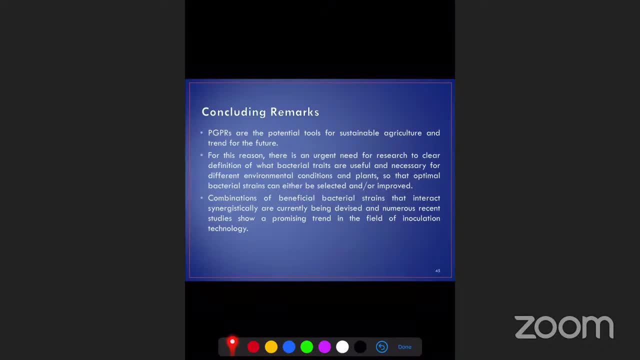 So they are present in the soil and they can reduce such type of contamination also, and lot of research papers are also present regarding this. So combining the beneficial bacterial strain that interacts syngenistically are currently being devised and numerous recent studies has so promising trend in the face. 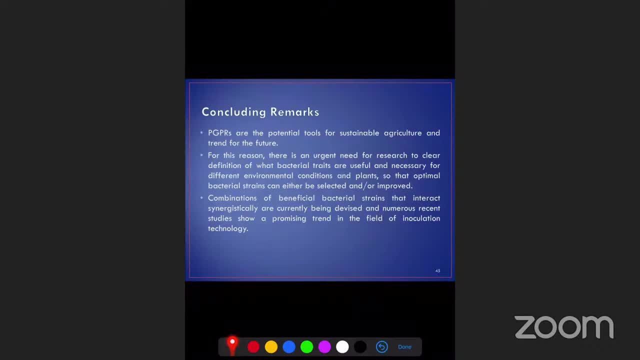 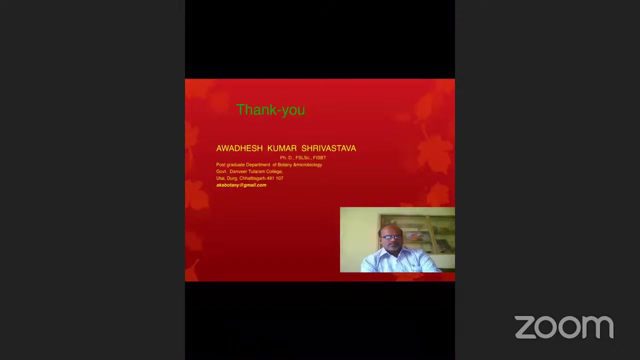 So we should either use this as the natural harbour of the soil or by artificial inoculation, by culturing them in the laboratory, and this is all about, for my information, I think I was able to say something about this sustainable development, If I have told you. 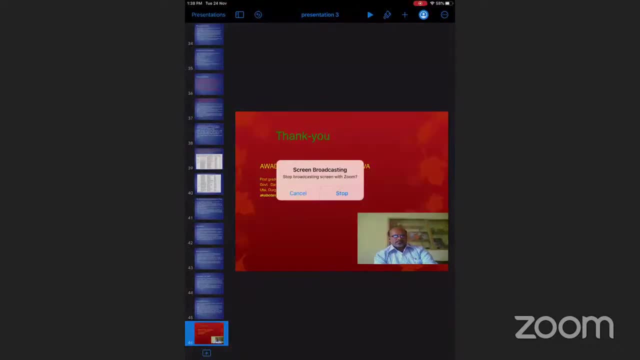 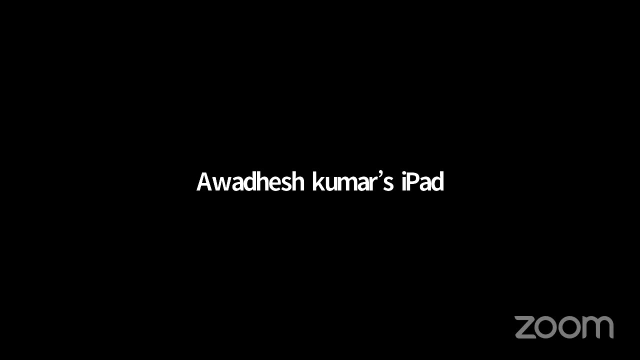 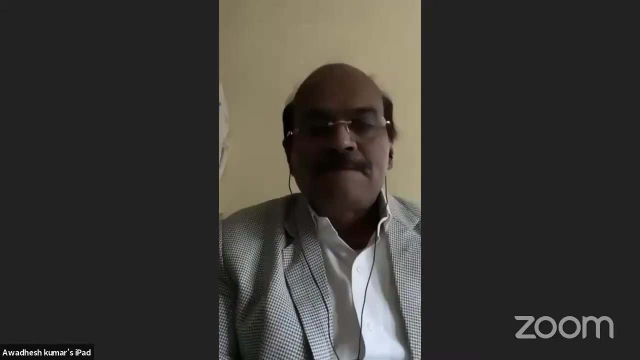 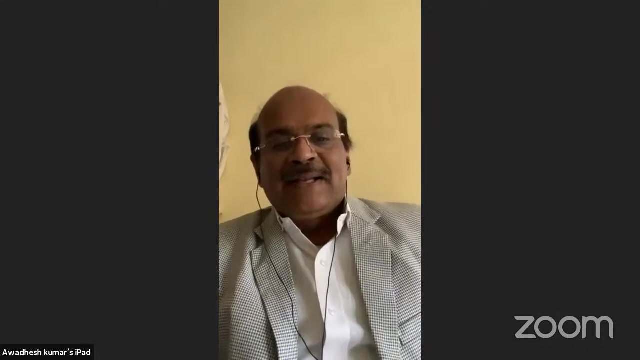 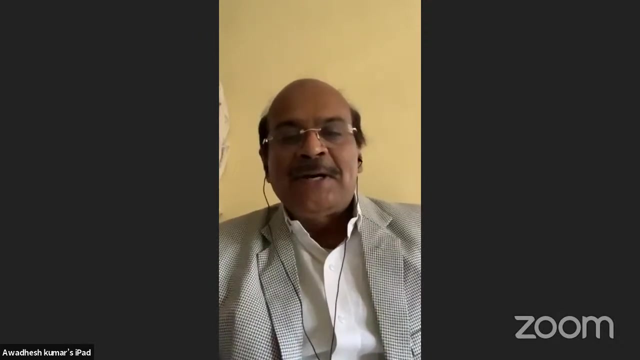 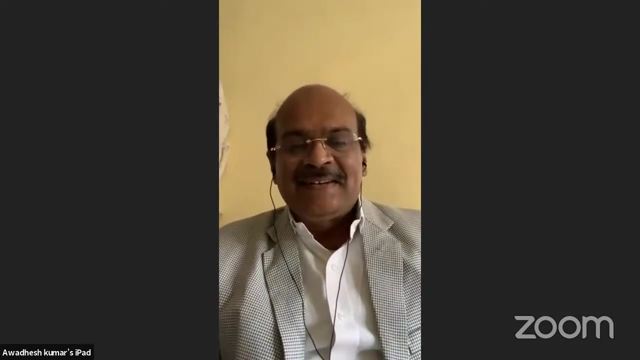 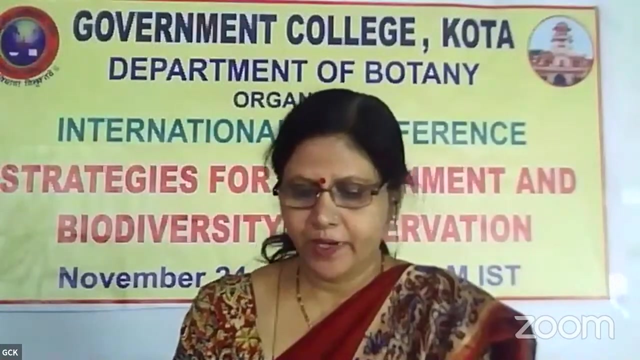 then I was successful. Thanks to all of you who has given this opportunity, and I really enjoyed much with today's participation. Thank you very much, ma'am, Over to you. Thank you for sharing the knowledge, sir. Really your lecture was innovative and interesting. 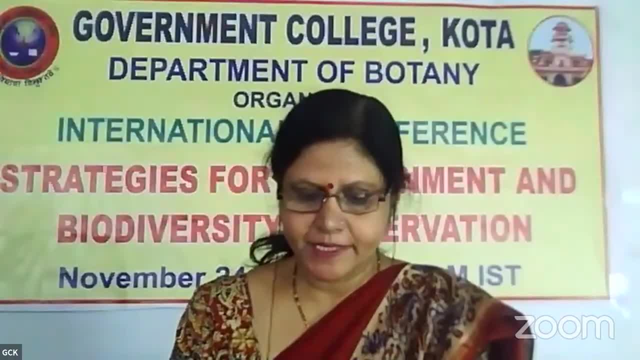 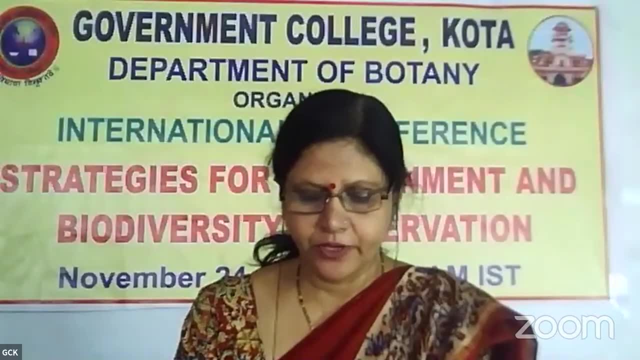 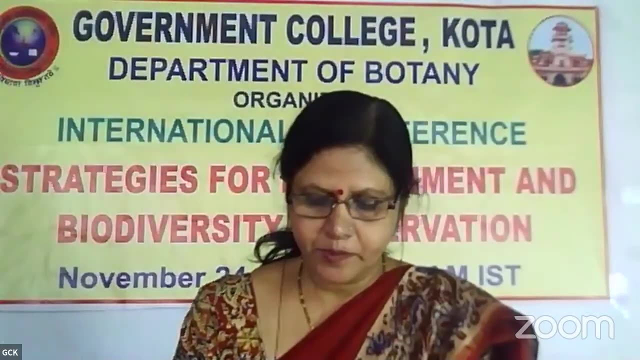 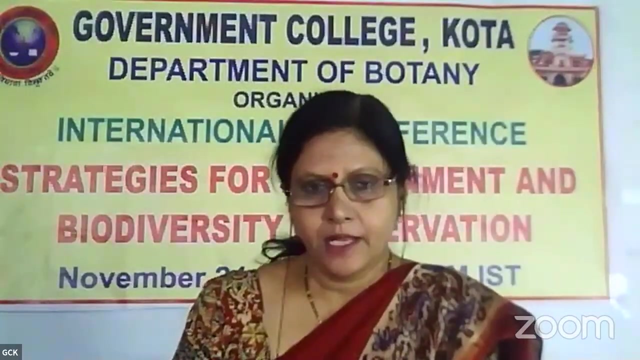 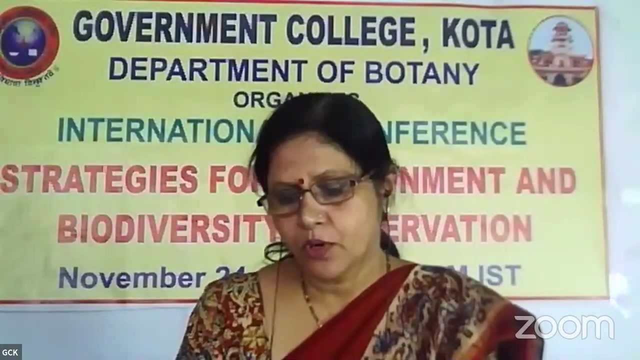 Soil fertility is decreasing day by day, but it is maintained by biopotential. Livestream is responsible for nitrogen succession And cyanobacteria. how to promoting agro-field and maintain sustainability and fertility to field. Sir, your lecture was, I conclude, how to go green agro-field through PGDR. Thank you, sir. 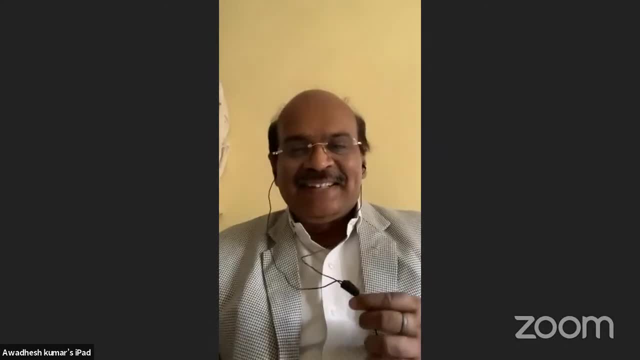 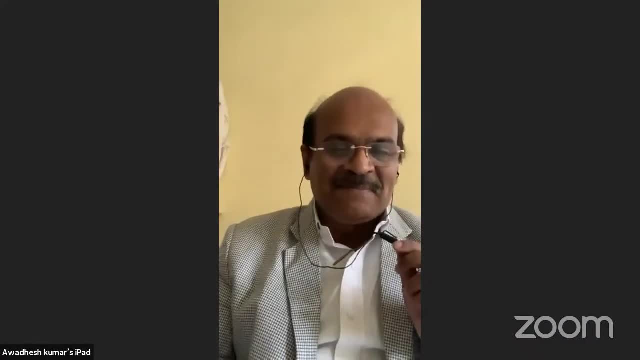 Now the verklp is challenging. pathelujah, Yeah, Thank you, Hague B' Scary tak, Thank you, Ms. Thank you, Ms The Nose King. Now I Mclàes Mcoth, Mc orth, Okay, Mcoth. 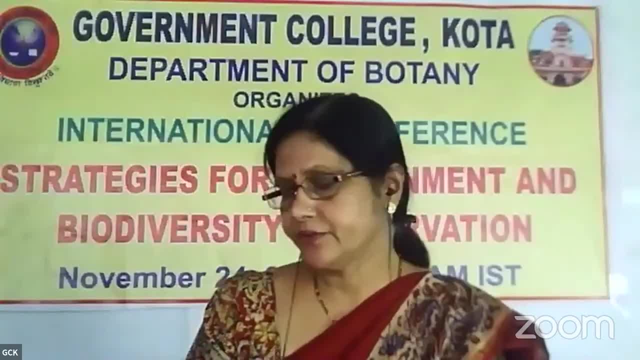 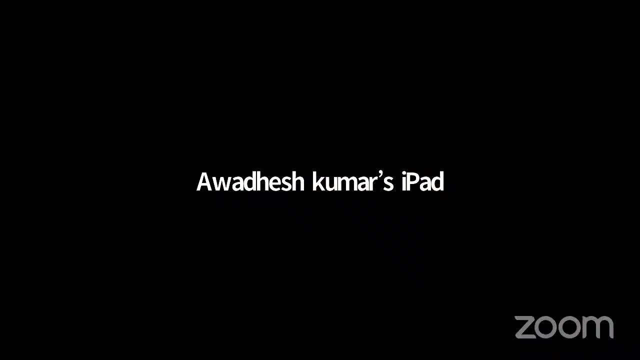 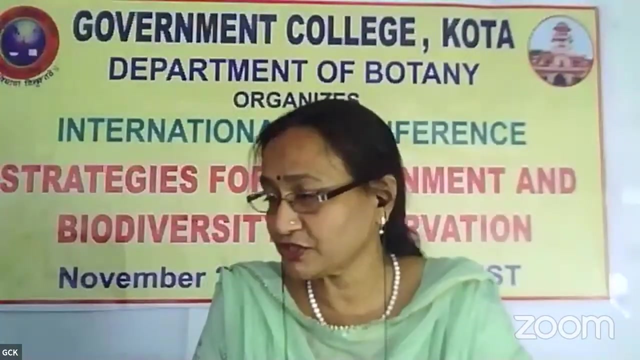 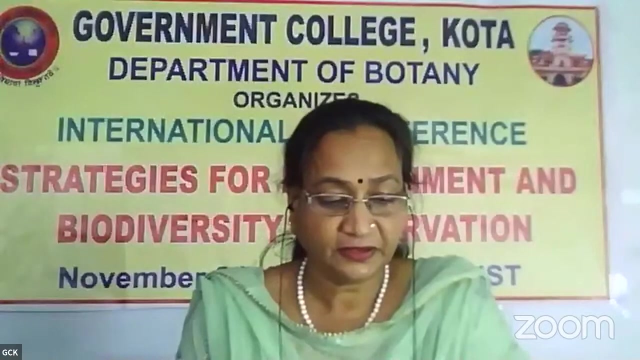 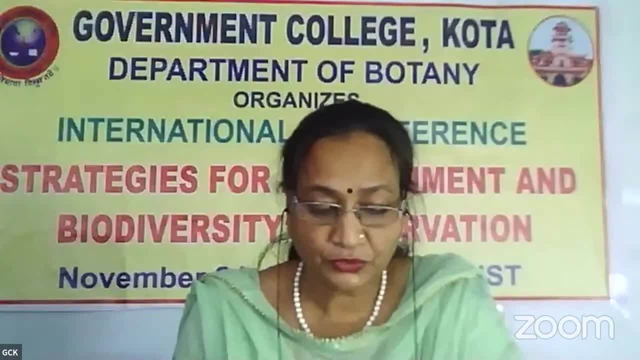 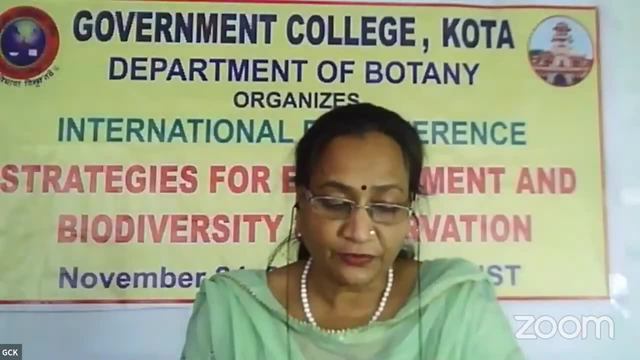 informative day. It is my privilege to deliver this vote of thanks on behalf of Department of Botany, Government College Kota. First and foremost, I would like to express our gratitude to our eminent speakers, Professor Deba Bahadur Khadka from Thirubhuvan University. 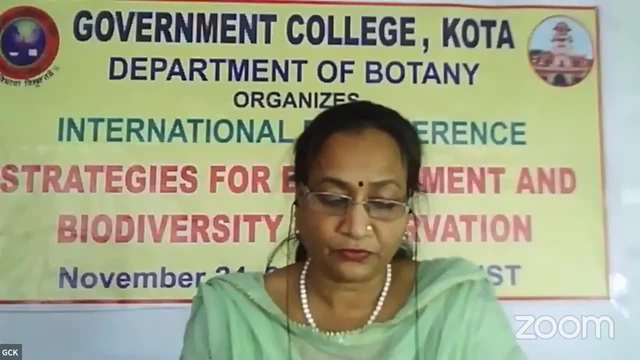 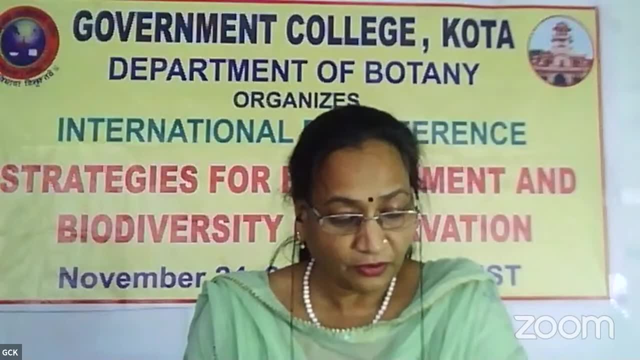 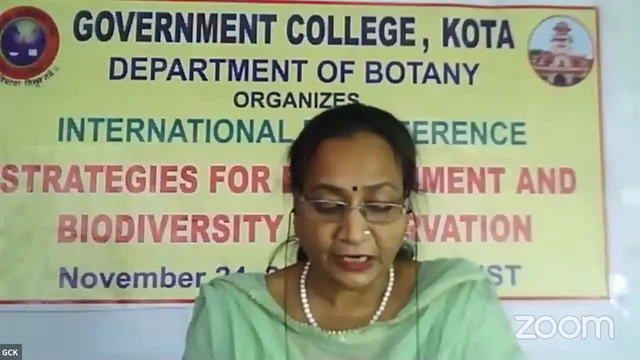 Kathmandu. Dr Varla Andrew Venkar from Imul State University, Nigeria. Dr Prashant Singh from DHU Varanasi and Dr Avdhesh Kumar Srivastava from Durga. Dr Deba Bahadur Khadka, their valuable insights into biodiversity and conservation. 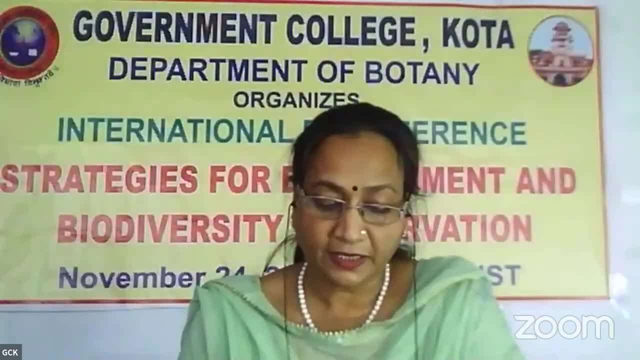 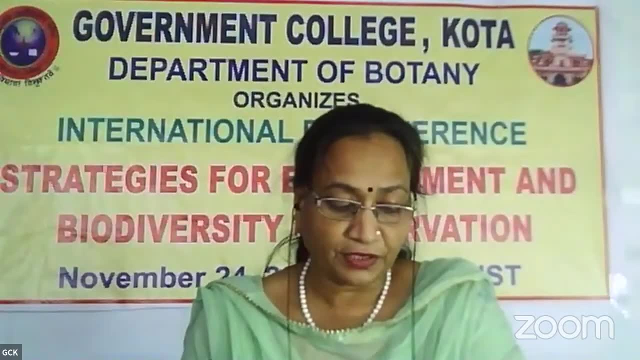 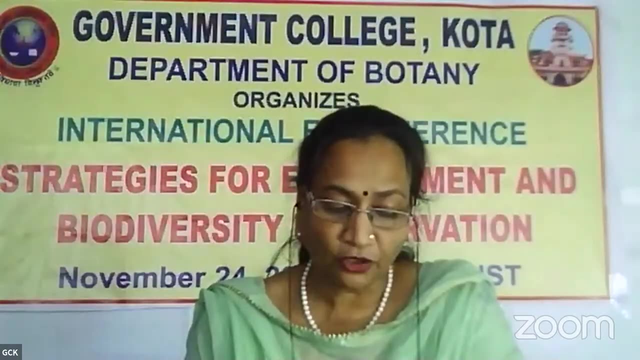 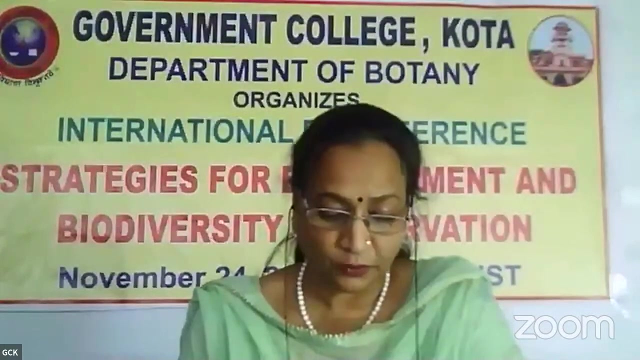 green vaccination, role of PGPR in agro-fields and effect of chemicals on biodiversity have given us a lot of food for thought. It has been wonderful to hear the views and opinions of these scholars on these topics. I would also take this opportunity to thank our special invitee, Dr Sanjay Bhargava. Assistant Director. 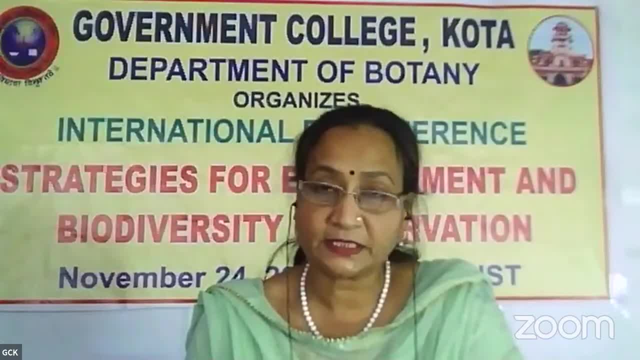 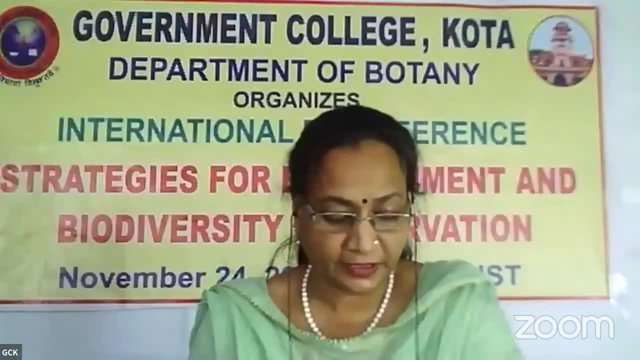 College Education for gracing us with his presence and thoughts. This event would not have been possible without the support and valuable guidance of our respective principal, Dr Jayanthi Jivarghia. I would also like to thank Mr R R Parihar, Zonal Secretary. 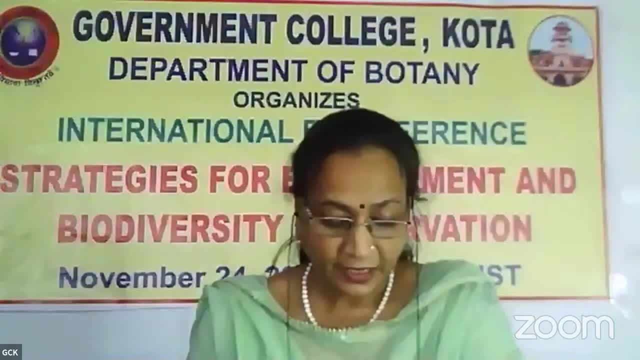 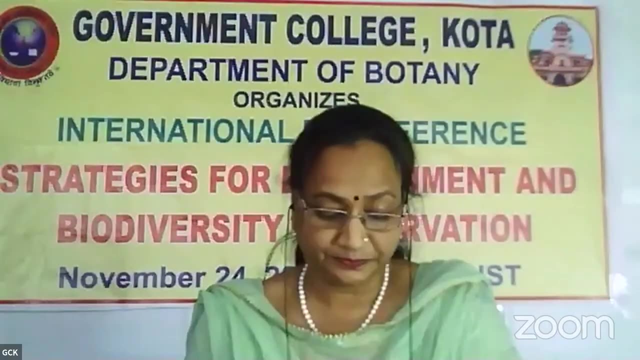 AI Phukto, for his cooperation. It was the vision and tireless effort of the head of the department, Botany Anju Kapoor, that has made the successful completion of this conference possible. We are also thankful for her contribution to this endeavor. I would